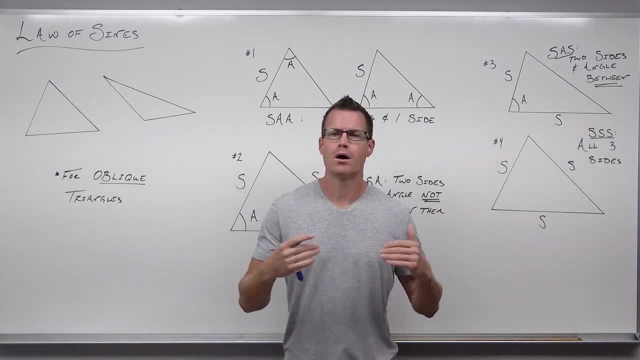 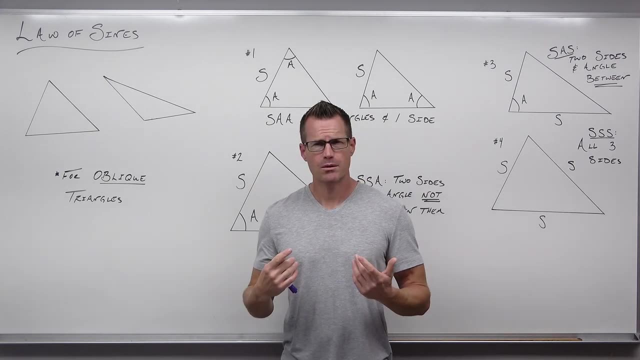 angle sum, that's great, Or the law of sines or the law of cosines. So we'll deal with the law of sines right now. We'll talk about the types of triangles you can get besides a right triangle. We'll talk about this idea, if you know. 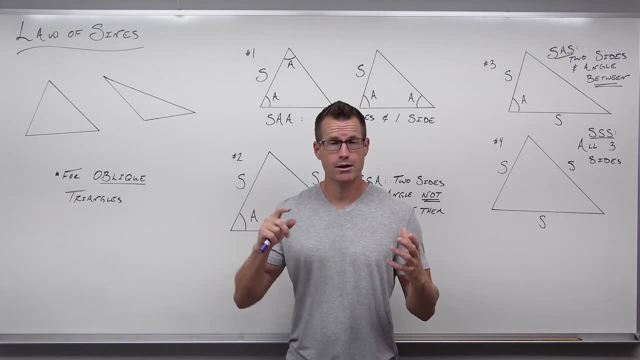 two things in a triangle you can find a third, and how that changes just a little bit when we're talking about a non-right triangle, how you need to know three things, to know a fourth and why in the world that is So. firstly, what are these non-right triangles called A non-right triangle? 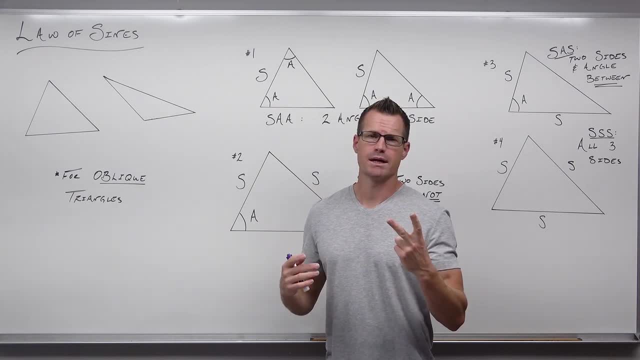 is called an oblique triangle And really you can have two cases. Honestly, in all of triangles you will only have three cases. You can have one right angle, You can have all angles less than 90 degrees or one angle greater than 90 degrees. The triangle: 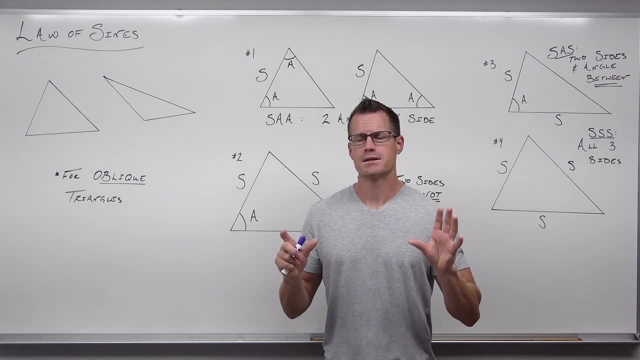 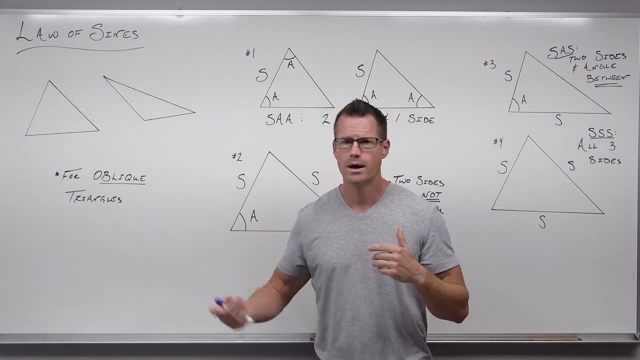 with a right angle is called a right triangle. But the other two cases, if you have no 90 degree angles and all of them are less than 90, you have what's called an acute triangle. They're all acute angles. Or you could have a triangle with one obtuse angle, So all acute are all less than 90.. 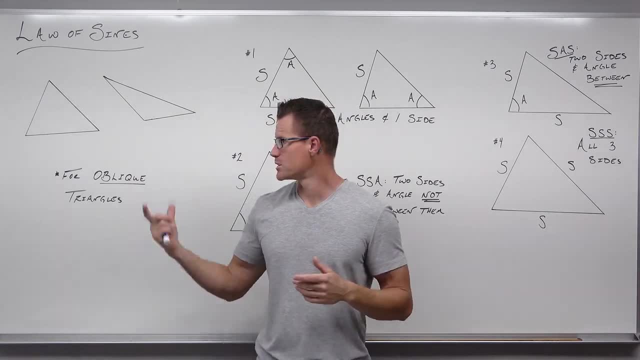 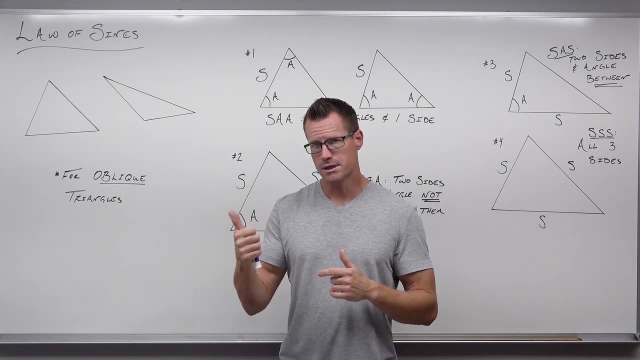 One obtuse would be one more than 90. And that's really it. Those are the two cases of oblique triangles that we can get. So when you're categorizing this, oblique triangles are solved with law of sines or law of cosines. 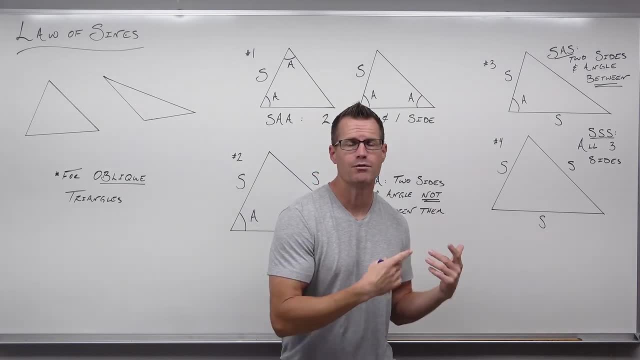 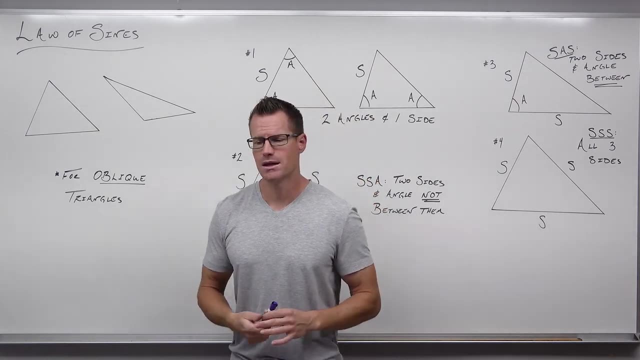 Right triangles are solved with our right triangle trigonometry. we've already covered, So we needed to know something else, because right triangle trigonometry does not work for oblique triangles. That's why we got this law of sines and law of cosines. So the first thing is: when do they work? 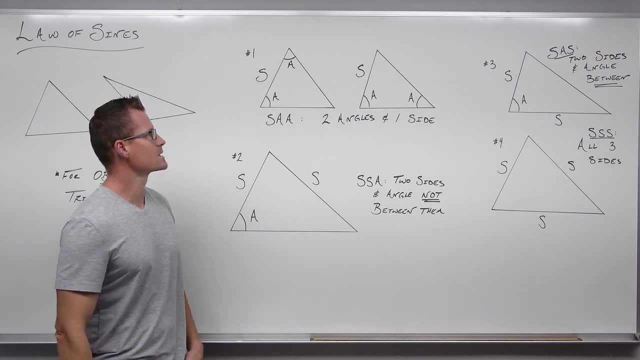 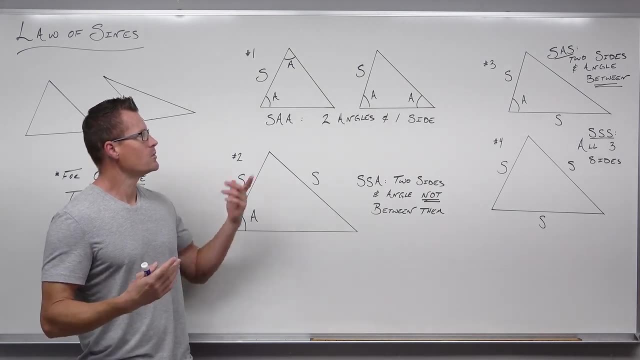 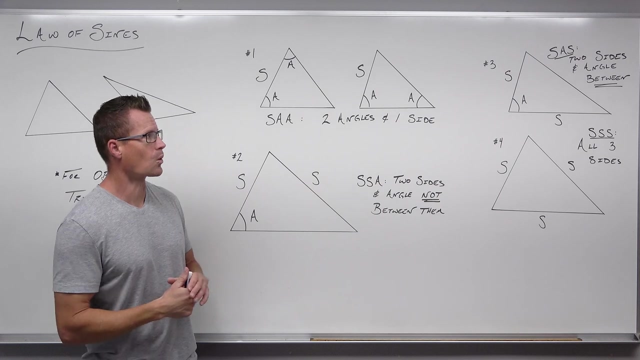 Well, there's really four cases, Four cases of these oblique type of triangles that we can solve. The first one is: well, what if you know two angles in one side, or one side and two angles? What if you know two sides in one angle, or all three sides, or two sides in an angle, but the angles between the two sides 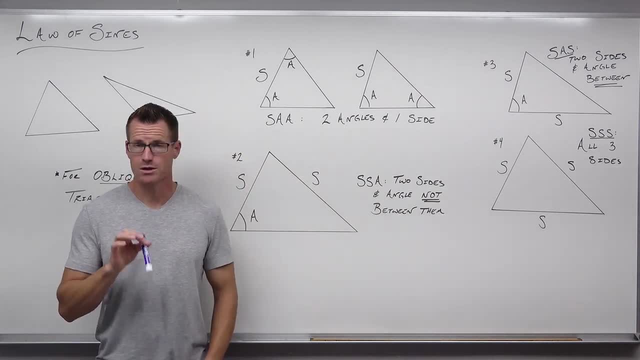 Those sides would be adjacent to the angle. These are the four cases that we can solve with law of sines and with law of cosines. Now I mentioned something a little while ago. I said that in right triangle trigonometry you need to know two things to find a third. 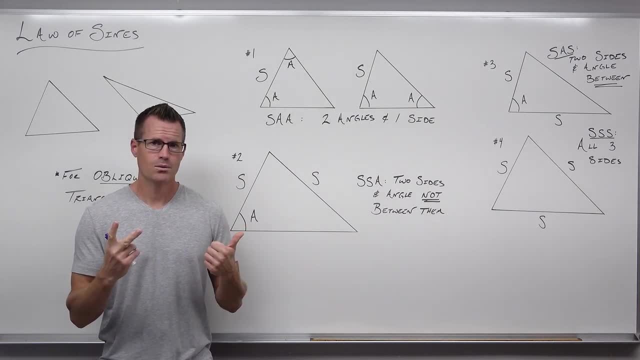 Like you would need to know two sides to find an angle or an angle and a side to find a missing side. Those are the two things you would need to know. You would need to know two sides to find a third. But really, if you think about right triangle trigonometry, you already know one thing. 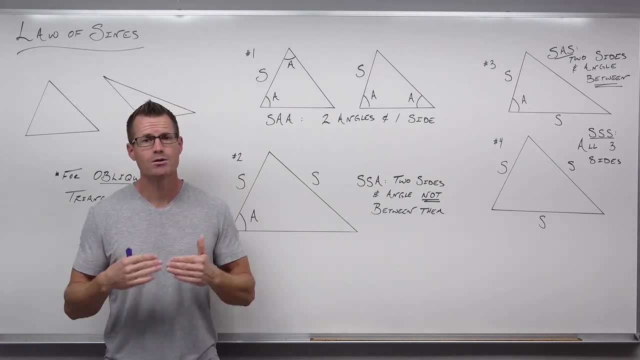 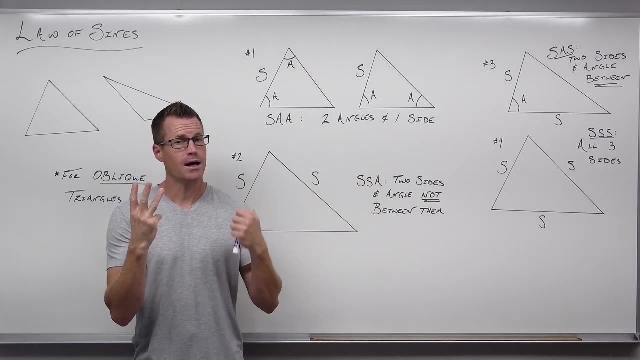 In a right triangle, you would already know one angle. You would know a 90 degree angle. So really, in right triangle trigonometry, you need to know three things in order to find a fourth. You need to know it's a right triangle. You need to know an additional angle and an additional side in order to find a fourth side. 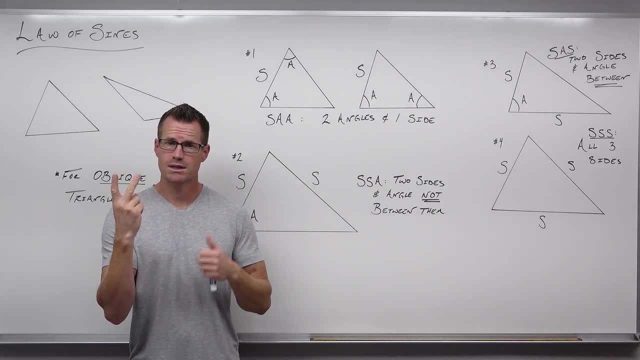 Or you need to know 90 degree angle, You need to know two sides in order to find a missing angle, And so, really, because you already know it's a right triangle, it kind of reduces that to: oh, I need to know two things to find a third. 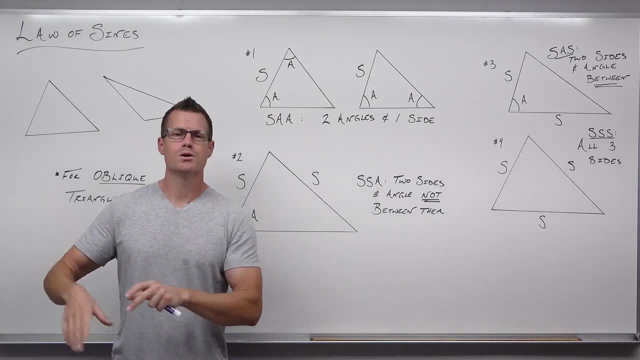 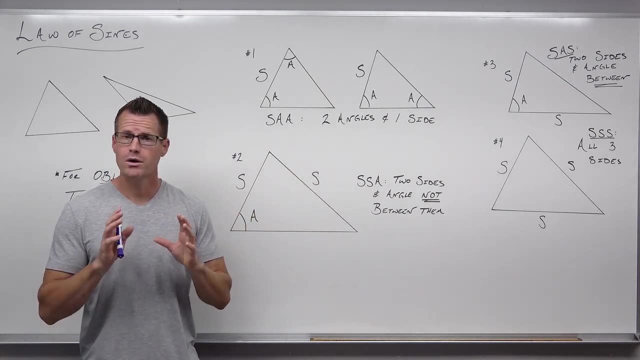 But in right triangle trigonometry- remember you already know it's a right angle. So you know three things to find a fourth. That's exactly where we find ourselves in law of sines and law of cosines With non-right triangles. you need to know three things in order to find a fourth thing. 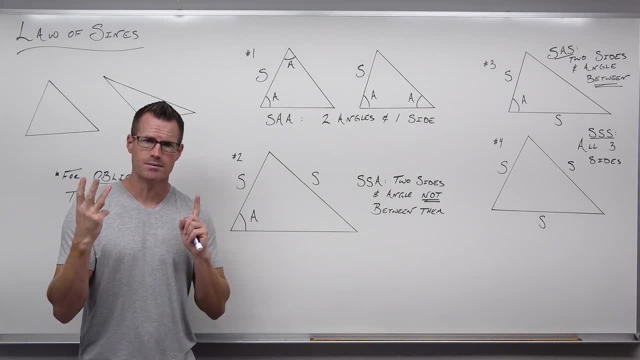 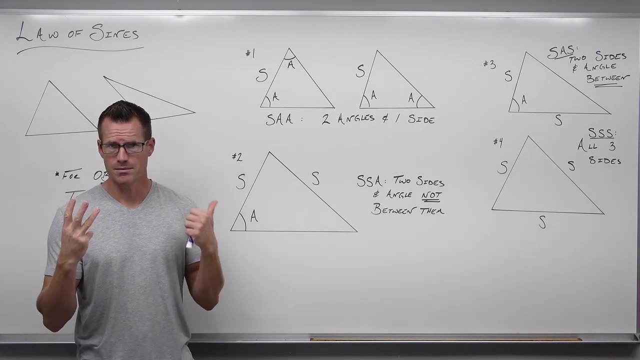 You need to know. You need to know two angles and a side to find a missing side. You need to know two sides and an angle to find a missing angle. You need to know all three sides to find a missing angle. So those are our cases here. 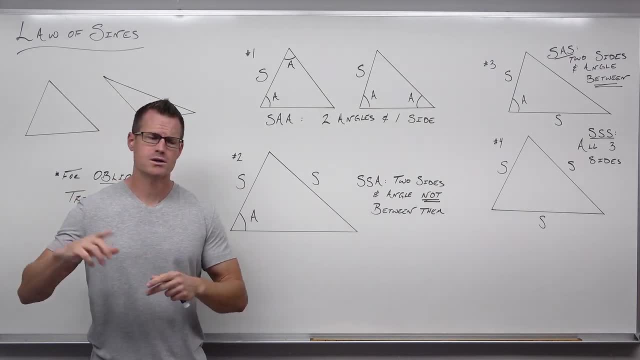 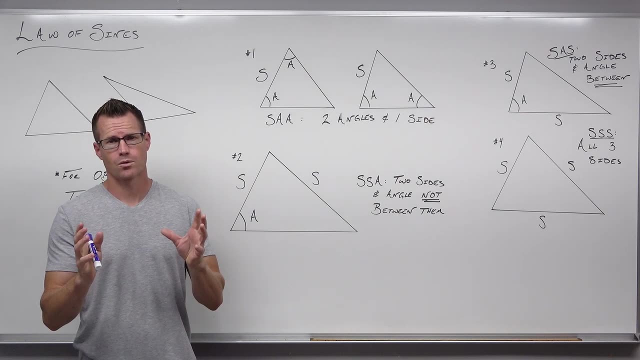 I hope that you can see that That in a right triangle you already know one angle, And so it reduces that to just two missing things, And it would actually fit a lot of these models. So we're going to take a look at what works for what. 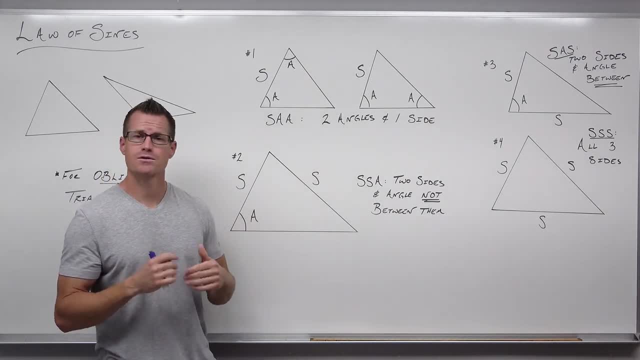 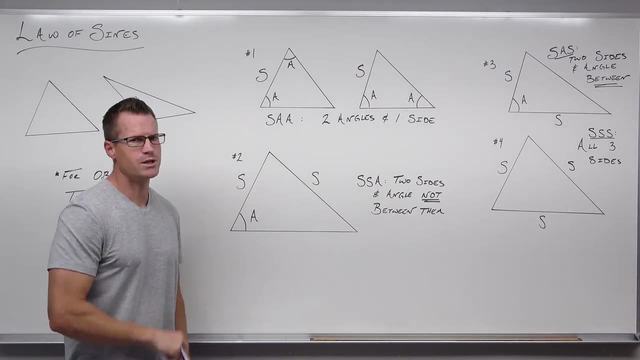 Our first two cases for law of sines, Our last two cases for law of cosines, And when we get there I'm going to show you that. So let's take a look at what works for our law of sines. Here's what we can do. 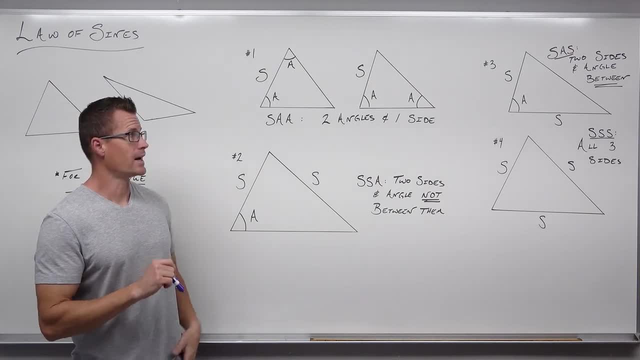 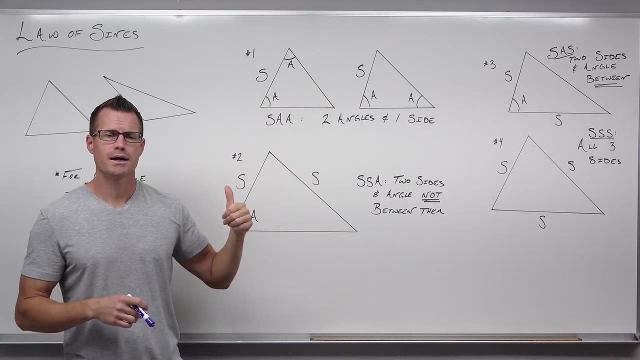 If we know two angles and one side, whether that side is between our angles or not. These are the two cases you could have. knowing two angles in one side, We can solve for the missing sides really, really easily with law of sines. 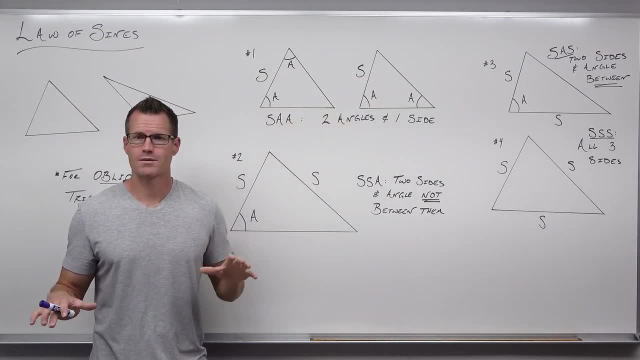 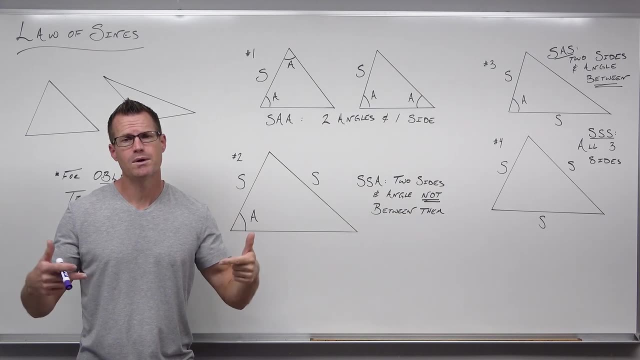 How could you find the missing angle? It would not require law of sines. Oh man, I remember. I hope you remember in the last couple videos I've been telling you: use non trigonometry stuff if you can, because it's easier. 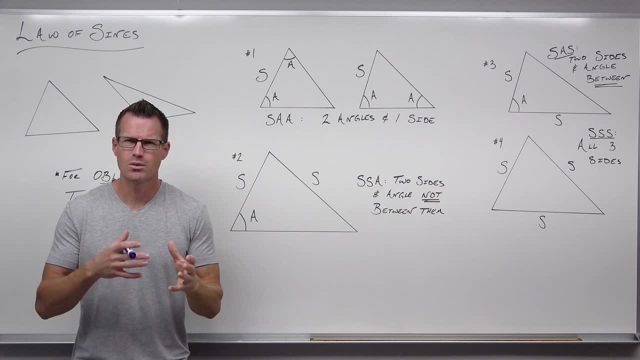 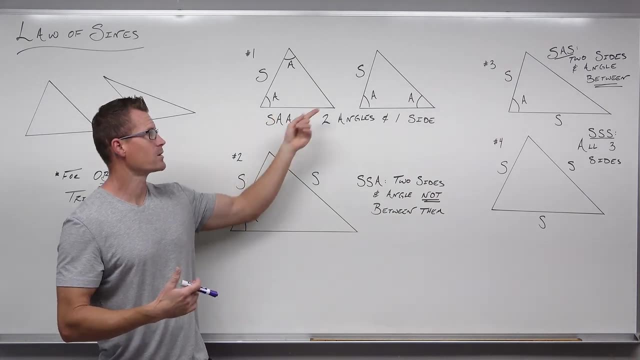 You would not want to find that angle by anything to deal with our trigonometry, like law of sines or anything. What we want to do is just use interior angle. sum All three angles, add up to 180 degrees. If you know two angles, you automatically know the third one. 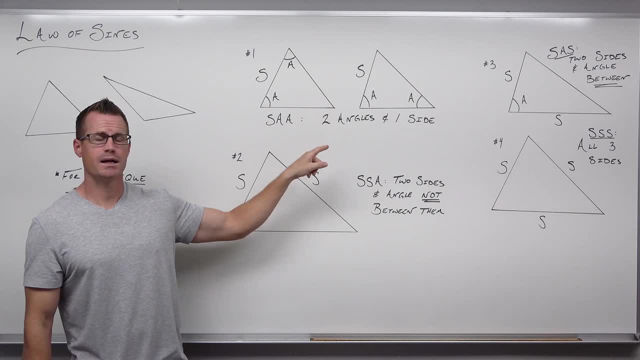 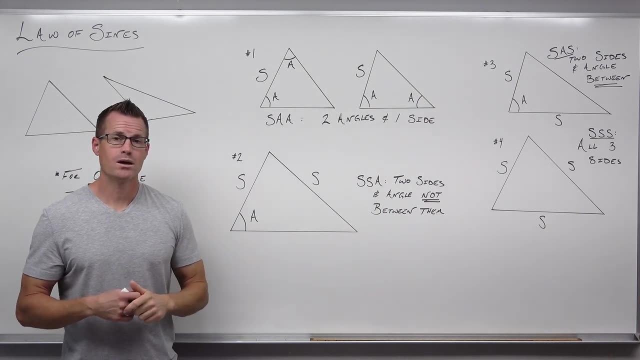 So that's pretty nice, But if you know two angles in one side, you can find the missing sides with law of sines, That's what that does. Now what if you have two sides in one angle And the angle is not between them? 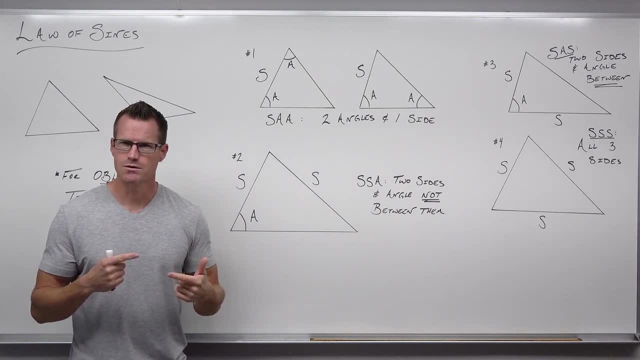 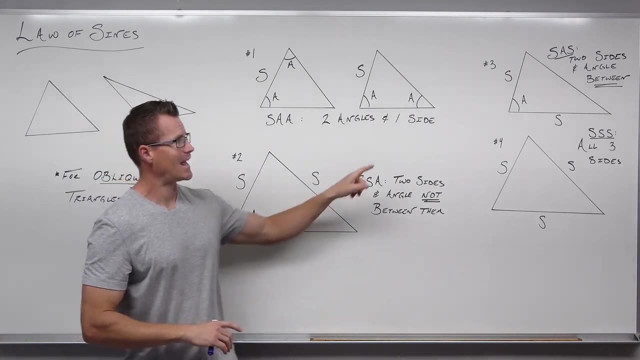 That's pretty key. So one of the things about the next two videos is understanding what works Whether we're using law of sines or whether we're using law of cosines, because this one and that one get confused an awful lot. You can probably see it. 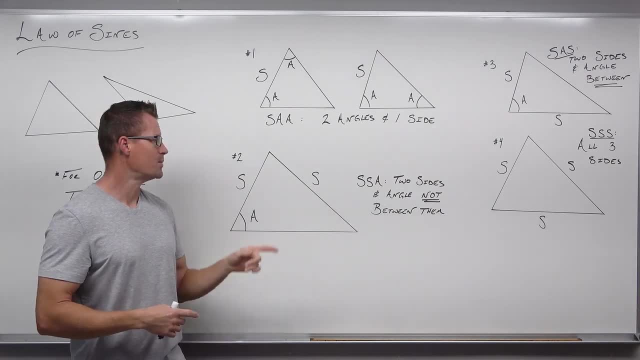 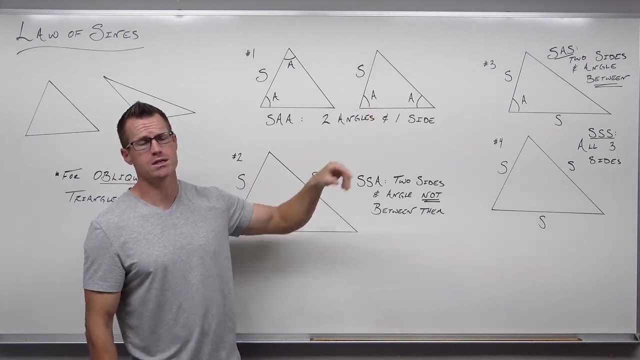 In both cases you know two sides and you know an angle, But this angle is not between the two sides. These sides are not adjacent to that angle. In that one the sides are adjacent to the angles you know. So law of sines says: 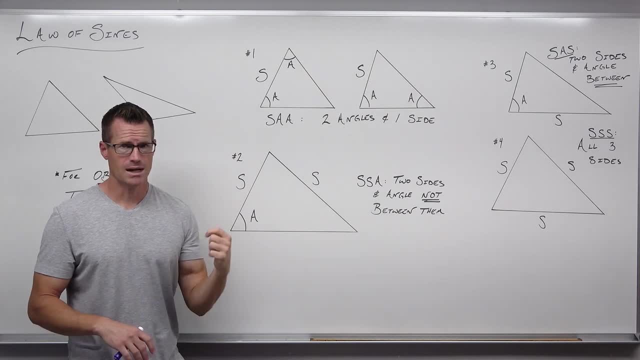 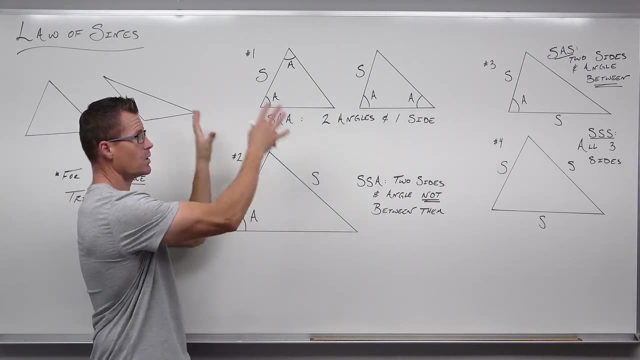 If you know two angles in one side, use law of sines. If you know two sides in an angle and the angle is not between those sides- the sides are not adjacent to the angle- use law of sines. These are both cases where you use law of sines. 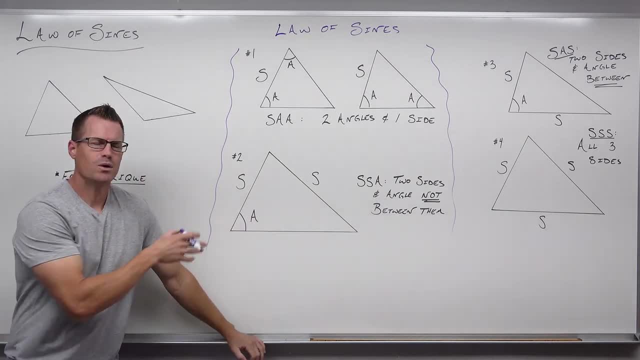 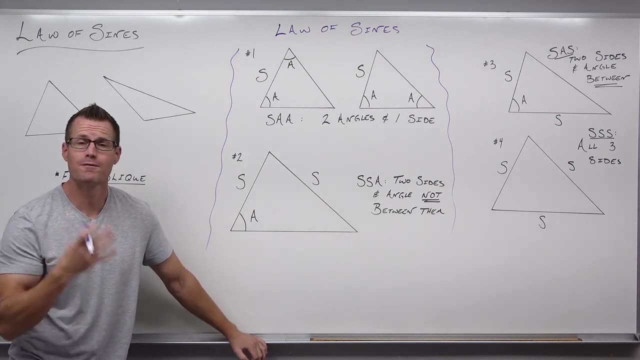 I do want to talk a bit more about this guy. This is what they call an ambiguous case, And the reason why is because this can give you one of four results. Four results. How in the world does that happen? Well, I want you to think about this. 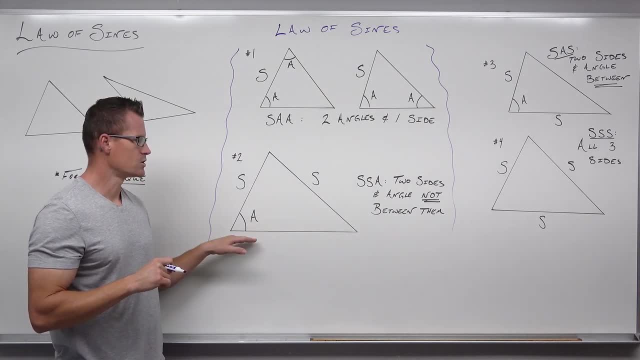 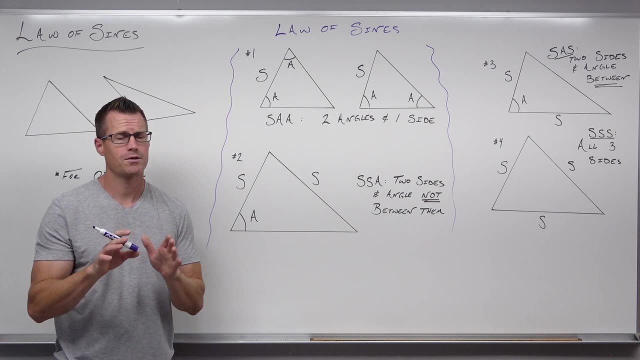 If you do not know this side, then this side can be really short, This side can be really long And this side can be not long enough to make it down to it. So there's one of four things that can happen here. The first thing that could happen is you could actually get no solution with this. 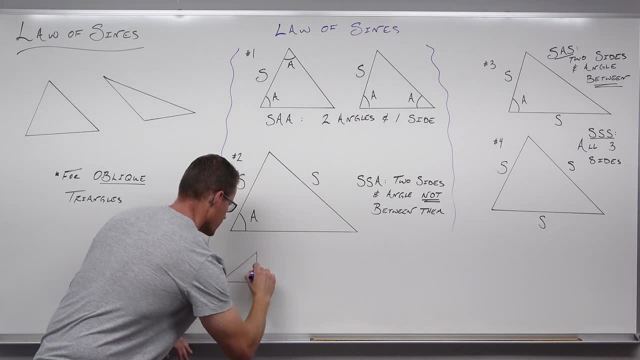 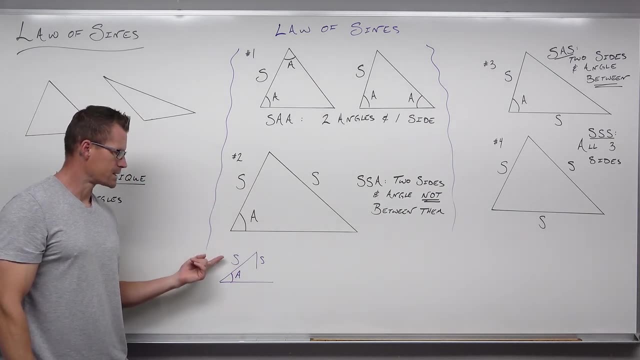 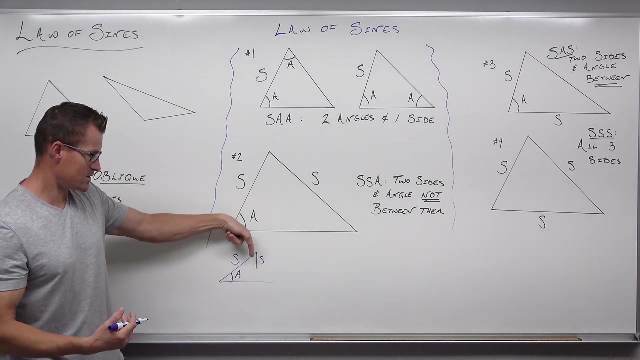 If you know a side, a side and an angle, not between them, you could actually end up with the case that this is too short to make it. No matter what you do cannot make it. This is not going to make a triangle out of it. 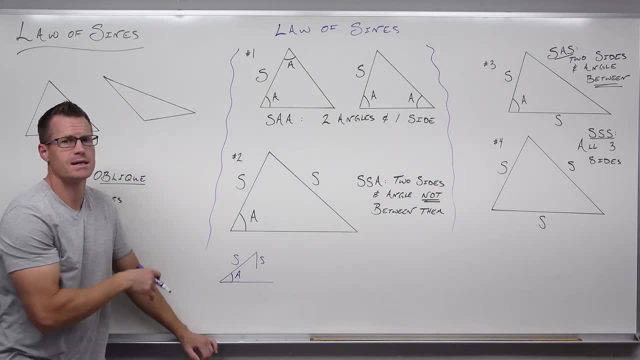 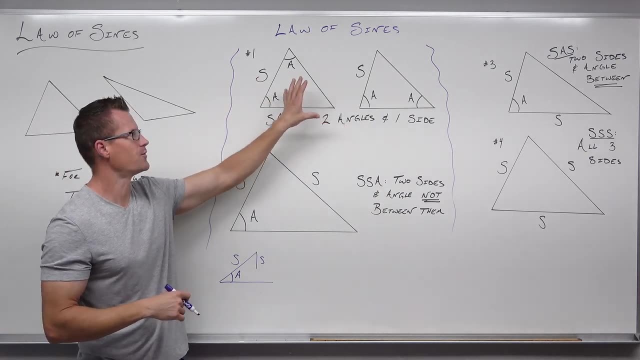 That wouldn't make a triangle. So this could happen in this case and you're not able to solve it, So there would be no solution here. If you know this, It will make a triangle and you can find the sides that it would take to make that. 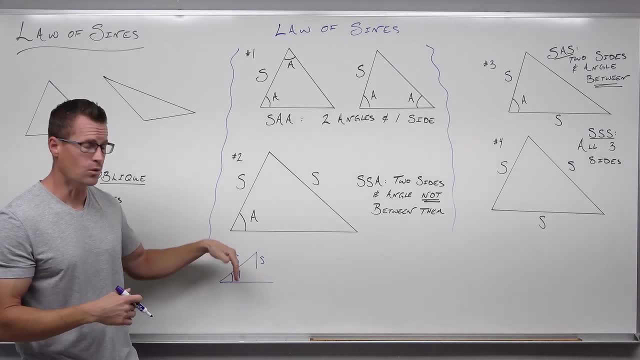 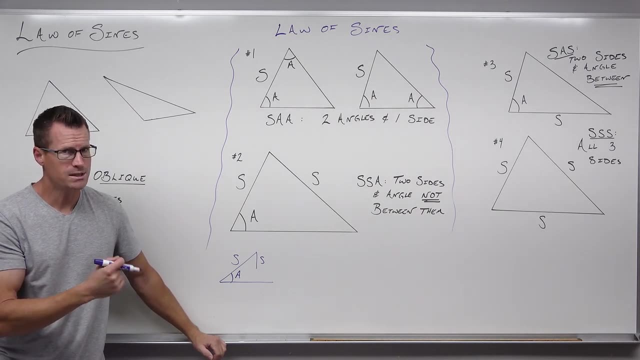 But notice, you're kind of fixing two sides here and you're fixing an angle. This side could be too short to actually make a triangle. This is one case where you would get no solution. What's the next case? The next case is that this could be perfectly long enough. 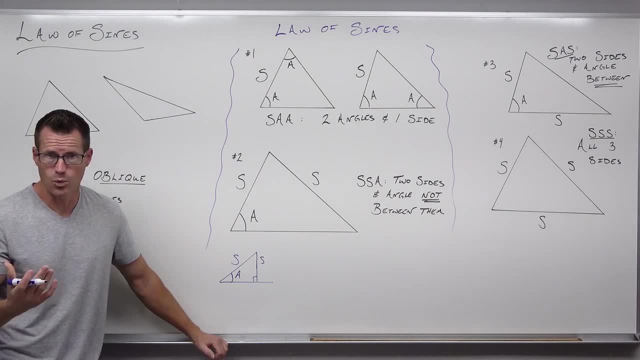 To make a right triangle, exactly one right triangle. that could be one of the cases. So first case is too short. You only make a triangle. Second case is you make exactly one right triangle. That would be if this is exactly how long it would take to make this side. 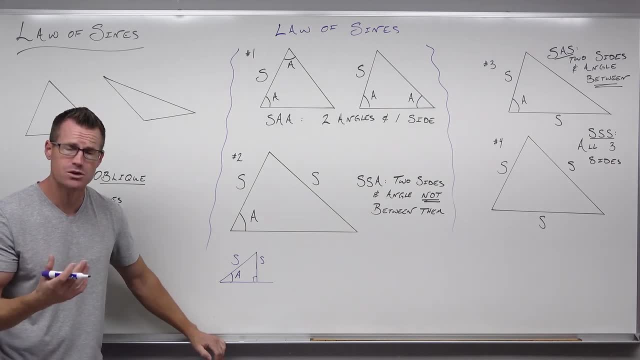 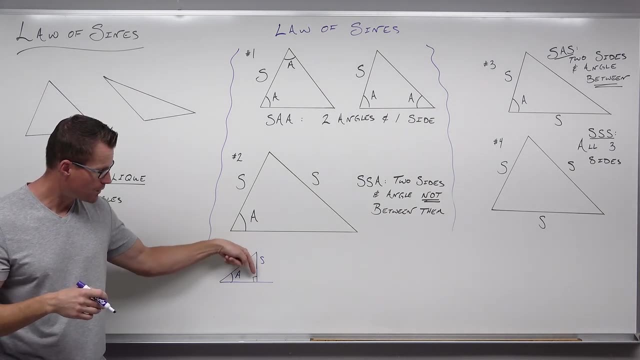 This side match up with the side on that angle. So you could, you could definitely do that. The third and fourth case is: what if this side is longer than this? What if it becomes too long? Well then, you have two more cases that could happen. 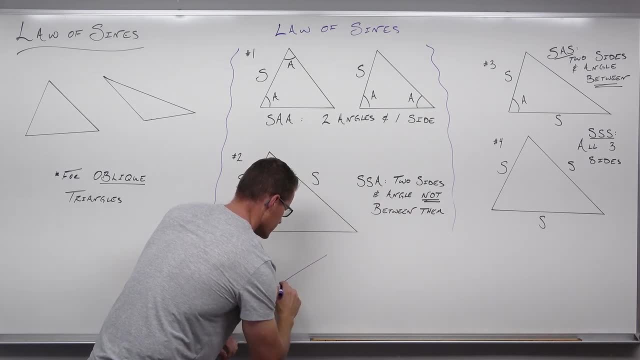 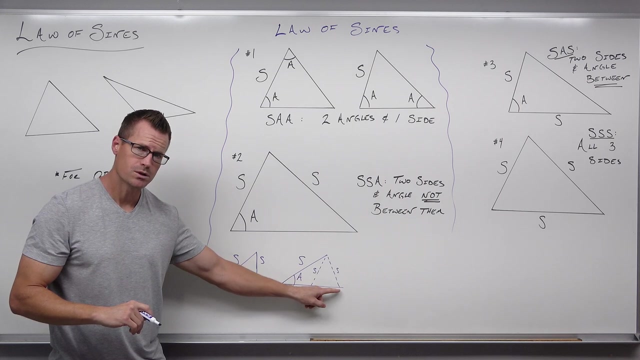 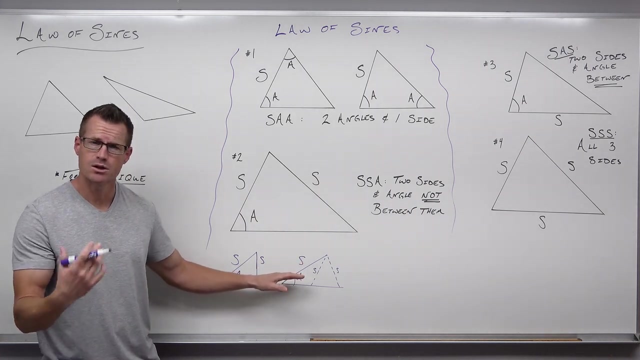 You could get. You could get one triangle, That's all acute, or one triangle is one obtuse angle, So they're both oblique. But this is two cases. Do you see how you could get two solutions? here You go. Oh yeah, this side would be fixed. 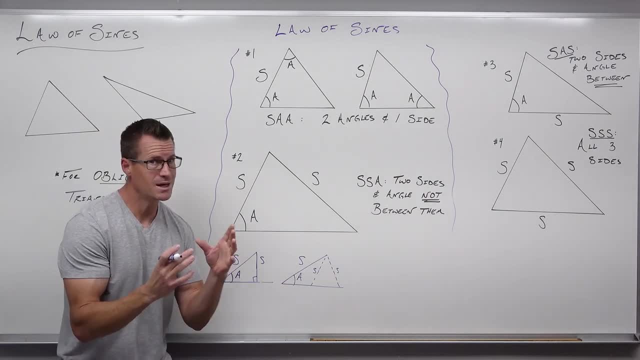 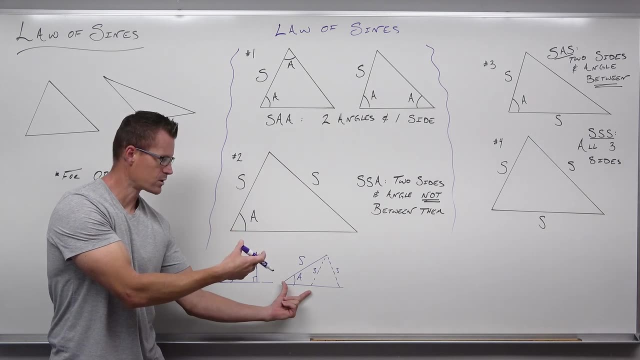 This angle is fixed. If you don't know this side length- and it could be anything that you could do- Maybe think of a shorter side that would cause an oblique angle, Sorry, an oblique triangle with an obtuse angle. Or you could have a longer side. 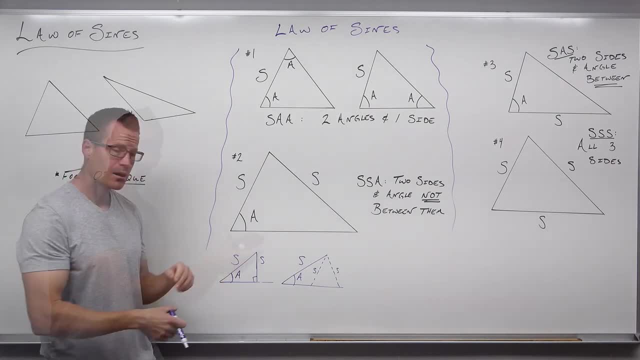 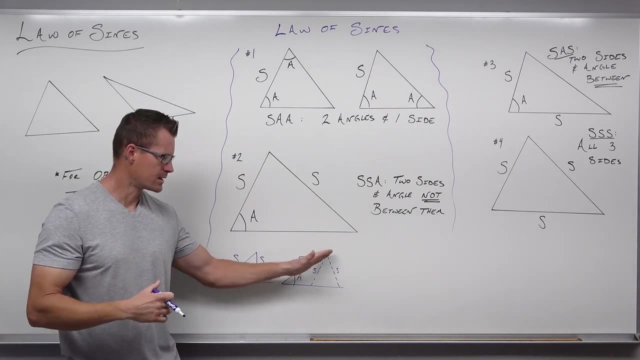 Would you cause an oblique triangle with all acute angles? There's two cases. They're an obtuse triangle and an acute triangle. Hope you're seeing that that this side could kind of kind of pivot. So our three cases so far are no triangle. 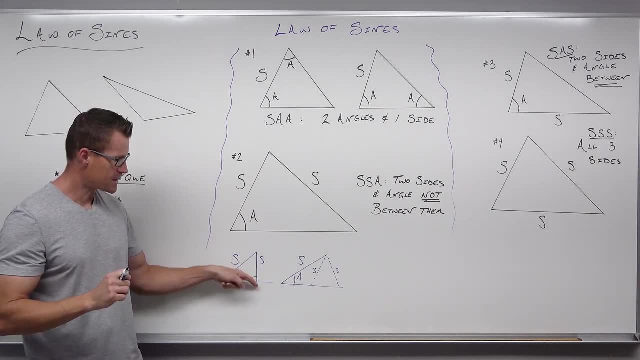 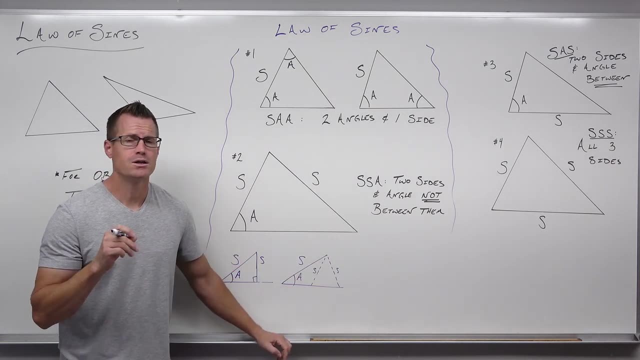 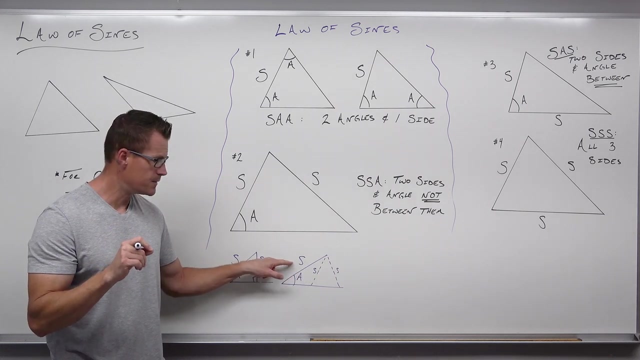 It misses a right triangle. It's perfect. If this side's too long, you could get two cases: one an obtuse, one an acute. Now I need you to notice something: This only Can happen if this side is shorter than this side. 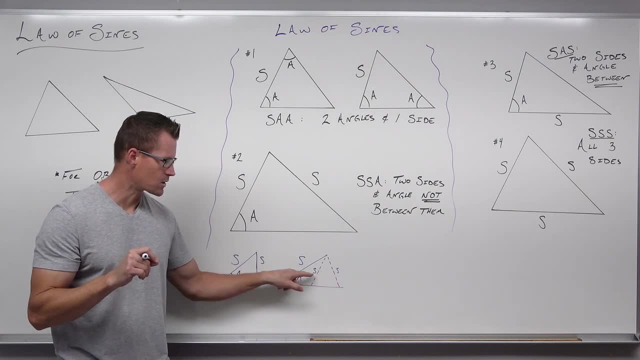 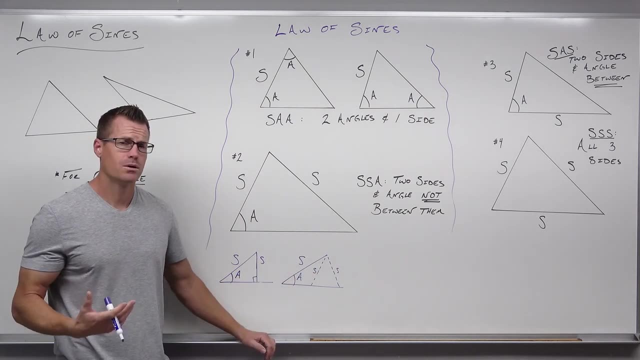 Why? Because if this side that can make your two options are shorter than this side, then you can go ahead and put that down to this missing side and not kind of overrun it. You don't have this this case, if this side is longer than this side. 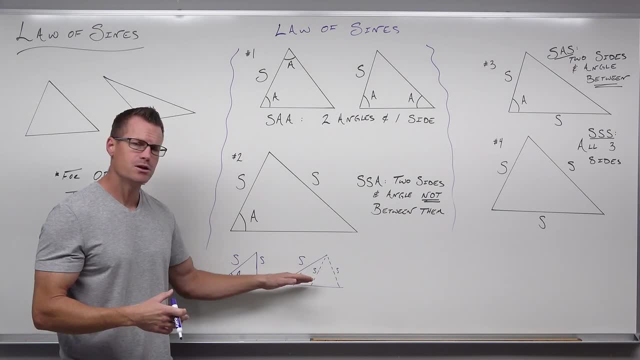 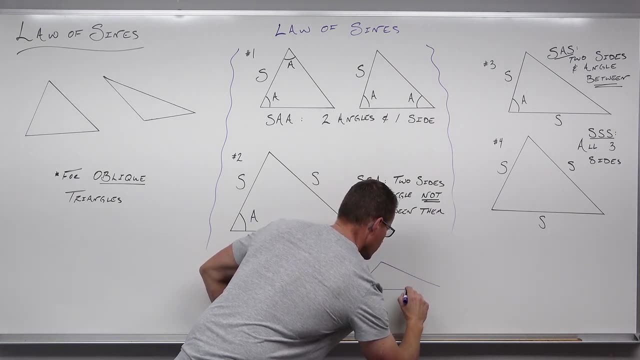 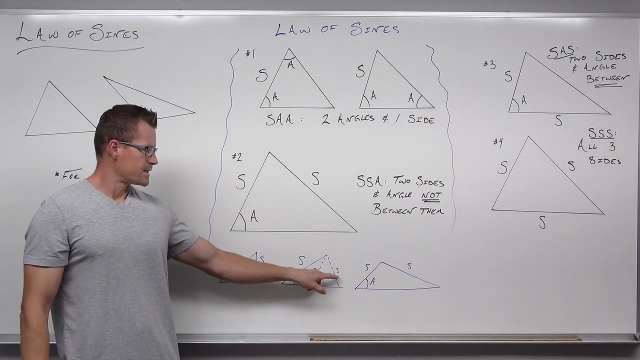 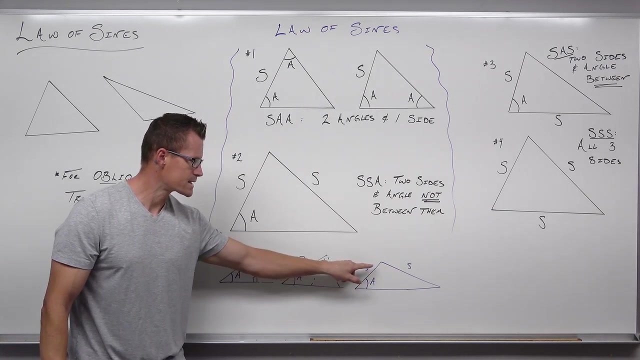 So if it is, if the second side is longer than this cult's first side, then you really only have one option: If this side is longer than you, can't make this obtuse angle come about. Why? Because if this side is longer than this side, 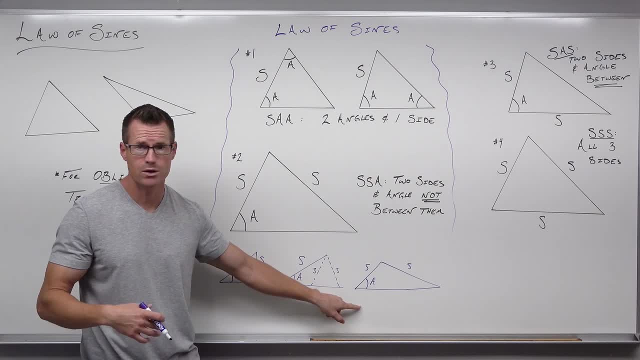 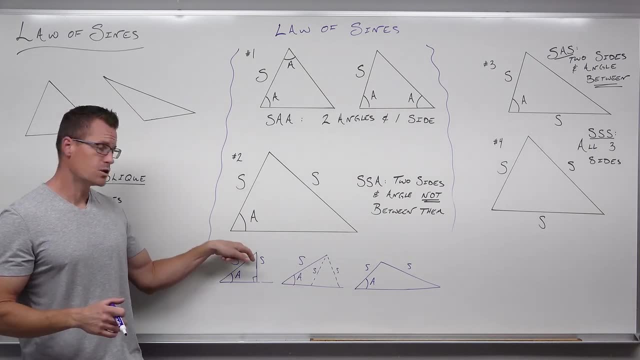 it would go past this side, that third side that you don't know. That would not cause a right triangle, or sorry, not cause a triangle, because that angle is fixed. So there's really four cases. You have this: no triangle. You have a right triangle. 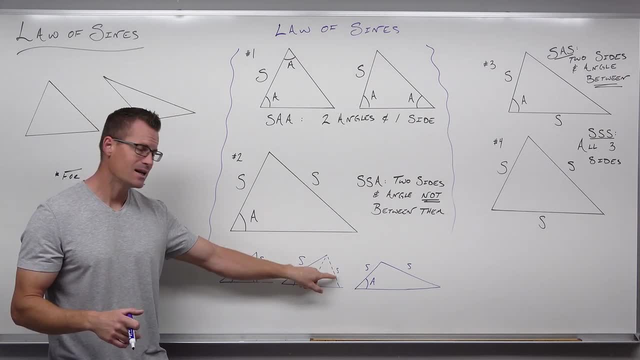 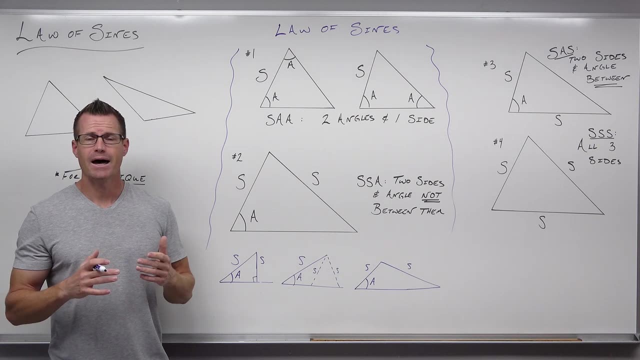 You have a. I could have two options. If this side is shorter than that one, I have one option if this side is longer than that one. Now, that seems like a lot to remember. Don't worry about it. The law of signs will take care of this for you. 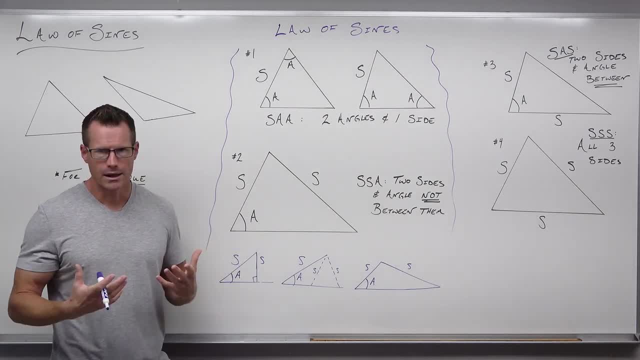 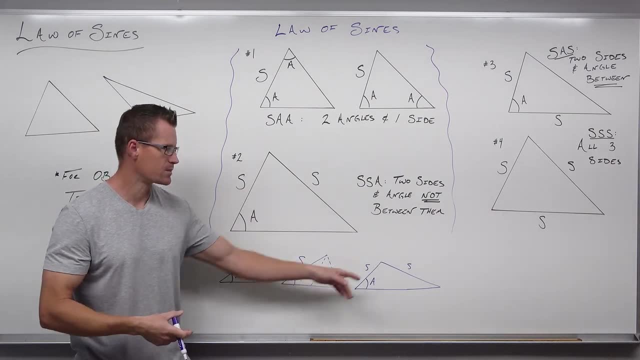 I really just wanted to go through these so that you would understand why Sometimes you get one right triangle and why sometimes you get no triangles, Why you get sometimes two and sometimes one. that's not a right triangle And it really just comes down to. 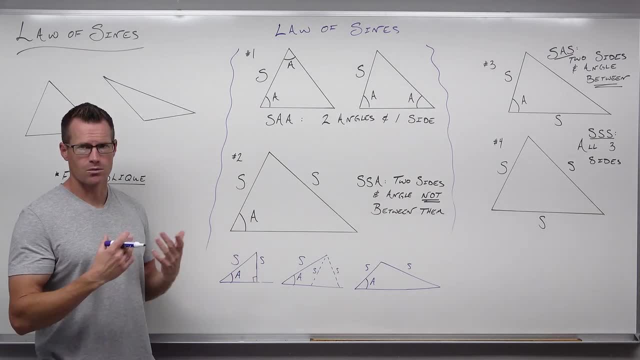 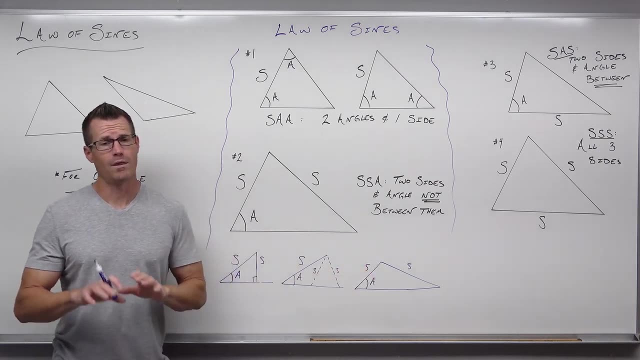 If this is too short, you can't make a triangle. If it's perfect, you make a right triangle. If this is longer than perfect, you could get two. If this is longer than this one, you only get one. That's the reason why. 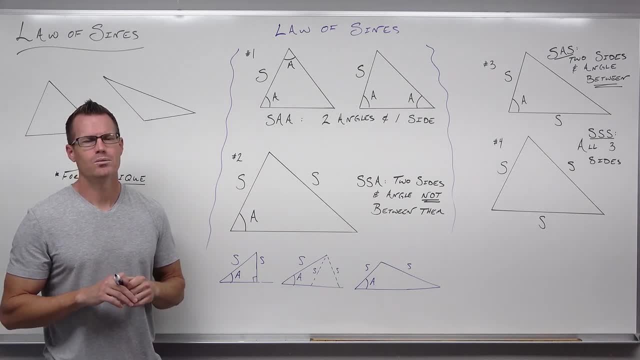 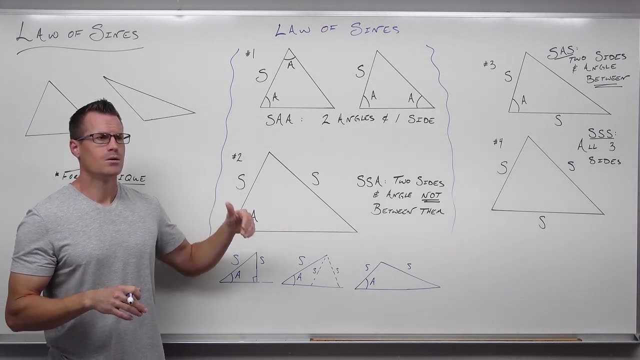 And so when the law of signs tells us what we're getting out of that? this is why You don't have to memorize it, which is very nice. This will take care of it, because sign will show you whether it's possible or not. 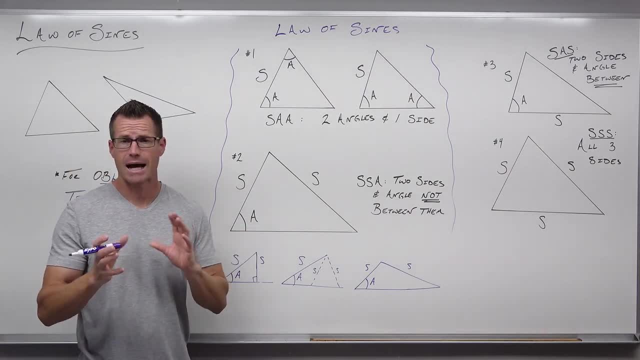 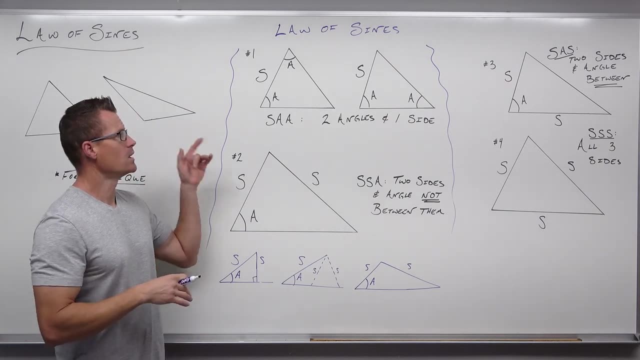 And we're going to get to some examples, of course, in this video that explain exactly what's going on, And I'll be referring to those cases. So the only two cases that really work for law of signs are: you know two angles in one side, or one side and two angles, or you know two sides and one angle. 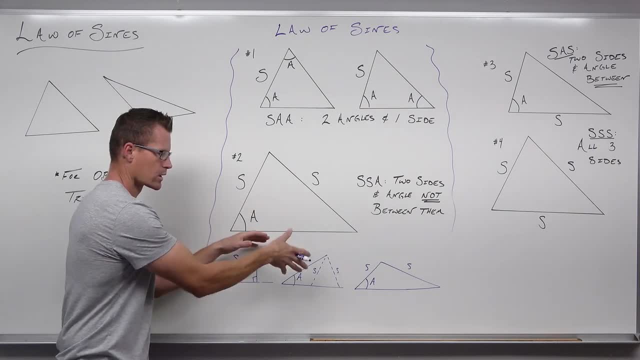 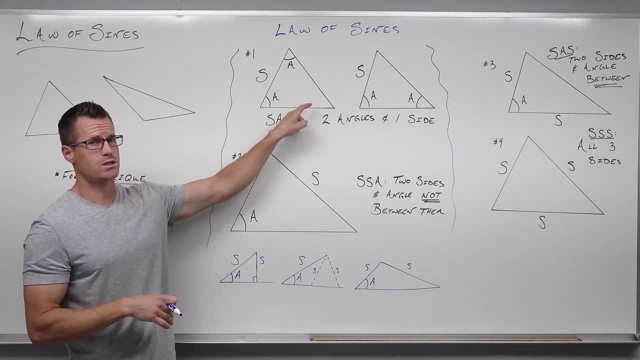 But the angle is not between them. This is when you use law of signs and it'll work itself out. You will know whether you have one, none or two solutions with this case. This one will only give you one solution every time, So this is easier. 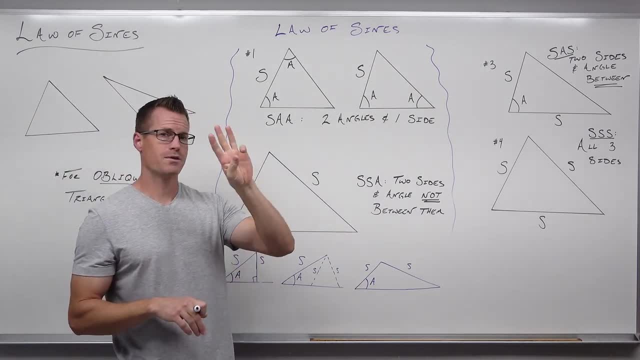 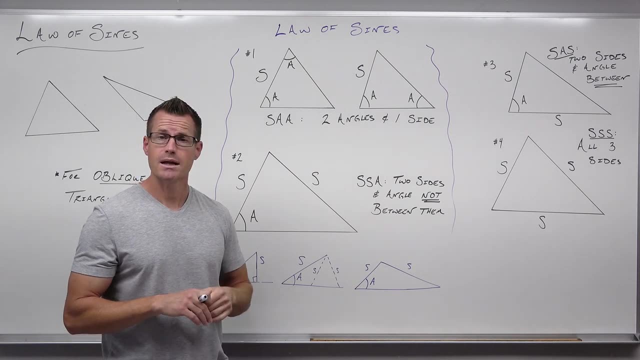 Now what if you had some other instances where you know three things, you're trying to find a fourth? You could have two sides and one angle between those sides. You could have all three sides that are known. Those would be known three things and asking for a fourth thing. 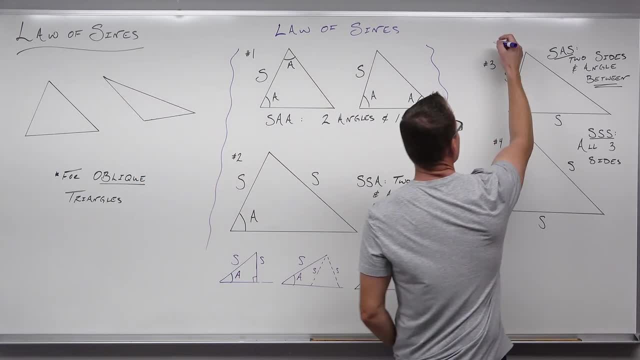 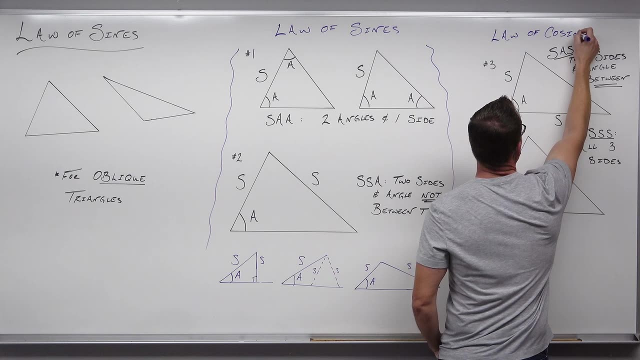 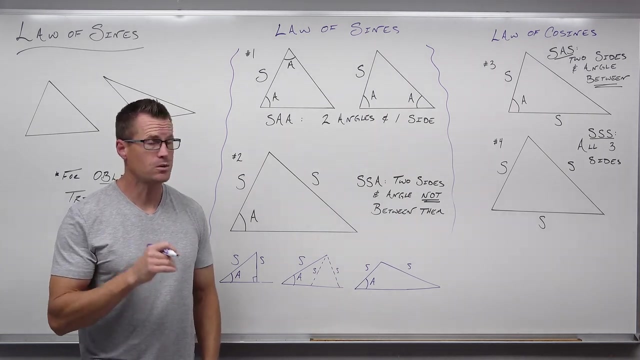 These are done with law of cosines. We'll also learn how the Pythagorean theorem is really a special case of law of cosines, How you can know one angle and two sides, and it will give you a third one. You go, wait a minute. 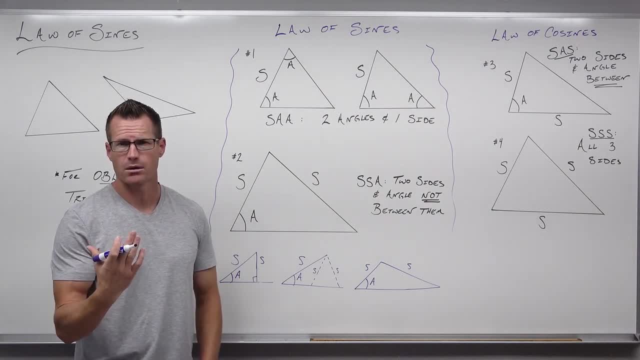 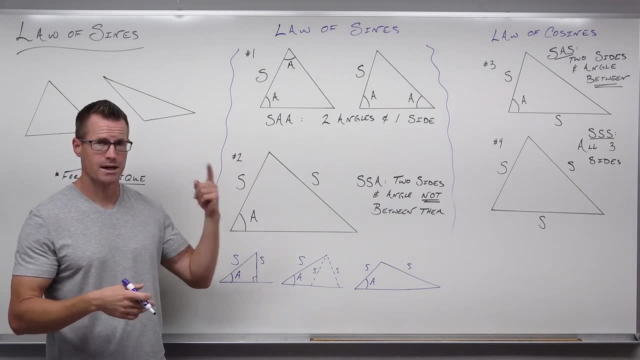 How would that happen? Well, you know one angle and right triangle already. you know the 90 degree angle. So I hope you're seeing, in all of these cases you need three things to find a fourth. You need two angles and a side to find another side. 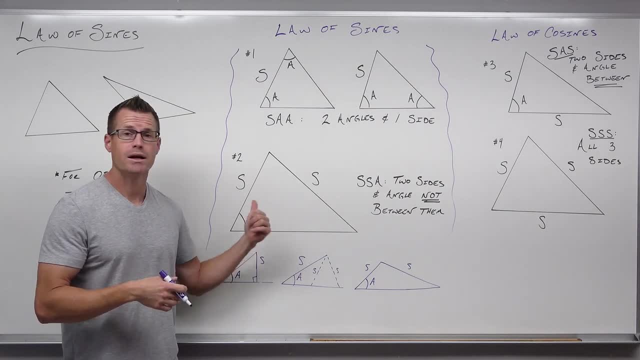 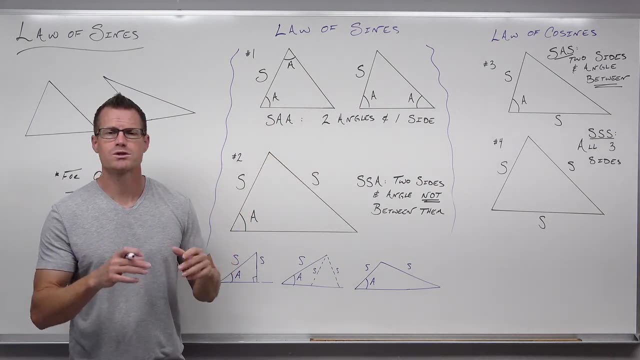 You need two sides and an angle to find another side or another angle. You need two sides and an angle to find another angle or another side. You need to know all three sides to find angles. So you know three things to find. 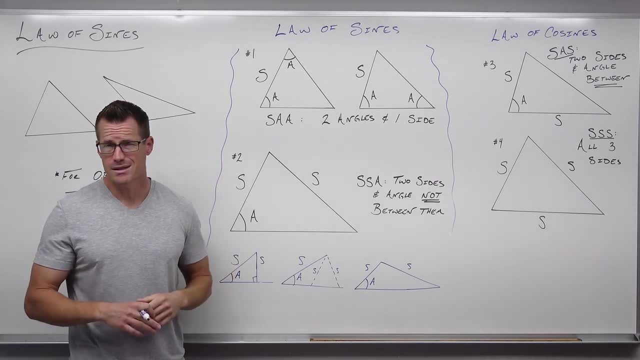 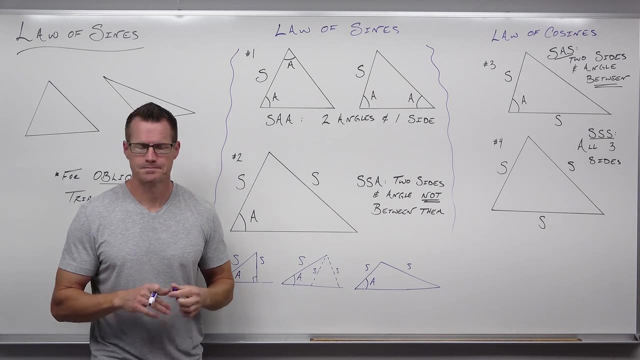 The fourth one. what we're going to do now is talk about what in the world the law of signs is, how it works. It's a very nice proportion. You will understand why you need to know this when we go through it. Now let's practice some examples. 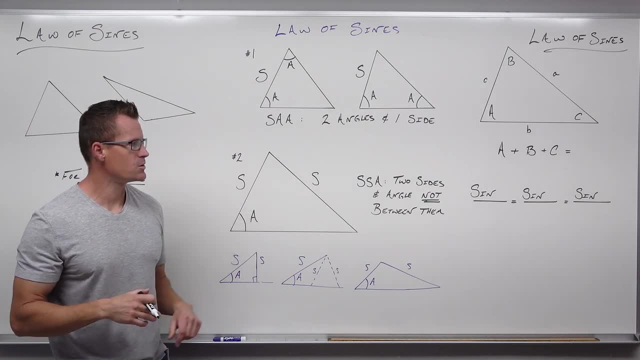 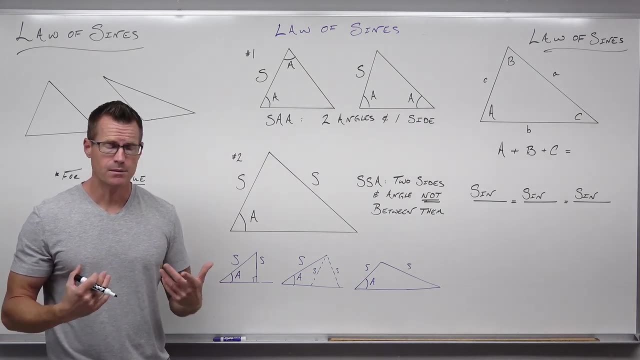 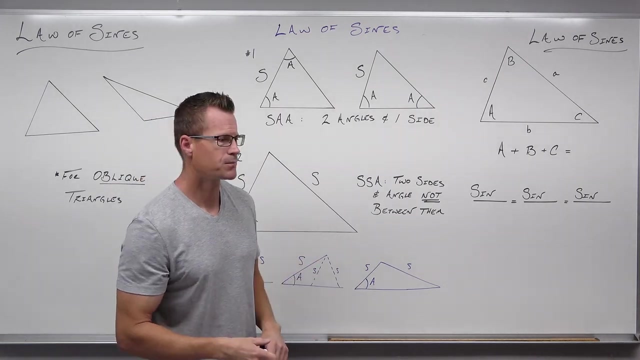 So, provided you have one of these two cases- one side, two angles, or two sides, one angle, not between them- You can use law of signs. What in the world does law of signs mean? Well, firstly, you're using law of signs on non right triangles because you have a right triangle trigonometry to deal with the rest. 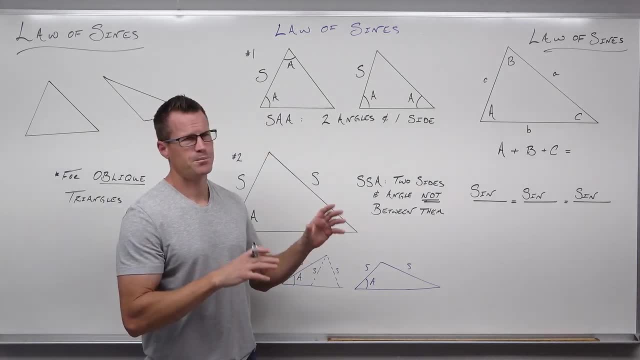 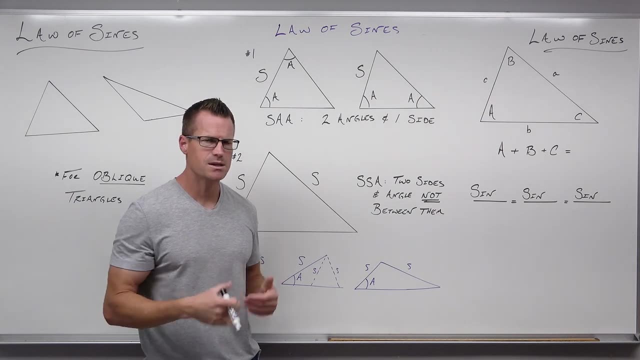 Could you use it on a right triangle? Yes, Yeah, you really could, but you don't need to. So law of signs says: if you have this triangle, this oblique triangle, with our angles A, B and C and our opposite sides listed as lowercase letter A, lowercase letter B, lowercase letter C, 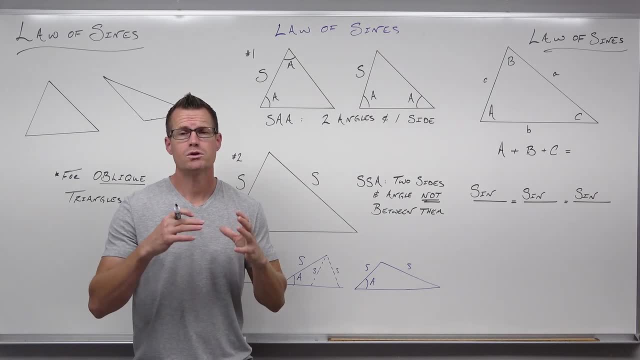 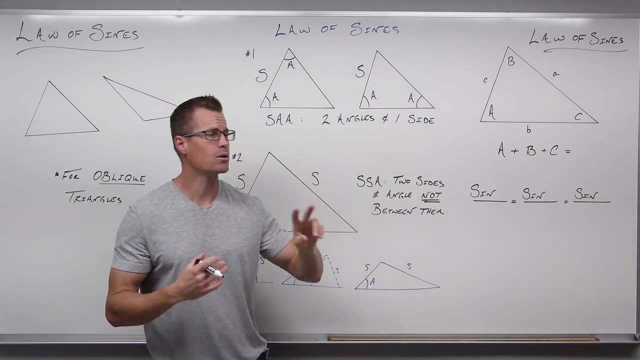 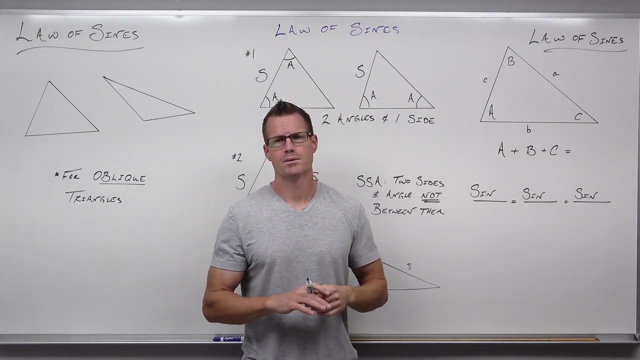 So A, B, C again. The first thing I want to remember is you don't need any sort of law of signs or law of cosines or right triangle trigonometry, if you know two angles, to find a third, Because A, B and C- those angles on a flat plane always add up to 180 degrees. 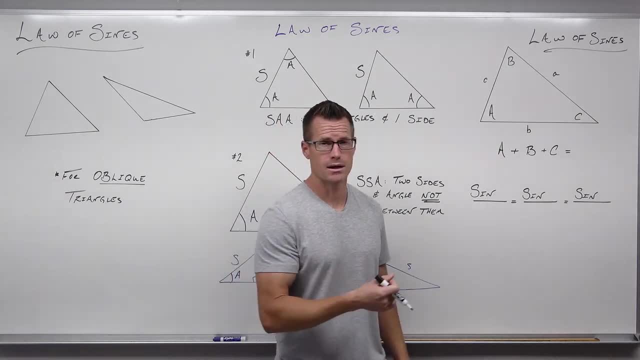 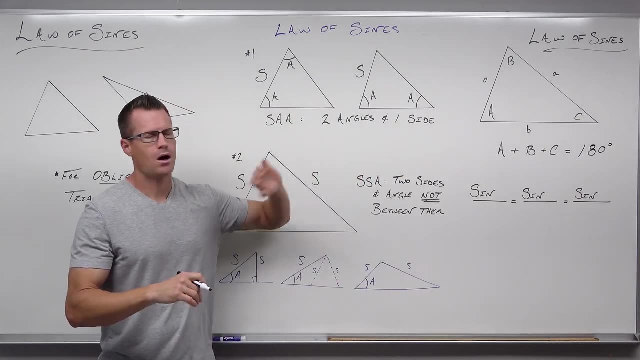 The interior angle sum of any triangle on a flat surface on this plane is 180 degrees. So if you know two angles you can automatically find a third. That's really nice. Don't use law of signs for that, Just use interior angle sum if you know two angles already. 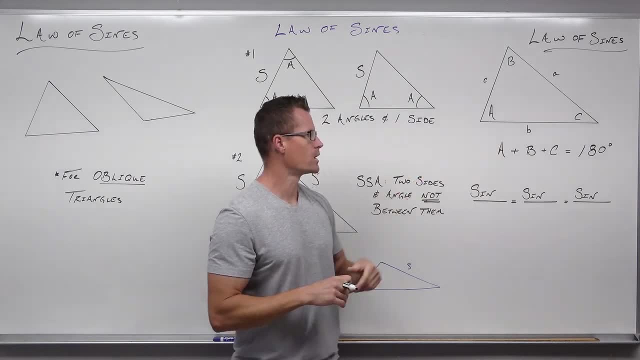 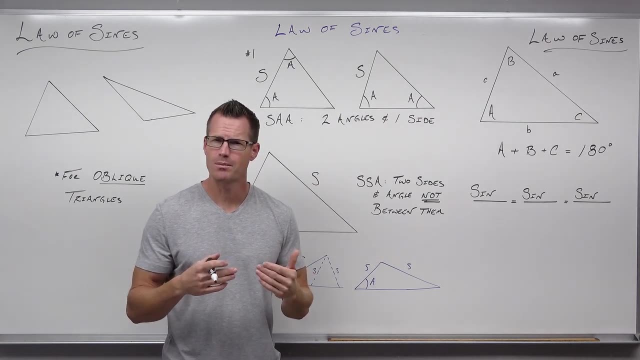 So anyhow we have, this is pretty important. Our angles are going to add to 180.. What the law of signs does is creates proportions for you, And they're really nice. It's probably something you'll be able to memorize pretty quickly. 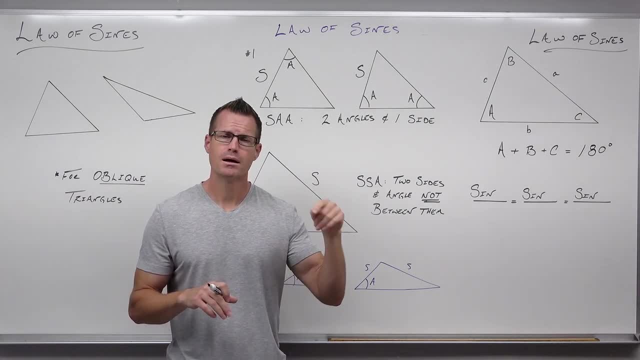 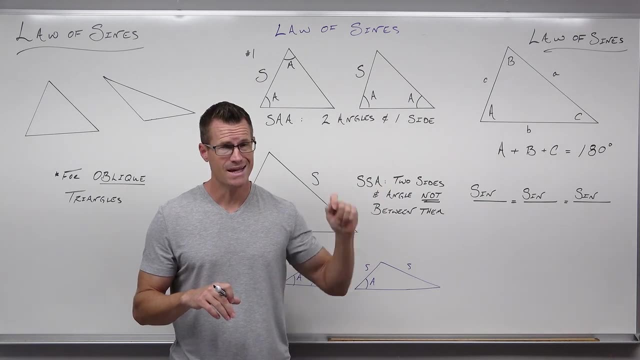 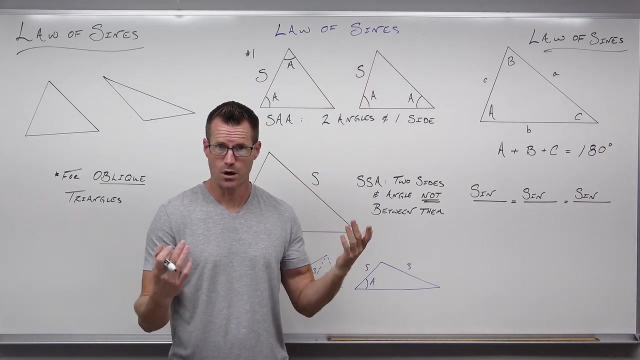 Here's what it says in plain English: Sine of an angle over its opposite side always equals sine of another angle over its opposite side. So all we've got to do is match up on each fraction angle with opposite side. So for law of signs, that's going to say find sine of angle. 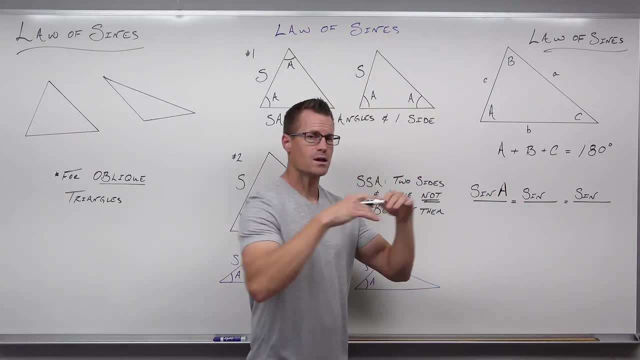 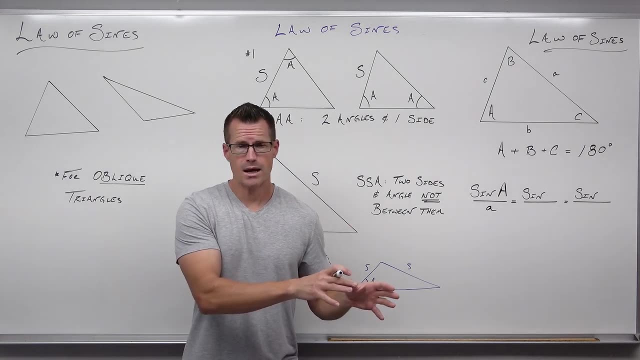 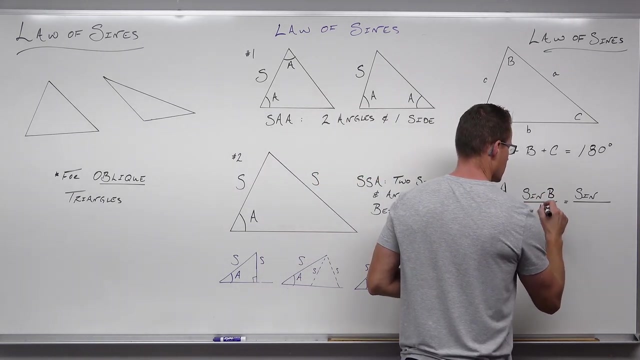 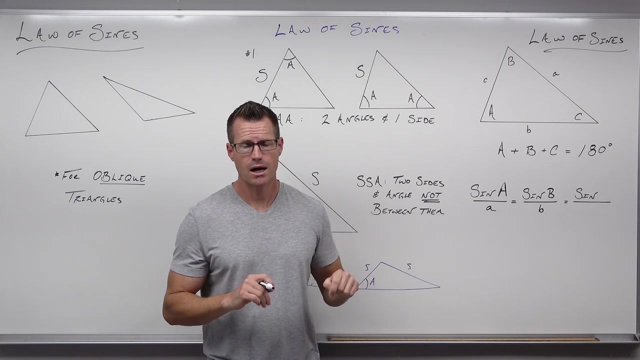 Let's say, angle A Over its opposite side, which is lowercase letter A, Equals sine of any other angle over its respective opposite side. So let's take sine of B. These two things are going to be equal. Sine of A over A equals sine of angle B over side B. 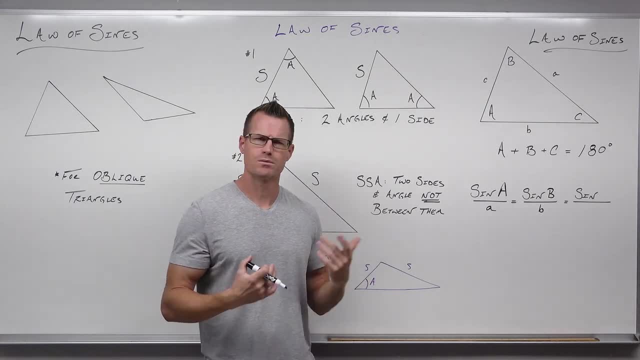 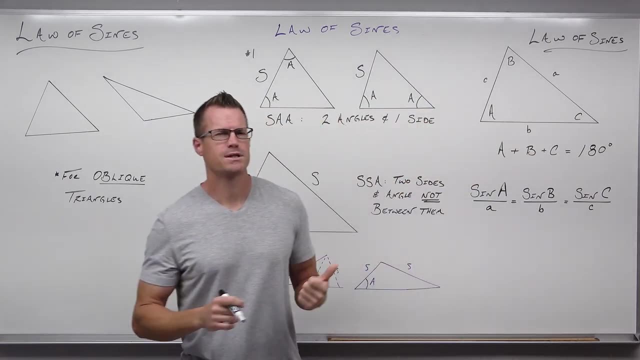 It's also equal to any other angle over its opposite respective side. So sine of angle C over lowercase C. This is the law of signs. Now there's one really common mistake that the students make because they don't quite understand what's going on here. 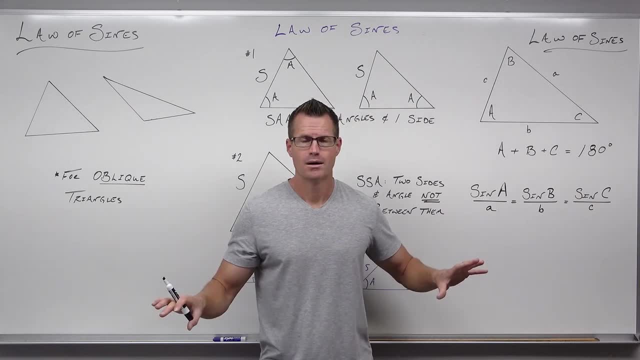 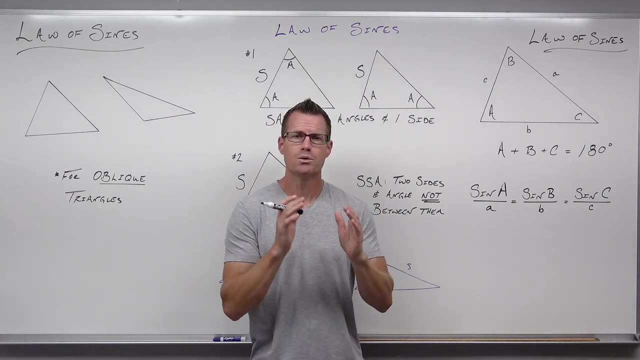 They try to use this whole thing at once. Don't do that. This is not meant to do this. This is meant to create a proportion. All it's saying in plain English is: you can create a proportion. What's a proportion? A proportion is simply two fractions that are set equal to one another. 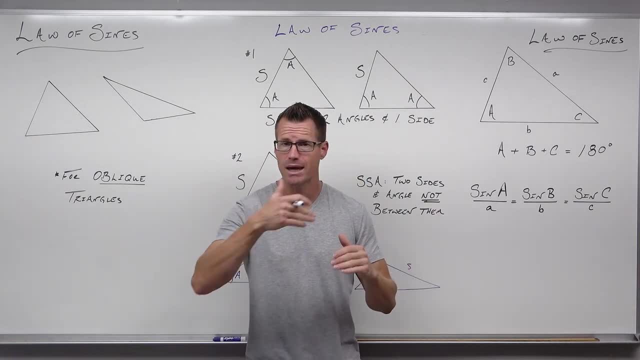 So just set two fractions, Not all three, because then you can't cross multiply. It's crazy. So all it's doing really is creating a proportion for you: One fraction equal to another. You don't use all three. It says: find an angle and its opposite side. 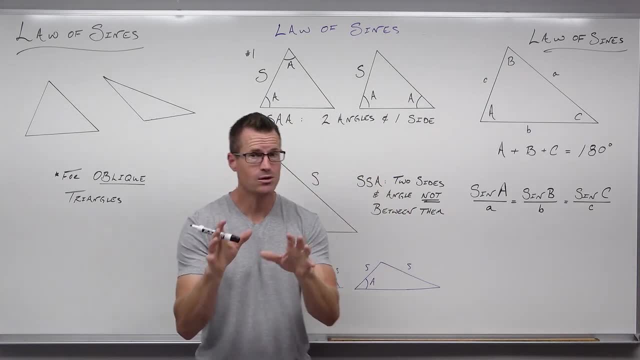 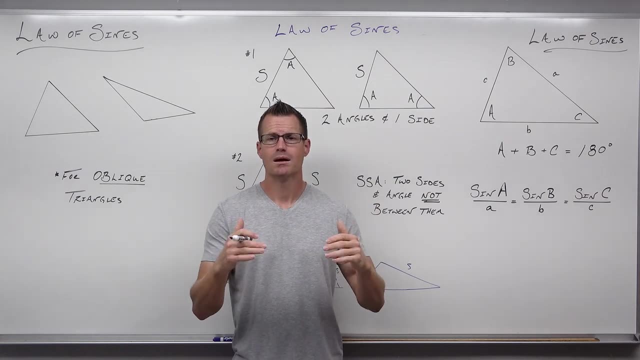 Set it equal to any other angle over its opposite side. Now, here's what I want you to see. Can you see that? because you need to know. Sorry, Can you see that? because you're setting up a proportion? Ignore this one for a second. 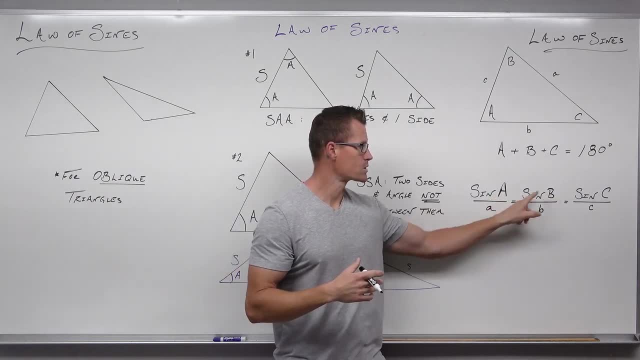 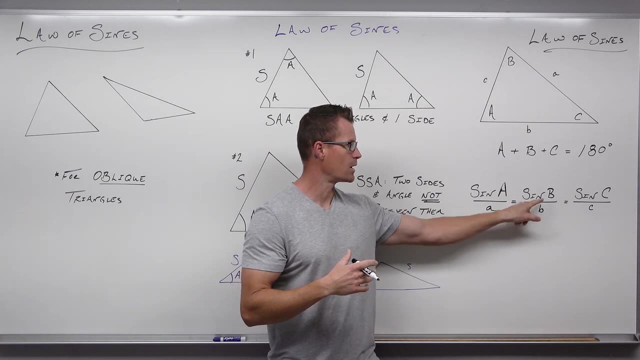 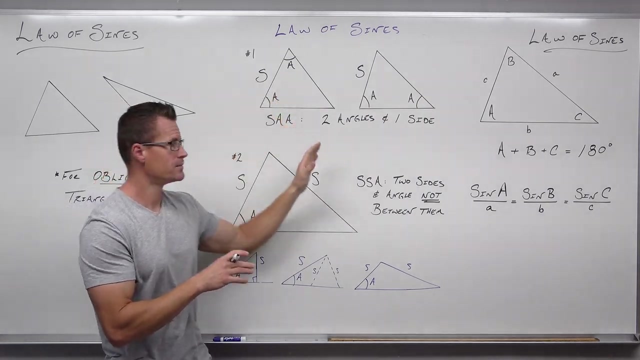 You would need to know either Two angles and one side- cross multiply to find this inside, or two sides and one angle cross multiply to find the missing angle. That's exactly what we have here: Two angles in one side, Two angles and one side- cross multiply finds this inside. 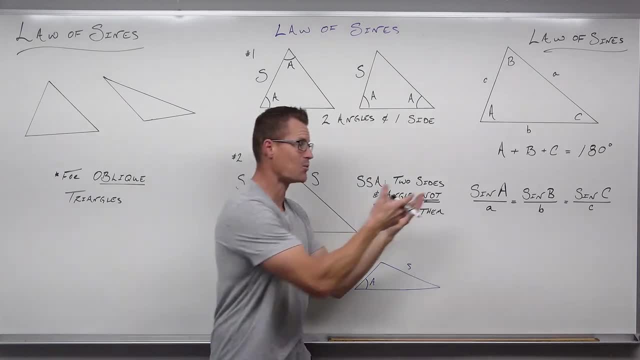 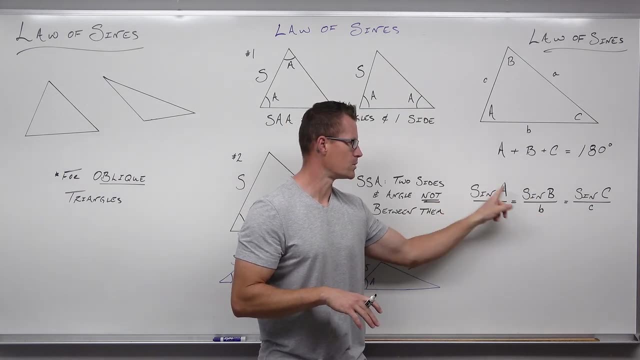 You don't need to find the missing angle because of interior angle. So that's why this works. How about two sides, One angle, No two sides and one angle Cross, multiply and figure out the other angle. That's. that's really nice. 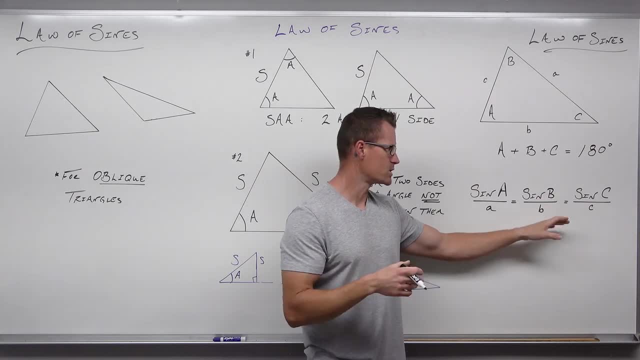 That's how this worked. You don't use all three of them. If you just need to find C, it's okay. It doesn't doesn't really matter what we call these things. You'll see that as we're going through that. 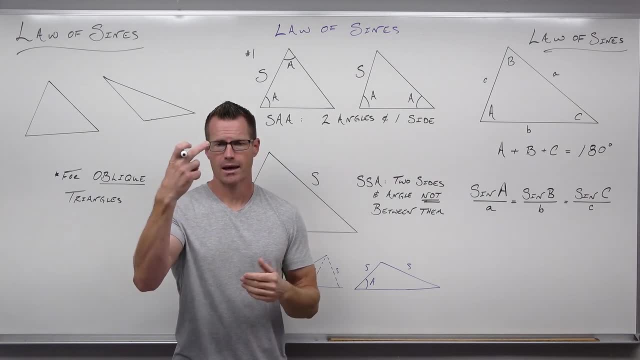 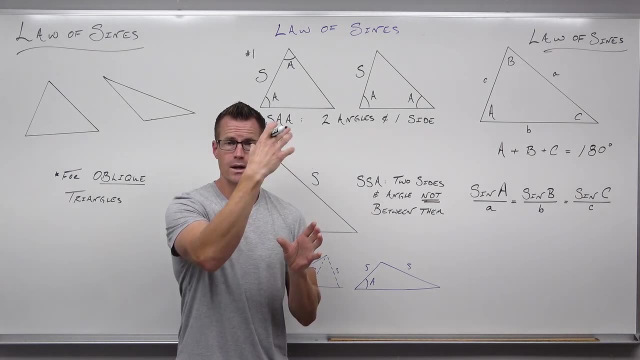 All we're really trying to figure out is: do I know an angle and its opposite side? Can I relate that to either a missing angle over its known opposite side or a known angle over its missing opposite side? And then we just cross, multiply. It's not a hard process. 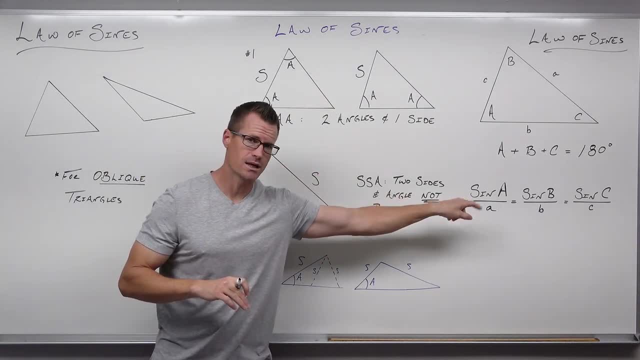 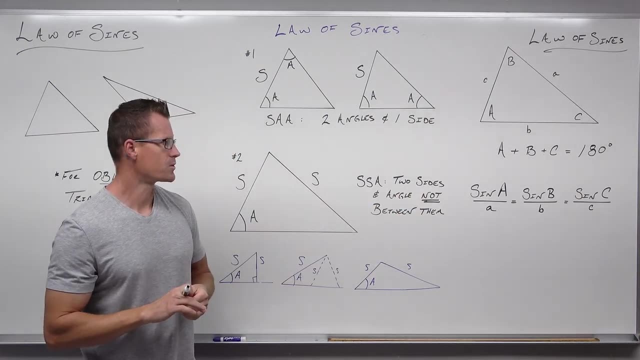 You just need to be able to identify that. two angles- one side, You use this, and two sides, one angle, but the angles not between them- You use this. So, anyhow, we'll see that as we go through some of our examples. But long story made short: use interior angle somewhere. 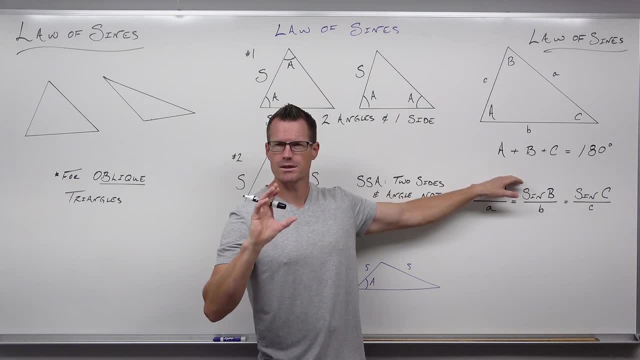 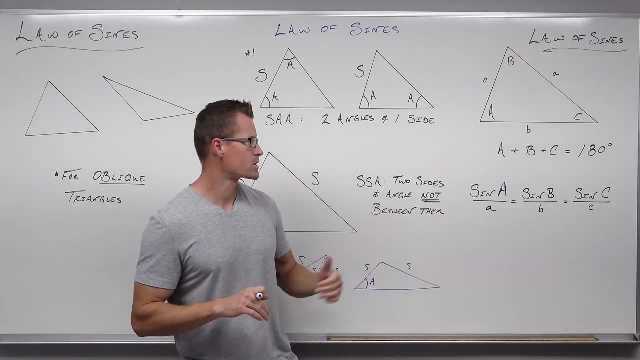 You can use it first. It's really nice to do. It doesn't cause any error in our problem. So the angle we find with it we can use for law of cosines or law of signs with no errors, And then really we're just using. 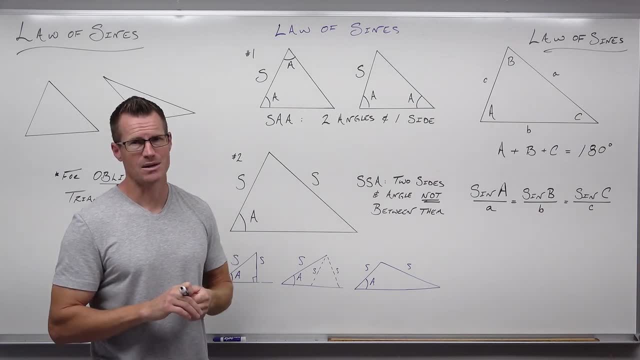 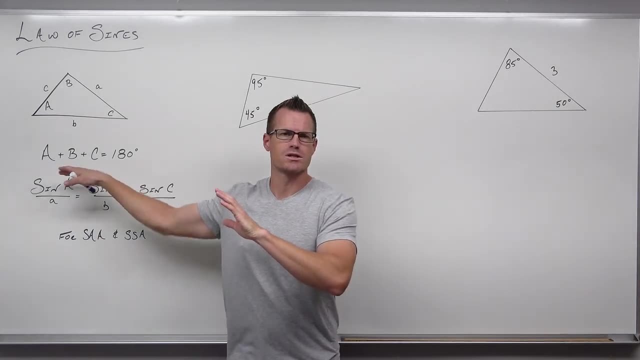 One proportion. You're not using the whole thing at once, So let's go ahead and try some examples. Let's go ahead and practice them So we have a bit the law of signs up there again. I put the interior angle of a triangle up there, just so we can have something. 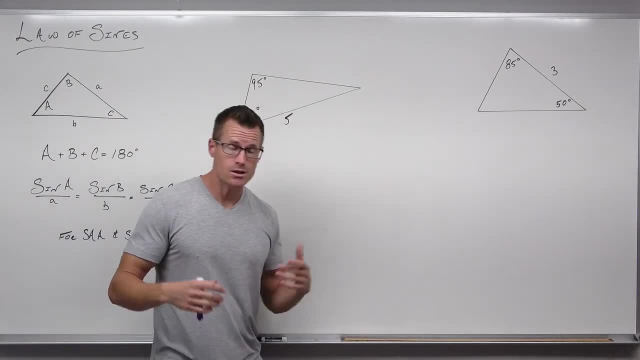 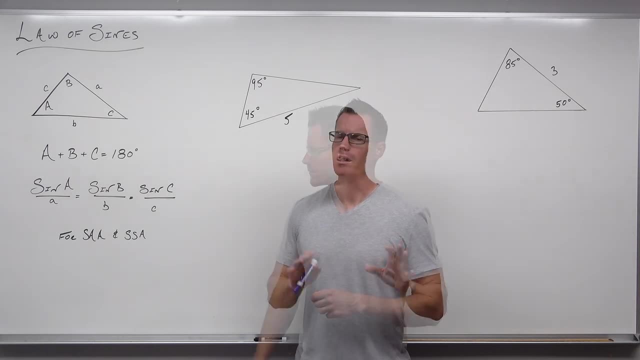 to reference to. Let's take a look at these examples, Let's determine if they fit law of signs, if we can even solve them, and then we'll set up an appropriate proportion and you'll find it's not too bad. You'll also find that this case angle angle- side or side angle angle- is easier. 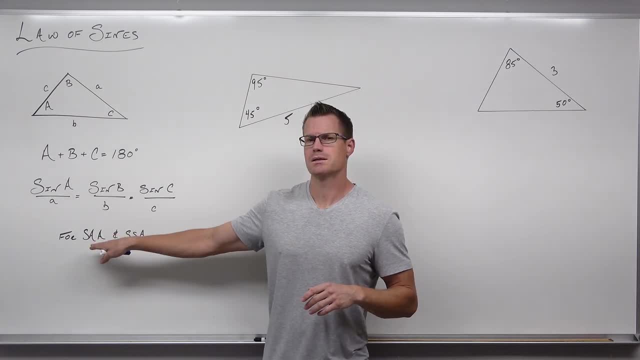 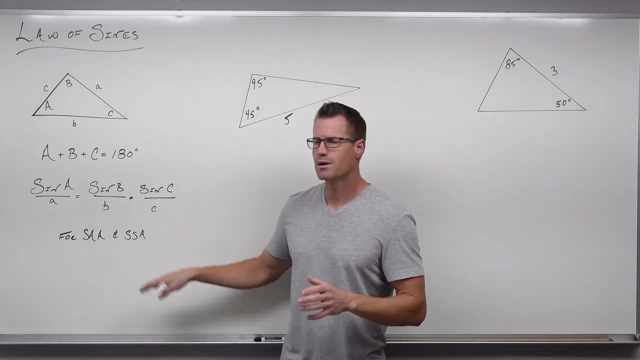 than side side angle, Why this only has one case. So if you have this, it is easier. You're finding a side with law of signs and there's not multiple options. for you. This one, you had four options. Now we don't need to know what those options are going into the problem. 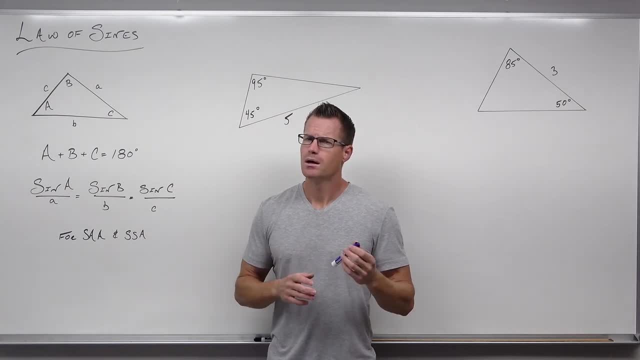 but it does cause us more work. I'll spend more time on side side angle, just because there are those options. Well, I'll give you an example of a no solution. I'll give you an example of a one triangle. I'll give you an example of how you have the options of two triangles. 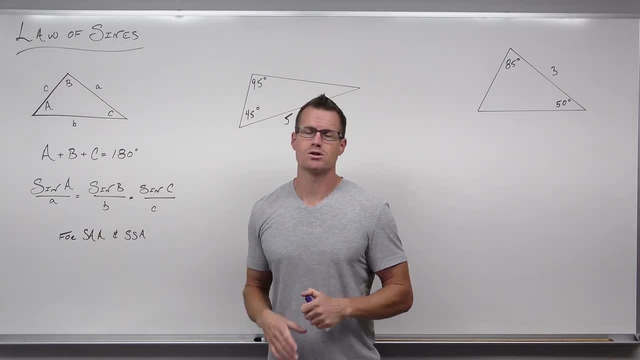 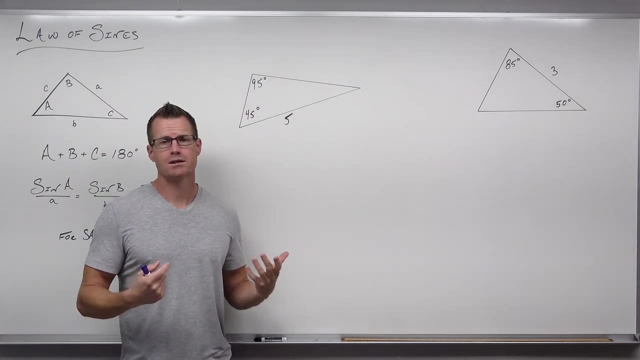 That are possible here. So we'll deal with that one. So these are nicer. So first let's make sure that it actually fits. Let's take a look at our triangle. in our triangle We're seeing that first It's not a right triangle. 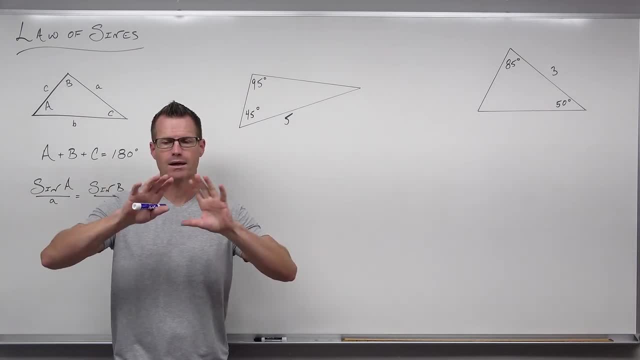 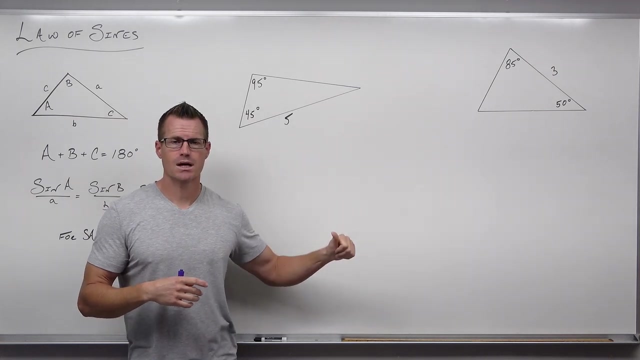 So right triangle trigonometry does not work right there, Like if you're seeing, right triangle trigonometry doesn't work, Put this in the category of all right, I'm dealing with either law of signs or law of cosines. We do need to know what works where three sides: law of cosines, side, angle, side with. 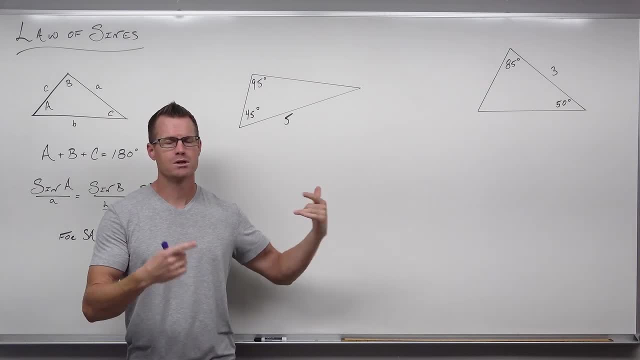 an angle between our sides, love cosines, anything else that we have. We're dealing with law of signs. So notice, we need to know three things to find a fourth in any triangle- right triangles. That was included because you had that right angle in there. 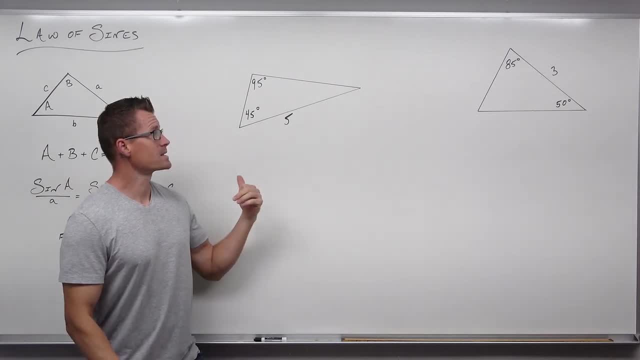 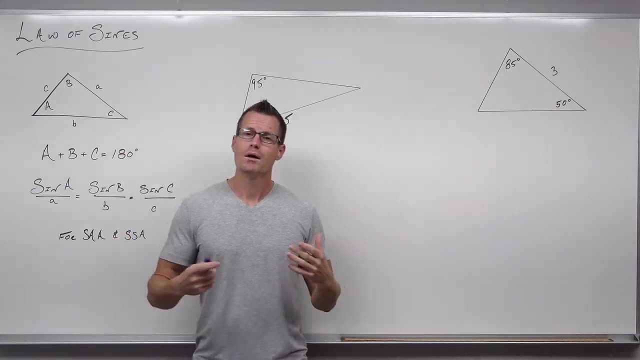 That means you need to know two to find a third, because I already knew one. So let's see, I know an angle and angle and a side. Oh, that's great. Hey, angle angle, side or side angle angle. That's something I can solve with law of signs. 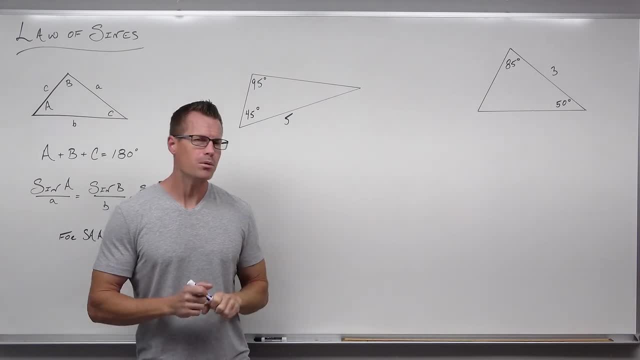 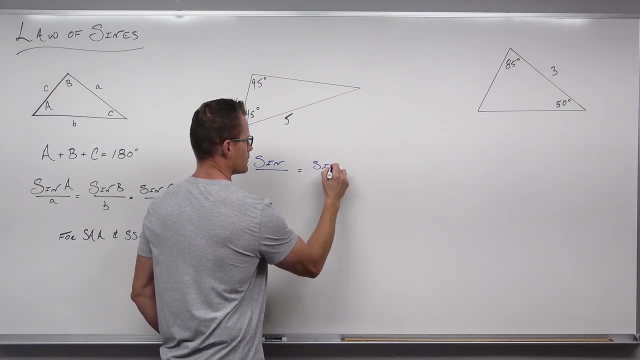 So right in my head, I'm thinking I'm dealing with law of signs. I'm probably going to write this out actually Right out of proportion. If you're going to deal with law of signs, you're going to be dealing with the proportion. 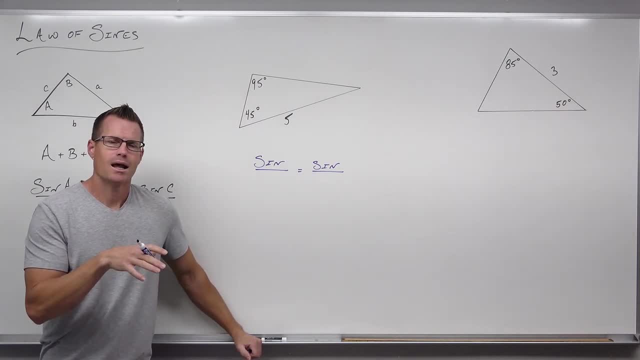 I'm going to write that out now. I'm going to let that kind of hang on for a second and I'm going to do what I've taught you how to do And all of right, triangle trigonometry, use non trigonometry things, or I guess it's technically part of trigonometry. 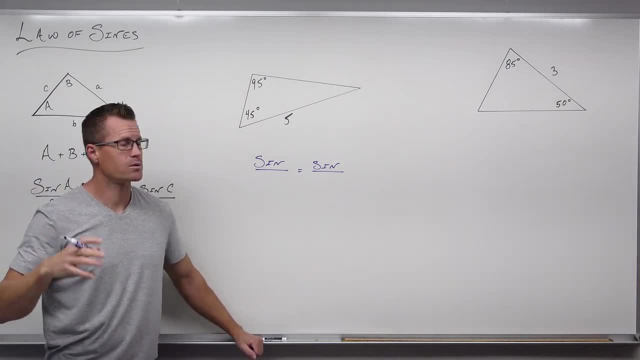 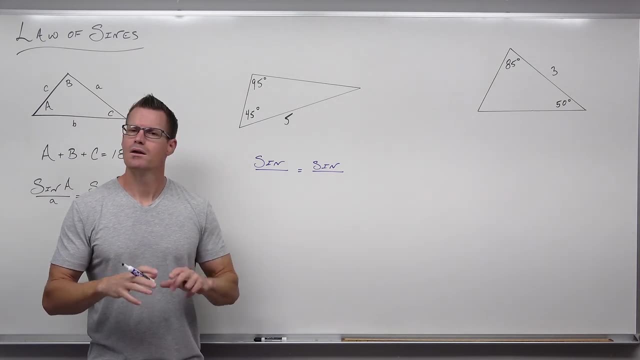 but use things that are not like law of signs or right triangle trigonometry to find missing pieces, If you can. So if I have side angle angle, if I know two angles, the very first thing I'm doing besides checking if it's a right triangle is I'm finding that missing angle. 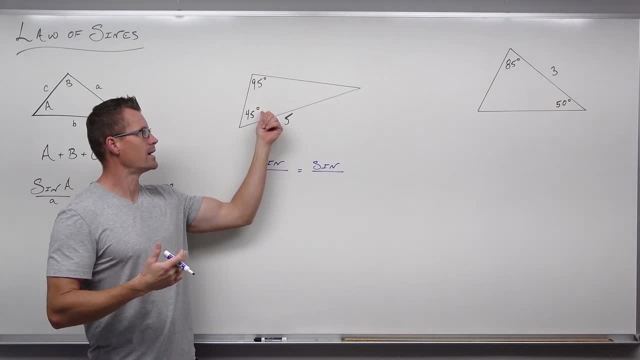 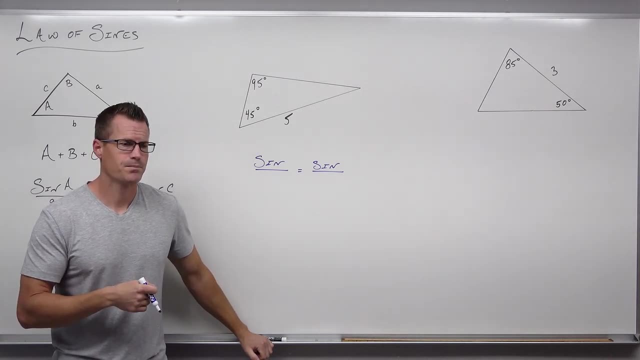 So if I know that this is 95 degrees, and now that I know that that is 45 degrees, I'm going to put this is well, 180 degrees minus those two angles. Another thing we might do, as we're doing that is start labeling your triangle. 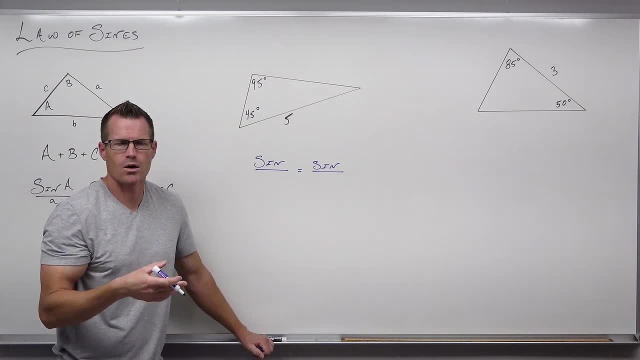 So I'm going to subtract 180 minus those two angles, but it is 90.. Nice to call them something. So here's. here's one point, though It doesn't matter what you call them: They could be angle a, B or C. 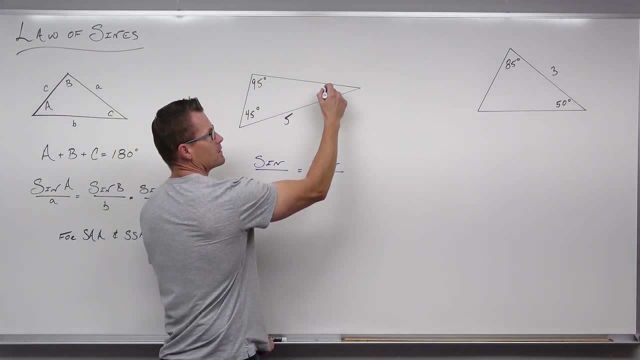 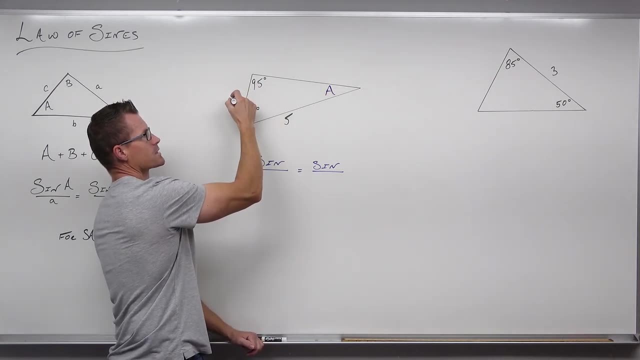 It doesn't really matter. So just just pick a letter. So I'm going to pick a and then after that everything kind of flows into place as far as your sides. So this is angle a. let's call this little a. I don't care what that angle is. 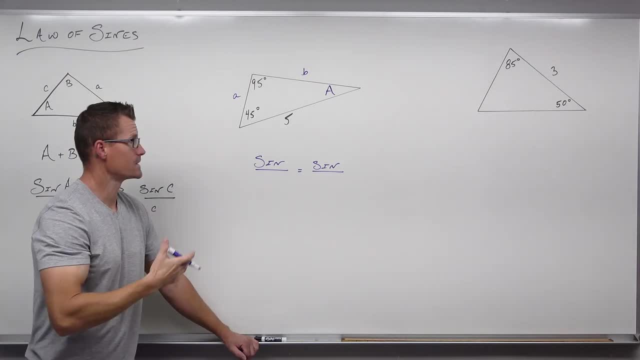 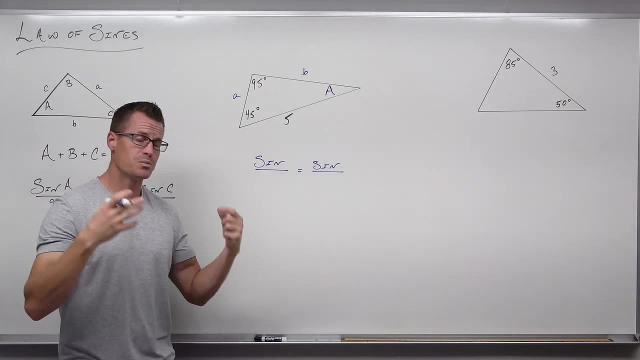 Let's call this little B or lowercase letter B. Why? because it doesn't matter if this is ABC or ABC for sign law of signs of work, All of signs. It does is puts sign of two angles and sides opposite them in a proportion. 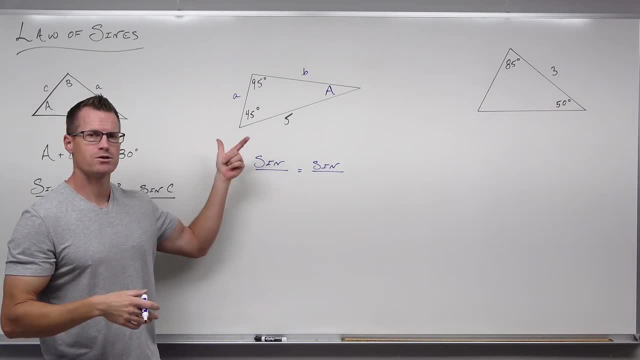 So you can cross, multiply. It's all it does. So I've looked at this. I said: not a right triangle. I thought, okay, What do I have? I've got two angles in the side. Great, I know three things. 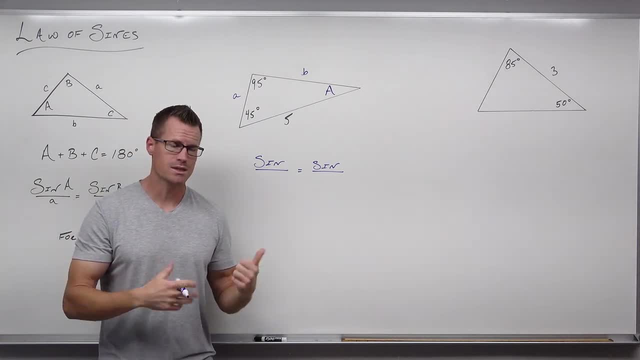 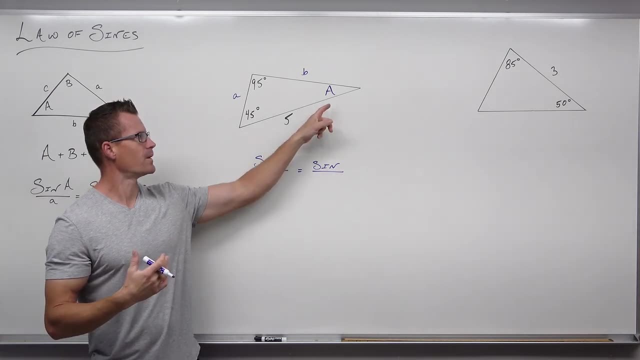 What category does it fit? It fits law of signs, because two angles- one side is dealing with law of signs. I've written out my proportion. I know I'm going to fill this out in a minute. I've labeled a triangle using a because it was a missing angle. lowercase letter a because it's opposite. 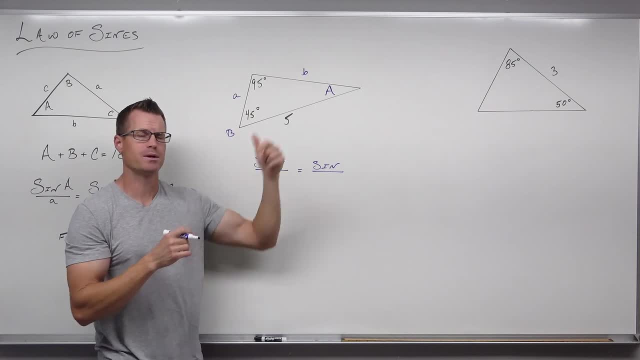 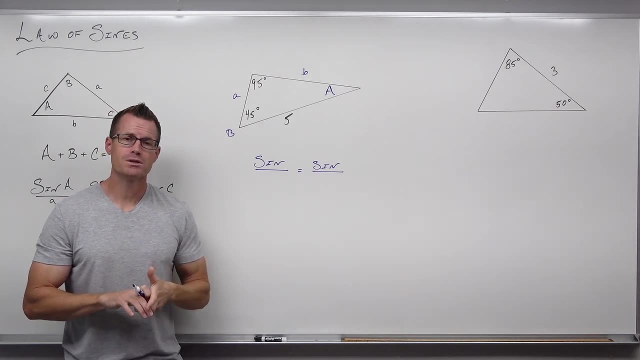 Lowercase Letter B, because if I wanted to call this angle B, that would be the side opposite. again, It doesn't matter whether that's B or that's B, That's C or that C, that doesn't matter. Then I'm going to be using non trigonometry like law of signs: type things to find missing pieces. 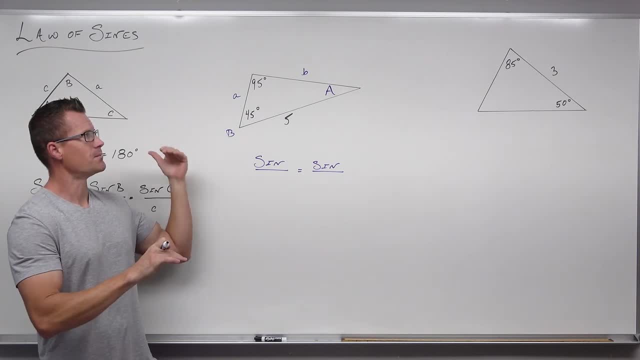 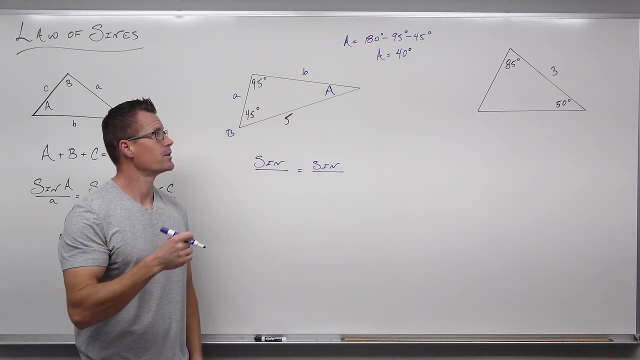 So I can find angle a. angle a is just 180 degrees minus 95 minus 45. So already we know that angle a is 40 degrees. Now here's why that's useful: It's because when you find that angle, you subtracted, you're not compounding error. 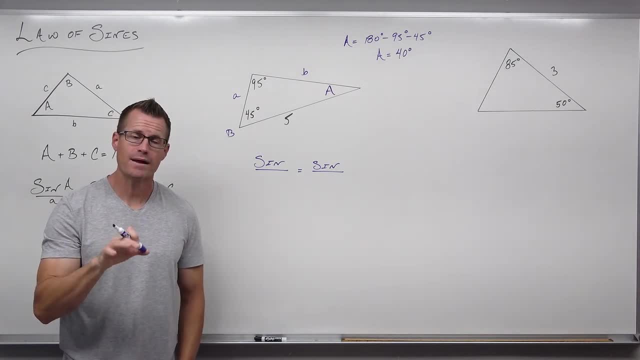 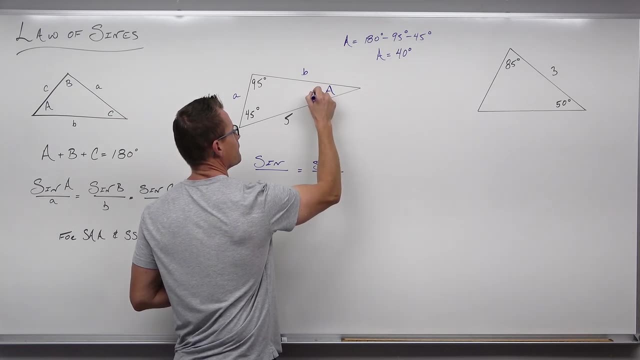 You don't even have any error. We know that this is exactly 40 degrees, and why that's important is because you can now use it in other formulas without having any error. So now we're ready to go. We know all three angles and we know one side. 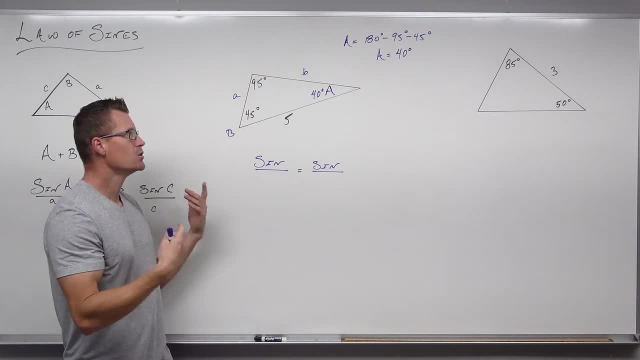 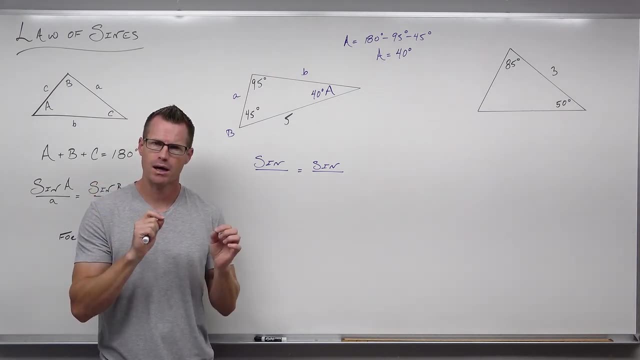 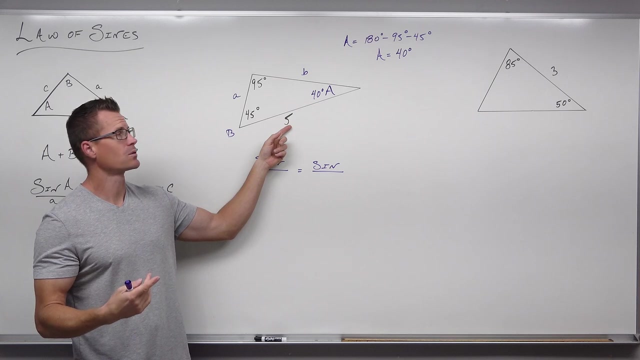 All right, So what do we do now? Create a proportion, whatever side you want to find. all we're really looking for is no three things to find A fourth, So you need to know two angles and one side that's opposite them. What that really means- since that's the only side we actually know- is we're going to have to create this proportion with an angle over the side. 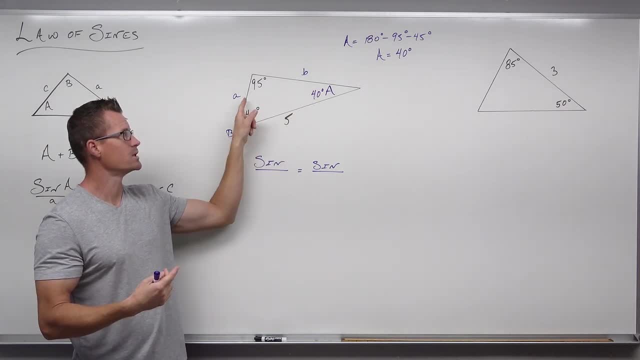 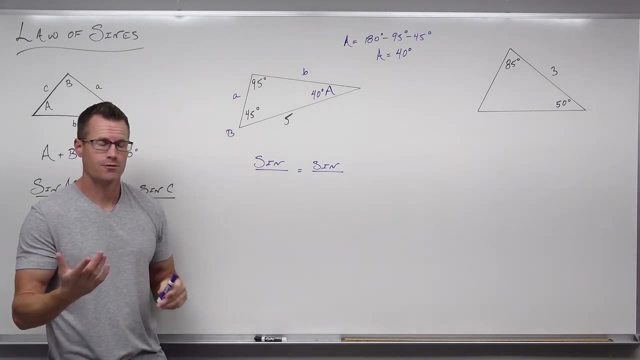 We know equals an angle over side- We don't know- or an angle over side We don't know. that means you can be doing two equations here. Let's go ahead. Let's solve for lowercase letter a first. So all we're going to create a portion. 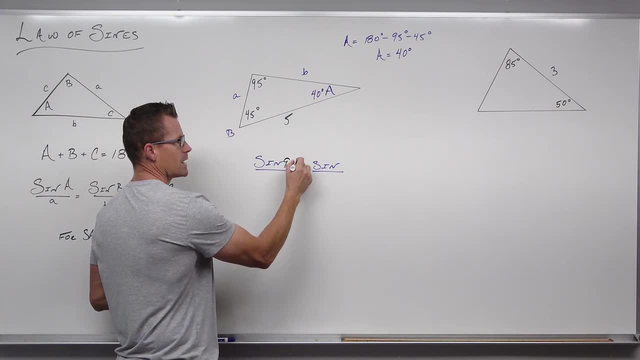 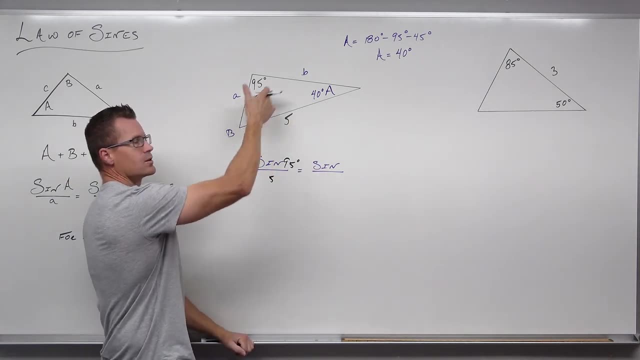 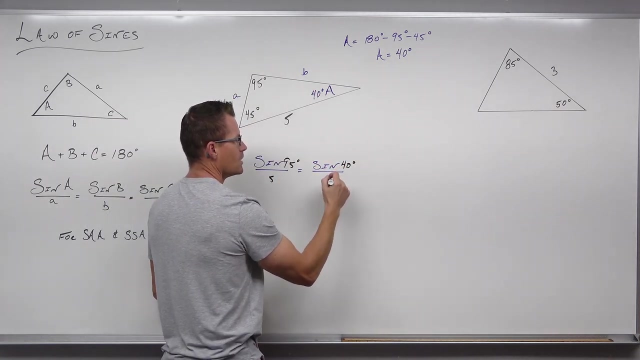 We say, hey, sign of 95 degrees, An angle, I know, over five. the side opposite, that I do know. equals sign of. either one of these will work. use 45 over B or 40 over a. I said I'm the software a, so I'm going to take side 40 degrees over side a. so now that we have that, we have sign of 95 degrees over five. 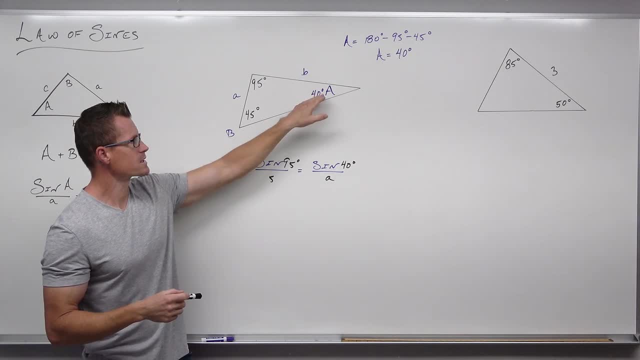 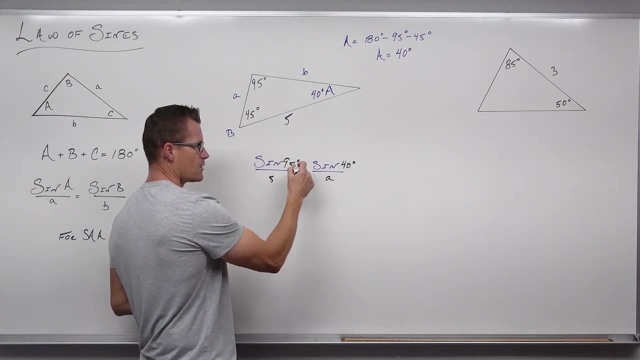 That's an angle I know over side that I know equals sine of 40 degrees over a. that would be an angle that I know over side that I don't. I'm going to cross multiply. every proportion can be solved like that, So let's do it. 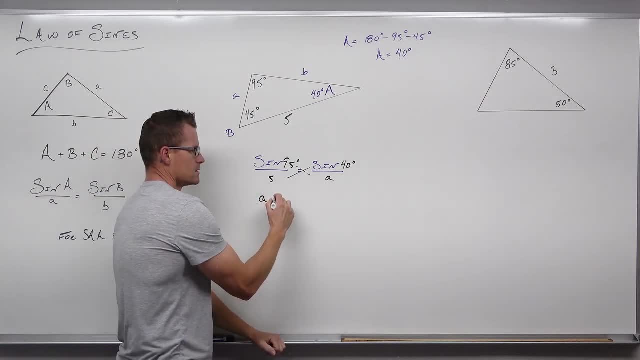 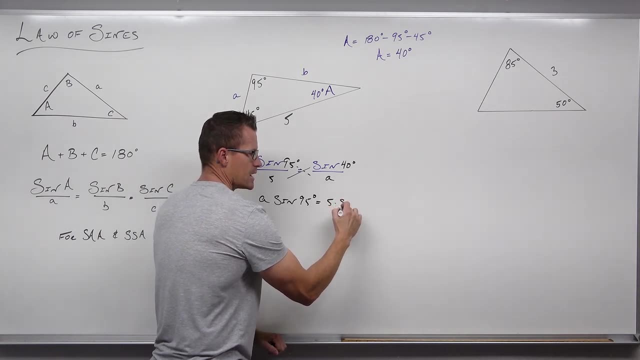 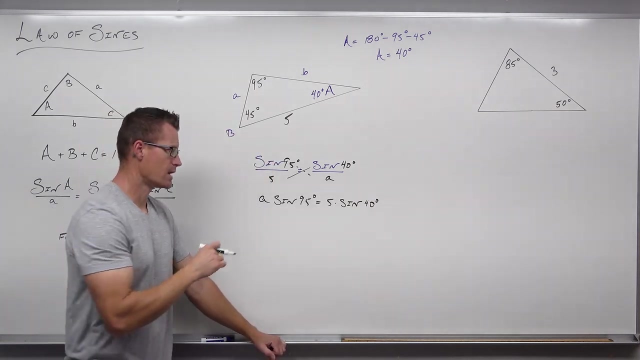 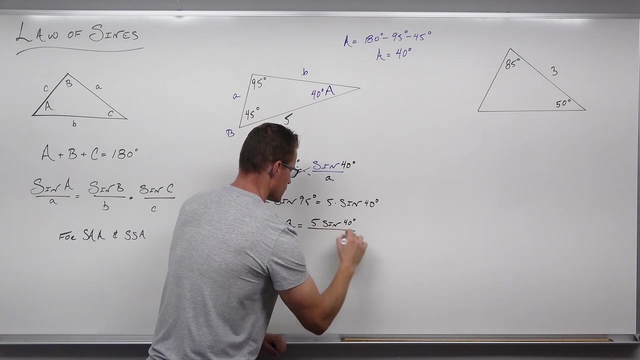 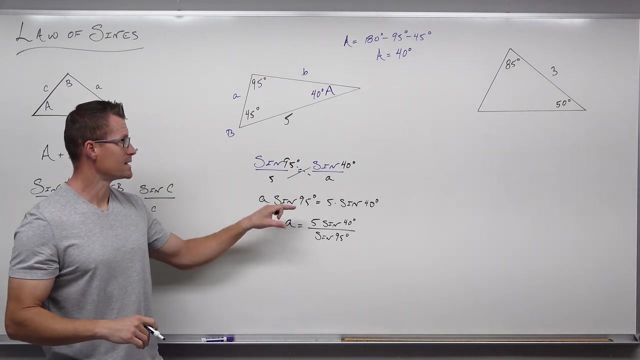 What we're going to end up getting is a times sine of 95 degrees equals five times sine of 40 degrees. If we divide both sides by sine of 95 degrees, This is what's called an exact answer. This is the exact length of that side. use lowercase letters for your sides, that way when you solve them. 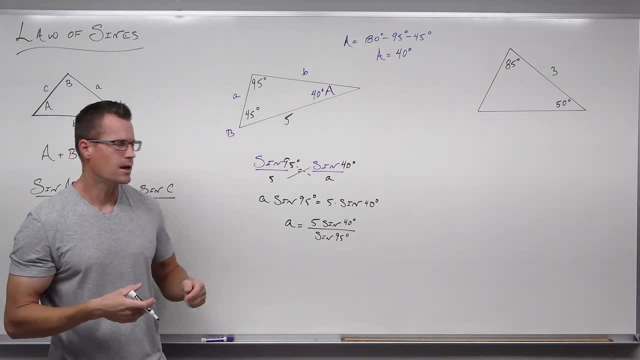 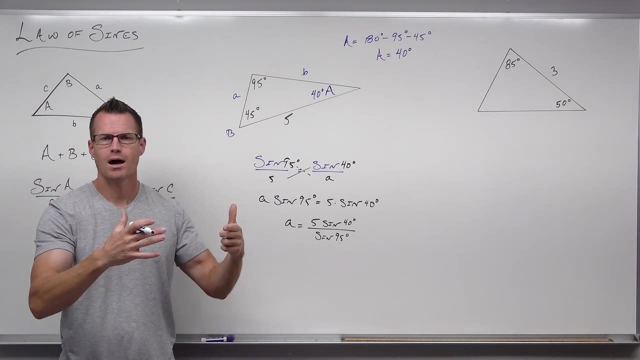 you won't make the mistake and actually call a side and angle or something like that. So that's a side length. This is the exact amount, but it's not super useful in application because we don't really understand how much that is. So we're going to approximate. 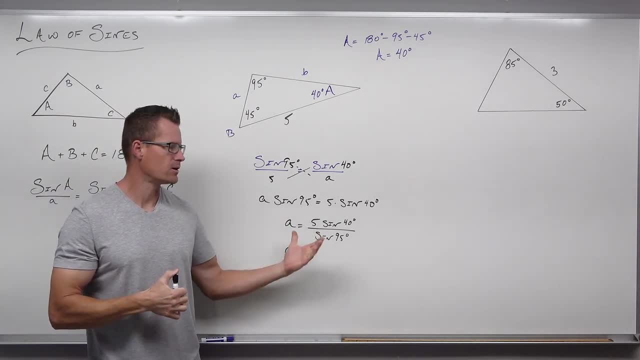 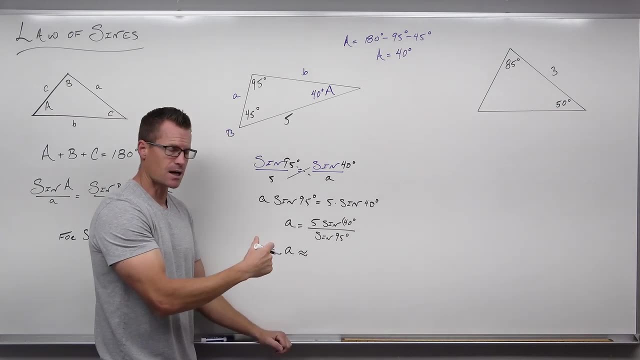 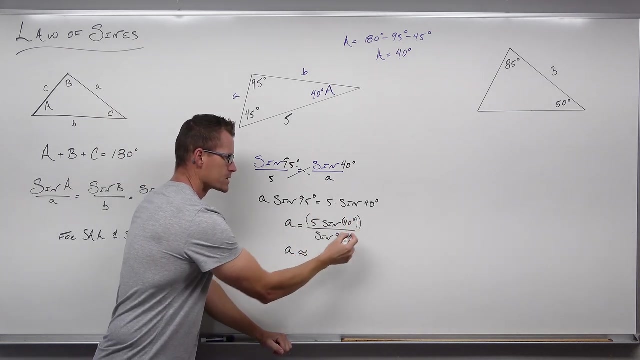 You can put this entire expression on your in your calculator if you use parentheses appropriately. So most calculators. what they do is they would open up a parentheses around that sign So close that before you start plugging this in, put a parentheses here and then close that one and then press divide or press fraction and it'll make a fraction out of this. 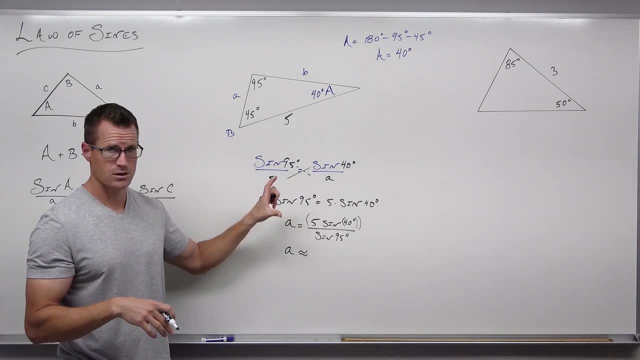 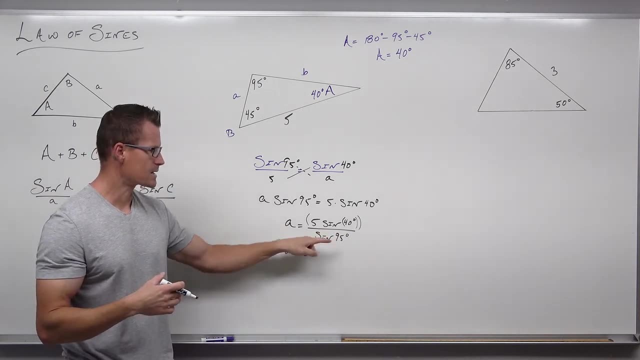 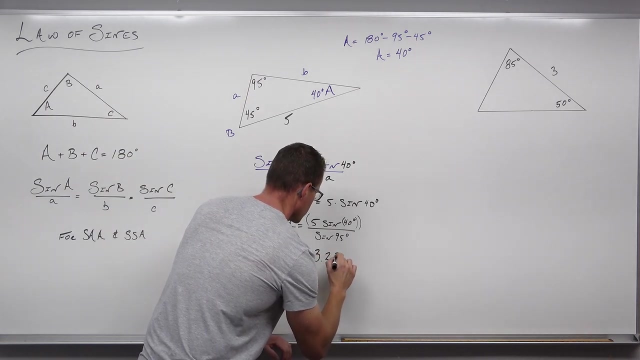 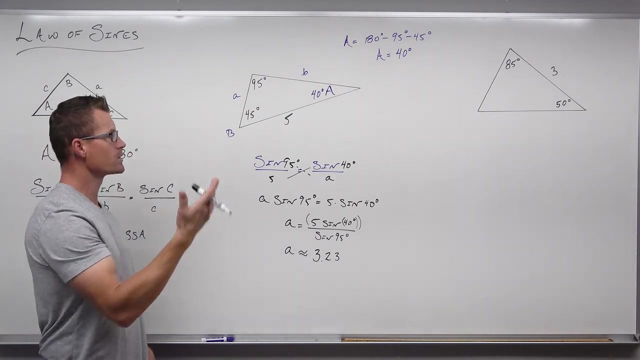 So I would put parentheses five sine and that's going to open parentheses: 40 degrees. I'm going to close that one, close my, my numerator, Press, divide or press fraction and then sign 95 degrees. Make sure your calculator is in degrees. We get that a. that side is about 3.23, whatever the units are, and give you any units here. 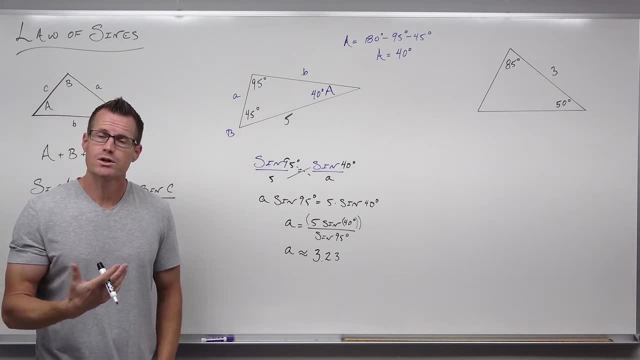 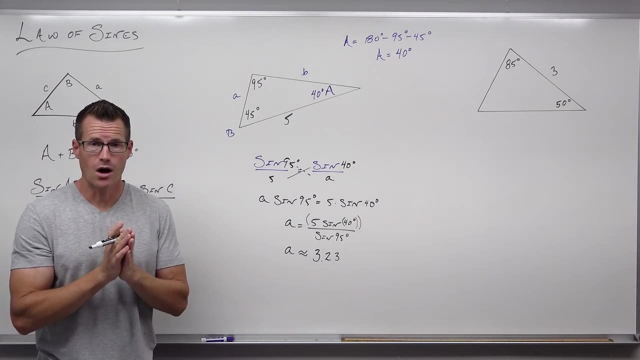 but 3.23 units in this case, which is pretty impressive that we can do that. now Here's what not to do. Begging you, please don't do this. Please do not try Pythagorean Theorem with this being 3.23.. 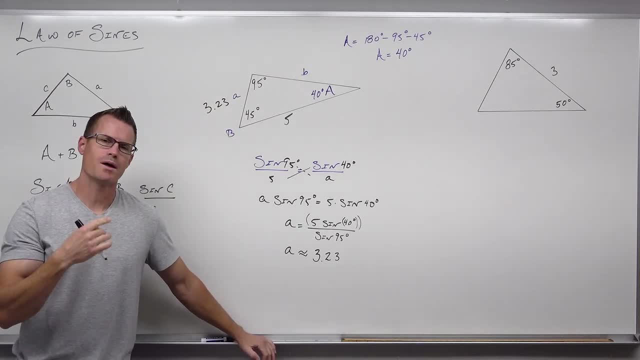 Why not? two reasons. number one: that's not a right triangle, So Pythagorean Theorem will not work. Secondly, that's rounded, And so, if at all possible, we do not want to use rounded values in future math. Now we're going to come up with some cases that you have to like law of science. 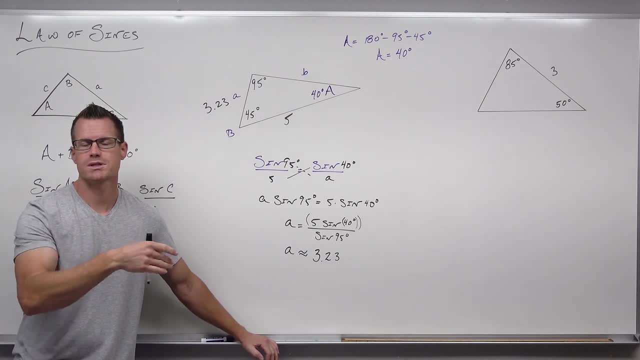 Sometimes you have to, especially when we have multiple steps in a problem like the last example to give you, but try not to because that compounds your error. So we've looked at it. We said that is angle, angle side. Great, find another angle, put it in there. 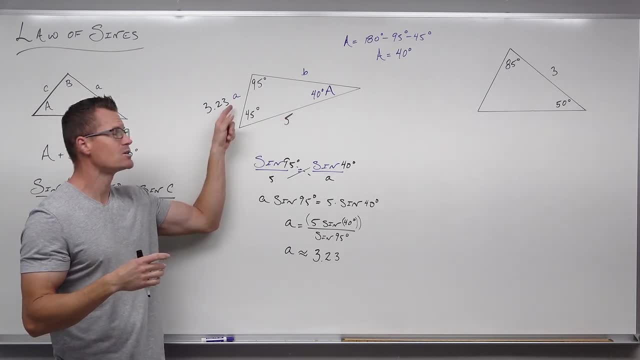 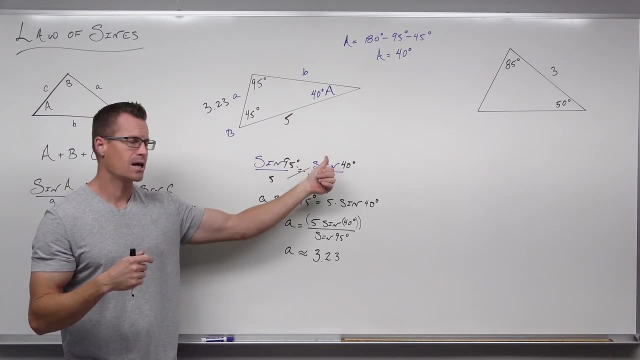 Now you can use that. find other other pieces- and you actually had to to find that. then create law of science as a proportion. angle, you know over side. you know equals angle, you know over side, You don't. then you can cross multiply. next find the other side. 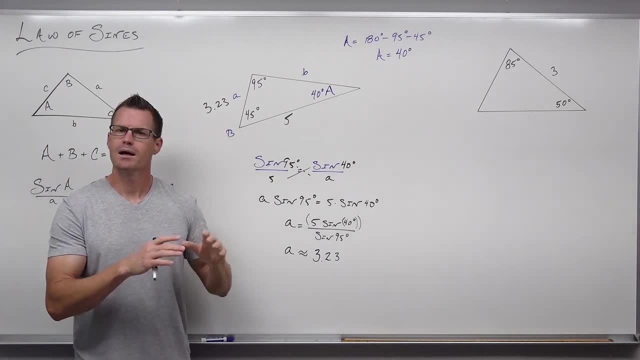 but do not use that in your proportion. Why we just talked about it? if that has error in it, Because you rounded says it right there. Don't use it again. So find another proportion that relates an angle, you know, to a side you, you also know equal to an angle. 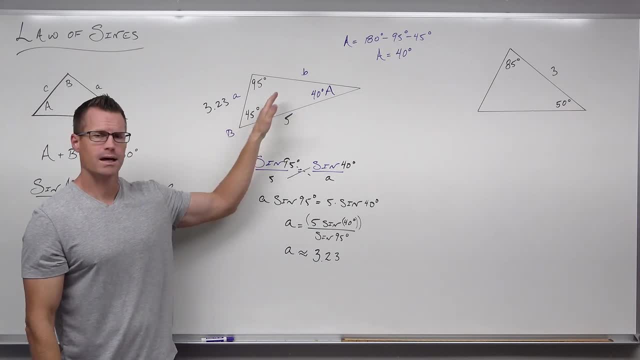 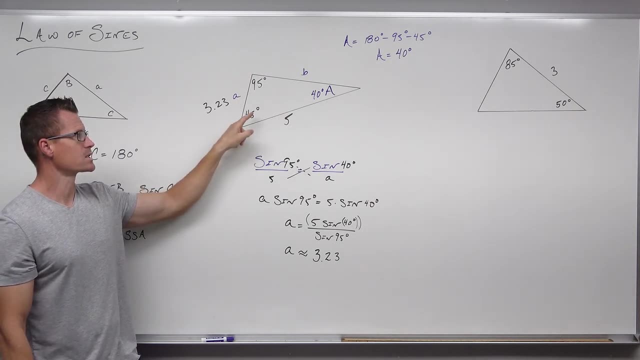 you know over the other side You don't. if you know all three angles, it's fine. You should be able to do this just fine. So we're going to put sine of 95 degrees over 5 again equals sine of 45 degrees over B. 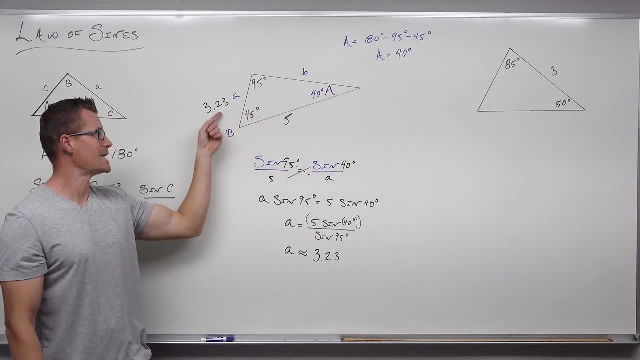 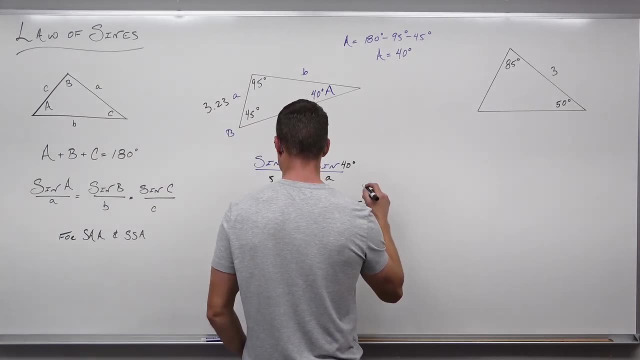 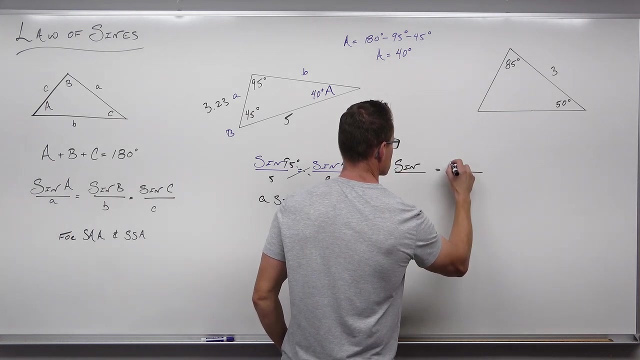 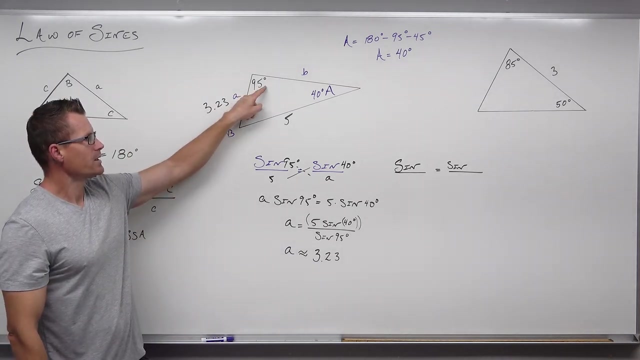 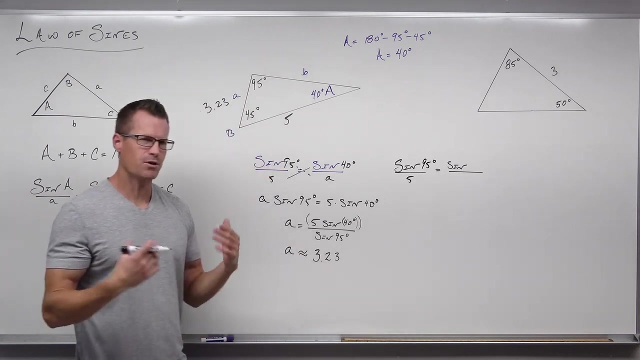 You do not want to use this as your known angle inside because that is not really fully known. It's an approximation, So we take a look at it again. angle: I know over side, I know using stuff that was given to me, not stuff that I found that I rounded equals angle. 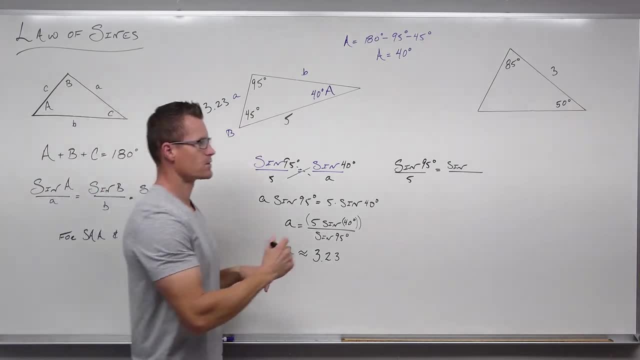 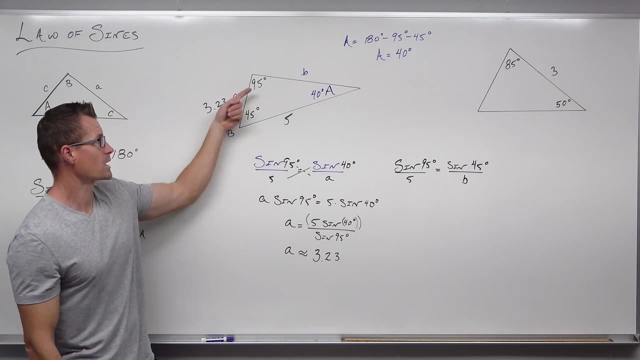 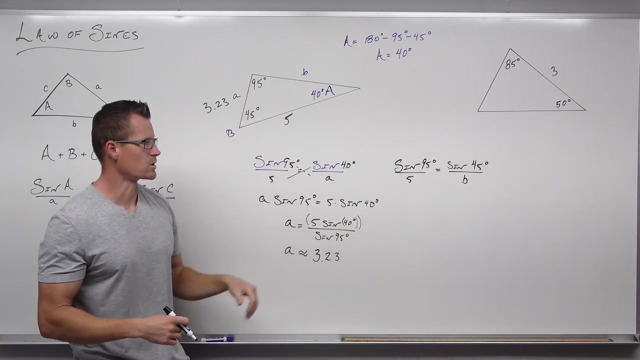 I know over side. I still need to know, want to find. so 45 degrees Over lowercase letter B. So I'm gonna double check. Yes, this is angle and opposite side. This is angle and opposite side. I'm not using approximations, looks really good. 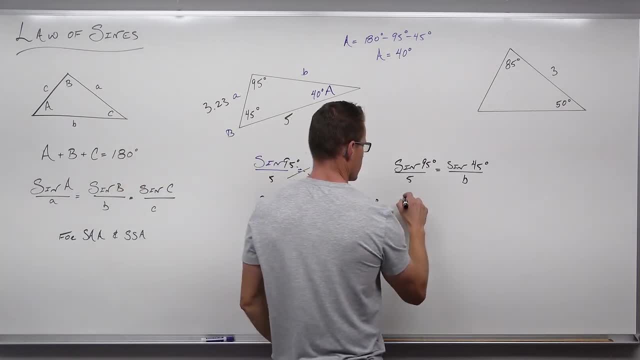 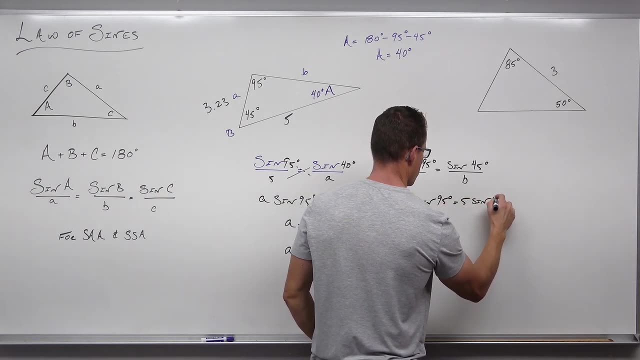 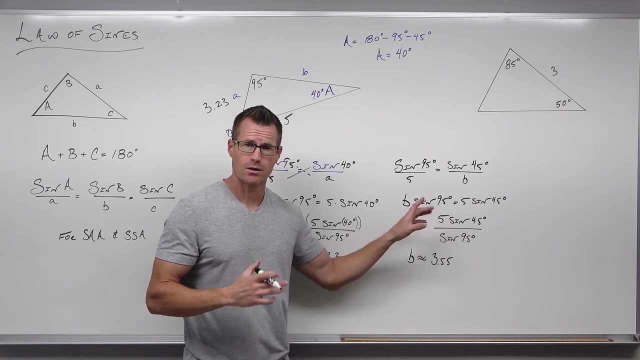 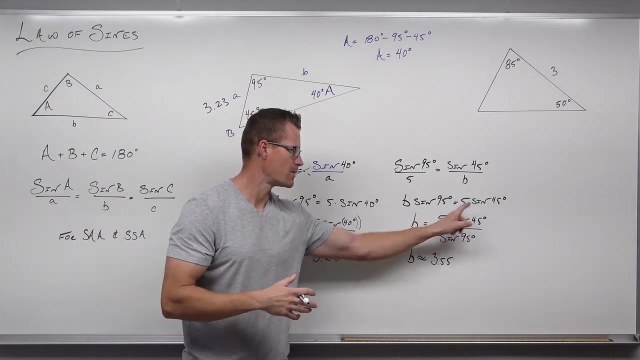 Now we can cross, multiply and divide. So we've done the work. We've cross multiplied, We divided. I put this in my calculator all at one time, Just so I don't make the mistake of rounding and using that in future math. So I put parentheses here and around my numerator: press divide. 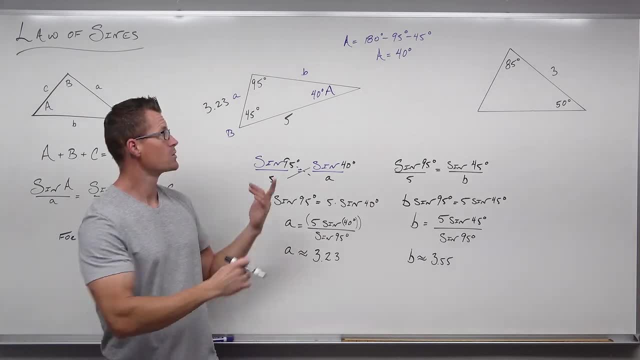 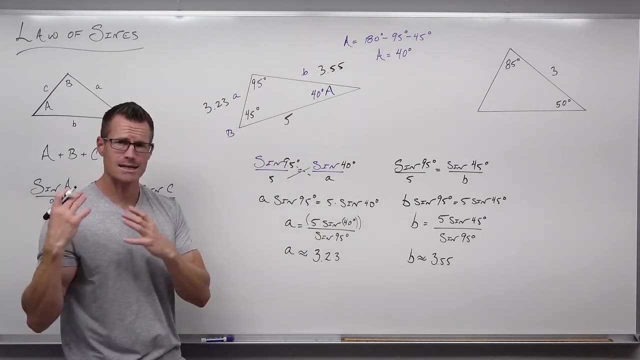 You should end with about 3.55.. You rounded the same decimal place, So this side is approximately 3.55.. That's done. We've solved the entire triangle. We've all three angles. It did not take a lot of signs to do it. 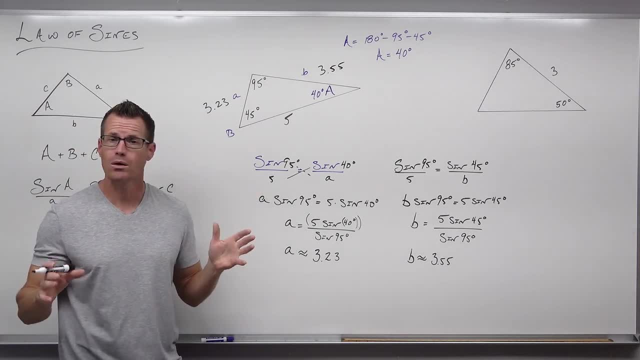 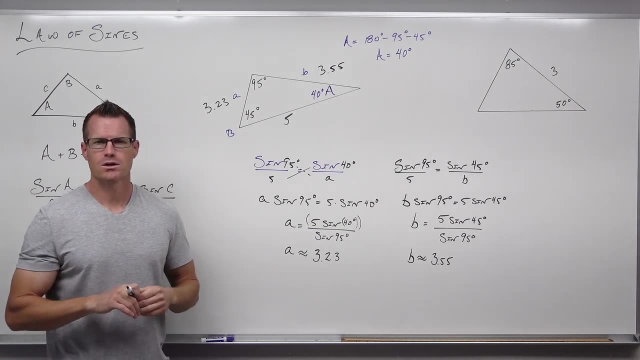 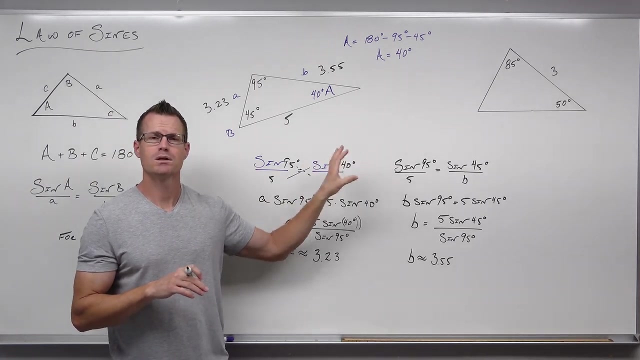 We use proportions to figure out the other two sides. That's it, It's all. offside says creates proportions of you can cross multiply. the last thing I'm going to mention: what if you were to use this on a right triangle? Well, if you were to use this, you would get sine of 90 degrees at some point in your proportion. 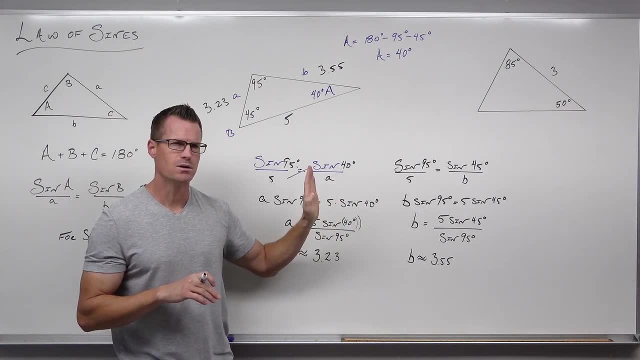 What's sine of 90 degrees? It's the same thing as sine of pi over 2. That would give you just one, and what would happen is you would create just a right triangle trigonometry equation out of that, where you would get sine of an angle instead of sine over sine. 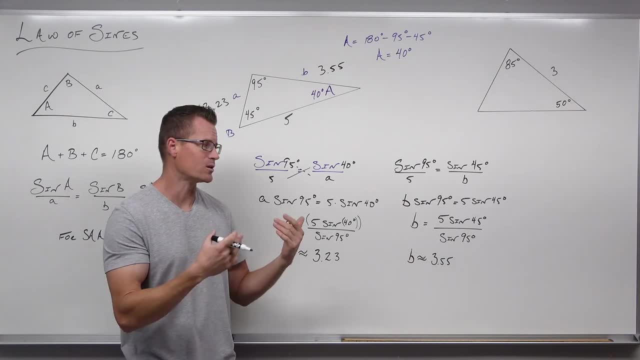 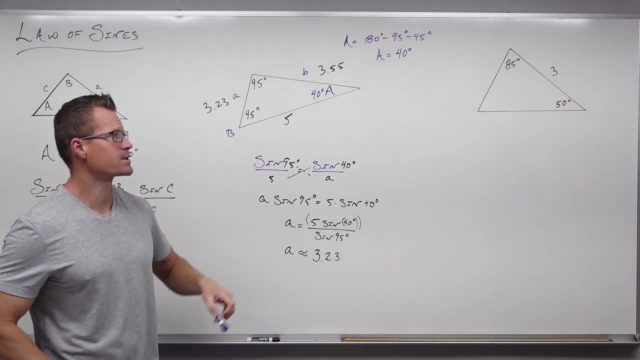 So it's? that's really all it is. You could use it with the right triangle. It's just a sine of 90 degrees: gives you one and eliminates itself from that equation. All right, let's move on and try another example. So I'm going to model my thinking. 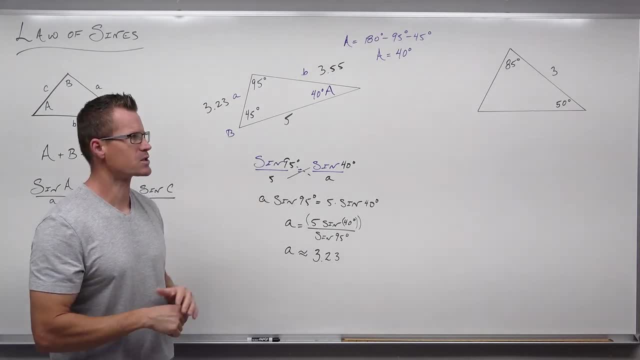 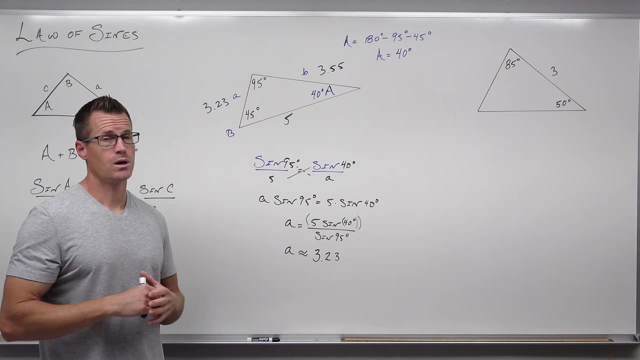 I'm going to move a little bit quicker because we've already kind of experienced this once. If you would like to, you should probably stop this video and try that on your own. See if you can solve that using what, what we know about it. 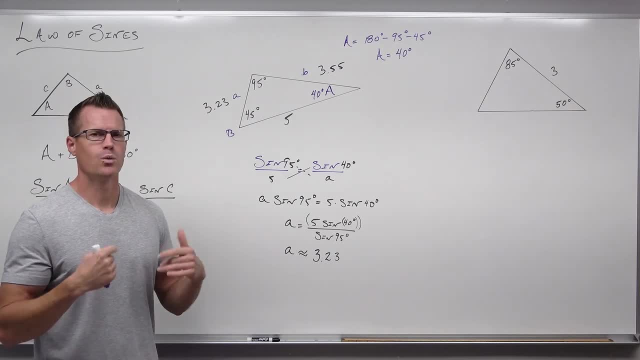 So here's here's my thought process. The first thing I'm looking for is: will right triangle trigonometry work? Can I use sine cosine tangent and make it easy on myself? It doesn't look like it because that's not a right triangle. 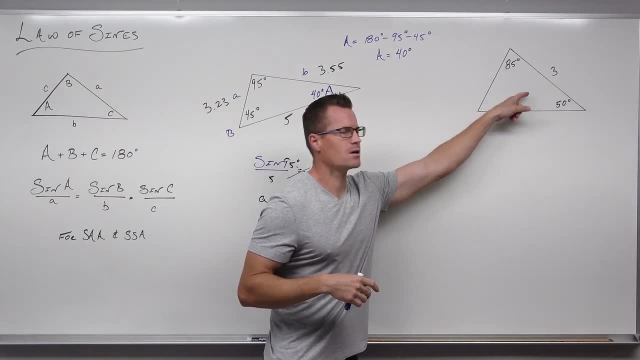 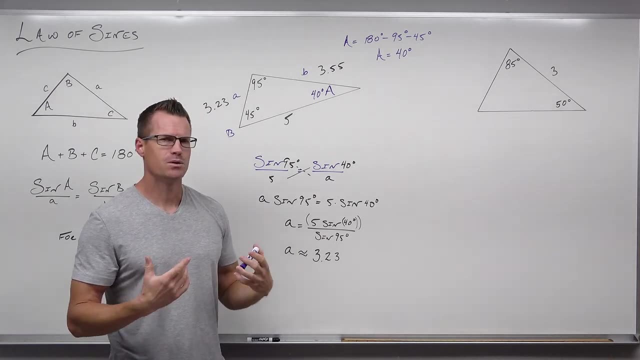 So how do I know it's not a right triangle? I'm doing some math kind of quickly in my head, realizing that's also not 90 degrees. So this is not for sure not a right triangle. The next thing I'm doing is I'm probably thinking what's going to work to solve. 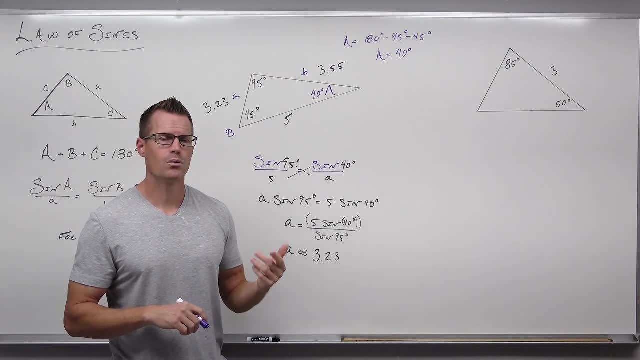 So I'm looking at this going: Hey, I know two angles and I know one side. with two angles in one side, It means I can use law of science for this. So in my head I'm thinking law of science. The other thing I'm thinking is, if I know two angles, I'm going to be able to find a third one. 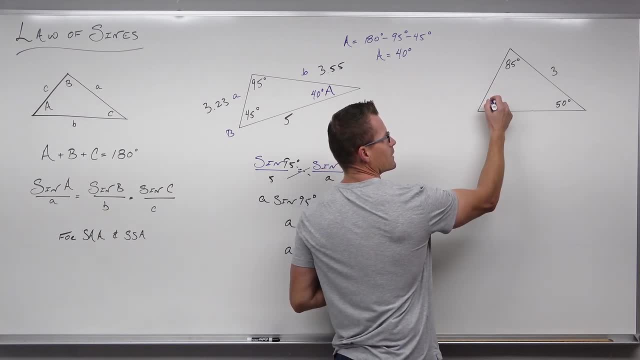 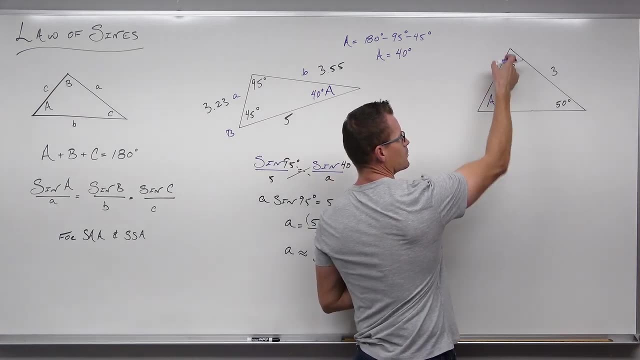 So I'm probably going to label it first and think if this is angle a, Then that would be lowercase letter a. We don't really need to know that right now. If this is angle B, then this would be lowercase letter B. If that's angle C, this would be lowercase letter C. 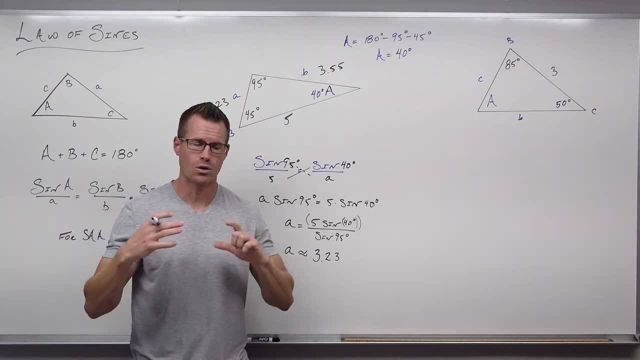 It does not matter what you call the angles of the sides, because law of science only works on proportions. You just need to know two angles in one side to find a fourth, or two sides in one angle to find a fourth piece of information, whether it's a side or an angle. 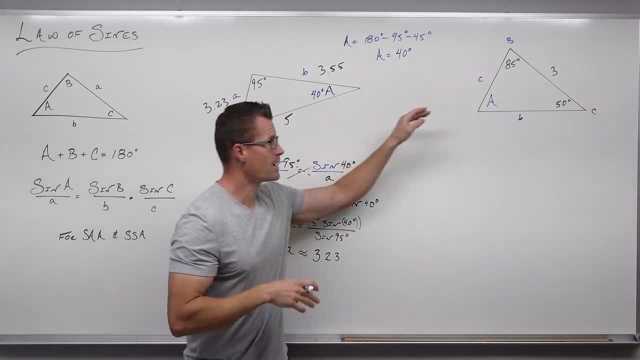 So that's what I'm thinking. I'm thinking not a right triangle, I'm thinking I can find that missing angle first. I'm going to do that first. I've labeled my sides, Now I'm going to use the interior angle. 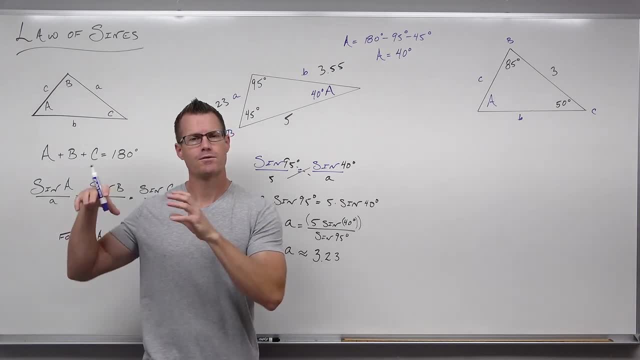 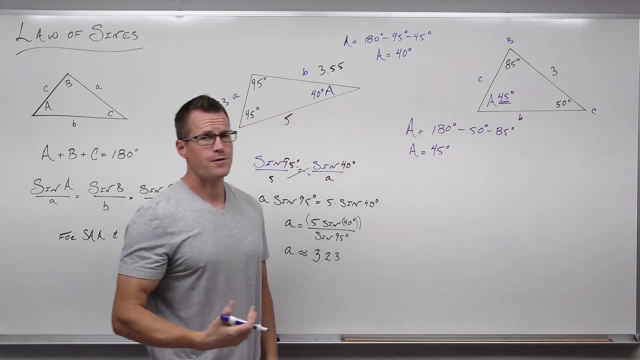 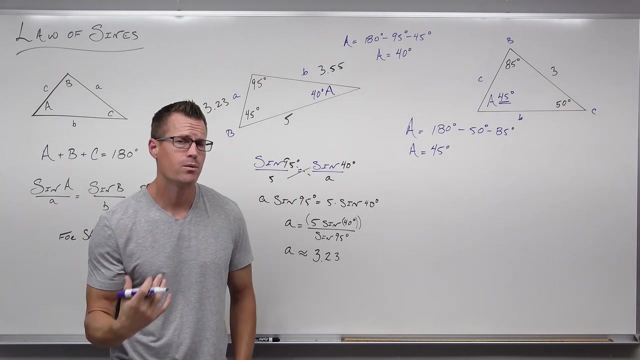 So I'm going to find that angle because I want to do that in order to use it for law of science, So let's take care of it. So we found that angle A is exactly 45 degrees. This is not an approximation. This is why we can use it in our law of science and why we want to find it first. 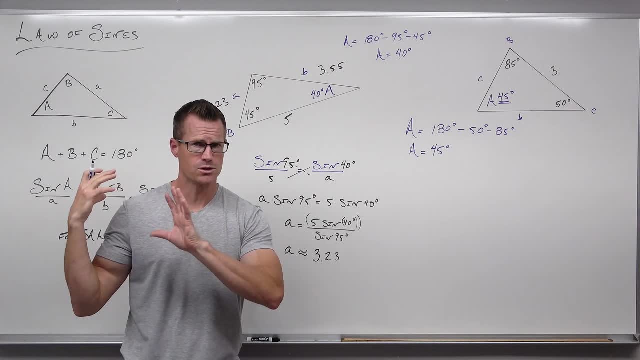 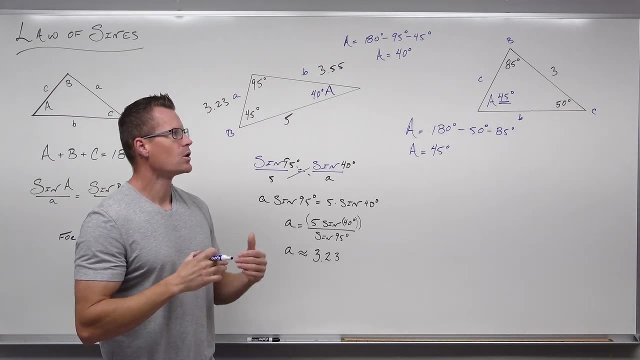 So I thought: what do I need to do first that doesn't use the trigonometry I'm about to use, like law of science, love, cosines or right triangle trigonometry- I found that this angle. Now what I'm going to do is look for three things I know and one thing I don't, in a proportion. 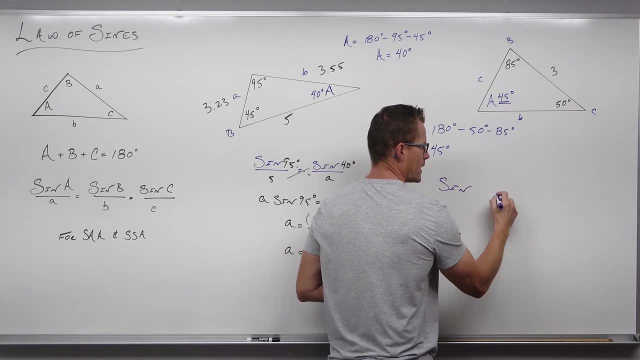 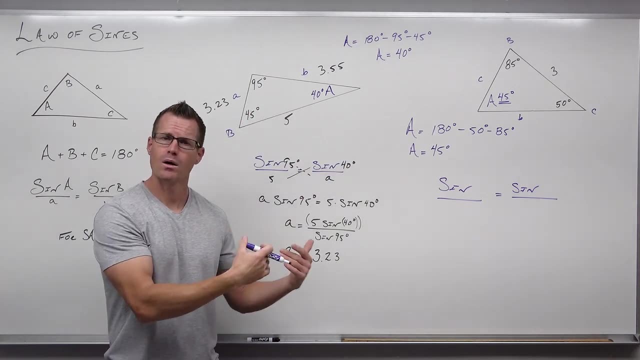 So if I'm thinking law of science, I probably am going to write out the proportion law of science first, the proportion that creates. Then I'm going to put two angles. I know over one side I don't, because that's exactly the case that we have for law of science. 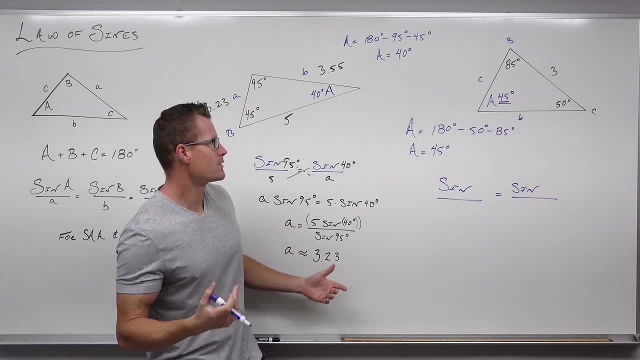 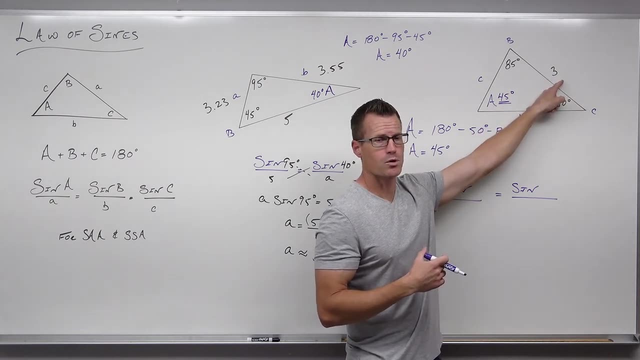 We know two angles, actually three. We know one side, So I'm looking at this thinking, hey, this is the only side I know, So I'm going to have to use this angle with this side in one proportion. I don't know the other sides. 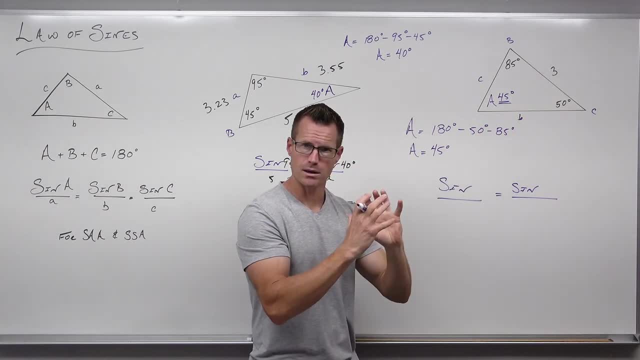 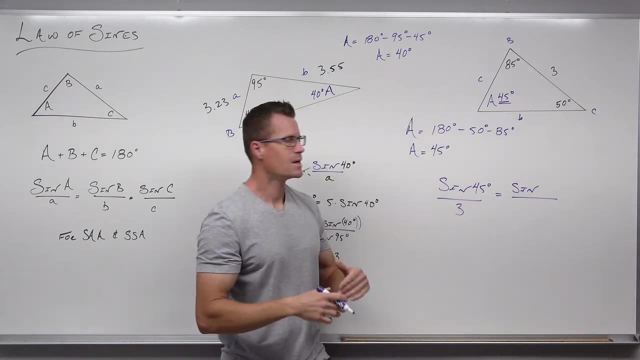 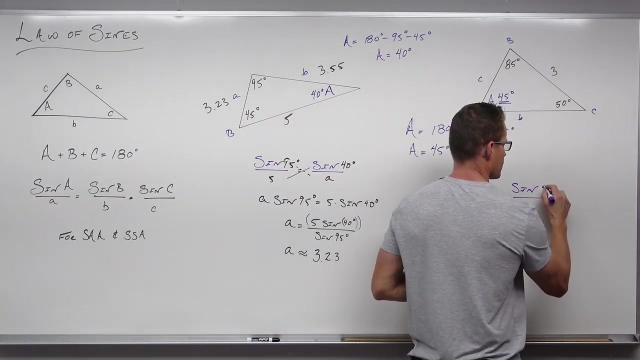 So I'm going to take sine of 45 degrees over three, an angle I know over a side that I know that is opposite Equals any other angle over one of the sides that you don't know. I'm going to pick sine of 50 degrees over the side opposite it. 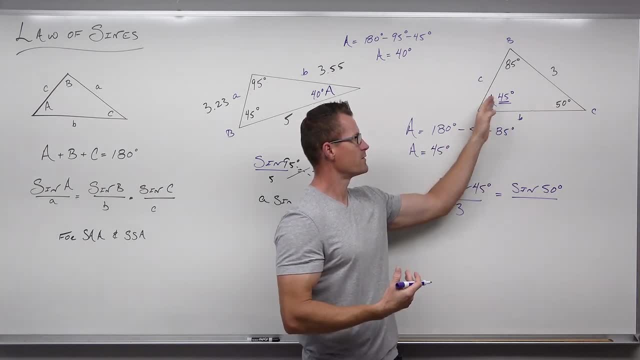 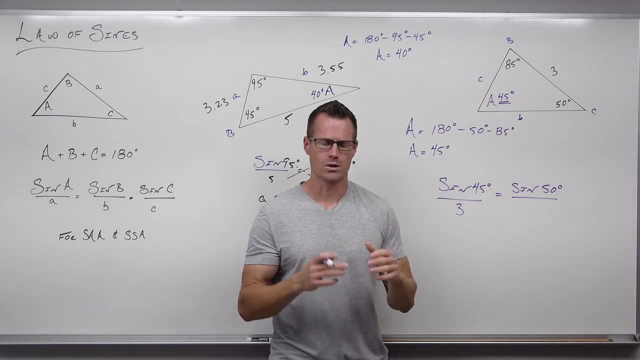 Now here's what you can't do. Don't go. sine of 45 degrees over three, That's great. That's an angle over on the side equals sine of 50 degrees over B. That's not how law of science works. Law of science takes an angle over its opposite side. 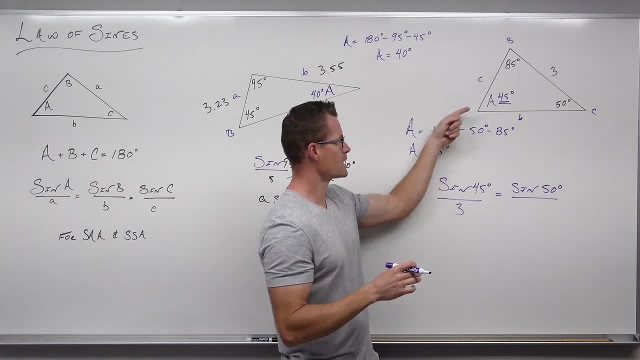 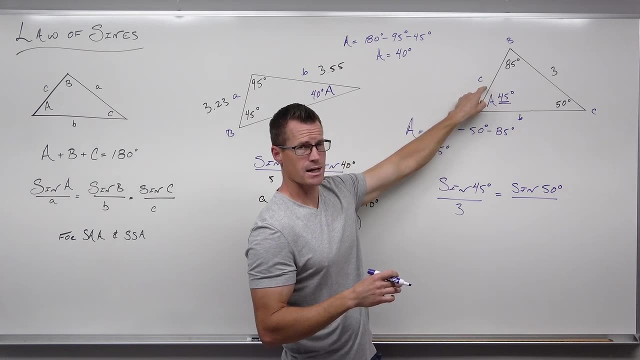 So as long as you're doing that, that should be fine. So I thought: sine of 45 degrees go across the triangle, That's the opposite side. Sine of 50 degrees go across the triangle, That's the opposite side. It's going to be lowercase letter C. 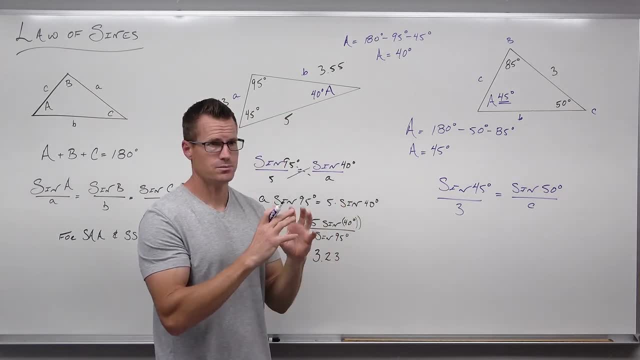 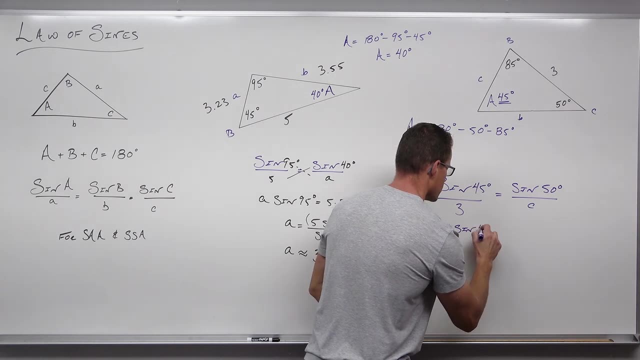 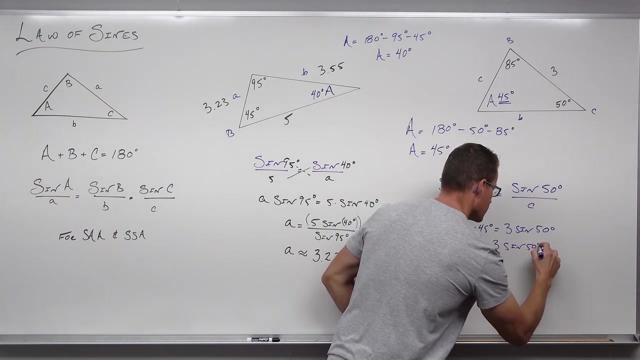 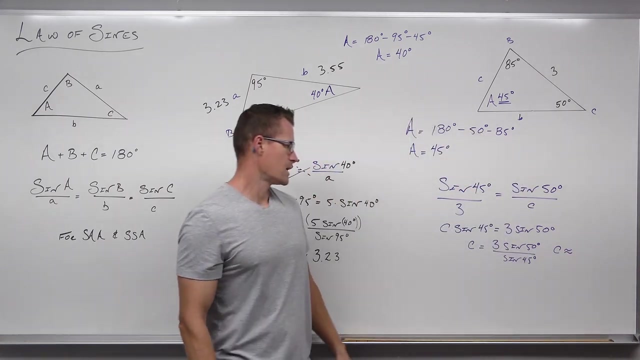 If we cross, multiply and divide- which you can do pretty quickly- We're going to get C times sine 45 degrees, equals three times sine 50 degrees. And if we divide, we get three sine 50 degrees over sine 45 degrees. 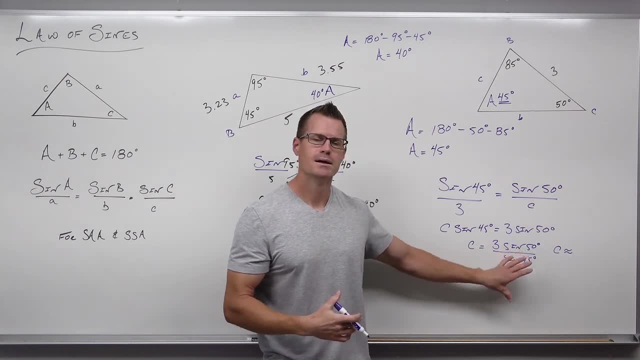 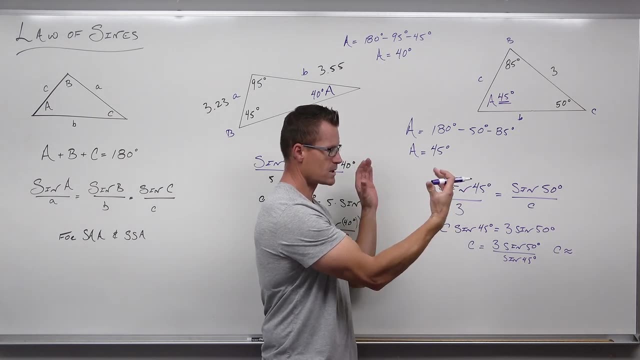 And we use our calculator, We're going to get an approximation. This would be your exact, exact solution. But that right there. Well, let's see, We can put this in parentheses: three sine 50 degrees in parentheses again, And this parentheses over. 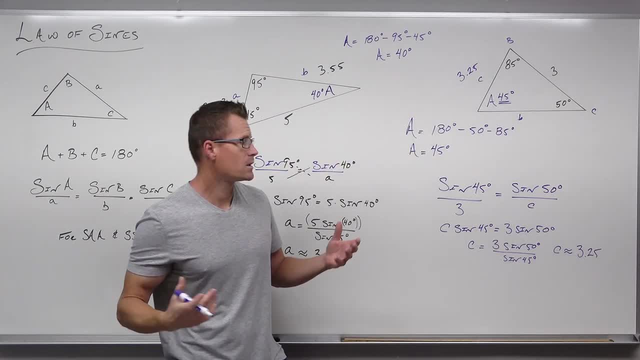 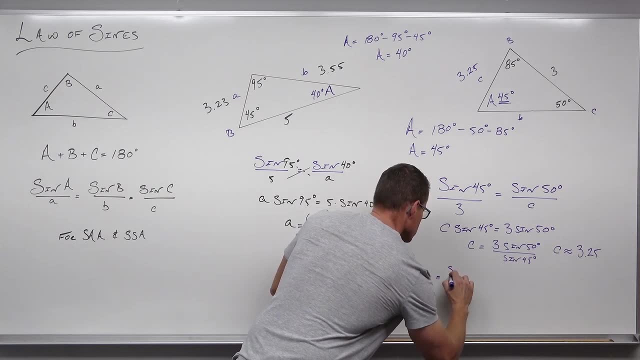 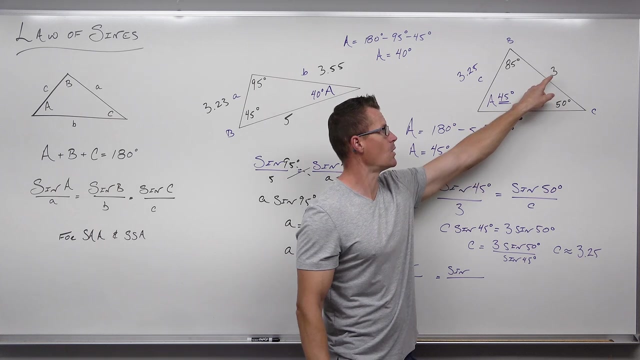 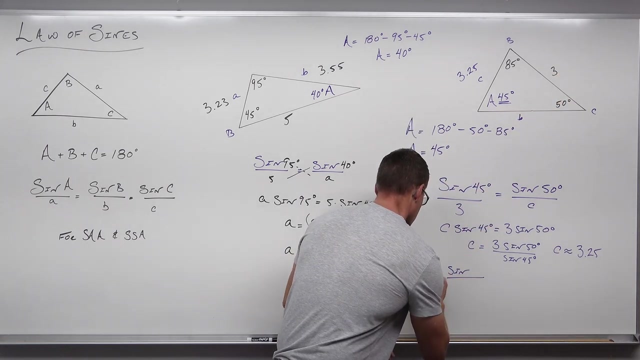 45 degrees We get approximately 3.25 units. So I'm going to create my proportion, But really I'm thinking I've got to use this proportion again because it's the only side I know that is not rounded. So sine of 45 degrees over its opposite side. 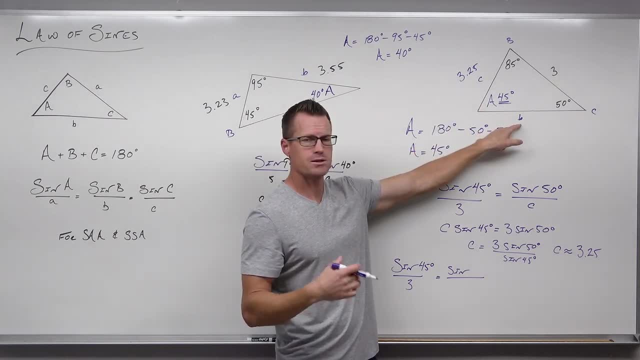 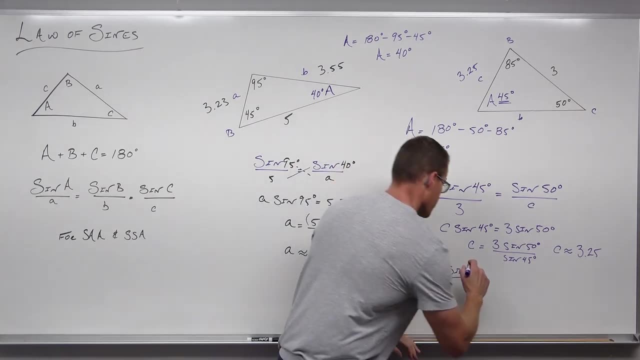 Equals sine of. I want to find this missing side. It's only one left and that's its opposite angle. So I'm going to take sine of 85 degrees over the side I want to find. I'm going to double check. 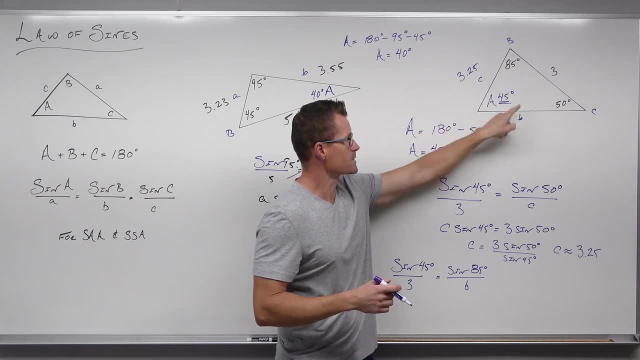 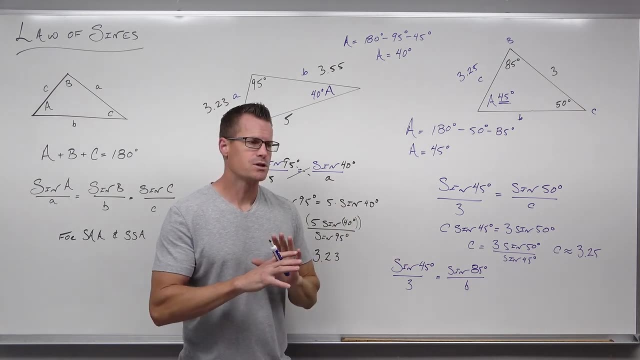 Let's see angle opposite side. Got it? Angle opposite side. that I don't know. Got it? I'm not using rounded numbers, It looks pretty good. So we're going to cross, multiply and divide. Remember there's no, there's no two options here. 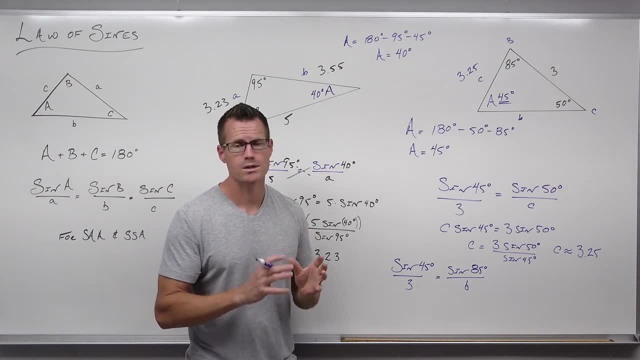 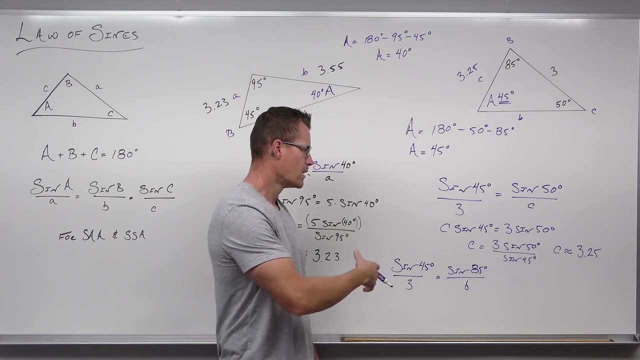 You're just finding a side length and there's going to be only one solution that makes that happen. It's not a multiple case scenario like the next few examples We're going to deal with. so cross, multiply and divide. We're going to ultimately end up with B equals 3, sine 85 over sine 45 degrees. 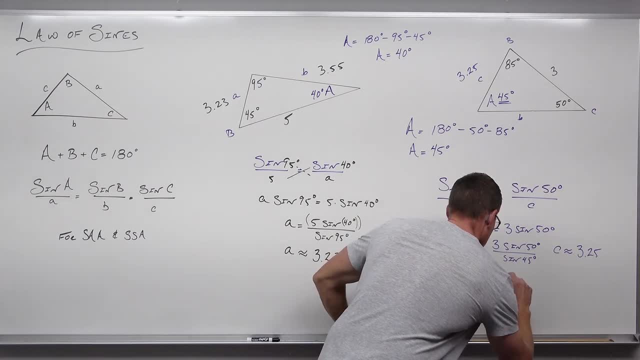 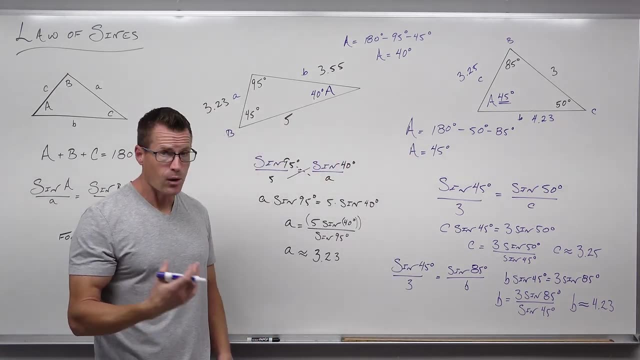 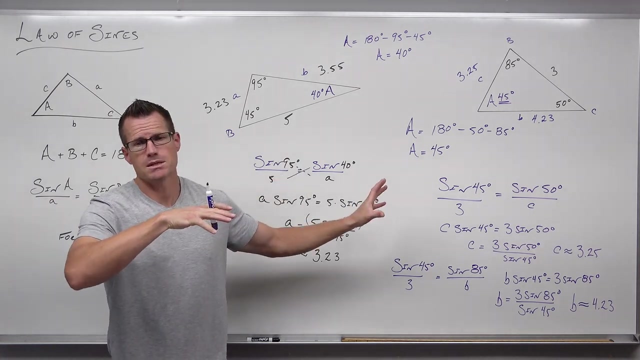 You should really work that out for yourself. We get that B is about four point two, three. So we've solved this triangle. We use interior angle sum to find the missing angle. That was pretty easy, And then we're using the proportions that law of Sines creates. 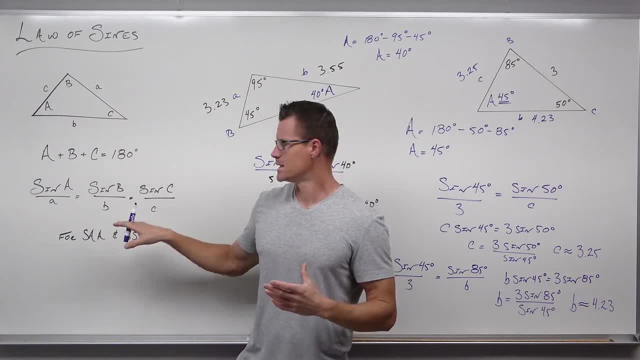 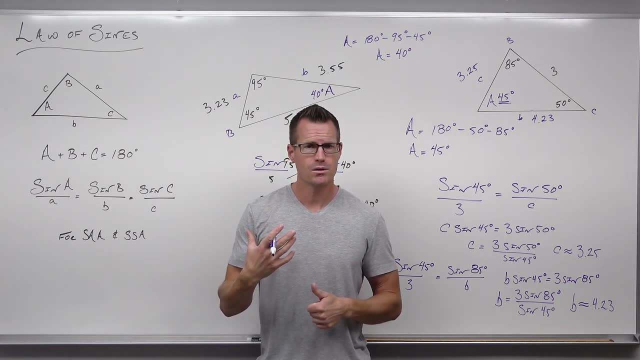 Remember, you're not using all three of these at once. That's not the idea. The idea is this will create a proportion for you of either two known angles and one side that you know to find this inside, or two known sides you know. 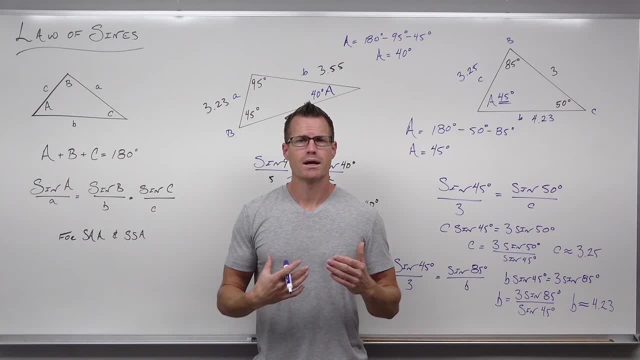 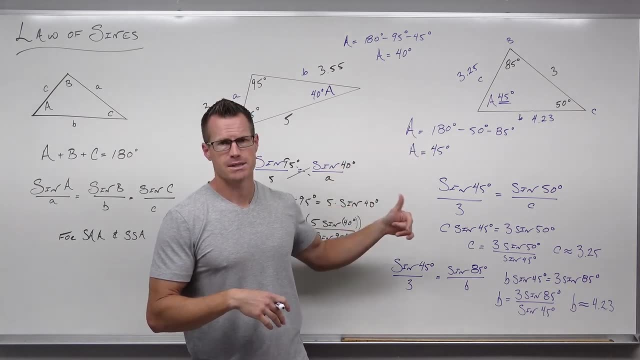 with one angle, you know, to find a missing angle. What we have done right here so far is we just used the two angles we know on a side to find a missing side. That's the easier case We're about to get into. the case where you're trying to find a missing angle. 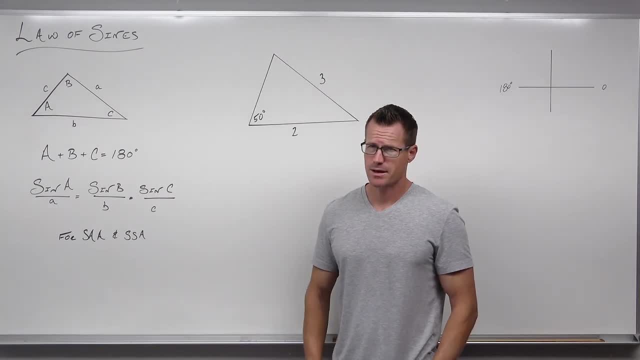 and more options can happen. Okay, let's start another example. We're going to take a look at the case where you're not finding just a missing side with law of Sines, which is what we did. the first two examples. It's pretty easy. 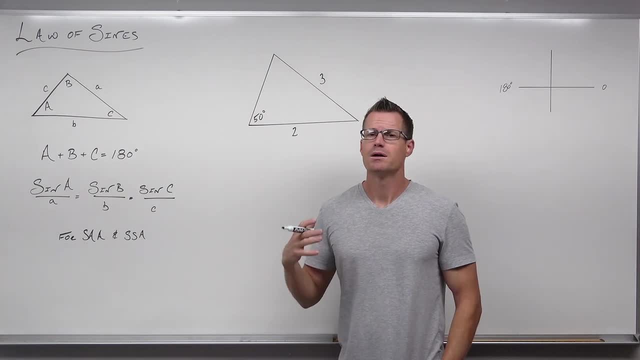 At least it's easier. We're going to be finding the missing angle with law of Sines. We need to be really careful about this. This is one of those cases Where you could have four options. now do you need to know which of the four? 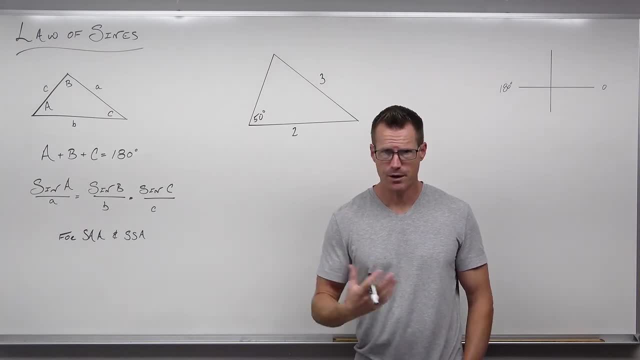 options happens before you go into the problem. No, that's the beautiful thing about law of Sines: The sine function will tell you what's possible and what's not possible, And so we'll deal with that, Not a problem. So let's take a look at it and see if it even fits our model. 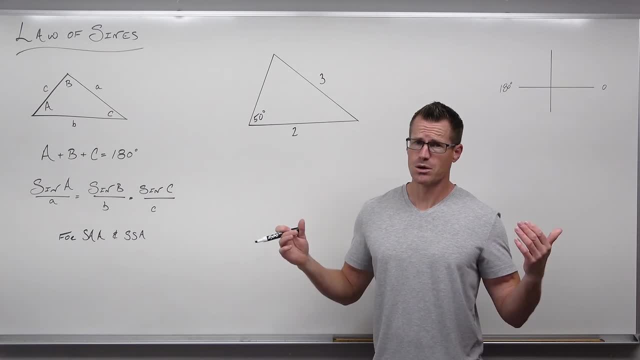 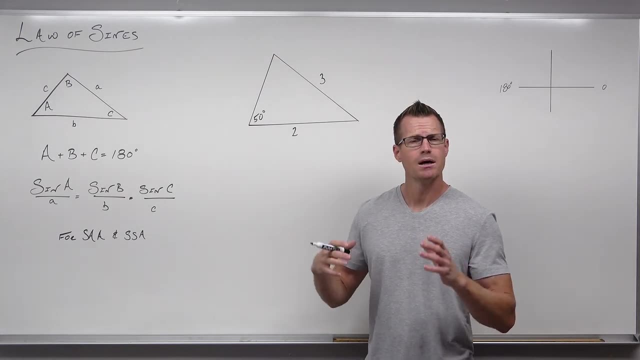 So I'm looking at triangle. I'm thinking. I actually don't know if it's right triangle or not. The only thing that I know is I don't know for sure if it's a right triangle, So I'm not going to be using a right triangle trigonometry. 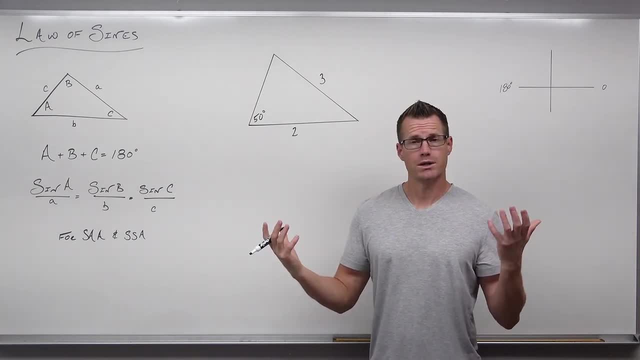 I hope that makes sense. We don't know yet. All we do know is that we are given two sides- Hope you see it- and an angle. Where is that angle? That angle is not between those two sides. That would have to be here. 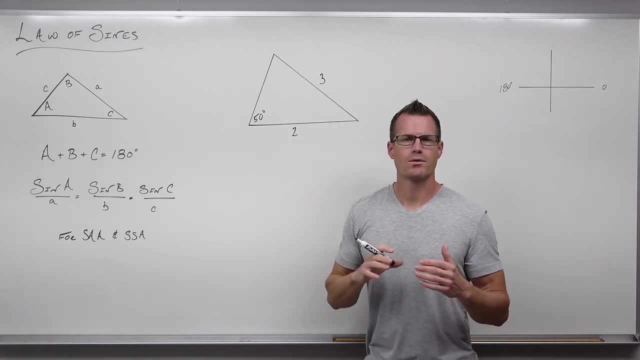 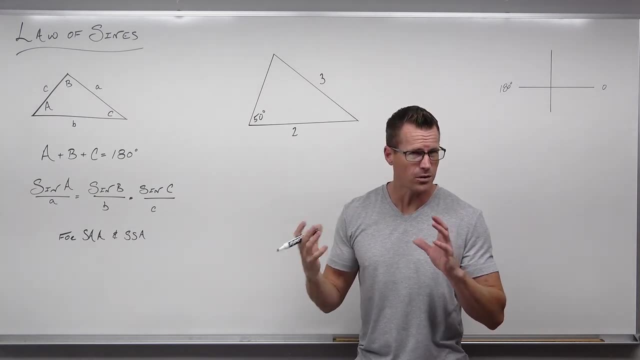 If that angle is between those two sides, it would be here. So we're going to categorize this. Can you see that a lot of students would use either law of cosines or law of Sines on the wrong thing. So we're going to look at this and say, hey, I really know a side, and then 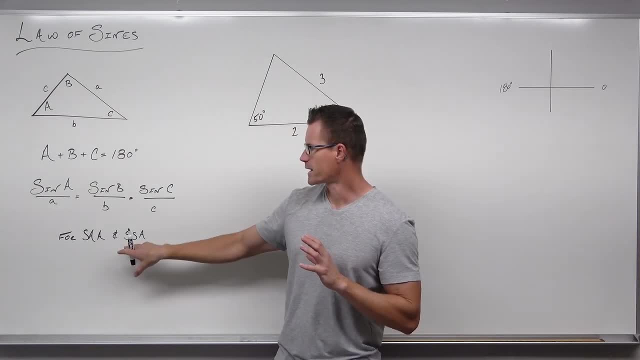 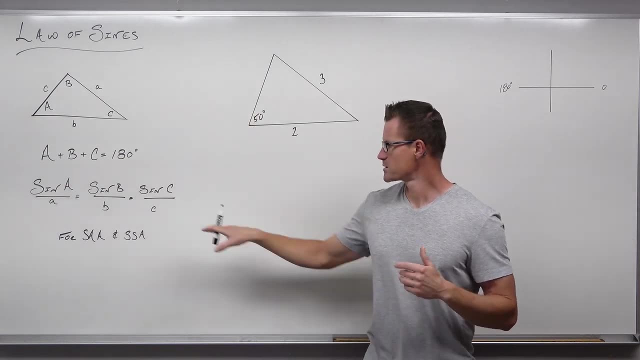 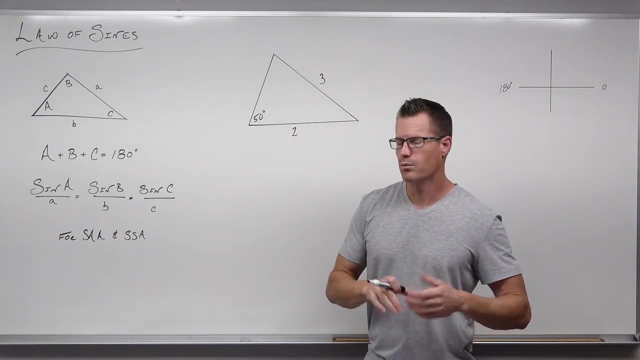 an angle that's not between them. That is exactly what this is talking about- Or an angle and two sides. in that order That's fine. It's just we don't say that because, Anyway, so we know two sides and we know one angle. 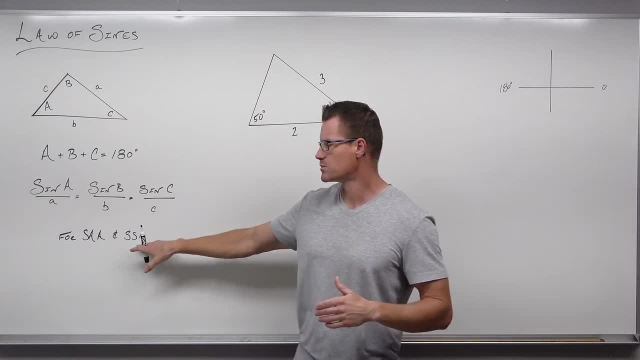 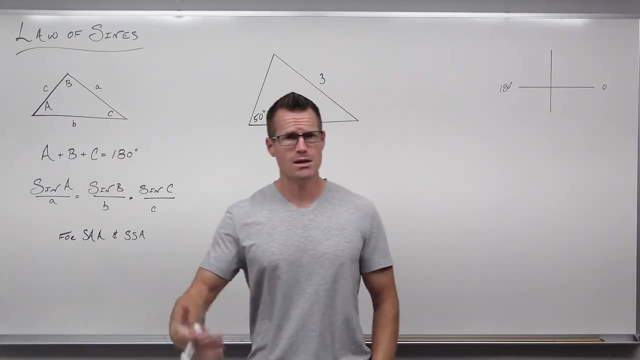 This is a case for law of Sines, but I need you to know that with this, more than one thing can happen, and we're going to see that as we go through it. So first things first. after identify, it's not a right triangle, or maybe not. 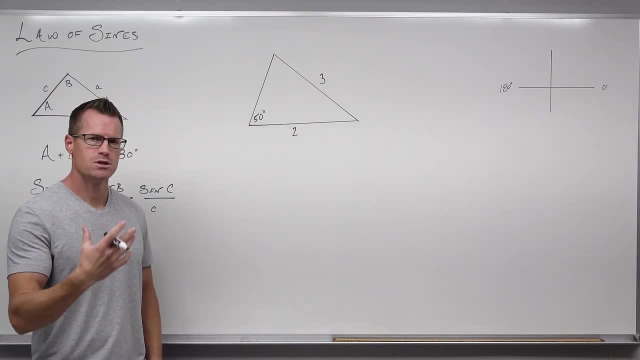 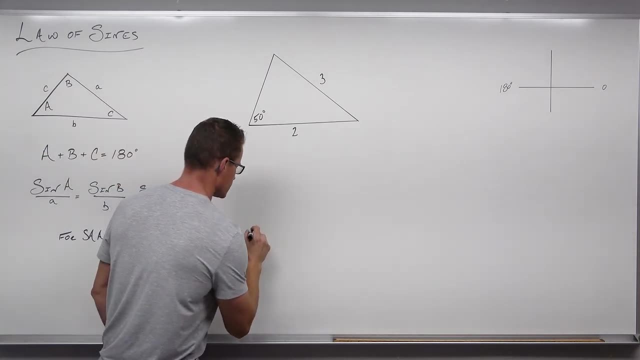 a right triangle. We're not sure about what it is. We just have two sides and angle, not between it. I want to think in my head: This is law of Sines. I might even write down the proportion. I might think in my head: what do I need in order for this to work? 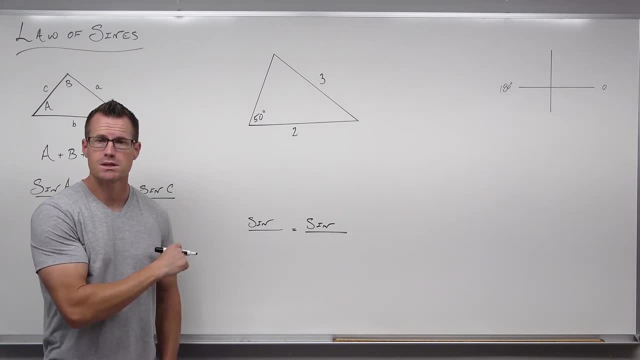 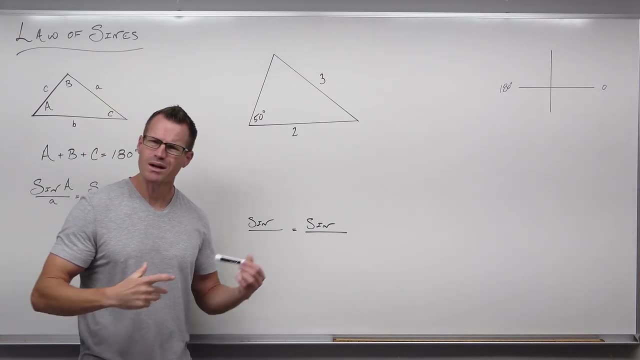 I need two angles and one side, or I need two sides and one angle. Hey, that's exactly what I'm given from there. I'm going to be labeling What else is going on in my triangle, So I want to give names to these things I'm about to find. 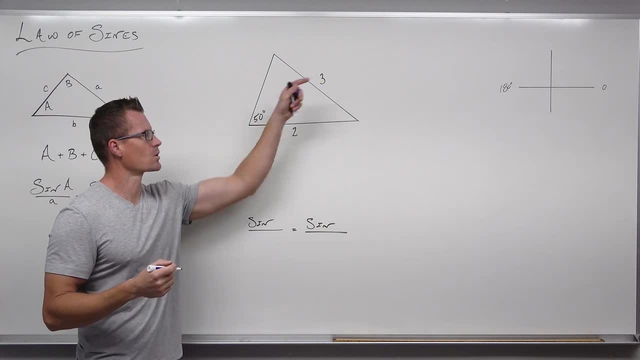 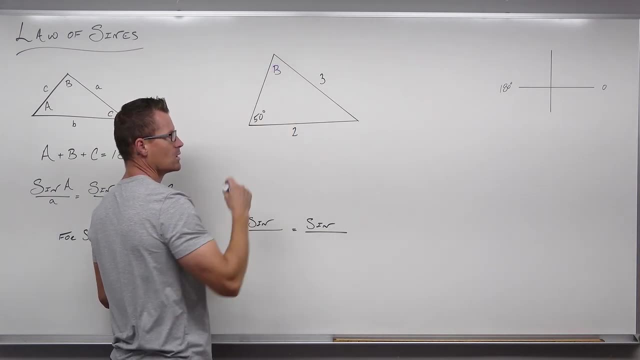 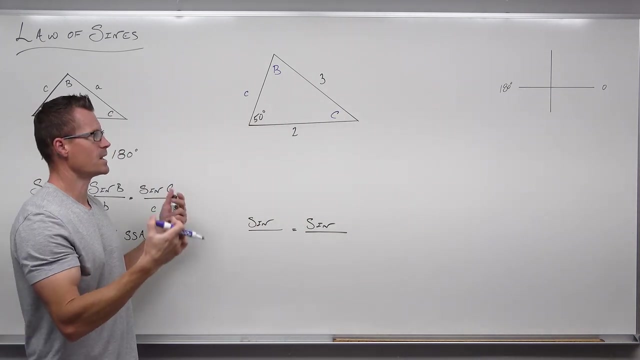 So I might call this angle A, and this would be lowercase letter A. I might call this angle B, Then this would be lowercase letter B. I might call this angle C, and this would be lowercase angle C. I might do that just to give it some names. 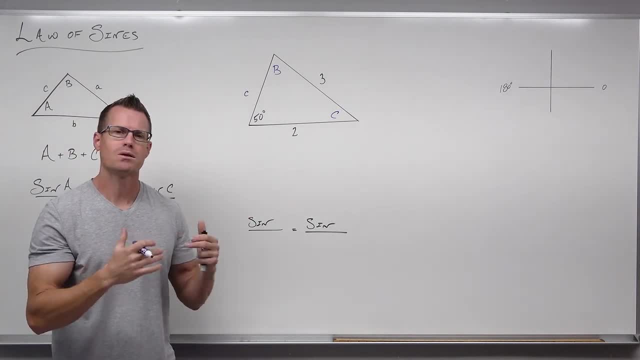 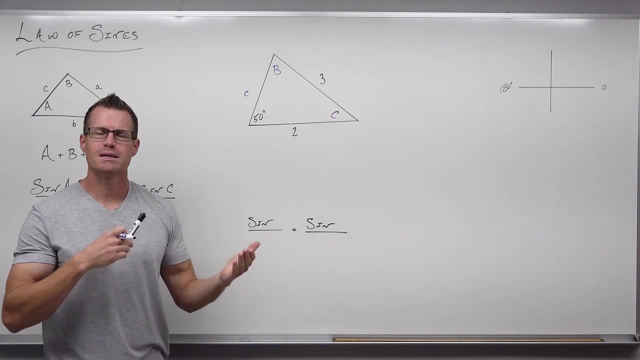 It does not matter what sides or angles you call them, As long as your letters you're using match up. So C with C, B with B, A with A. That way it's a little bit easier to see what's going on. 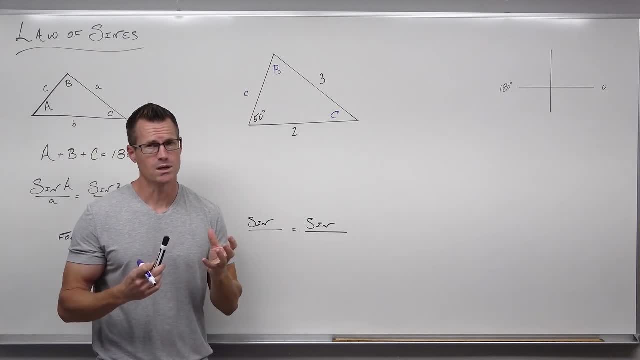 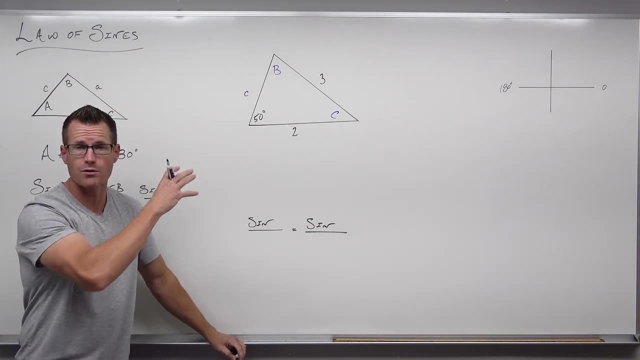 You don't want to confuse those letters, because a lot of signs really would get confusing them. So that's what I'm doing. The next thing I'm doing is I've seen if anything besides my law of signs will solve for any of this. 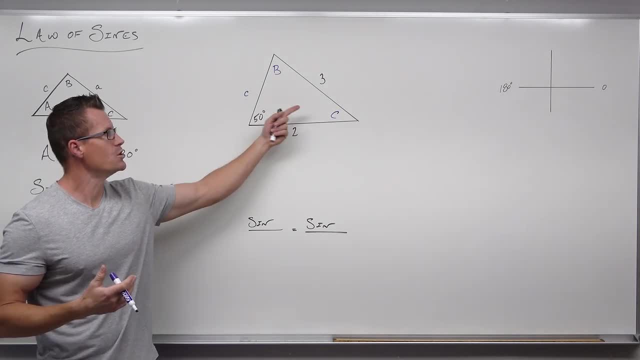 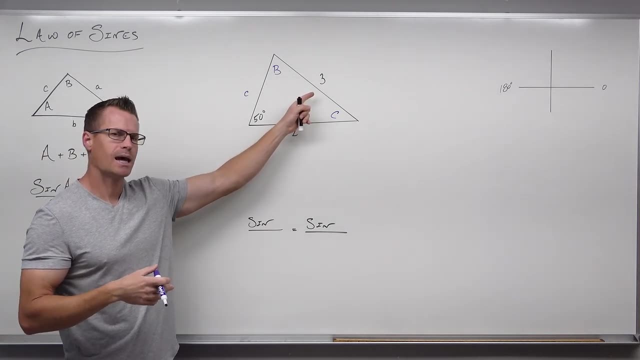 Man, I only know one angle, And so there's no way for me to find those other two angles without something besides interior angle sum. I know two sides, but can I use Pythagorean theorem To find the third? No, because I do not know if it's the right triangle. 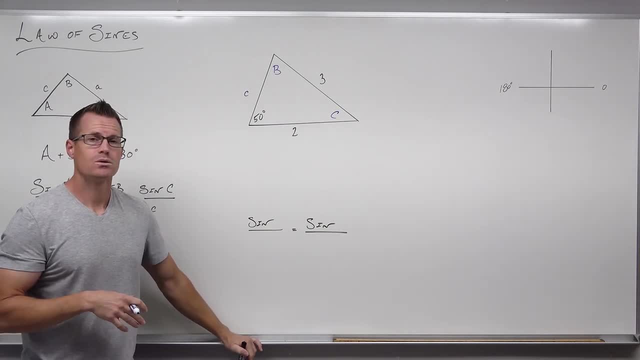 So I can't use that. We're stuck with law of signs, So let's go ahead, Let's figure it out. Well, let's see If I go ahead and I try to use law of signs, I know two sides and I know one angle. 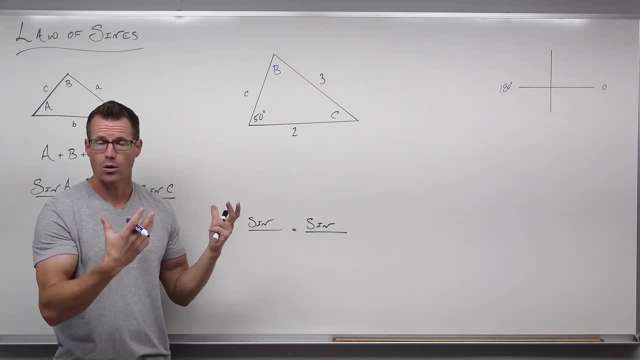 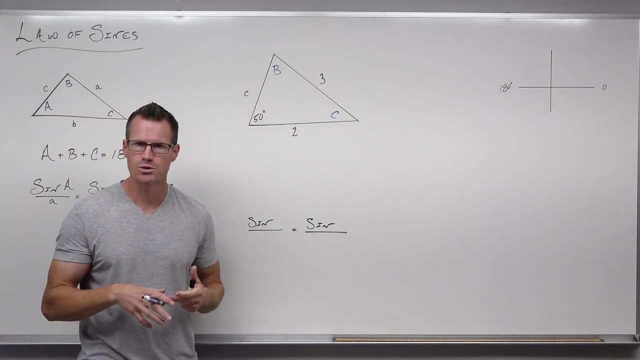 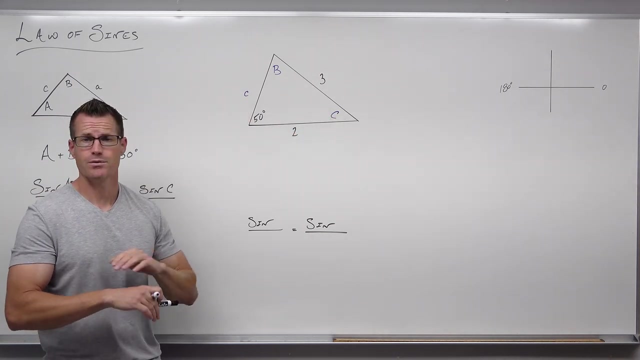 So I'm going to create a proportion out of one of the things that I already know. I know one angle and I know one side opposite to it. Do you see that that has to be one proportion you use? If not, you'd say, well, an angle, I don't know, over two equals an angle, I don't know, over a side, I don't know. 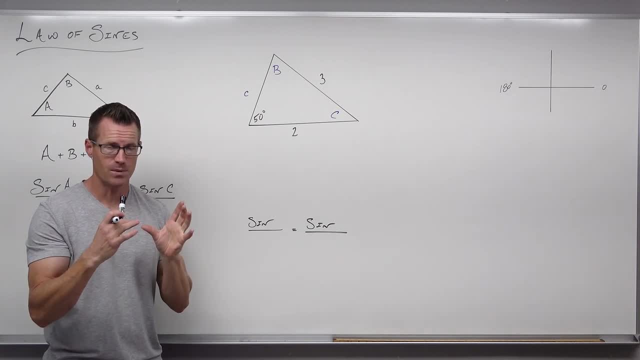 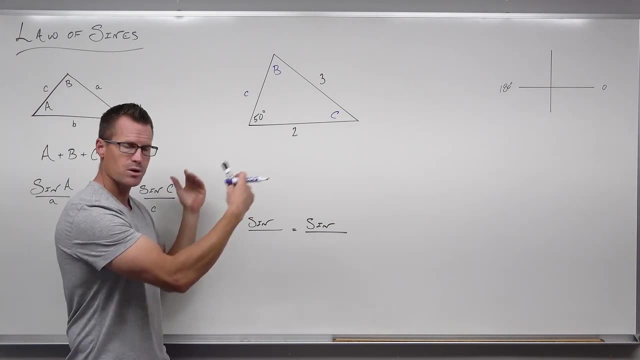 That's not helpful. So you need to know one complete piece of information. That's why, in both these cases, you need to know an angle and one side that's opposite to it. We saw in the previous two cases you had to know at least one angle and one side opposite to it. 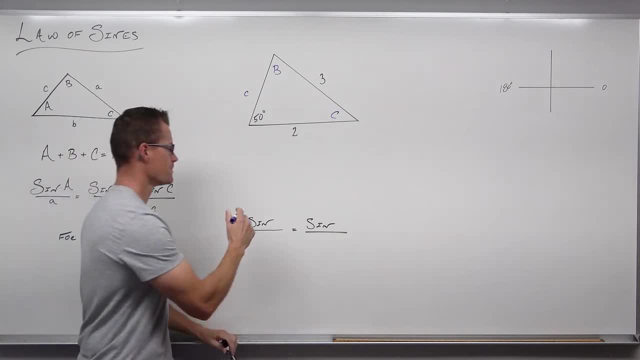 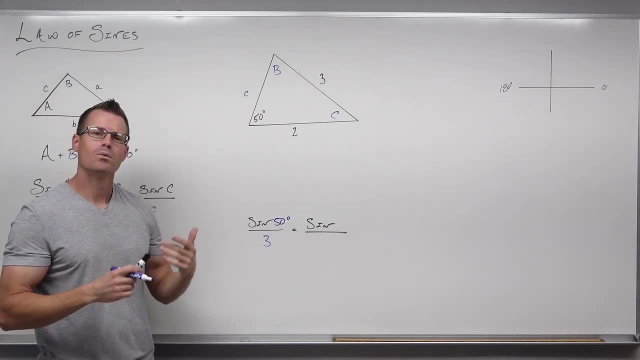 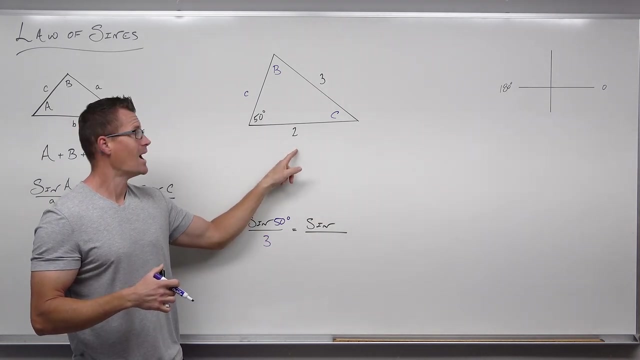 Now we know one angle, one side opposite to it. Let's create that proportion. So angle with opposite side Equals. Well, what do I do? now? I need to have another proportion with only one unknown. That means that I'm going to have to use that too, somehow. 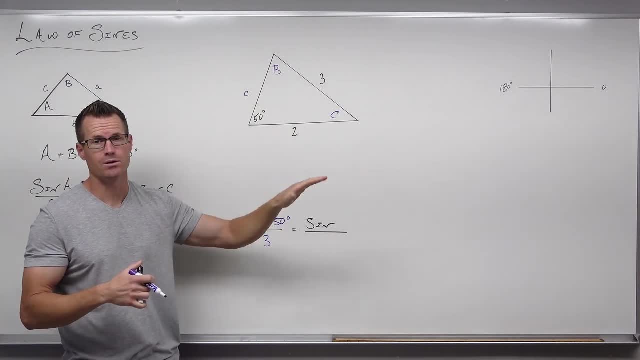 I can't use that letter C and that letter C because I know neither of those. We wouldn't want to do that. We want to say: sine of 50 degrees over 3 equals sine of angle. I don't know. over side, I don't know. 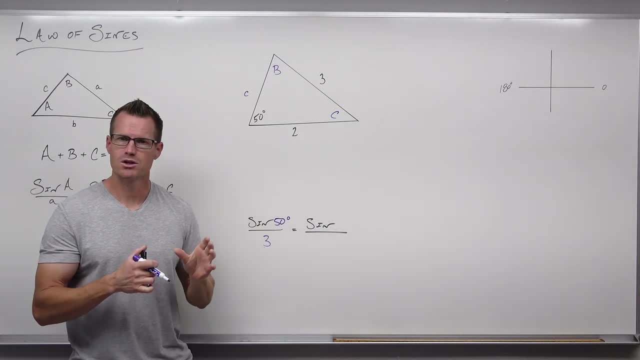 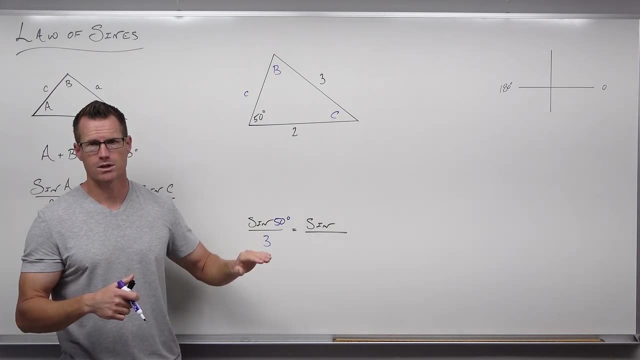 That's also not useful. It's too many variables. So pick out this relationship that you know one complete proportion and you know half of the other one. It's half the other one. You either know an angle or a side. We dealt with knowing the angle in the last two examples. 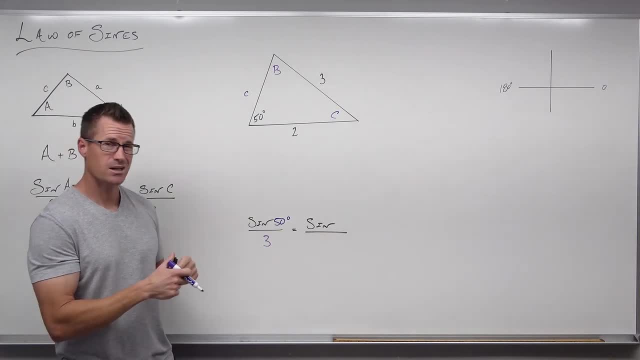 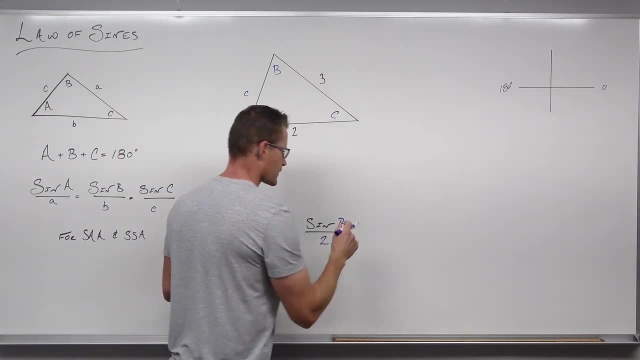 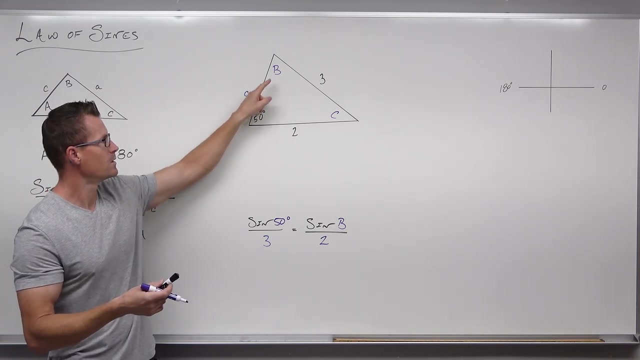 Now we're dealing with. you know a side, So what side do I know? I know side 2.. What angle is opposite that side? Angle B? I'm going to double check. Let's see 50 over 3.. So that's one proportion equals. I can do sine of B over a known side. 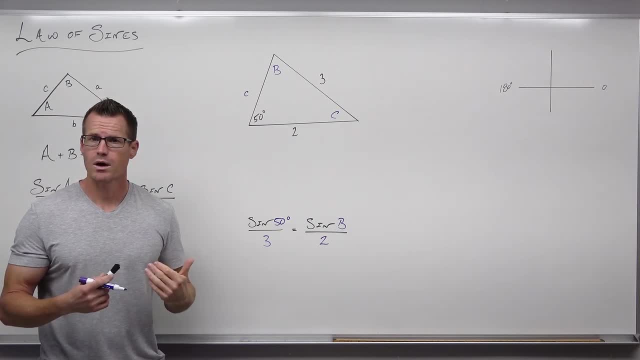 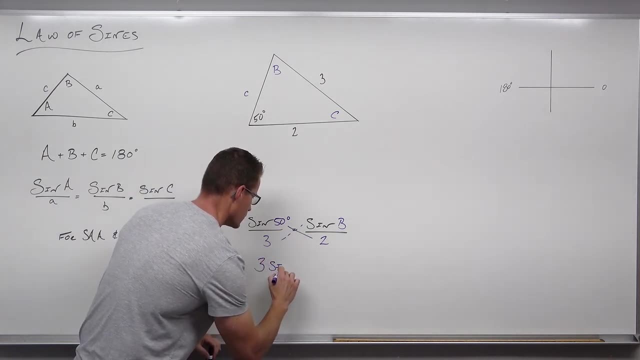 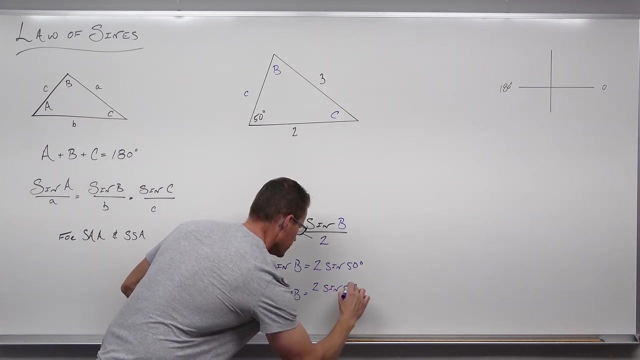 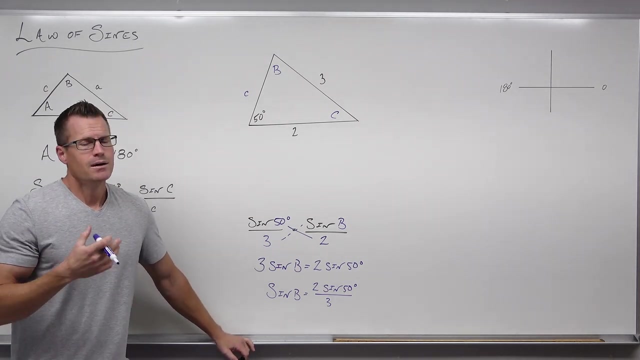 That's great. This leaves me with just one unknown. Now we're going to cross, multiply and we're going to divide, So sine of angle B equals 2 sine 50 degrees over 3.. This is where some other information has to come about. 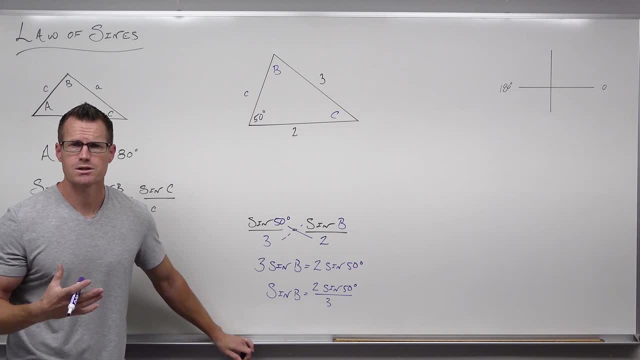 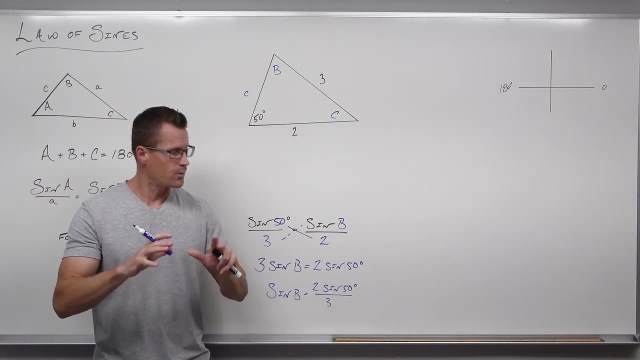 I'm going to tell you exactly what we're going to do before we get there. That way, it's not a surprise. So here's what's going to happen: in order to solve for angles and you need inverses. Do you remember that? 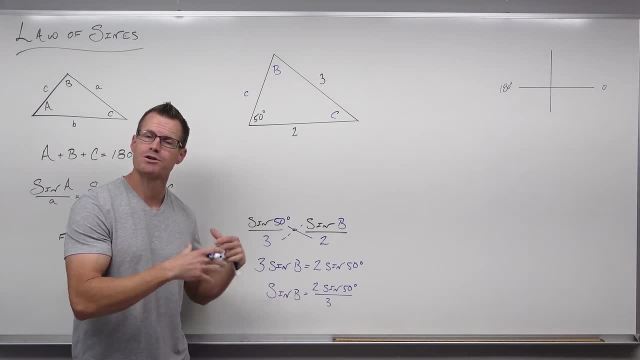 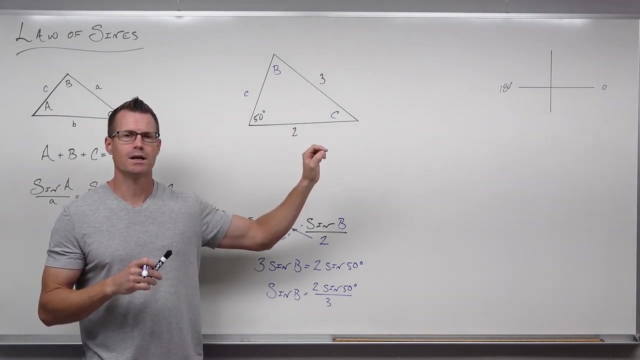 I hope you remember that in order to solve for B, you need to take sine inverse of both sides. Now I also need you to remember that on a unit circle, from 0 to 180 degrees, on a unit circle, you can get two angles that give you the same Y coordinate. 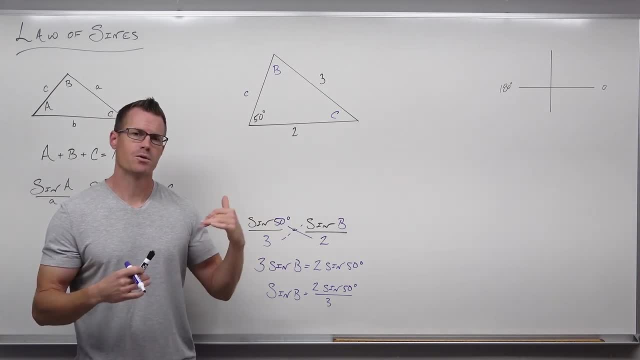 This is why we get more than one option for sides. Side angle is because sine of an angle or an angle can have two equal Y outputs, One on one side, one on the other. They're both positive that we can use, And I'm going to show you that in just a minute. 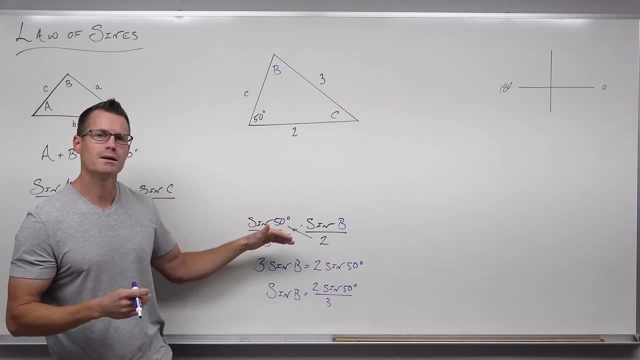 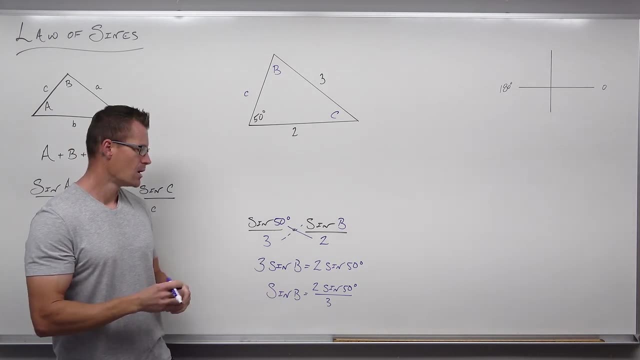 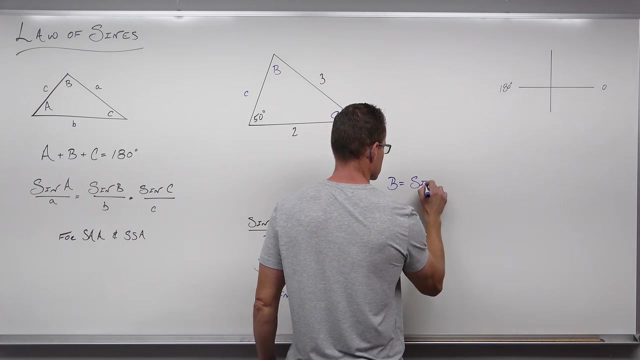 So step number one is creating the proportion correctly. We're cross multiplying. Step number two is: after you get there, you need sine inverse. That's an old piece of information to bring up. We're going to solve for B. Step number three is we need to find Y. 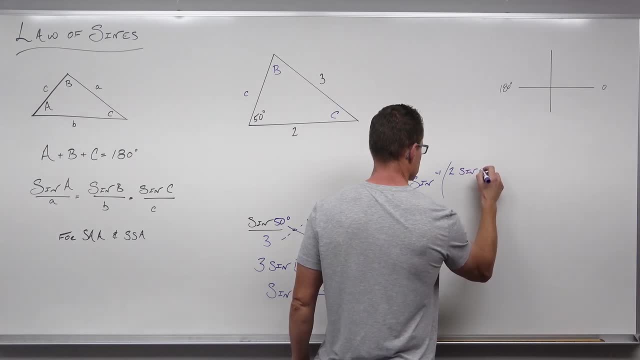 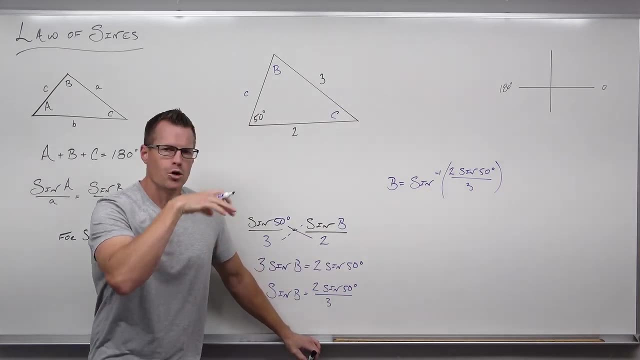 So through the Yang function we actually will get Y, or we can call it the Yang function. But to do that we're going to use the Y function that we need On your calculator. you press sine inverse, It'll open up parentheses for you. two sine 50 degrees. 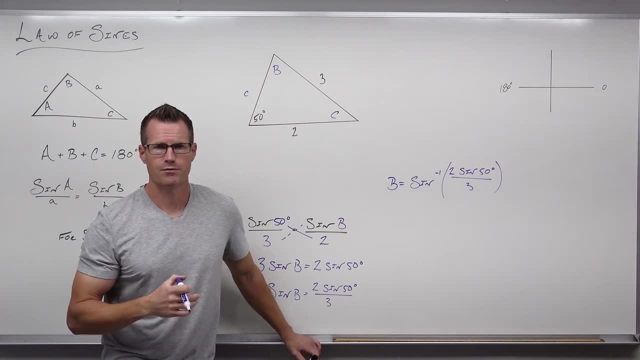 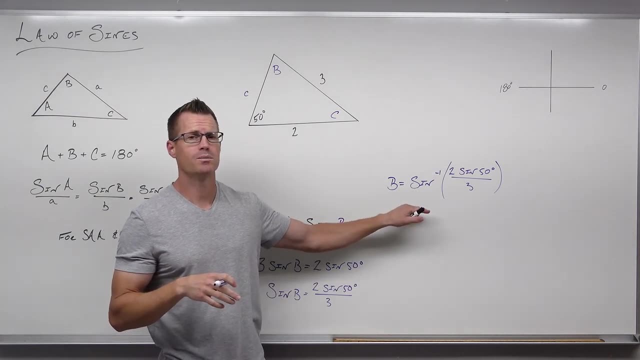 Close your parentheses, divide by three, and that will all be inside your sine inverse. We're going to get about some sort of an angle here. Notice it. This is the exact angle. This is what angle B is for short Contains. 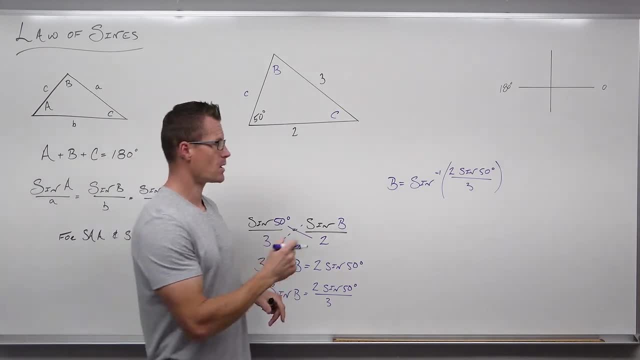 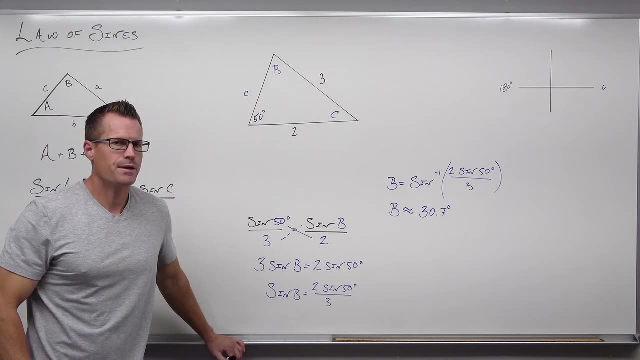 about angle B. it's just not super useful. so I'm gonna approximate and we're gonna get about thirty point seven degrees. I'm not gonna write that up there because it might be two different triangles that could give us this, and here's how to discover what that is. so this is the second piece of formation I told you. 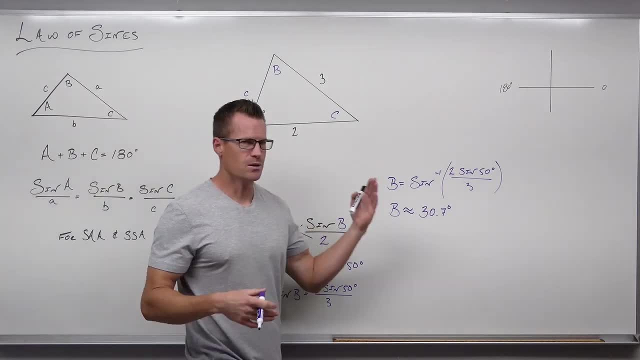 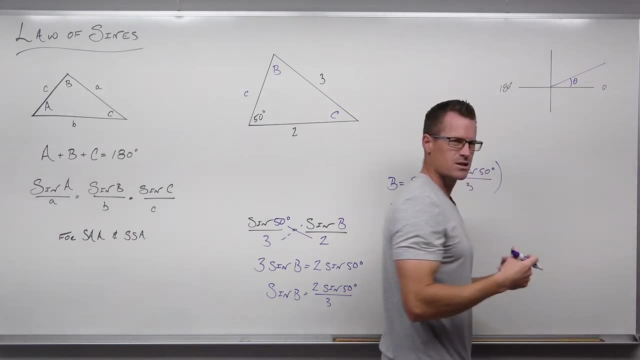 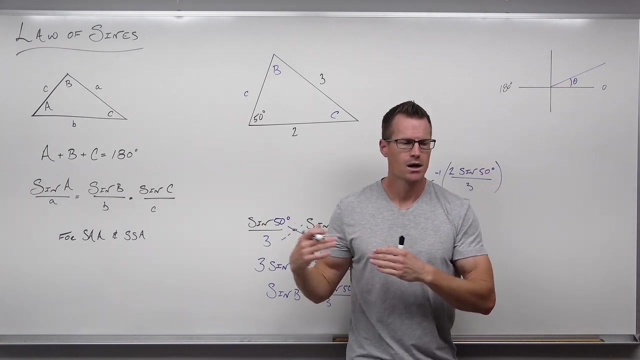 we're gonna get to. we need to understand that if we have some sort of an angle- let's call it a theta- on a unit, is circle that angle? if it's a positive angle, all of our angles are positive. on triangles, everything's between 0 and 180. 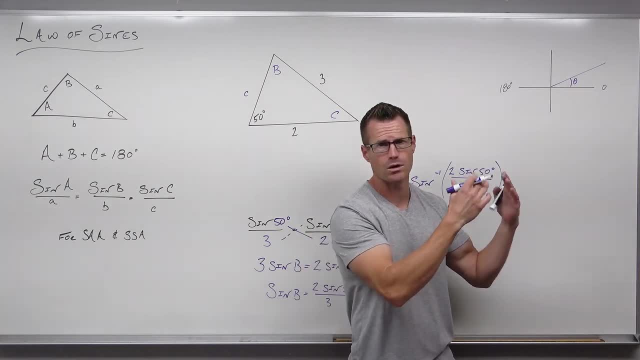 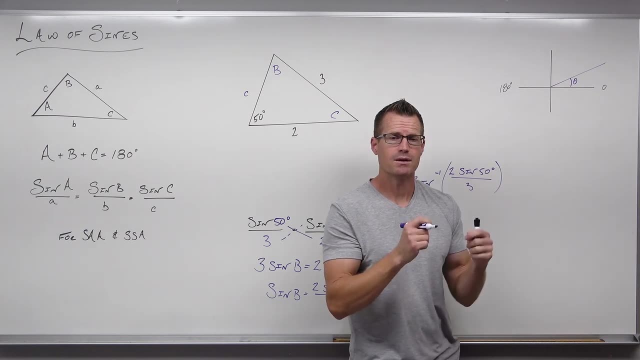 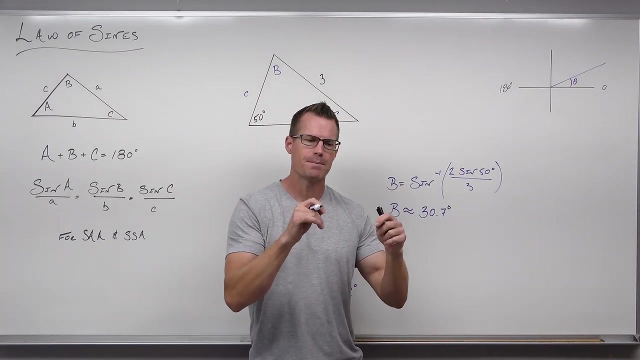 degrees on our, on our triangles, to create this, either acute or in Deus angle. it's passed 90 degrees. so every single angle, honor, unit, circle, positive angle is going to give you this Y coordinate now with sign. remember what sign does. this is where the old stuff comes back at you. is that the sign function on a? 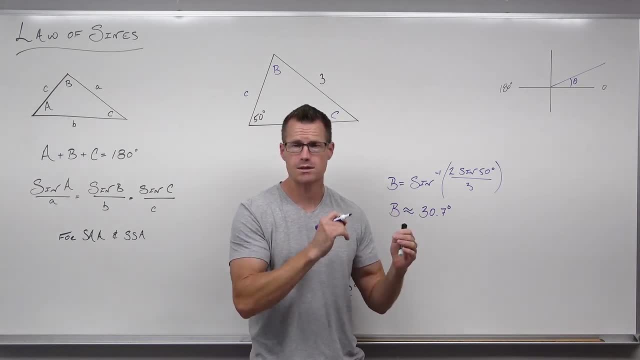 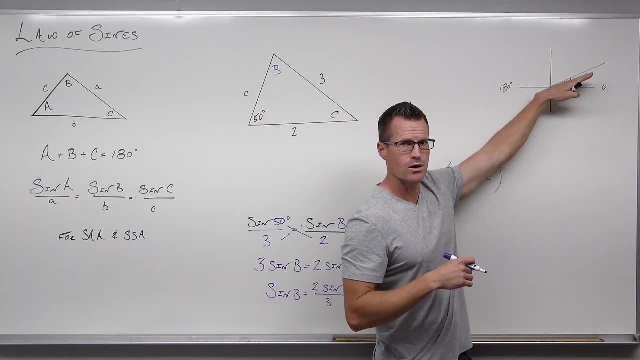 unit gives you out the y-coordinate. That's what it does on a unit circle. This angle would have a positive y-coordinate. Do you see why You see this positive y-axis? You're gonna have a positive y-coordinate, But you also hopefully remember that. 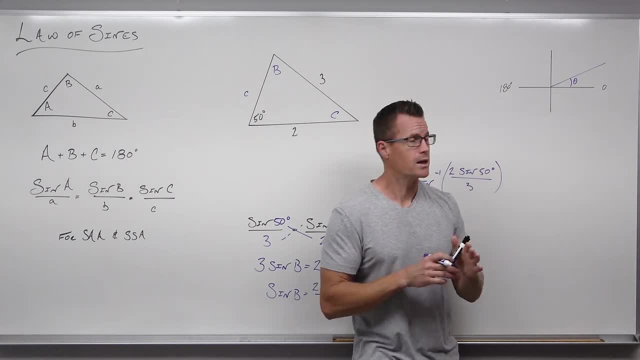 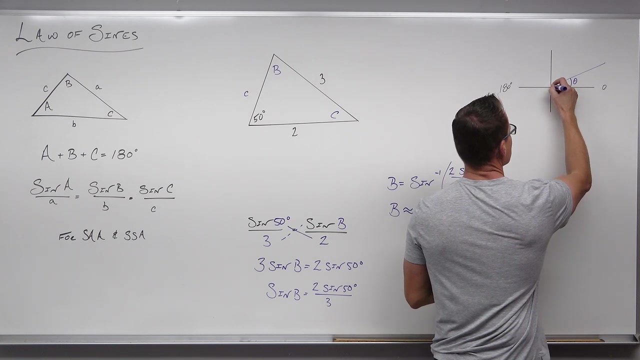 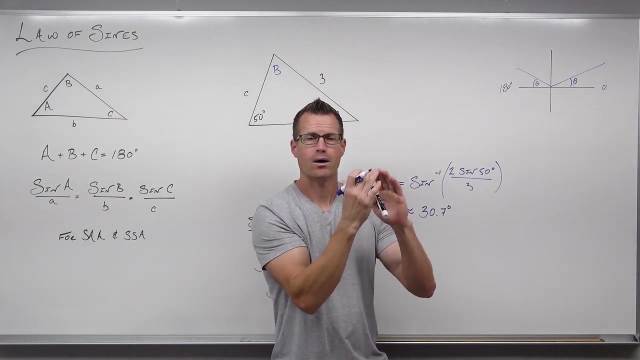 there was another case where you could get a positive y-coordinate. Anything in quadrants one and two sine is positive. Why? Because the y-coordinate is positive in quadrants one and two, So there's another angle that would give you out the exact same value. It's the angle that you would reflect. Now, this is great. this. 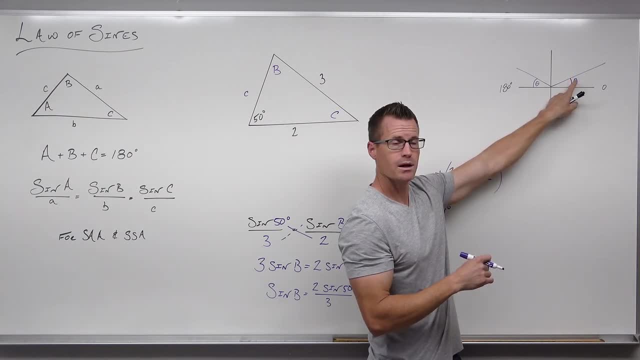 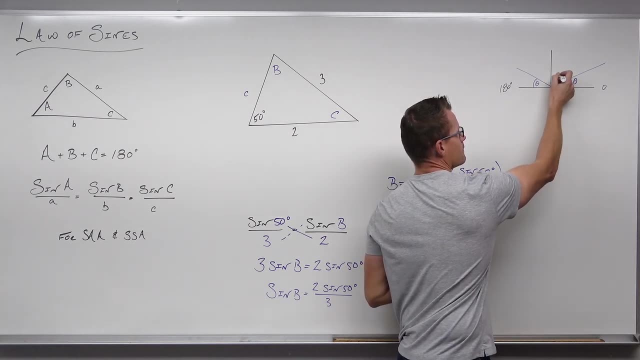 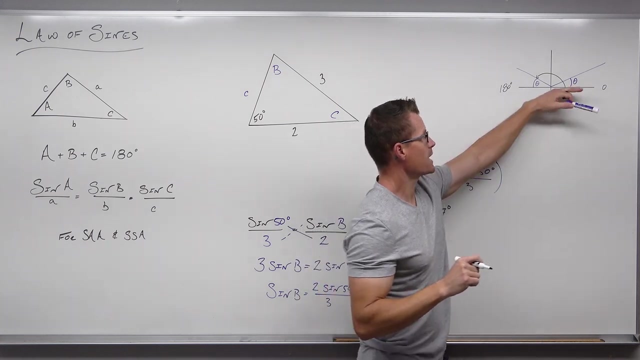 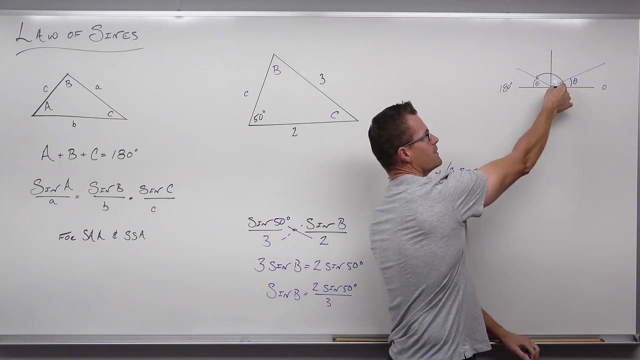 is okay, but I'm talking about this is option one, but this one right here is option two. I need you to think about what that angle is. So this angle is theta, theta, theta, theta, And the reflected angle gives you the same exact y-output, which it does Then. 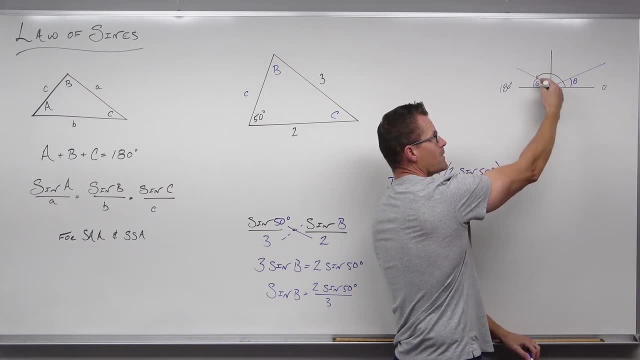 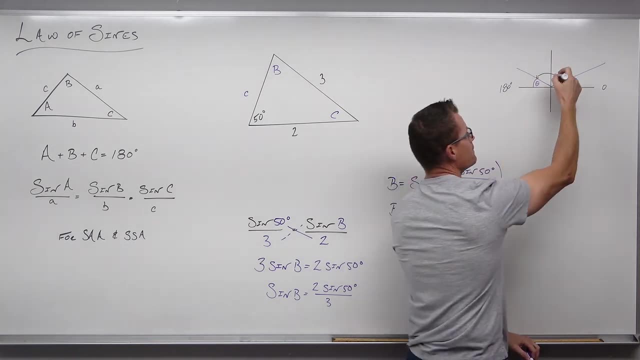 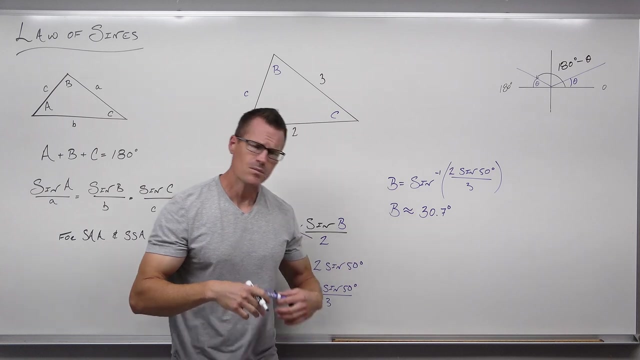 this angle would be 180 degrees minus that theta. It's like, oh, you went too far. How much did you go too far? I went too far, theta. So going to 180 degrees minus theta, That will give you the other option for a side-side angle. law of sines proportion. 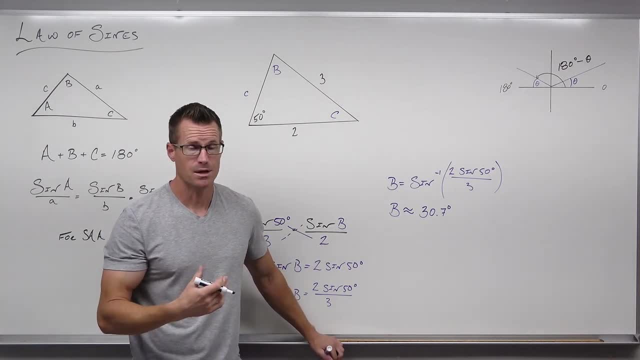 So I'm going to take this angle, and I'm going to take this angle, and I'm going to take this 30.7 degrees, And what I'm going to do is I'm going to subtract 180 minus 30.7.. 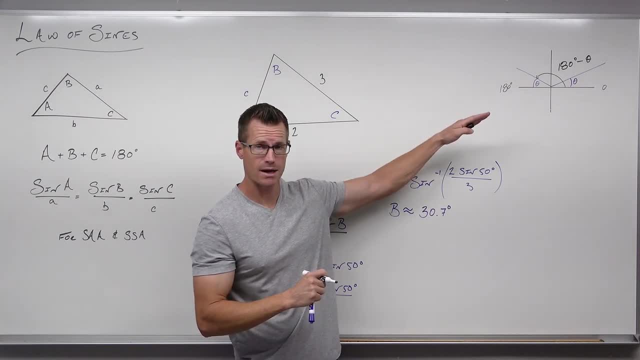 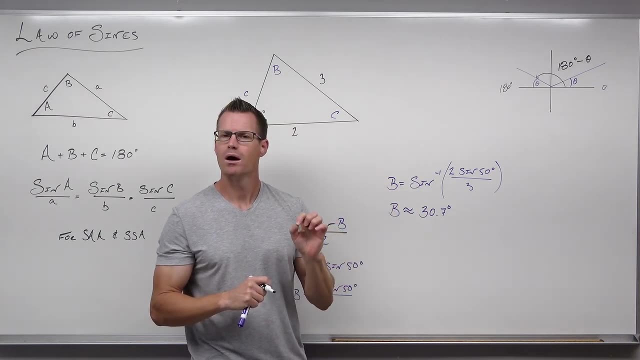 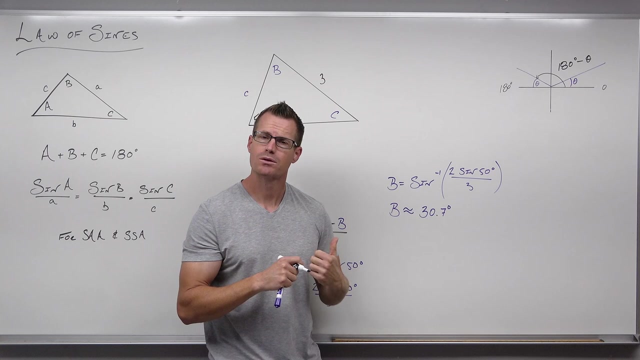 I'm going to go through it one more time with you. This angle, 30.7 degrees, will have a y-coordinate. 180 degrees minus 30.7 will have exactly the same y-coordinate on a unit circle. So therefore, sine of 30.7 and sine of 180 minus 30.7 will be identical. What 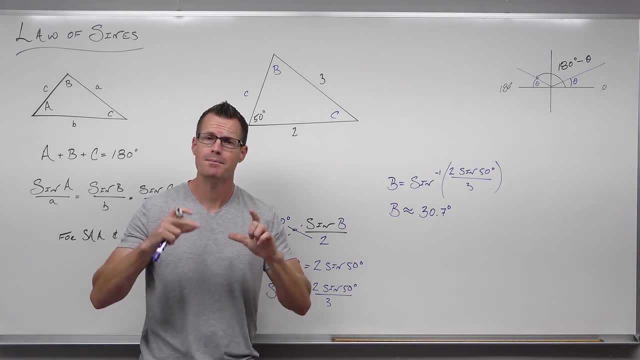 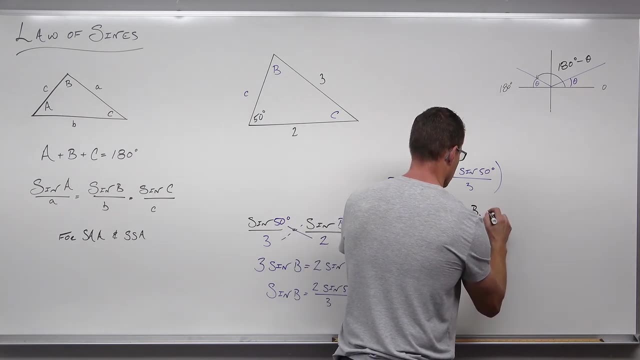 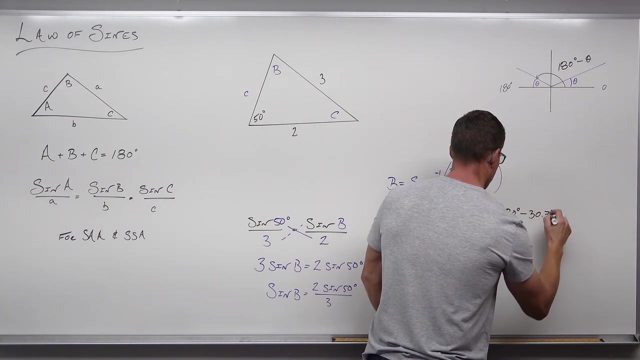 that means is that this angle could be one of two things, provided it makes a triangle for us. We're about to find that out. I'm going to call this option one for b. I'm going to call this option two for b Option. 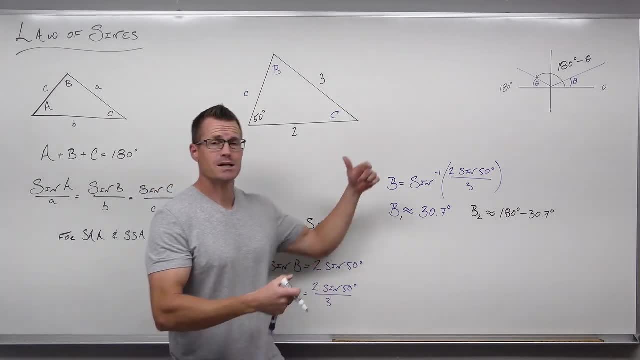 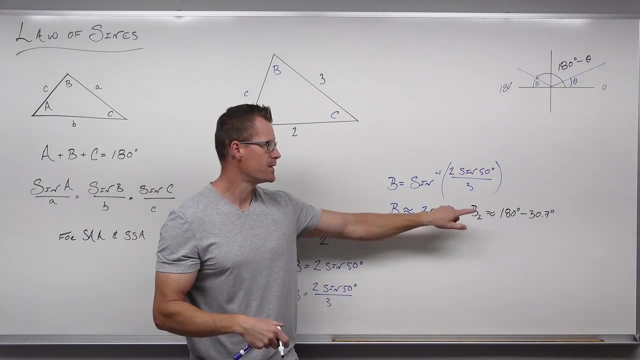 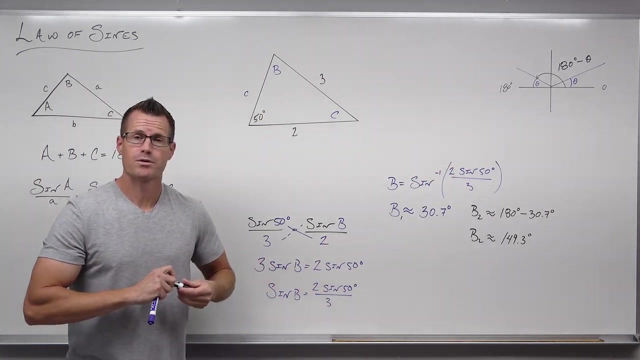 one is that we have 30.7 degrees. Option two: because of what I've just explained to you, because angles positive or 180 minus that angle will give you the same y-coordinate. then this can be 180.7.. Well, that's 149.3 degrees. Now how in the world do we know if those are both options? 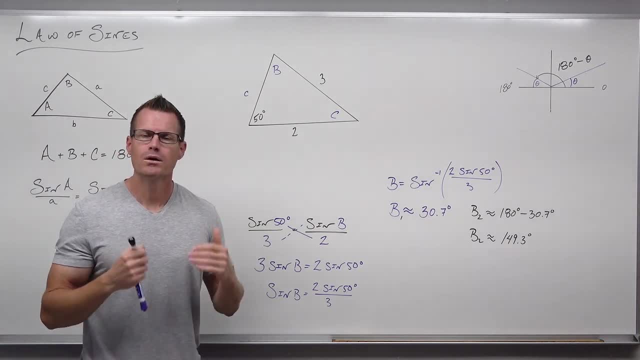 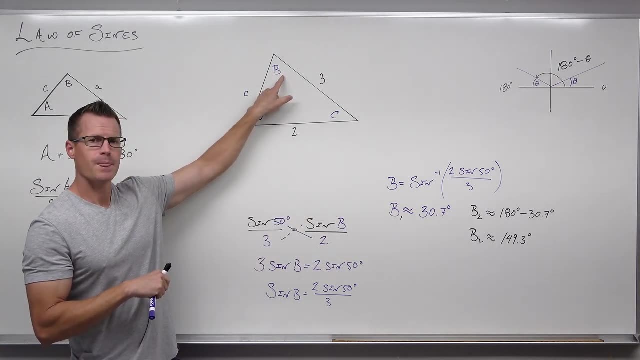 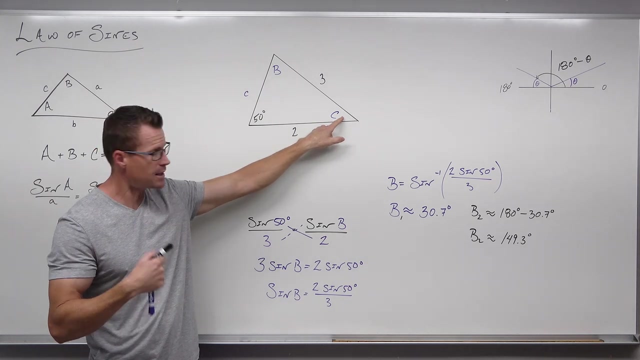 or only one of them works or none of them works. Look at your triangle. Look at your triangle and plug it in. If this option one gives you 30.7,, is there enough left over in your triangle to create an angle that adds up to 180?? Yes, Yes, there is. And if you 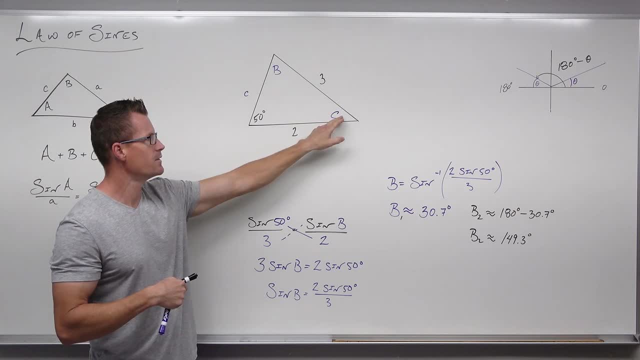 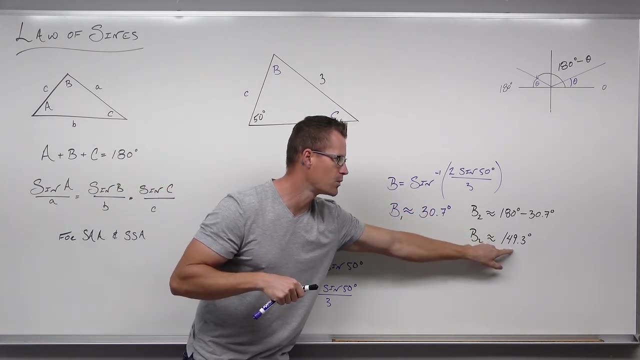 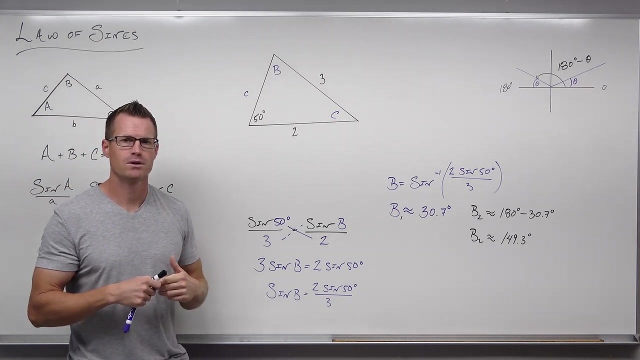 go. yeah, if this is 50 and this is 30.7, there's enough in 180 degrees to subtract both of those and still be left with an angle. Think about 149.3 degrees, Option two. try that here. Try option two in b: 50 plus 149.3 degrees, that's like 199.3.. Wait a minute. 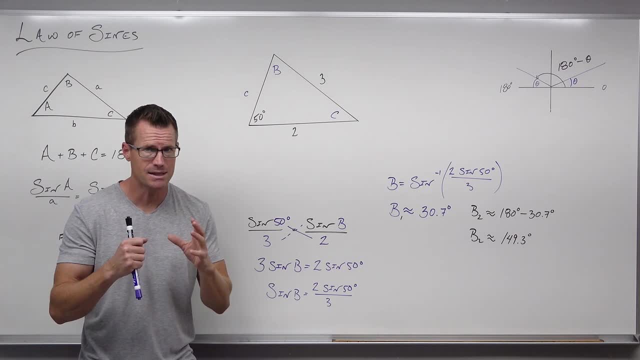 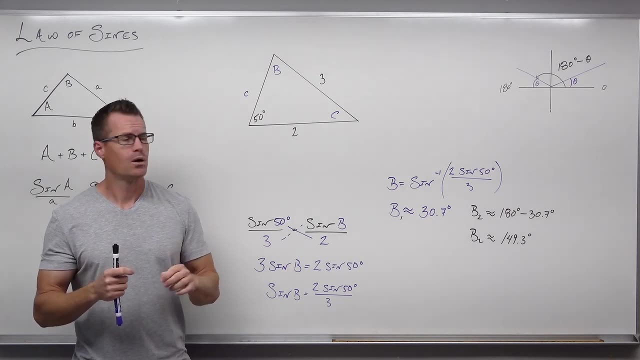 All of our triangles can have at most an exactly 100.3.. 180 degrees. So if you go over that you have a problem. That is how you determine whether or not there's two triangles or only one. I'm going to go through that again because 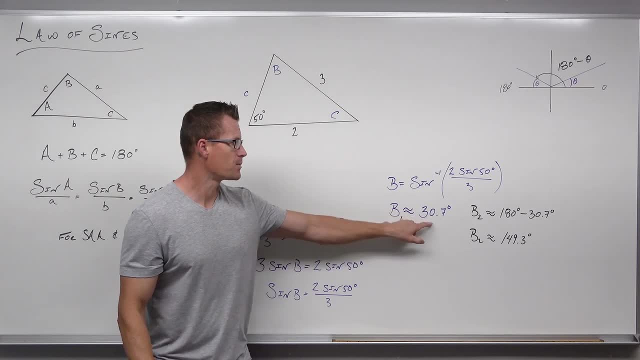 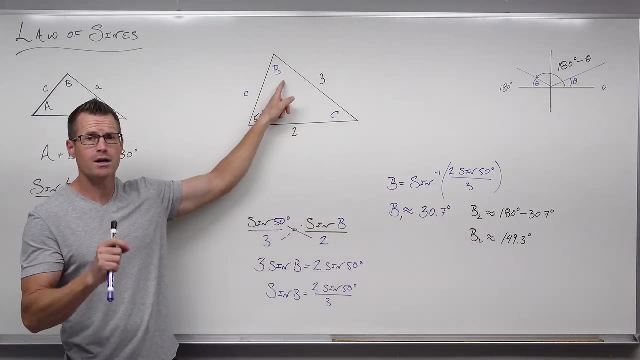 it can be confusing. the first time you hear it. We take a look at this and go: hey, if I plug that angle in here, there's enough left over for me to still have an angle. If I plug this angle here, there's not enough in the interior angle sum for me to still. 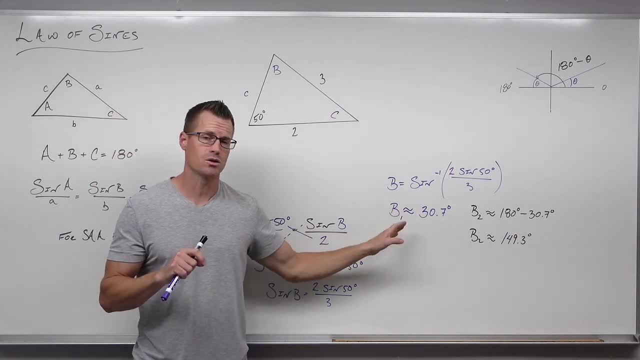 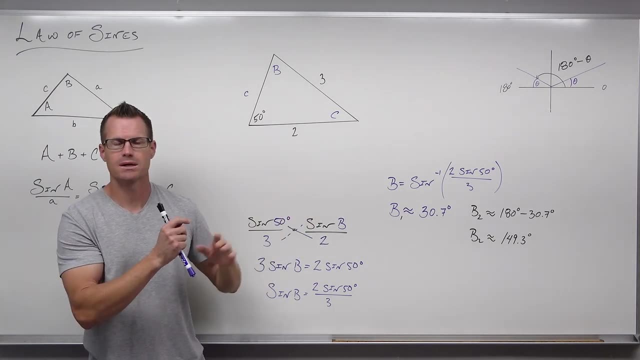 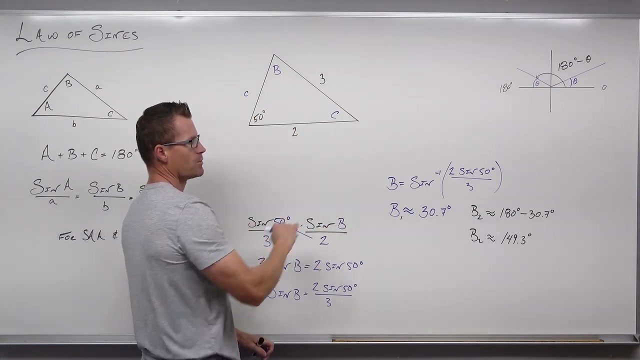 have that angle. Therefore, there's only one option that actually works. If that doesn't work, Then watch what will happen. Even if this doesn't make sense, watch what would happen if you keep on going. Let's try to find an angle c. If this is 30.7 degrees, then I would 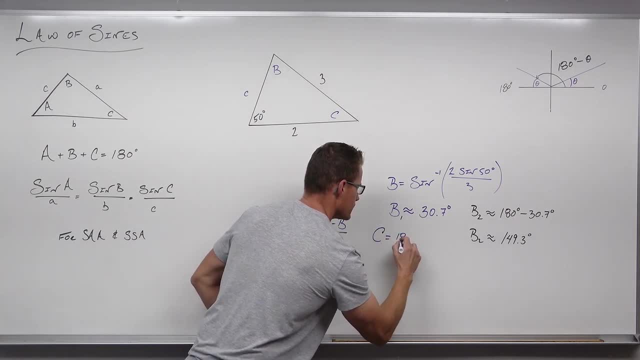 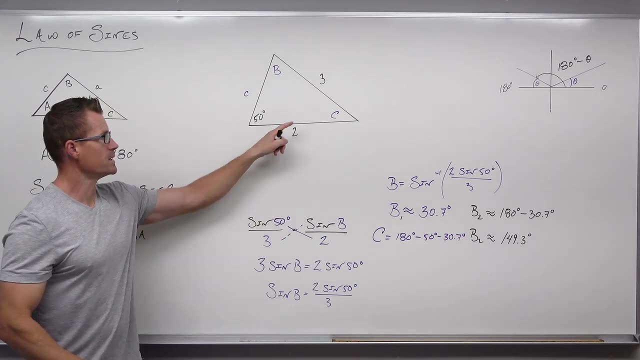 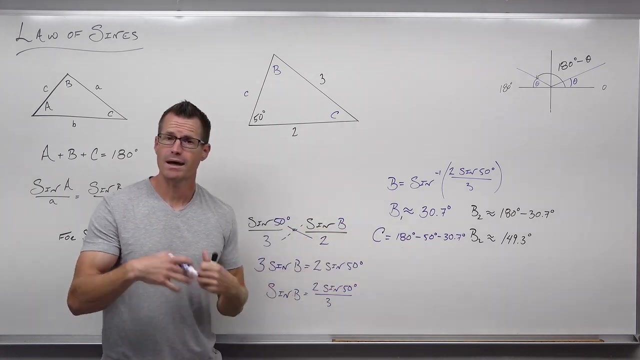 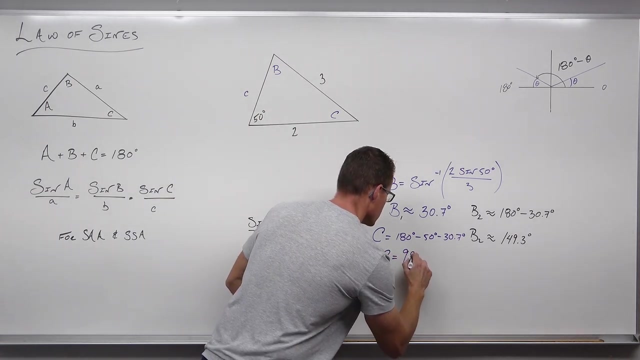 take angle c, Angle c would be 180.. Sure interior angle sum is 180.. Minus 50, minus 30.7.. Leave me with anything. Well, let's see. Angle c would be 99.3 degrees. Okay, that seems. 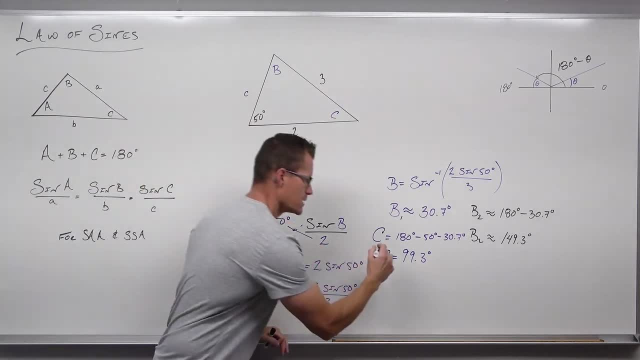 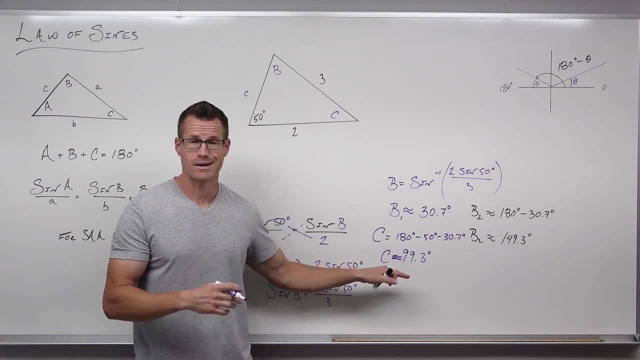 pretty reasonable, because 99.3 or about there. I should use equal signs that are approximated. Why? Well, because this is approximated. You can't use an approximated angle and somehow get an exact angle. So let's see if this works. If this is about 30.7 degrees rounded and 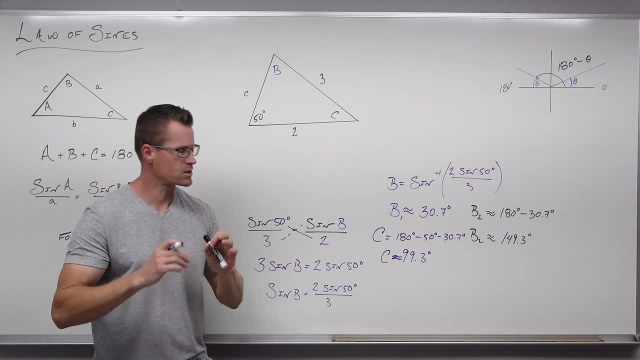 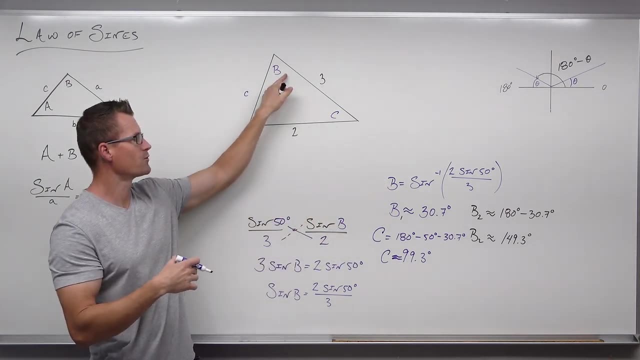 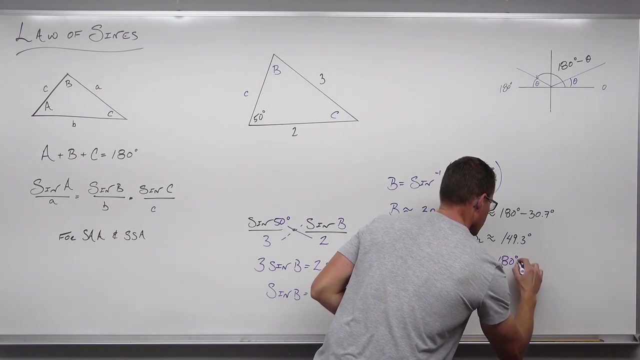 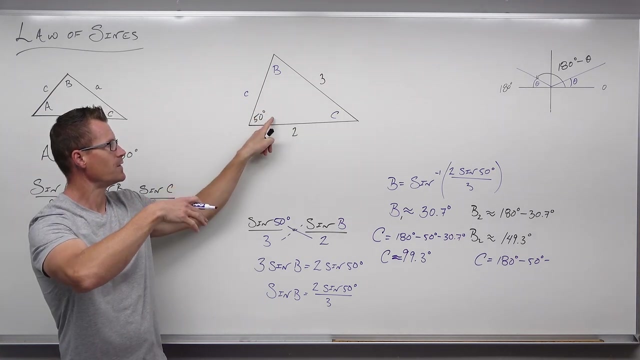 this is 99.3 degrees and this is 50, that still adds to 180.. That's great. That's exactly what I want. Check out: if option two were put in there, If option two were put in there at 149.3 and you tried to find angle c, we'd have. angle c would be 180 degrees minus 50. 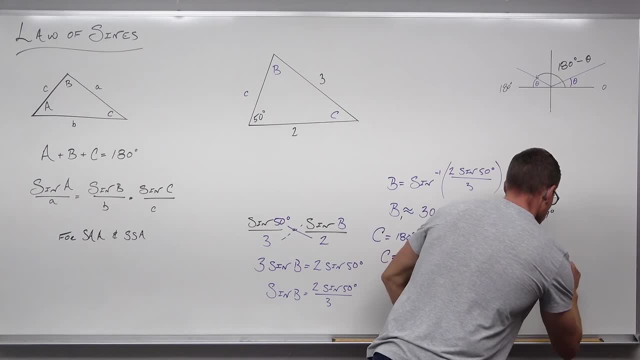 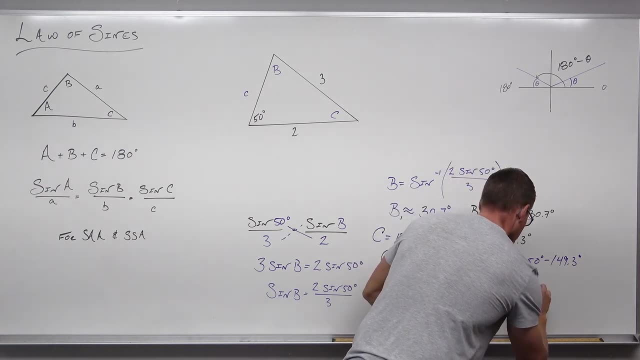 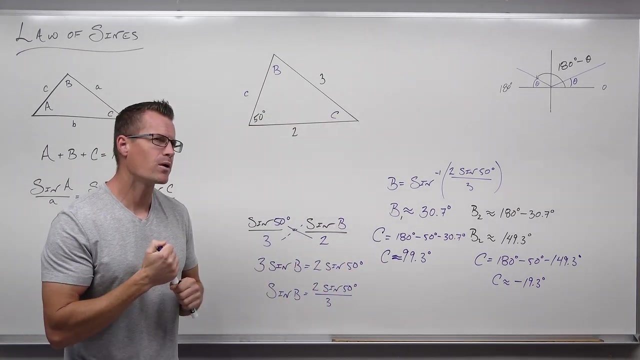 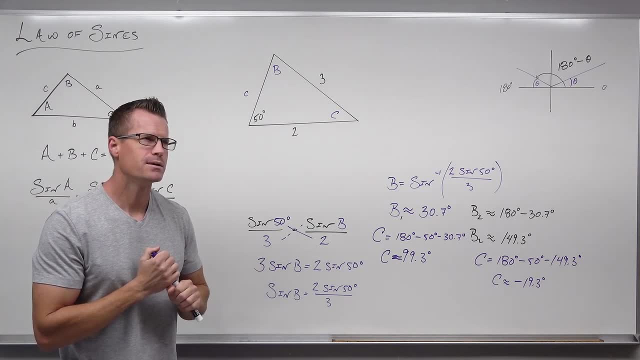 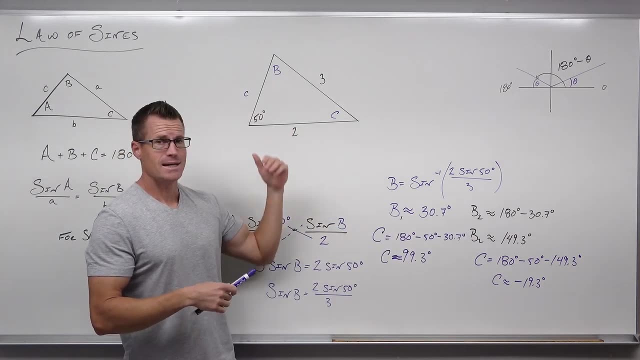 negative 19.3 degrees And you go wait a minute, does that? Hey, that's exactly what we talked about when I said: does that work? And we plugged it in, We got a 199.3.. That's 19.3. 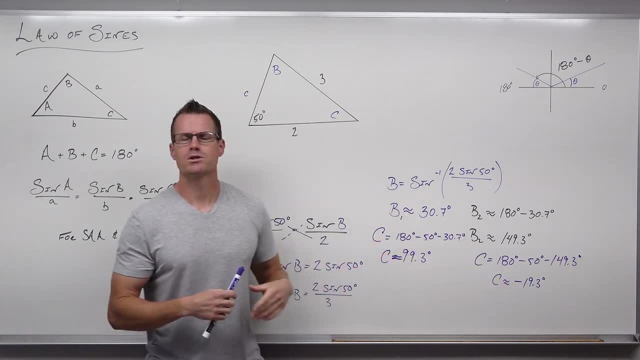 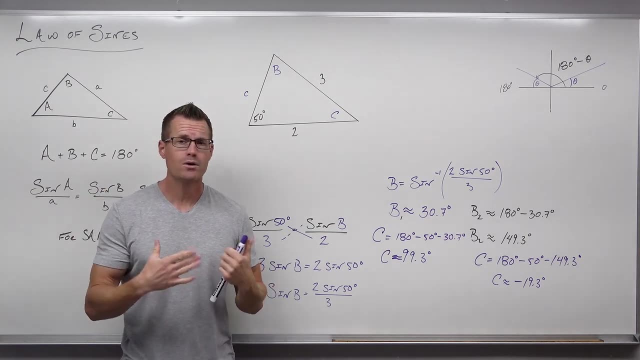 degrees over 180. That's going to show up here. So if you ever get a negative angle, your triangles can't have negative angles, not a real triangle that we're looking at, we're talking about right now. All of your angles are between 0 and 180 degrees. All of your angles. 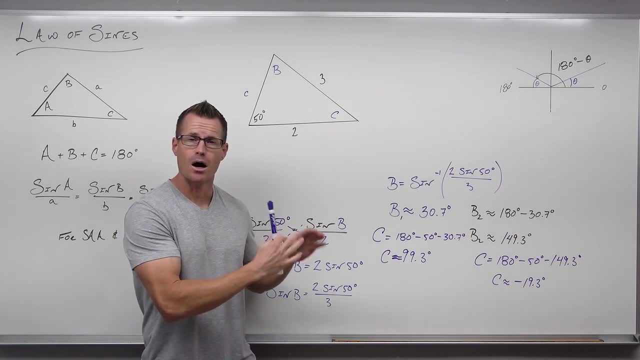 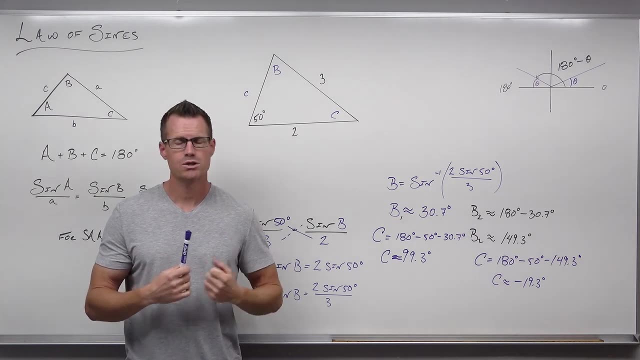 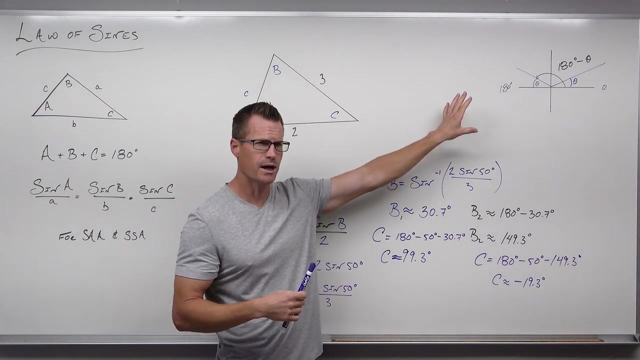 have to be positive. So if we break any of those things, then this option is not possible. This is how we determine whether we have one solution, two solutions or no solution. So when we're going through this, you do have to think about your options here with the angles that you're finding. 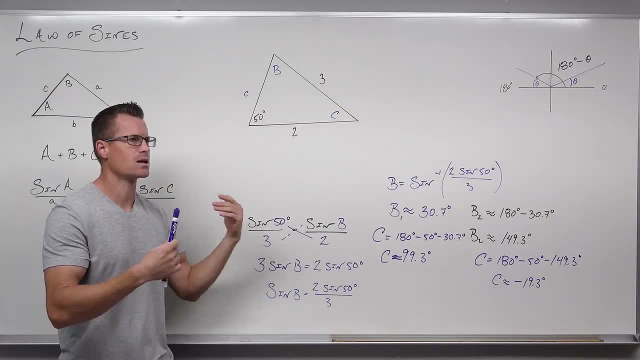 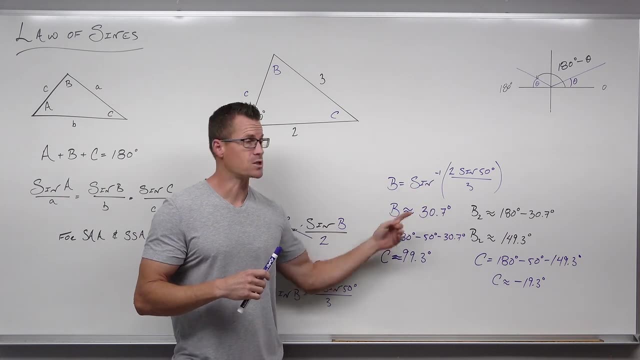 So find your first angle. Let me start. Let me kind of go back a little bit. If you are talking about side-side angle, find your first angle. Give it both options, using what you know about the sine function, that sine of an angle and sine of 180 degrees minus that angle. That's all you. 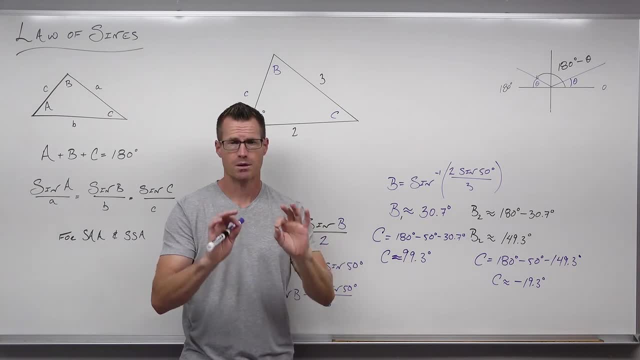 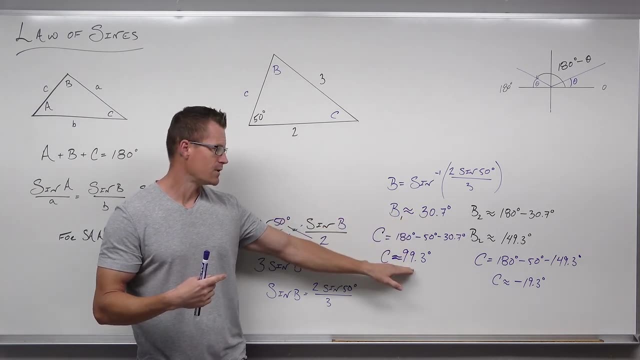 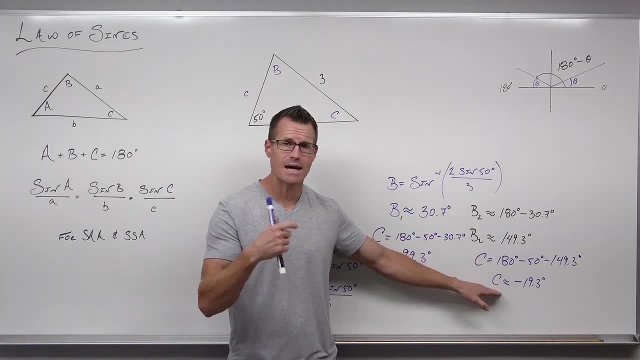 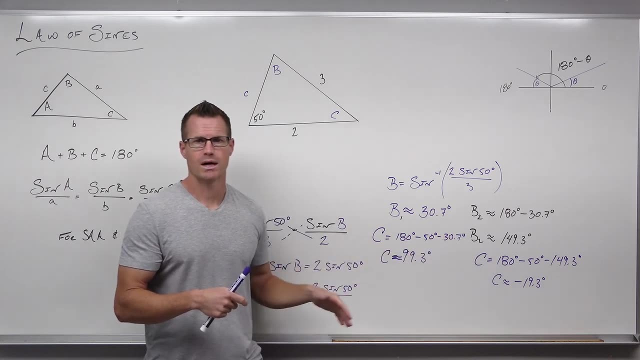 Use option two. If it gives you a valid angle, you're good. If it doesn't, then that's not possible, which means that this angle is wrong too. This is not an option for you. What if it gives you no possible angles? Then there's no solution, And that's exactly how we go through. 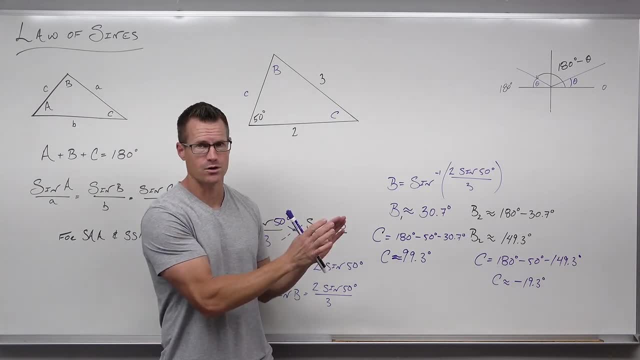 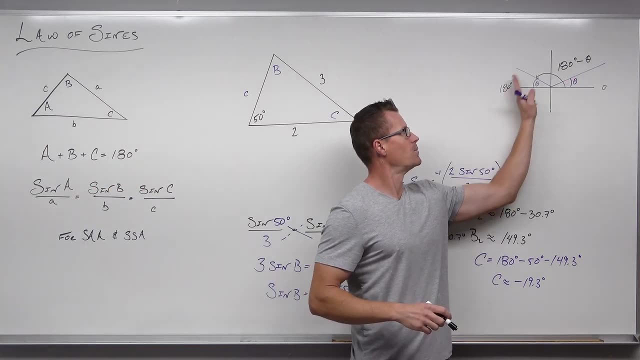 the cases. You don't need to know all four of them, It will work out in your sine function. So which is the valid case? Well, not option two. So this one worked, but this one does not work. Yeah, this isn't right for us. 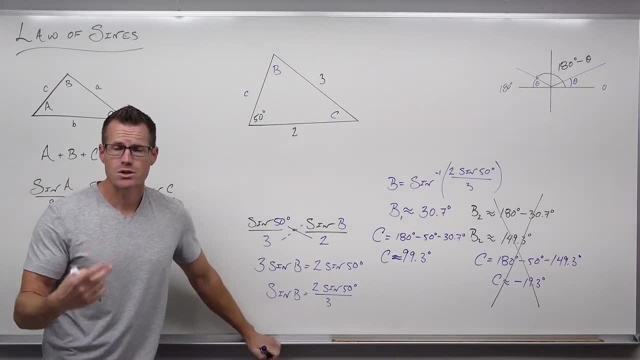 So we only have one option here. If we had two options, it causes you a lot more work because it says there's two triangles here. You have to use that to figure out your missing sides from those two triangles. So I know for right here that this is 99.3 degrees. 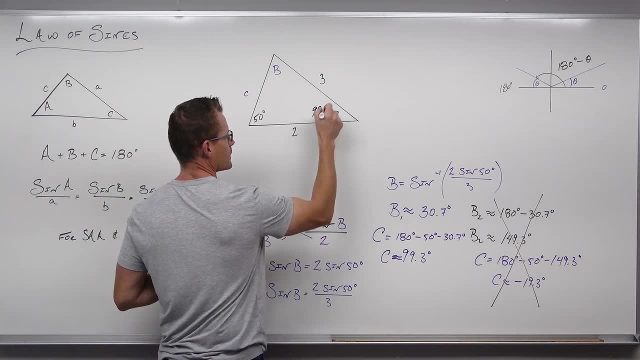 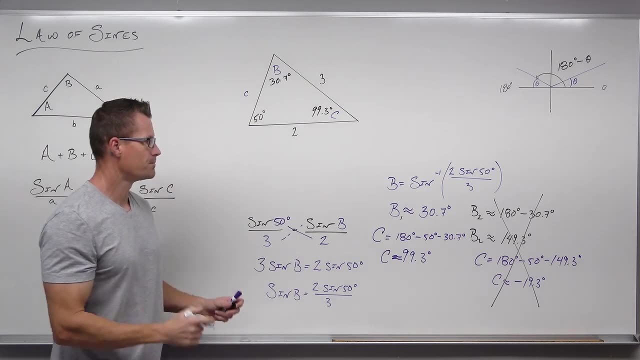 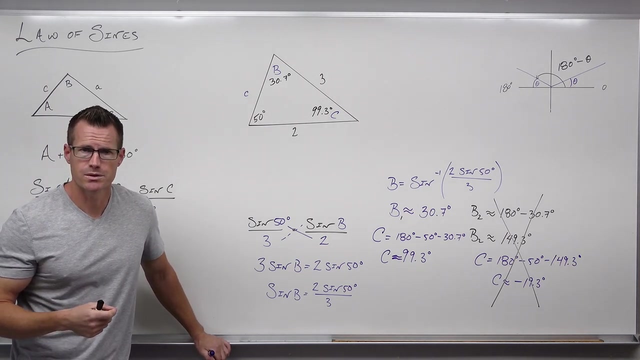 for angle C, because our only option for angle B was 37, 30.7 degrees. So we figured out that this is not an option for angle B, So we figured out both of our angles. That's typically what we do when we're using law of. 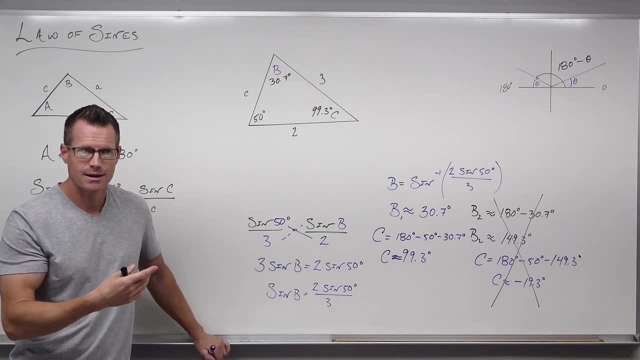 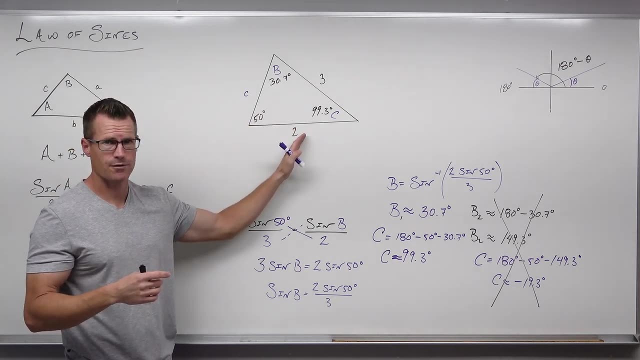 signs for side-side. angle is you find your first angle? Why? Because you have to. You can't find a side first? Why not? If you only know one angle and two sides, you can't find a missing side. You have to find another angle first. In fact, you had to find that angle first. That angle gave you. 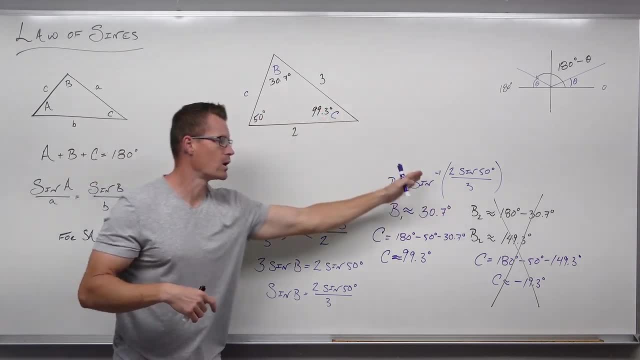 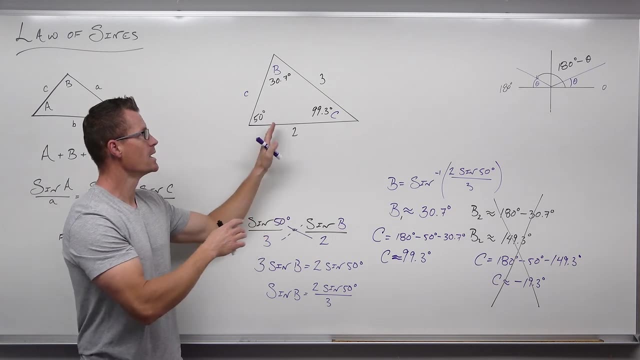 two options: option one or option two. Only option one was valid because option two came up with something that was a contradiction. You cannot have a negative angle in a triangle. You can't have a negative angle in a triangle. So we only had one option. If you had had two options, you'd be. 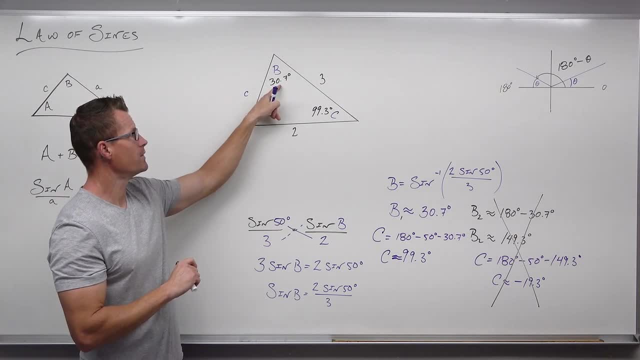 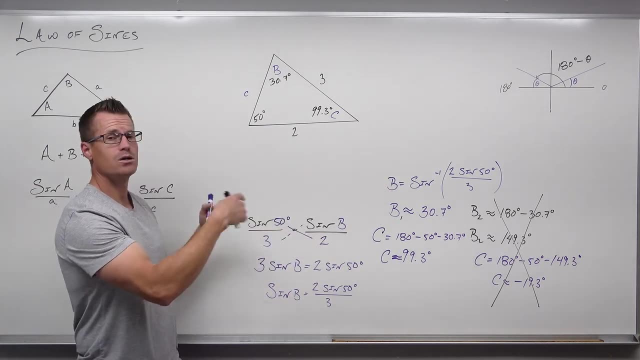 drawing another triangle right now. You'd be saying, okay, I have one that's 30.7.. I have another one that is whatever. it is 149.3,. if that had worked, And then you would use that to find the last. 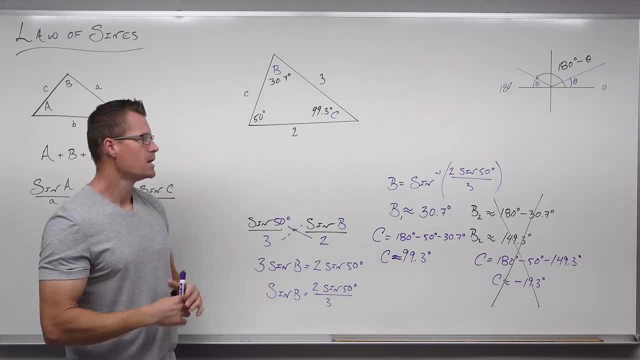 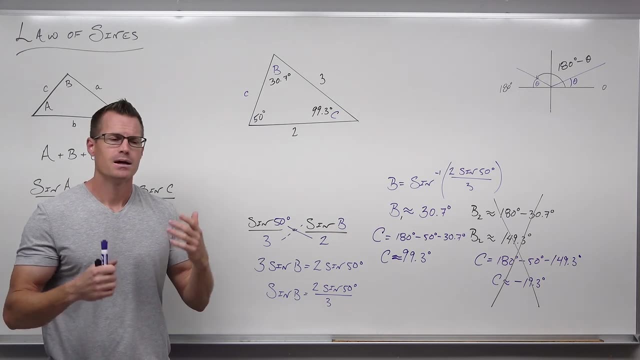 remaining side, So you could have more work on this, Now that we only have one option. we know that's about 30.7.. We know that's about 99.3.. We're going to find the missing side. Now what I've said. 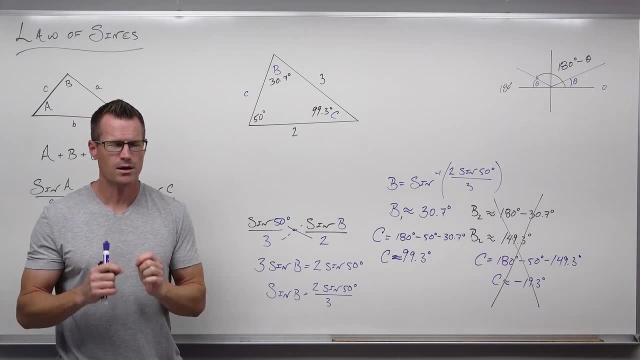 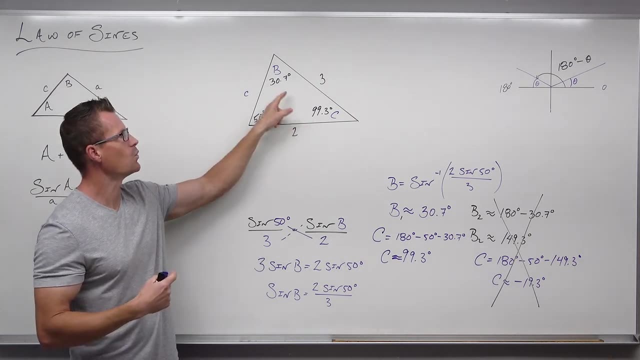 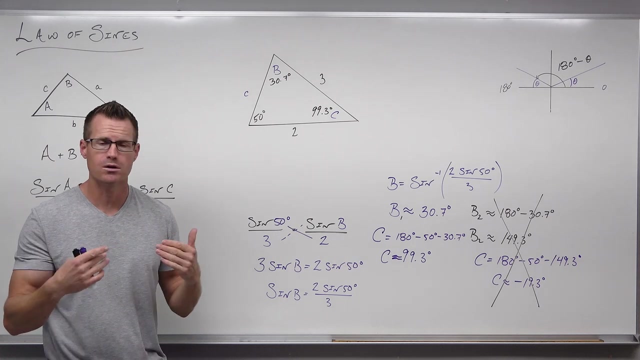 is avoid using rounded numbers if at all possible. In this case, it's not possible to avoid using those rounded numbers. You're going to have to use one of these two angles. Which one? It doesn't matter which angle you actually are forced to use. They're both going to be equally rounded. 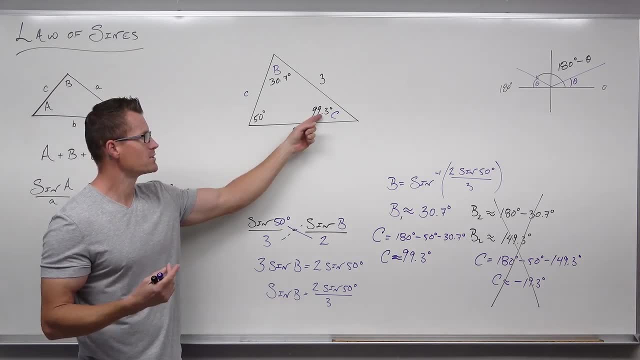 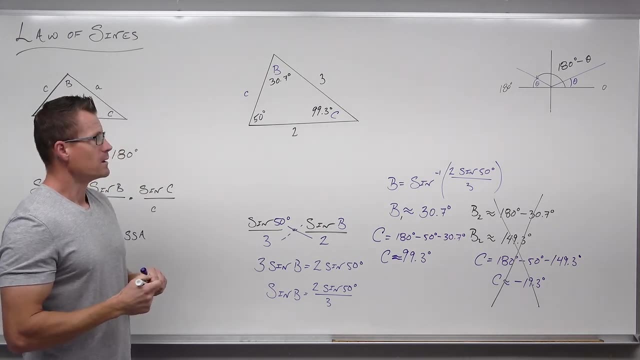 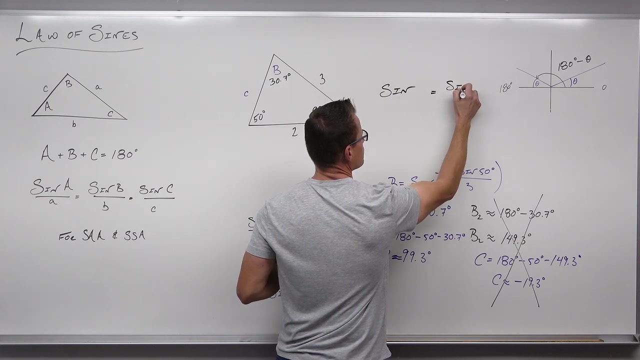 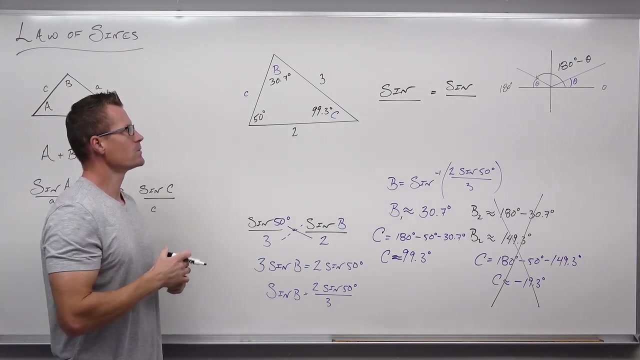 So it doesn't really super matter. So we have to use this at some point to find that missing side. That's okay, It's just something that we're dealt with. So let's set up the Law of Sines again. What Law of Sines says is: hey, if you know two angles and a side, you can find a missing side. 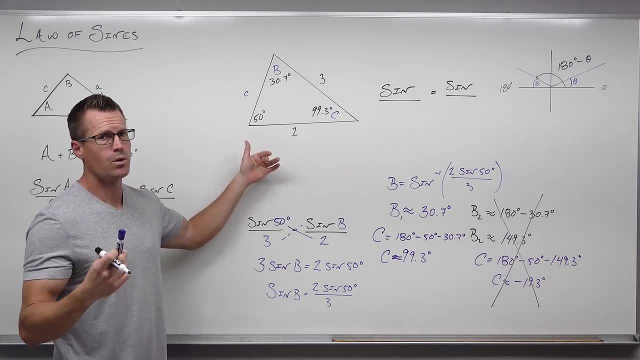 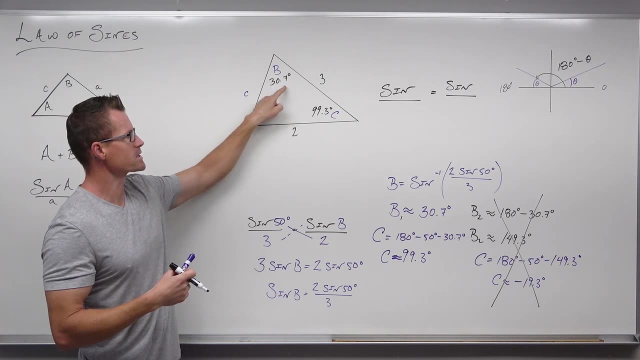 I do know two angles and a side. Now here's what I won't do. I won't use too many rounded numbers if I can avoid it. So what that means is I probably am not going to go sine 30.7 over 2. 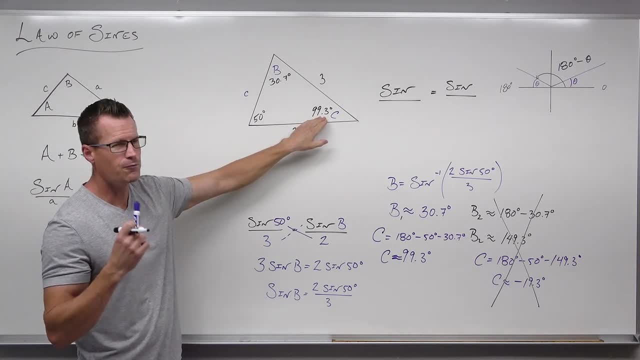 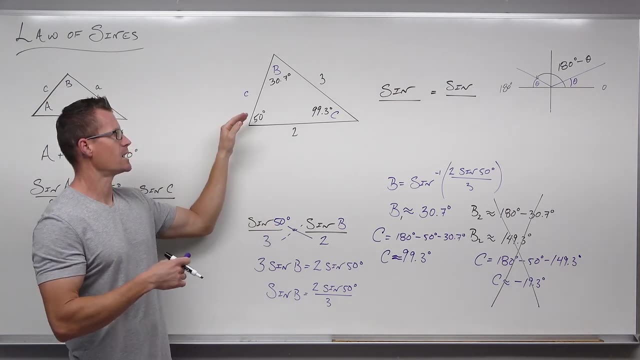 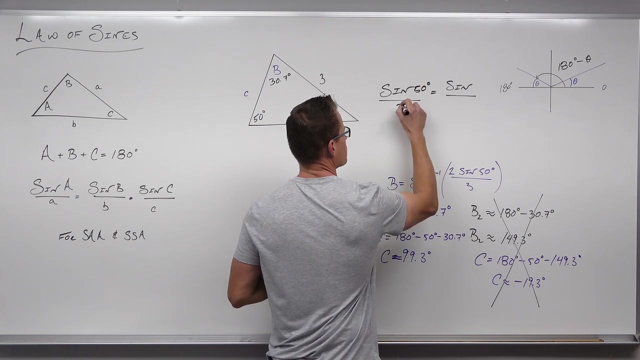 over c. Why? Because that's rounded and that's rounded. Avoid using rounded numbers as much as possible. Use the things that you're given if you can. So I'm certainly going to say sine of 50 degrees over 3, because both of those are given and they're not rounded. Equals sine of angle, I know. 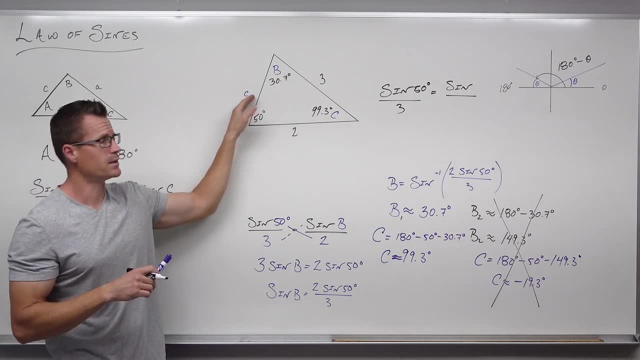 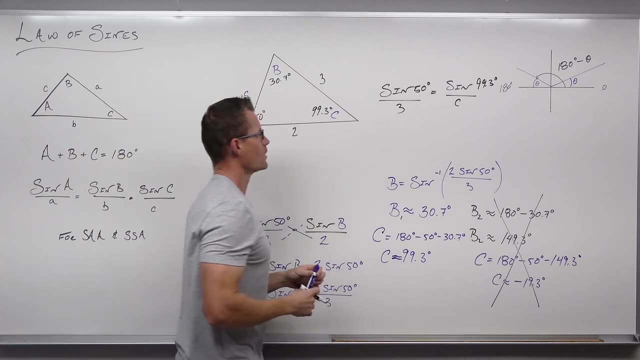 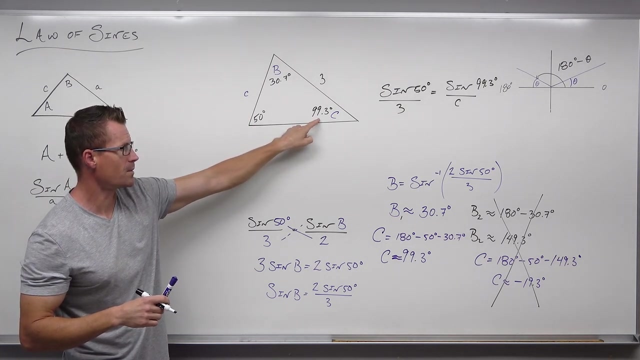 over opposite side that I want to find. So 99.3 degrees Over c. I'm going to double check Stuff. I know this is opposite Things. I want to know over an opposite angle. that looks pretty good. I'm going to cross, multiply and divide, So at this point 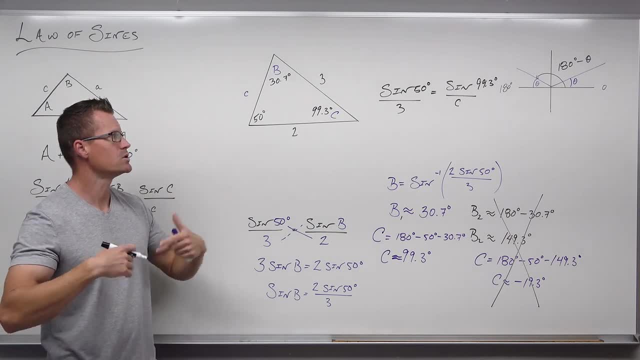 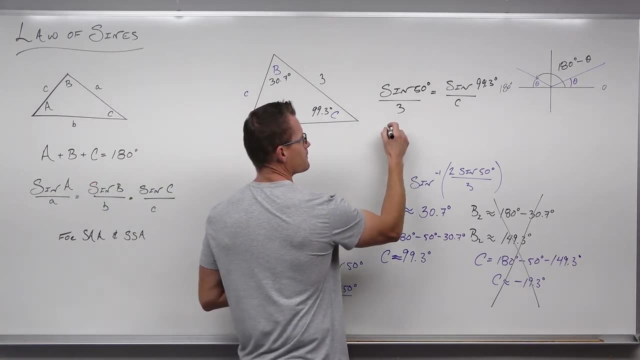 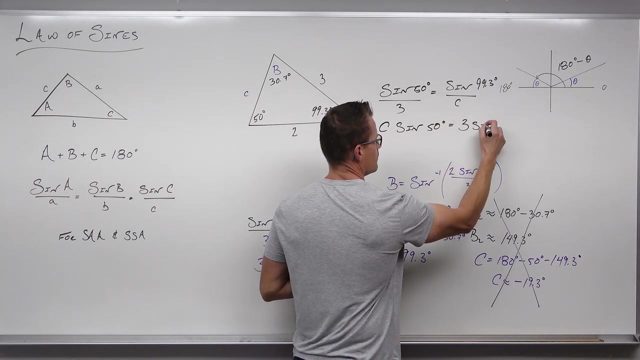 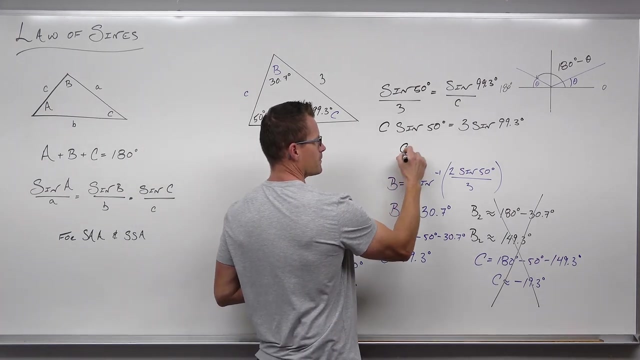 this is exactly like the first case, The first examples I gave you, where you knew two angles and one side. Now you know two angles and one side, So it's kind of simplified the case for you. So cross, multiply And we're going to divide. I hope you're seeing also that while we want to avoid using rounded 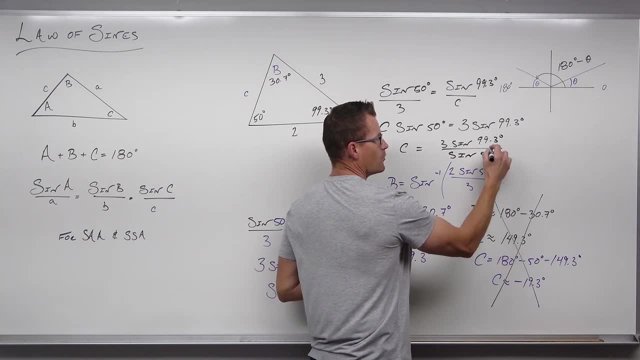 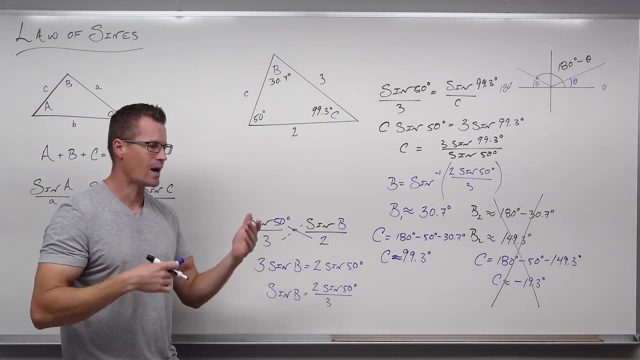 numbers as much as we can. we actually did that. We avoided using that rounded thing in lieu of using this one. Sometimes it is not avoidable with law of sines, because you had to find that angle, to find that side, and that's rounded, That's approximated. 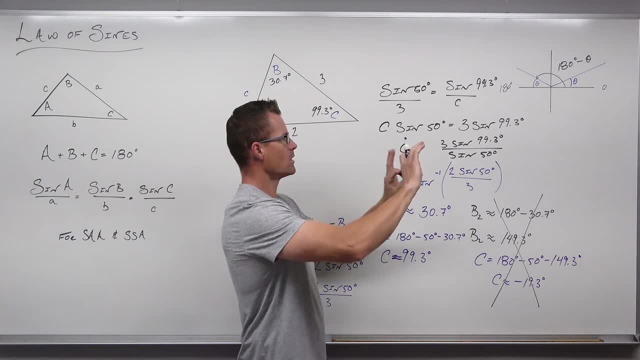 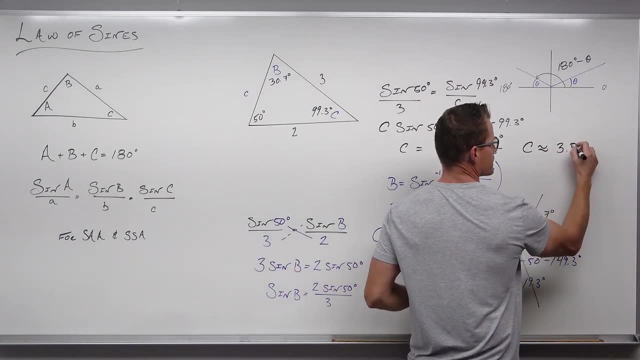 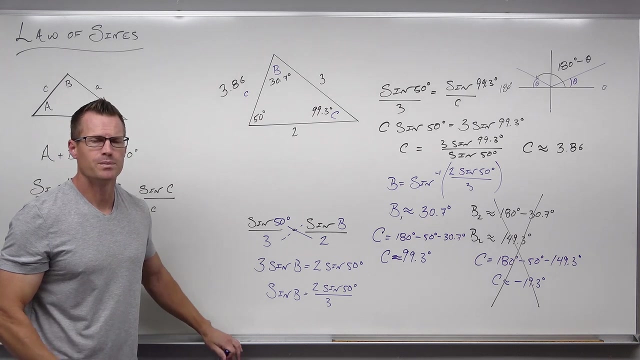 So c is going to be 3 sine 99.3 over sine of 50. That's about 3.86, whatever units those are. Last little bit to sort of check your work, not prove that you're right, not find mistakes. 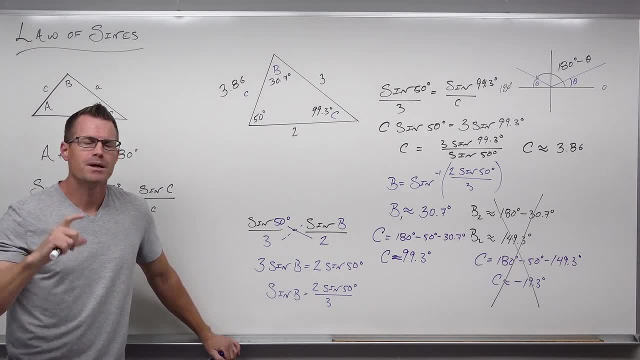 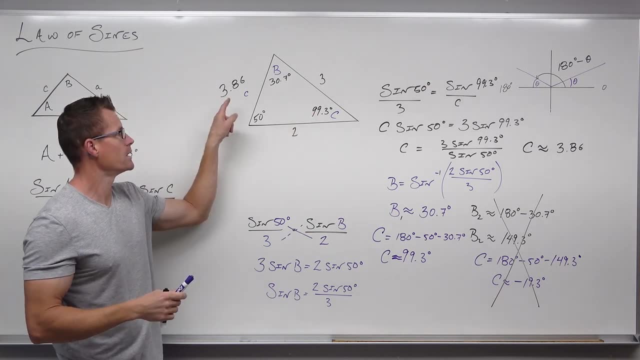 but at least that you haven't made one is that bigger angles open to bigger sides. So 99.3.. 9.3 degrees should open to the biggest side because that's the biggest angle It does. 30.7 should open to the smallest side because the smallest angle it does, And that should be right. 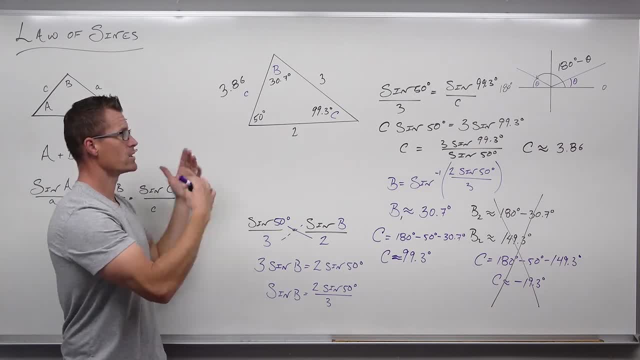 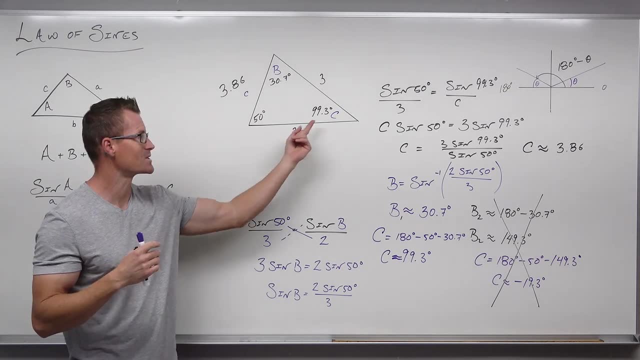 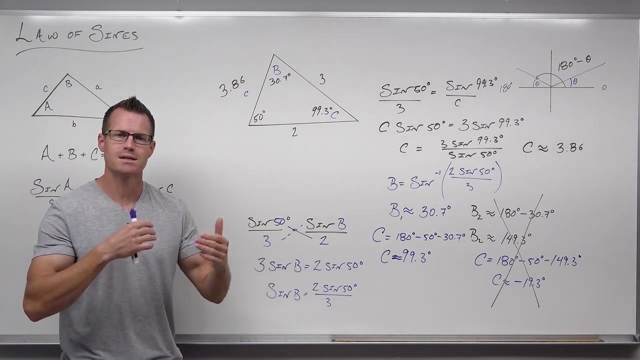 between them. So that's a great way to check your work. It's why I draw a triangle. The last one is- hopefully, it's obvious- These two not have to be to scale. They don't have to represent the correct angle. 99.3 is over 90 degrees. It's an obtuse angle. It's just a way for us to get a picture. 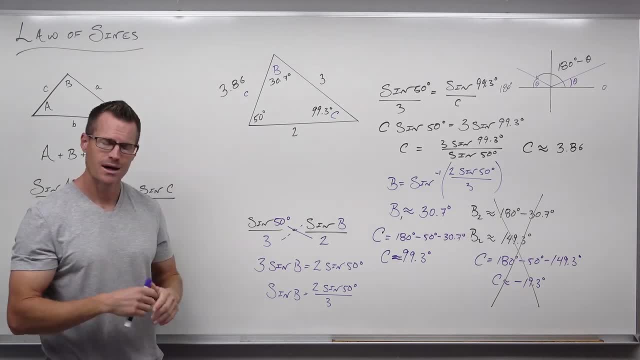 down so we can. we can visualize it. So it doesn't have to be the smallest angle, but it does. So it doesn't have to be perfect. Man, I hope that's made sense. I hope that you're seeing that while. 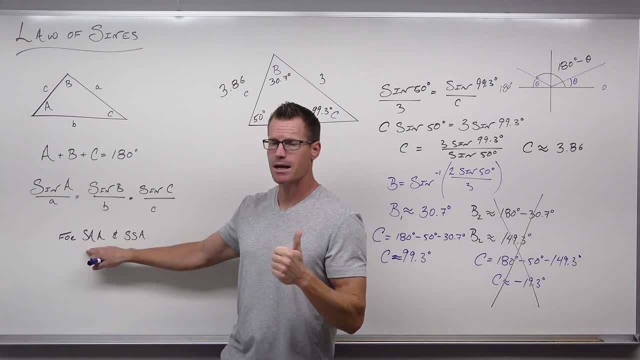 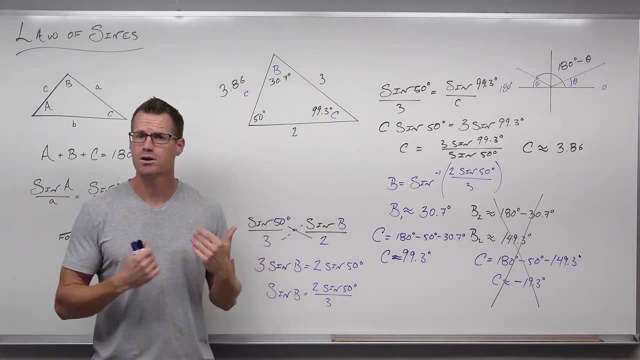 this one is pretty easy, because you're just finding a missing side and there's no options. This one can be a little tougher. We really have to know what we're doing and it relies on your knowledge of what sine function does on even circle. So when you find an angle, 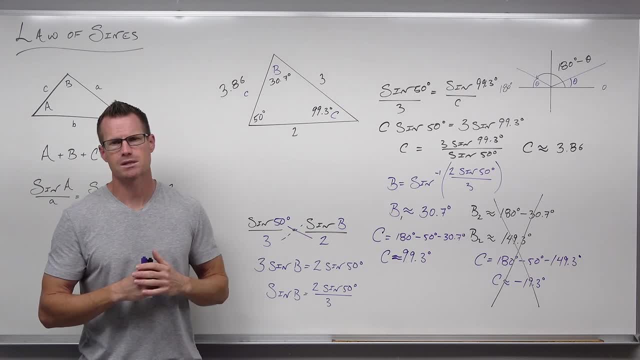 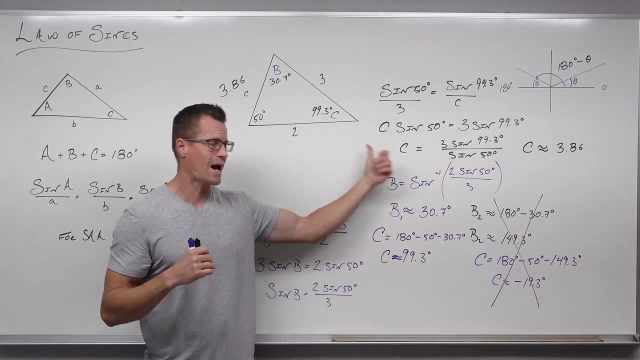 you need to have two options and we're going to do that with this, the law of signs. So we have our two options. We go through both of them. If they both work, you have twice the work. You have to do more work here. Set up two triangles If you don't, or at least draw. 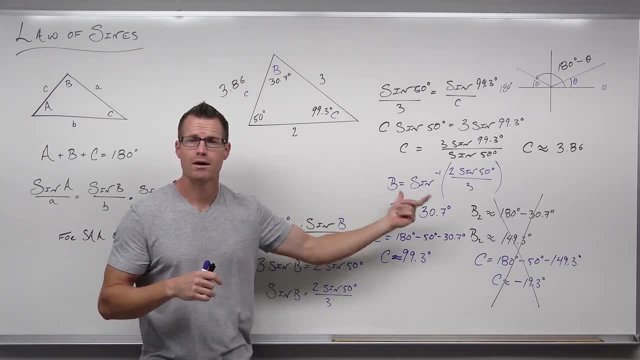 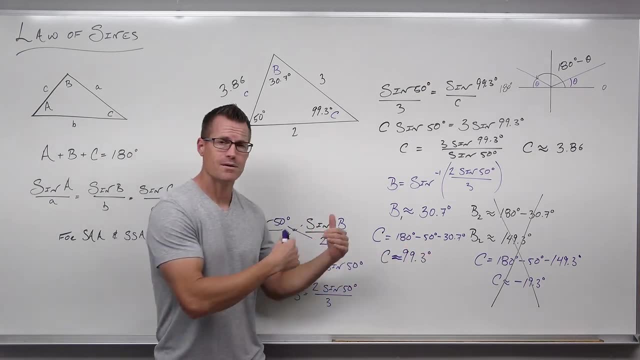 write this twice. That's fine. You can erase it If you. if you don't have two options, then it will show with just some logic you're going to get a negative angle somewhere. It'll show that you don't. if you have two cases that they don't work, both of them don't work. 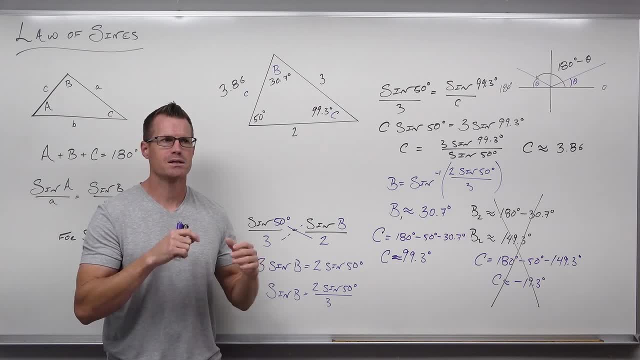 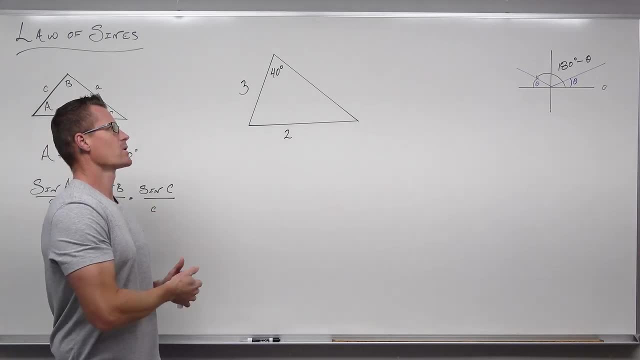 then you have no solution, So let's keep on going. I'm going to show you next the case where you have two triangles that are possible. All right, let's go ahead and try another one. So we're taking a triangle. We noticed that it's not specifically telling us the right triangle. We don't know. 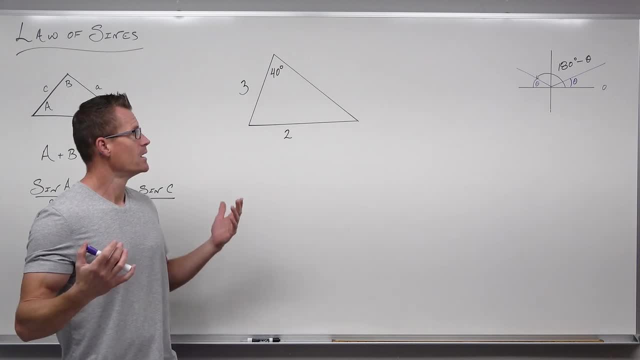 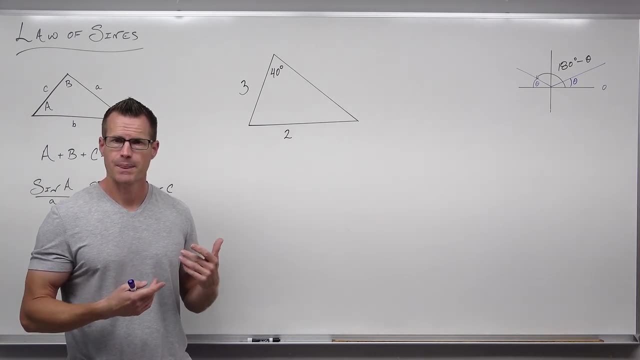 really what it is. So we're not using right triangle trigonometry. We're taking a look at it then. Are we in the case where we have law of signs? Are we in the case where we have law of cosines? Look at what you're getting. I'm given two sides, I'm given an angle that's not between. 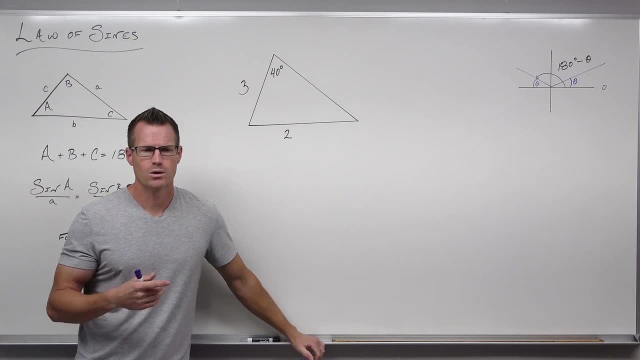 them. Also one thing I want to say: a lot of textbooks um will in in your homework or your practice or whatever. they'll give you a triangle with ABC and ABC is angles and sides, And they'll say, Hey, do this If little a is this and little B is this and angle C or whatever. 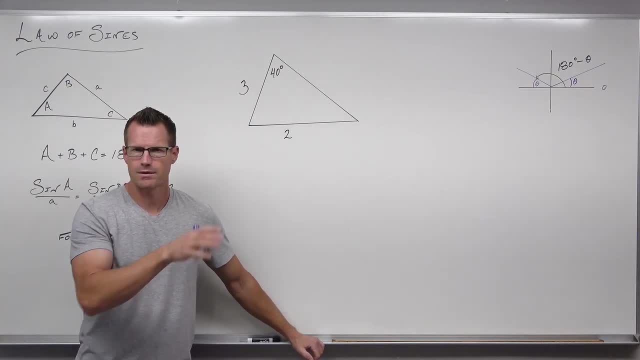 is, is this? um, when they do that, they're just drawing a triangle, Like I'm doing. you just have to do it yourself, because they probably don't want to waste space or something I don't know. Um, so that that could happen, Just draw your triangle, make sure you have the angles and sides. 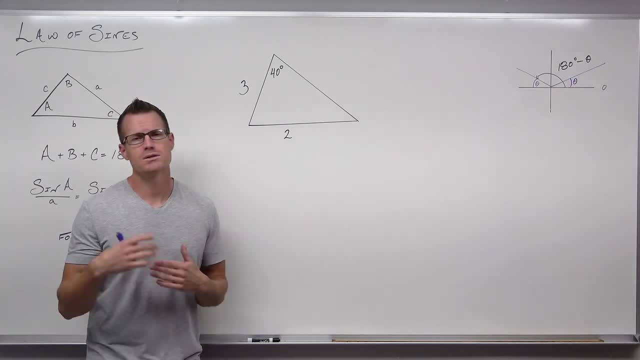 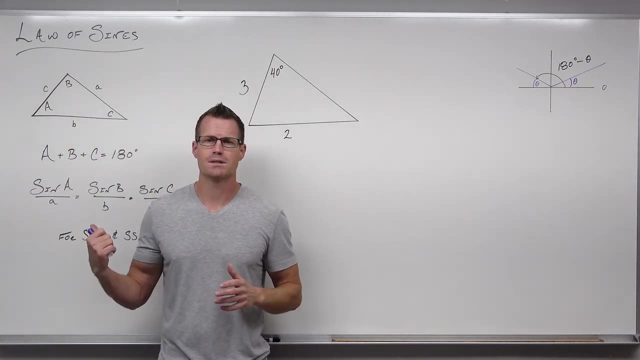 in the correct relationship. So I'm looking at this thing and I'm going to be using law of signs or cosines. Uh, I see that I know two sides and an angle, not between them. That's going to give you law of signs. Also, in my head right now I'm thinking I'm probably going 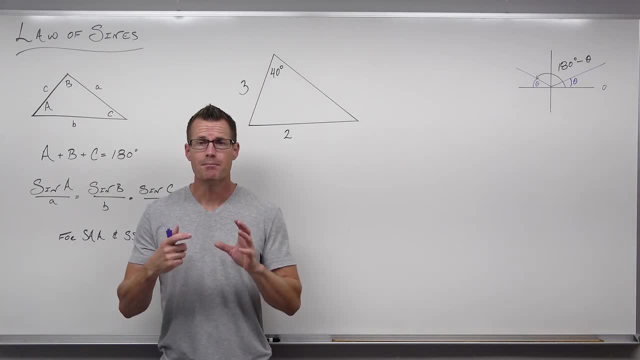 to have two options coming out of this. I'm definitely gonna have options. Maybe both of them work, Maybe one of them works, maybe none of them work, but I'm certainly going to have two options in finding that first angle. So I'm thinking law of signs, I'm thinking side. 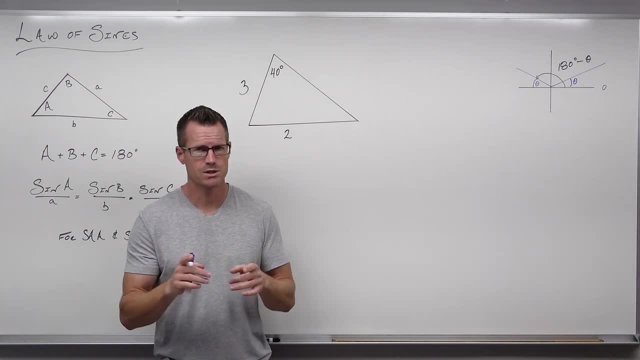 side angle. I'm going to have to find an angle first. I hope you see why you can't find a side first. here There's not enough information to do that. Um, so I know I'm finding an angle first. I might label it, I'm thinking law of signs. I might write down the proportion. uh, sign over. 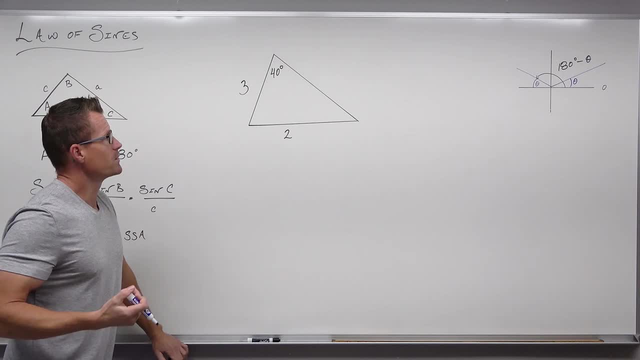 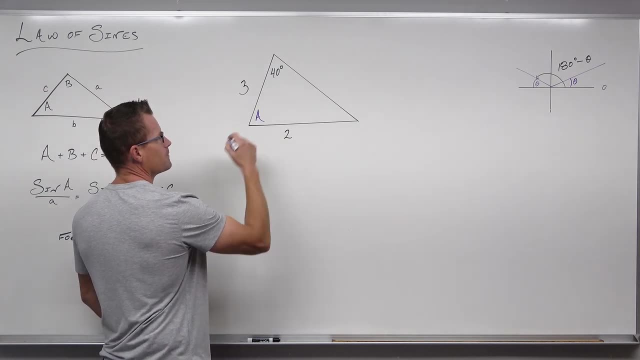 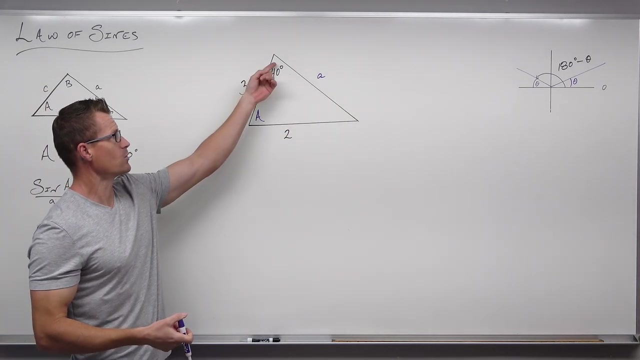 side equals sign over side, But ultimately, what I'm going to look at is: let's start labeling these. I might label this angle a, in which case the opposite side would be lowercase letter a. maybe this is angle B over lowercase letter B And this would be angle C over lowercase letter. 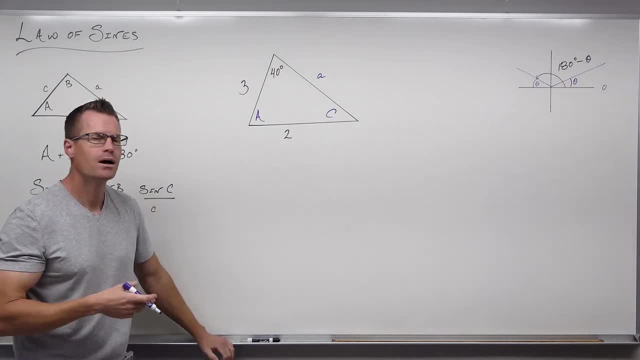 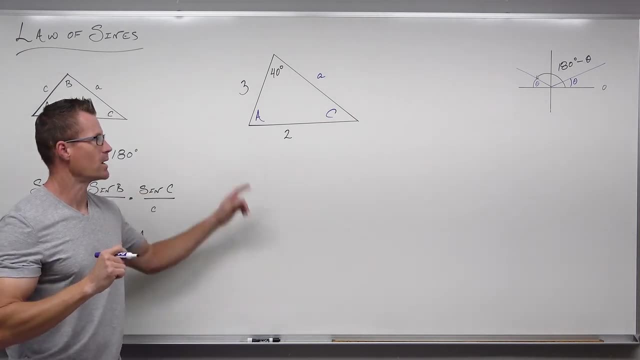 C. You don't have to write the B and the C. you can if you want to. it doesn't really matter. but you need to label the things that you, you don't know, and label them with the letters matching opposite. So a with a, C with C, B with B, If we know two sides. 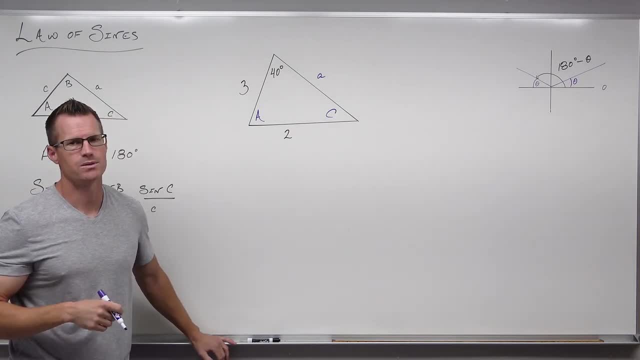 we are only missing one side, but we're probably missing other triangles. So what can we do? What can't we do? You can't use Pythagorean theorem, Uh, we can't use right triangle trigonometry because we're not sure. And we also can't use interior angle sum of a triangle, which means: 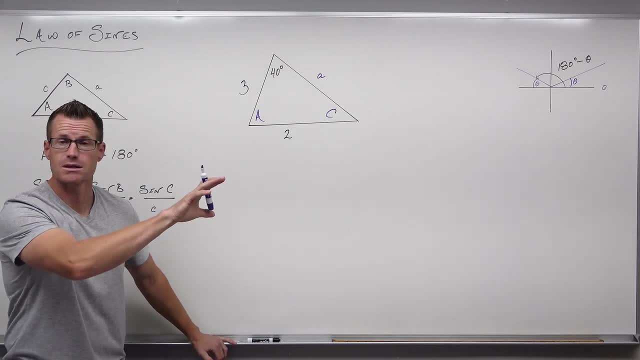 that we have to use law of signs, or, in other cases, law of cosines, first. Uh, it also means that we're going to have to use some rounded values in future math, but we're going to avoid using too many if we can. So I know that this is going. 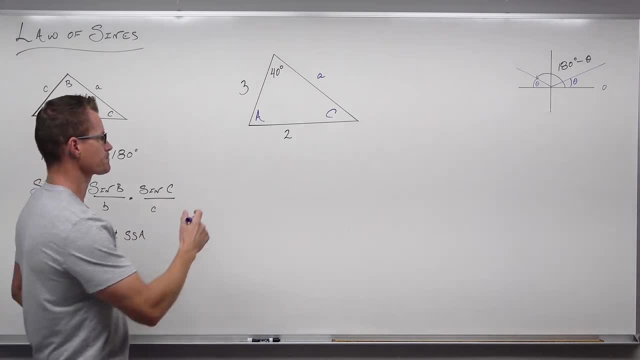 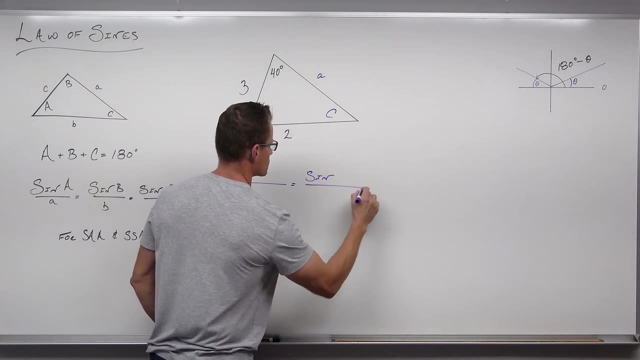 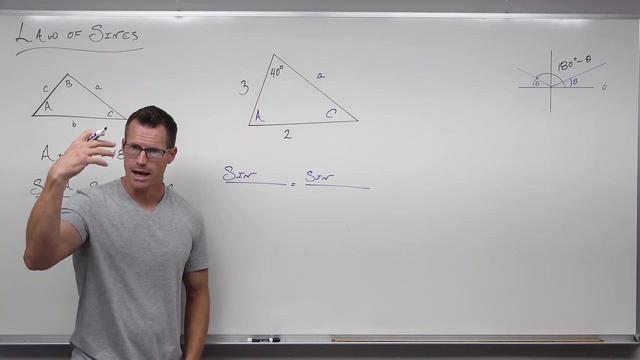 to be law of signs. I'm going to go ahead and I'm going to set up my proportion. Okay, What's that mean? I'm going to have to set up one fraction with things that I fully know. So an angle over a side. 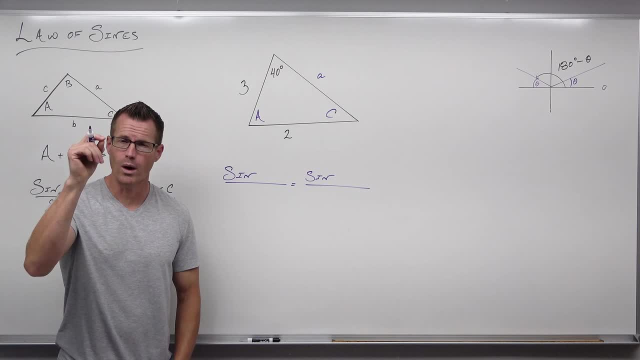 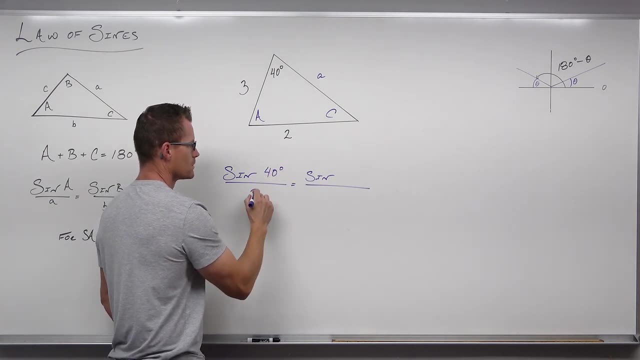 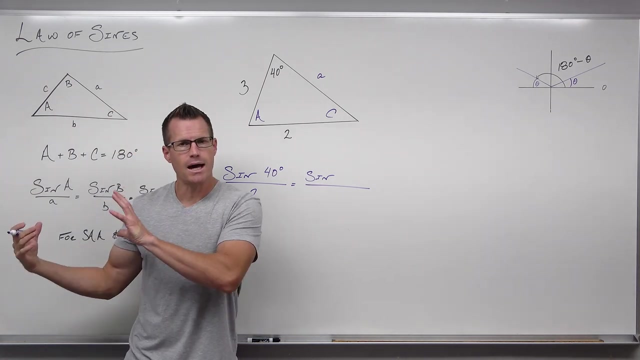 law of signs requires that you have to know at least one full relationship and angle, and it's opposite side. Now I know that I know 40 degrees and two, Perfect. Now to find a missing angle, you need to know another side. Well, we do. That's what side side angle tells you. You would know a. 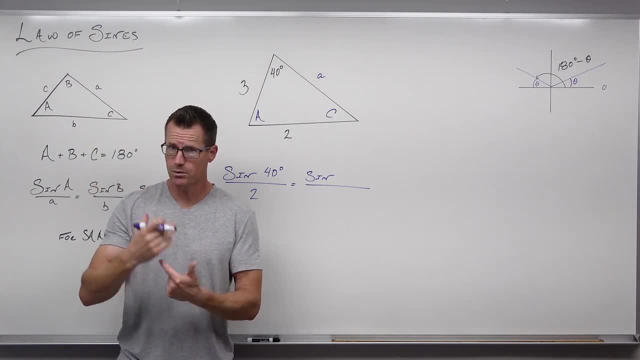 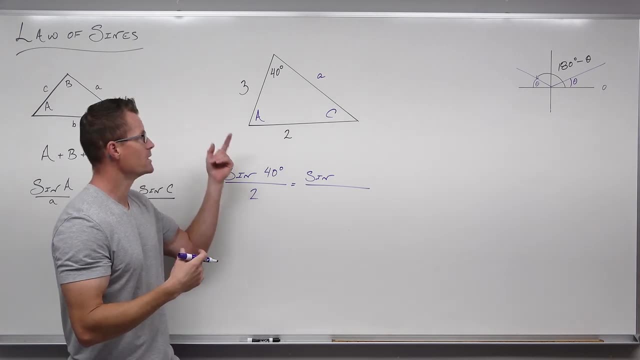 side and an angle. Those will be at some point opposite one another and you would know one more side but not an angle opposite. So I know this side. this is going to set up with finding angle: See notice right now. 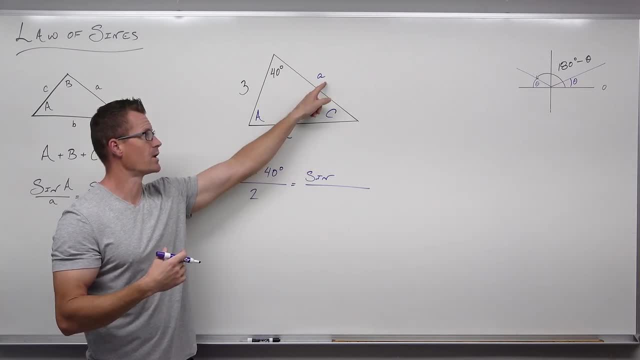 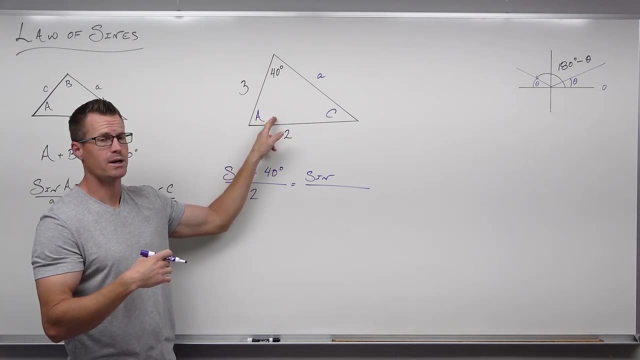 there is absolutely no way for us to find angle A angle a over a would not, would not, create something where you know three parts to find a fourth. Um, we do not know interior angles, So there's no way to do that. right now. You're forced to find angles. Well, it's kind of nice, It. 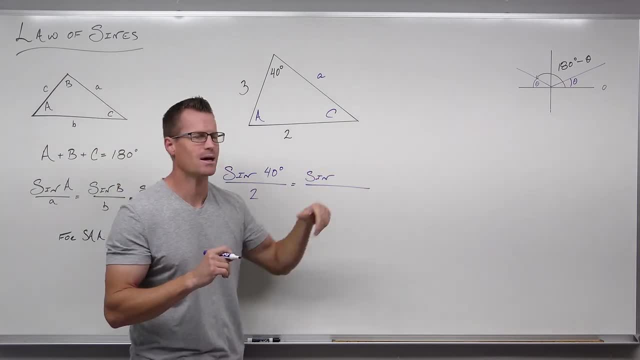 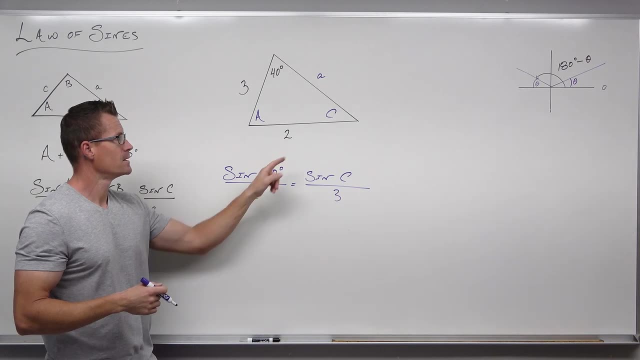 eliminates options but then it creates more by finding that angle. So sign of angle C over three. I'm a double check. Hey, 40 degrees side opposite, Got it. Sign C Of side opposite, that I know I got it. So at this point we're just going to cross, multiply, We're. 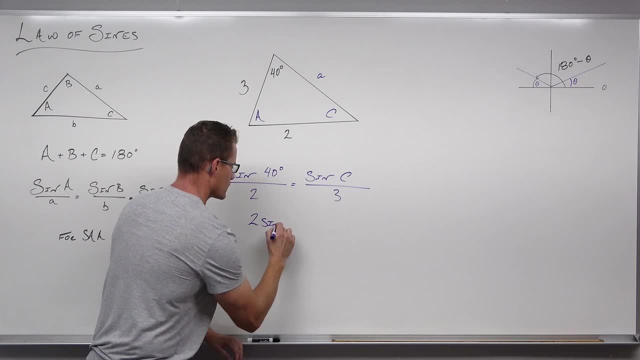 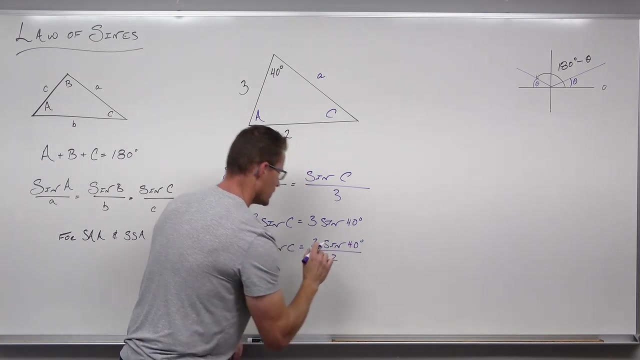 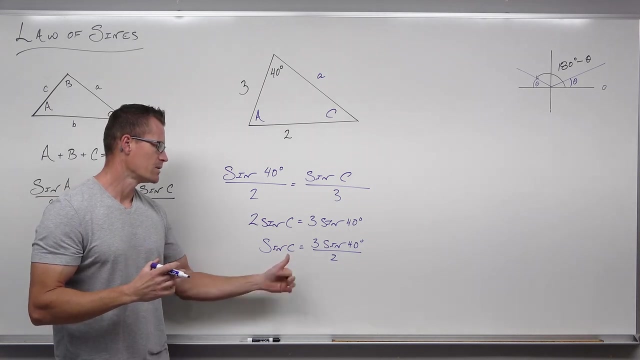 going to divide. We want to make sure that we're not dividing both sides by sign C, because you're you're trying to solve for the angle C, So we're trying to eliminate Everything around that angle. So divide by two and hopefully remember that if you have an angle. 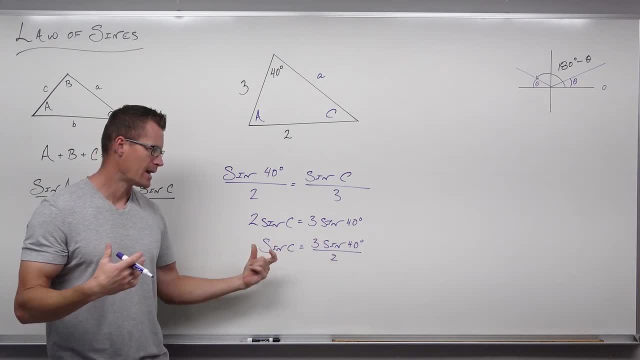 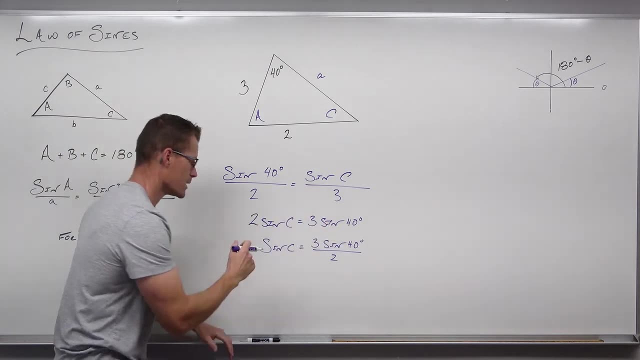 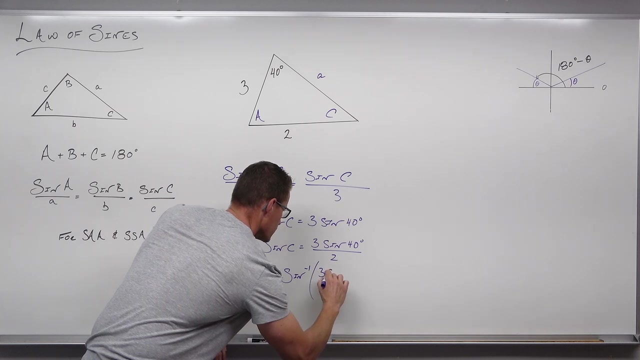 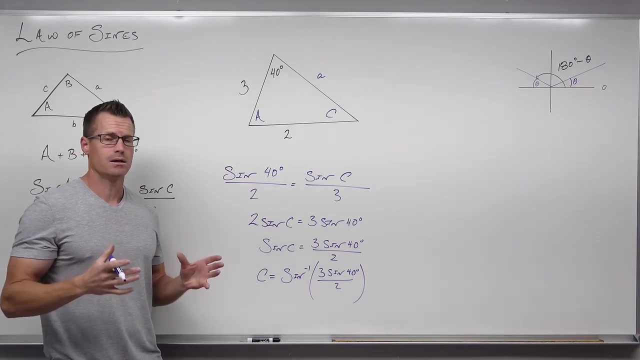 so sign of an angle equals some sort of relationship, that that angle is sign inverse of that relationship. So our angle C is sign inverse of all of this stuff. or take sign inverse of both sides. So Angle C is exactly sign inverse of all of that stuff. Use your calculator, approximate it. So C is about 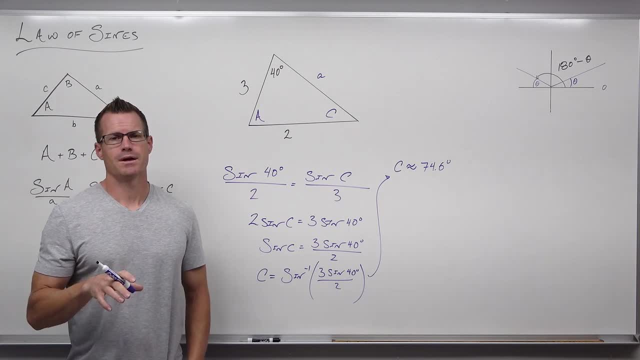 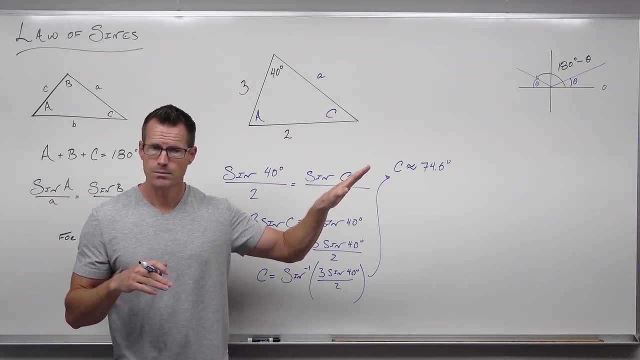 74.6 degrees. Now it's time to think. if you've just found this angle and you used sign to do it, remember that sign has two options. to give you out the same Value on a unit circle, You could have one angle, positive angle or 180 degrees. 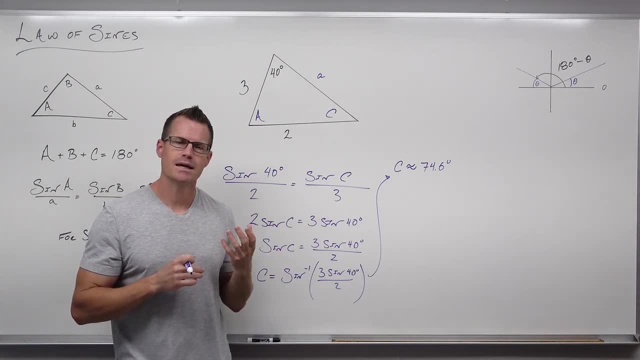 minus that angle, It would give you the same thing. It's kind of like taking a square root of a number. You do a positive and a negative. You go: Hey, because X squared will square both two and native two, to give me four. then both of those are solutions because sign of two angles. 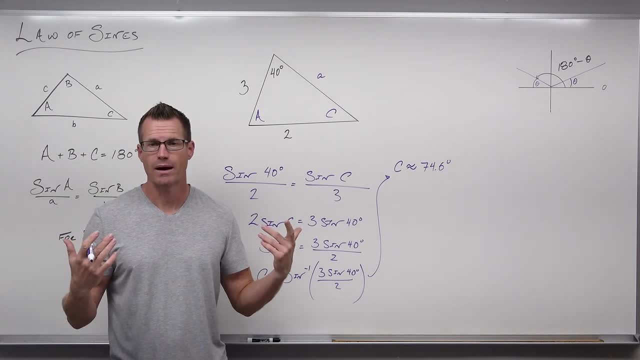 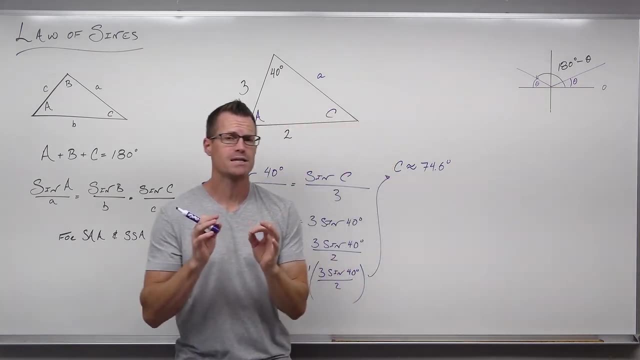 gives me out the same value. They both would have to be solutions here. Now, how do you find it? It's really right here. Your angle, or 180 degrees minus your angle, will give you out the same value according to the sign. 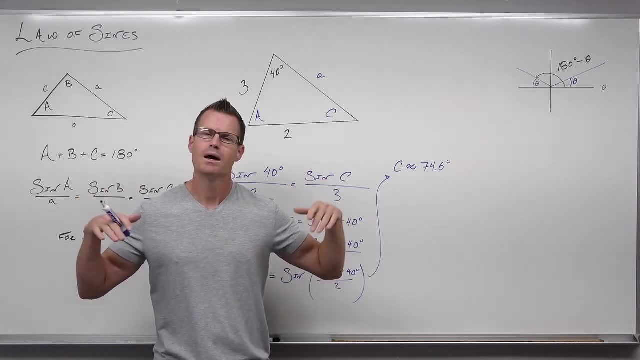 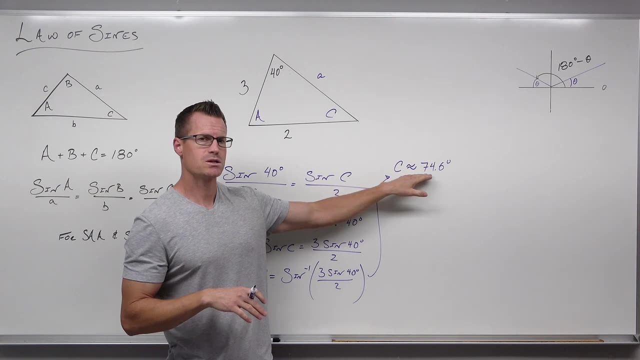 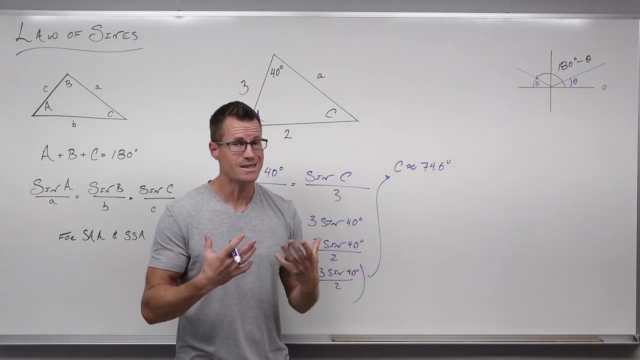 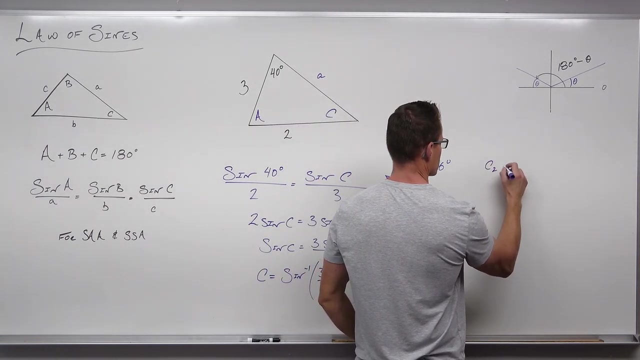 Function. They're both Giving you out the same exact output And therefore there would both be possible solutions. So we think through: if C is 74.6 degrees, then 180 degrees- 74.6,, 180 degrees minus 74.6 degrees would be the same thing According to our sign function. 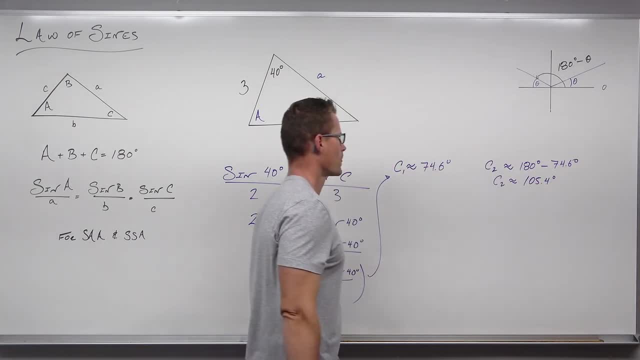 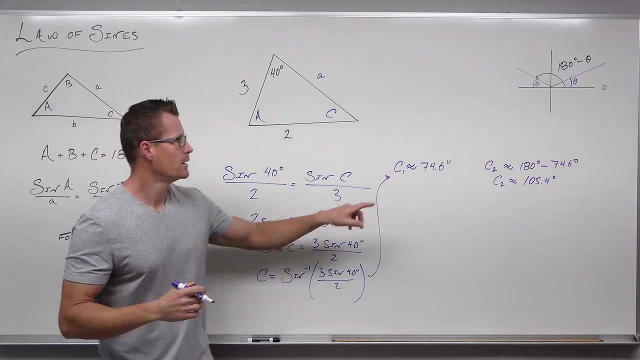 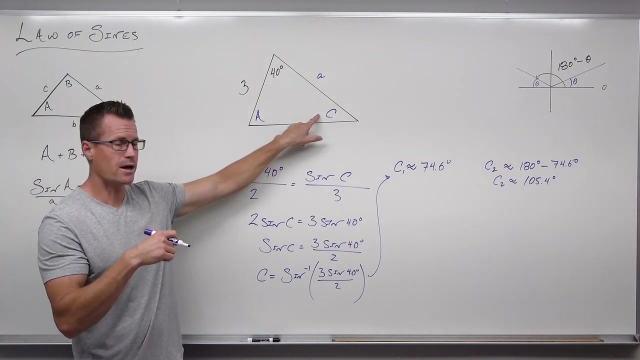 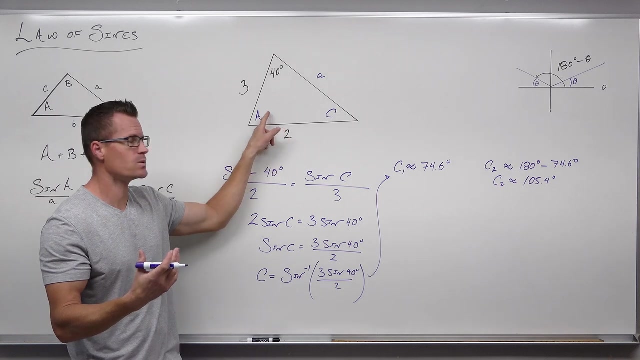 Now are both of those valid? This is the time that we check. We really have to think about it. Imagine that C is 74.6.. Is that going to leave you enough in your interior angle sum to develop another angle? Yeah, it appears. so 40 plus 74.6 isn't 180. yet That leaves you enough. 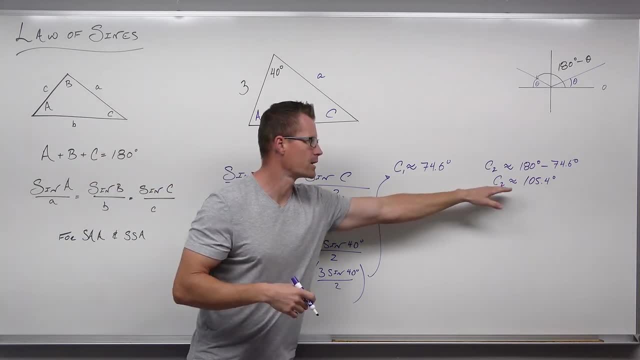 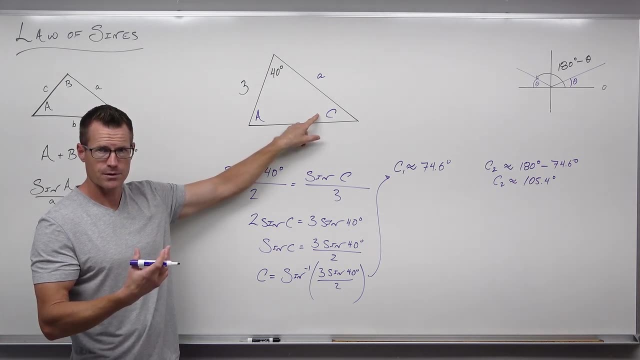 for to complete the interior angle sum Check. option two: plug in 105. Function. If this were 105.4 degrees and that's 40 degrees still, would that leave you enough to add up to 180 and allow room for the angle? Yes, This is the case where you actually have. 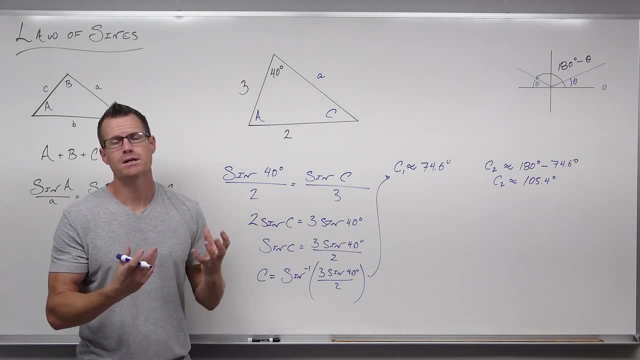 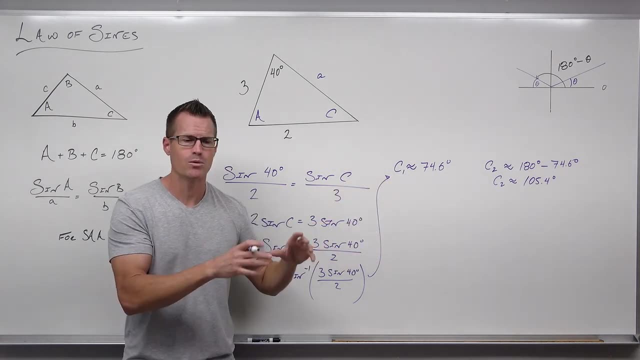 two solutions. So both of these are valid for interior angle sum. It will work out. if you just do interior angle sum right now, it'll show you you'll get no negative angles. So the last example, when we did it, option two gave us a negative angle. It was this impasse that you got to, That's. 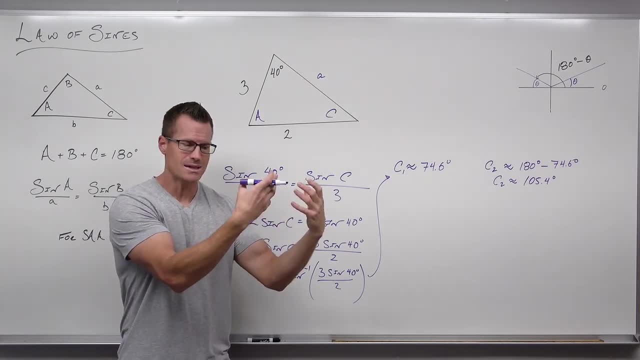 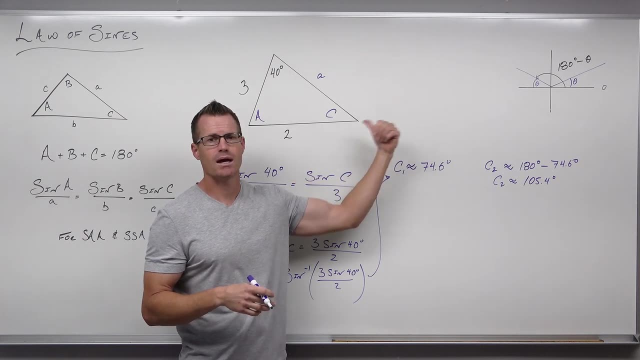 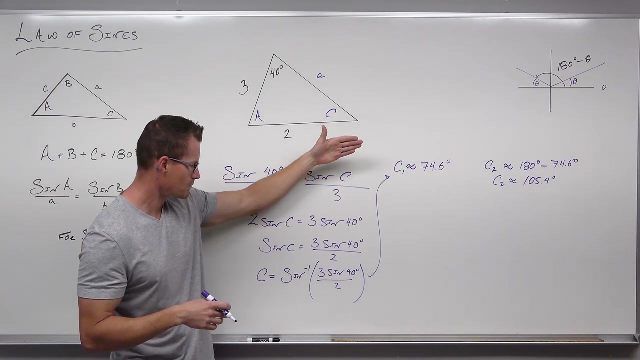 not possible? Perfect, We'll try everything until it actually shows you whether it's possible or not. So all we've done is say, hey, sine functions, give you these two angles out that have the same y value on a unit circle. So sine of 74.6 degrees would give you this out, or sine of 105.4. 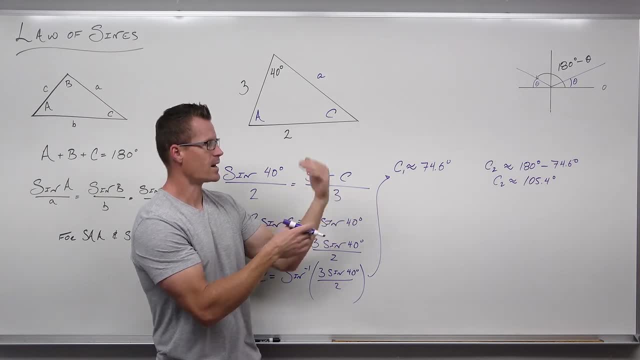 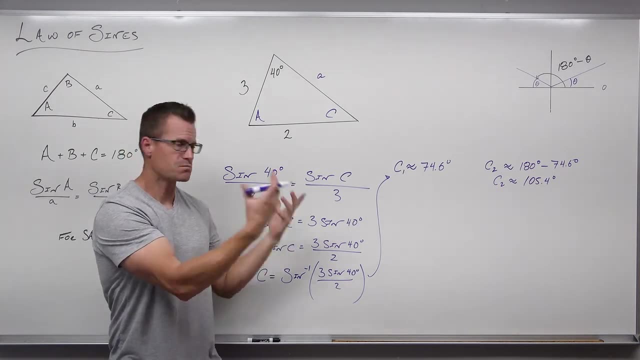 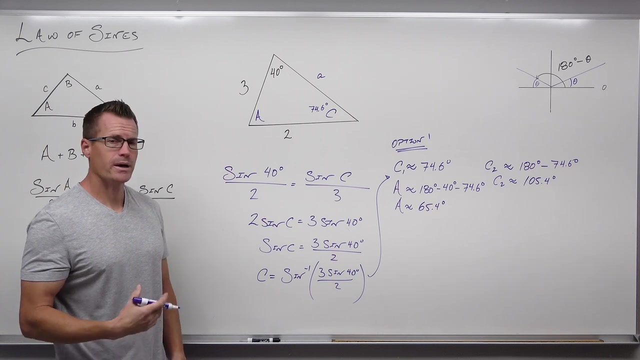 degrees would give you this thing out- either the angle or 180 minus the angle. Now walk through and see if interior angle sum- that's what you're using- is valid for both of these. So option one: if option one is 74.6 degrees, then angle A would be approximately 65.4 degrees. That makes sense. 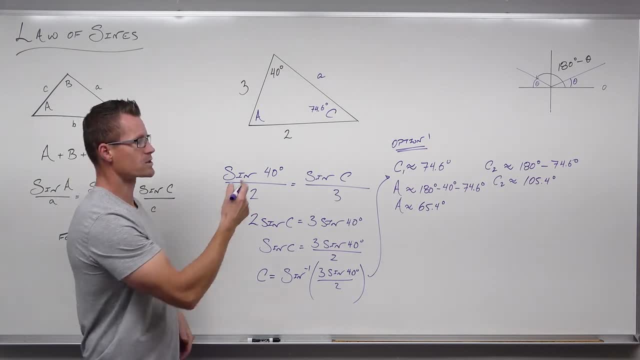 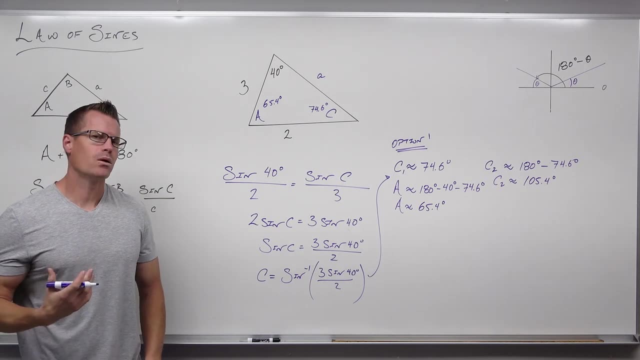 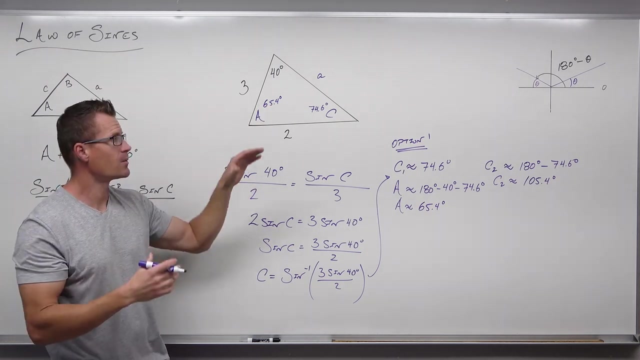 That's not a negative angle That doesn't ruin our interior angle sum. So I would put that down. Could you now go and use this information to find lowercase letter A? Absolutely So. you'd have to use a rounded number, but you'd use sine of 40 degrees over two equals sine of 65.4 degrees. 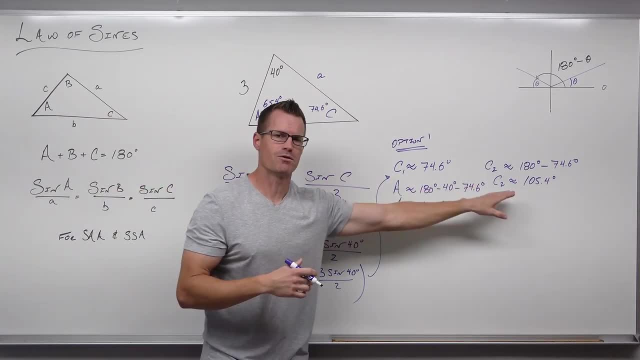 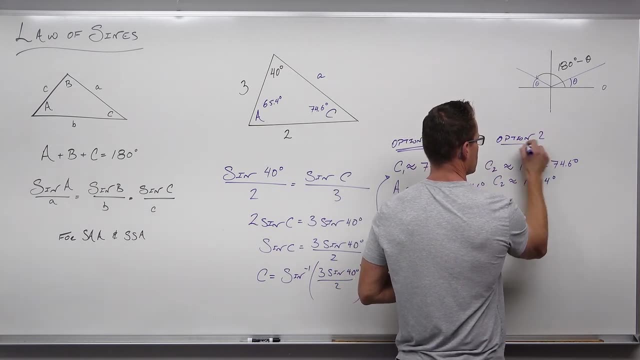 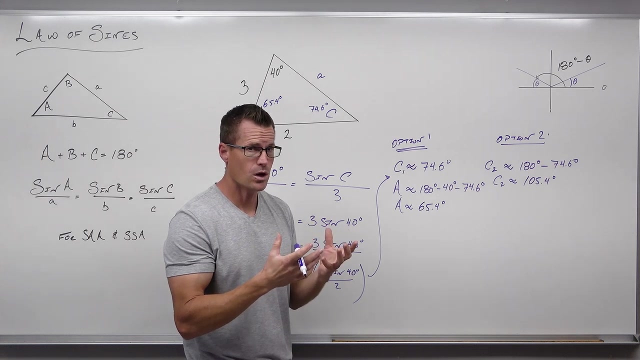 over the last remaining side that you need to find. What about this information? Option two: Option two would be: take the angle 105.4 degrees and then you'd use sine of 40 degrees over two equals sine of 75.4 degrees. 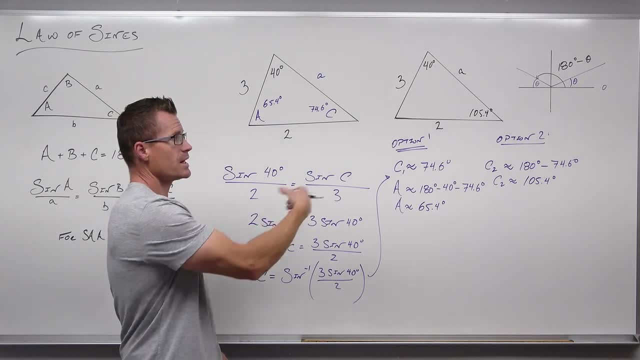 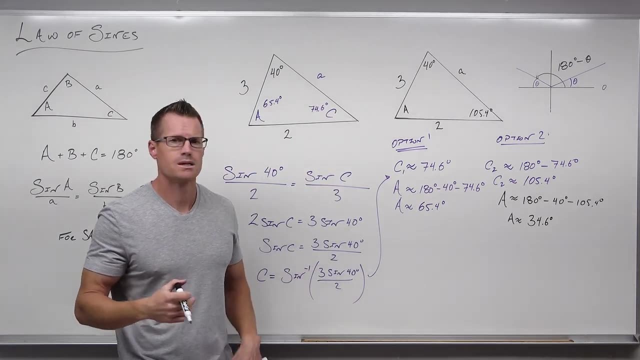 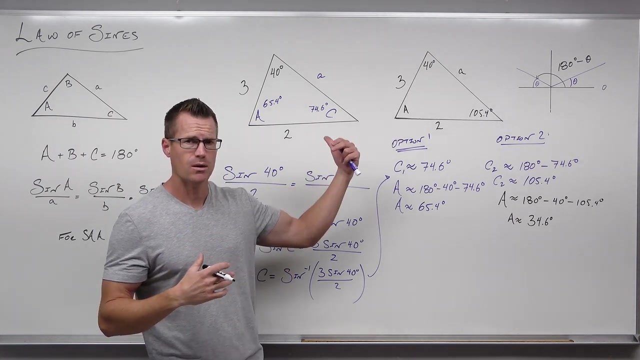 So that's valid for both of these. Think about this as that You might want to draw another triangle here, Option two. If option two is the case and we've drawn another triangle, then angle A would equal about 34.6 degrees. That's also valid, So we haven't run into anything. 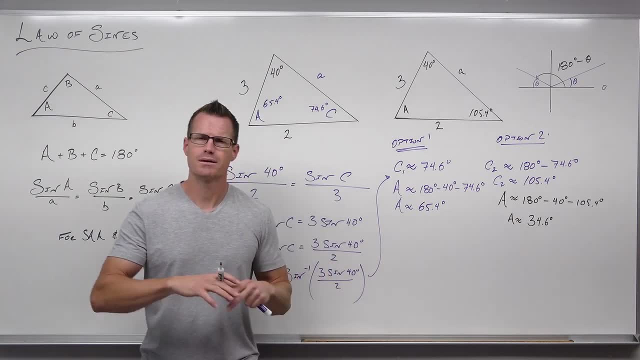 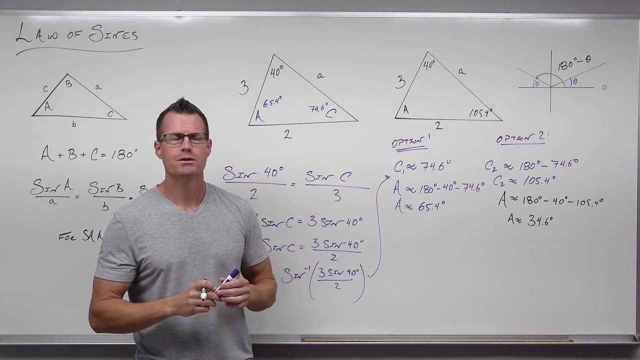 that says this isn't possible. We've used sine to give us two outputs, and both of those outputs are positive. So if there's enough to create triangles with both of these angles, you have two triangles available. Notice how you don't need to know the outcome before you start. 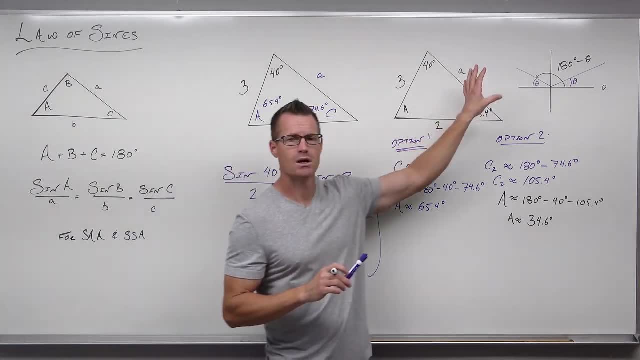 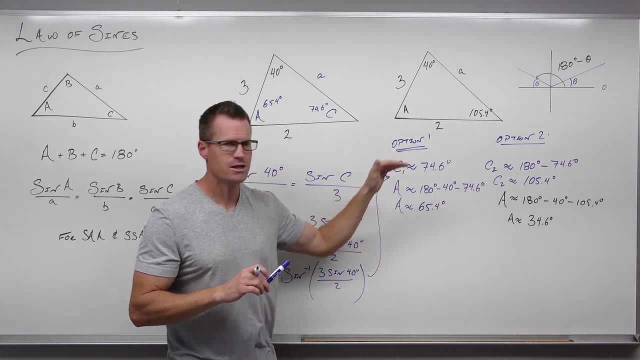 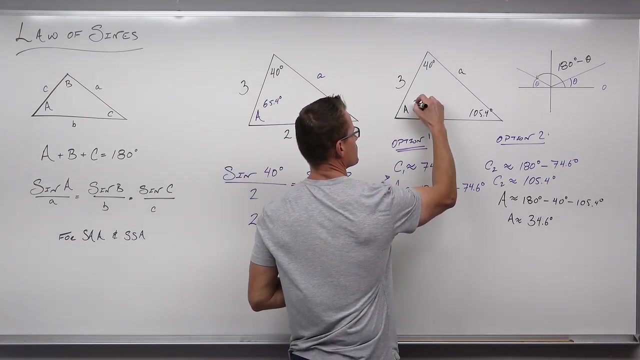 You just really really need to give two different angles, using 180 minus the angles. you find That's pretty important. So once we do that, if we haven't run into an impasse, this is right, This is right. They're both positive. I'm going to make this 34.6 degrees. 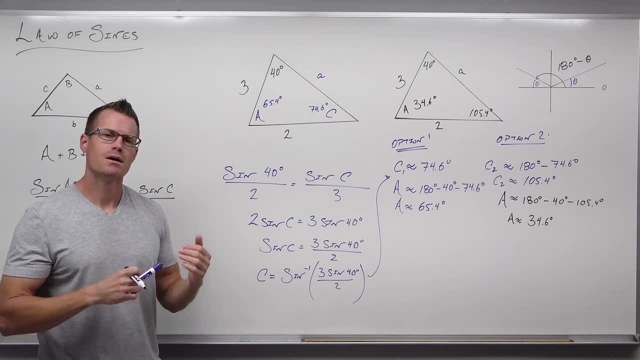 I'm going to make this 34.6 degrees. I'm going to make this 34.6 degrees And I'm going to make this 34.6 degrees. So what you're going to do is take sine of 40 over two. 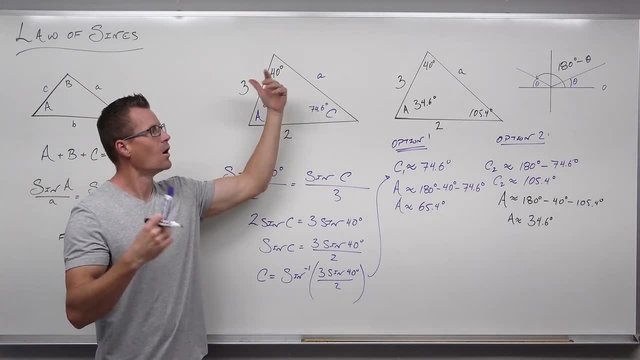 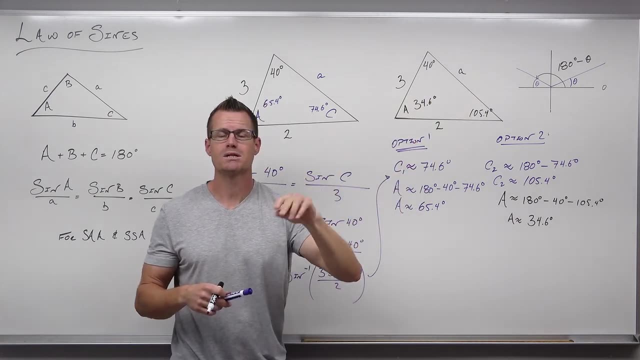 equals sine of 65.4 degrees over lowercase letter A. Or you can take sine of 40 over two equals sine of 34.6 degrees over lowercase letter A. It'll give you two options because there are two triangles: a shorter one and a larger one. This is exactly what's happening. 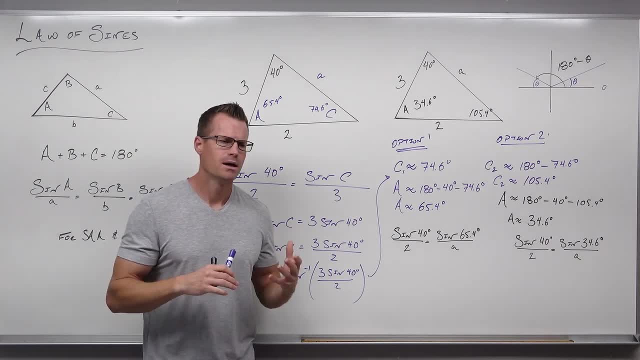 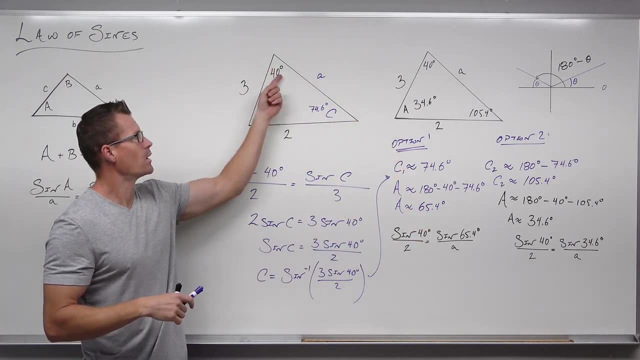 Okay, so I've drawn two triangles just to make it easier for my brain. You don't necessarily have to, but I think it's a really good idea. That way I can double check For option one, our first triangle I want to use, given information over using these rounded things. 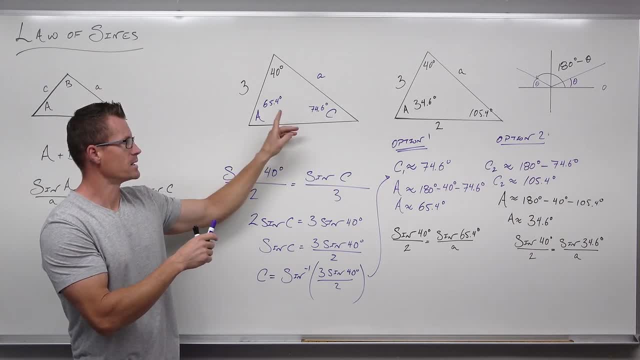 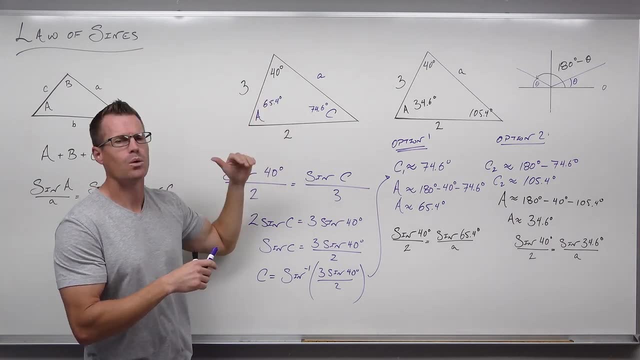 So I'm using sine 40 over two. I got it Equals sine 65.4 over eight. I can't avoid using this rounded thing, but I want to avoid using that one at the same time, So use only one if you can. 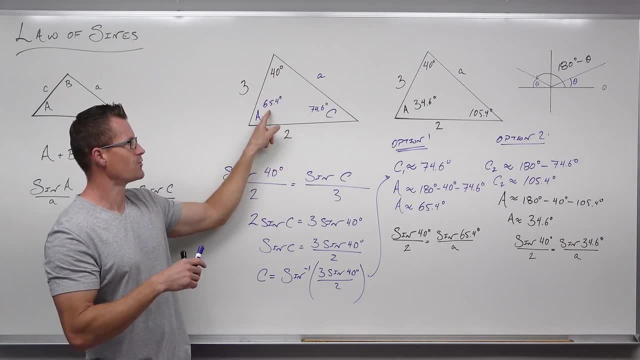 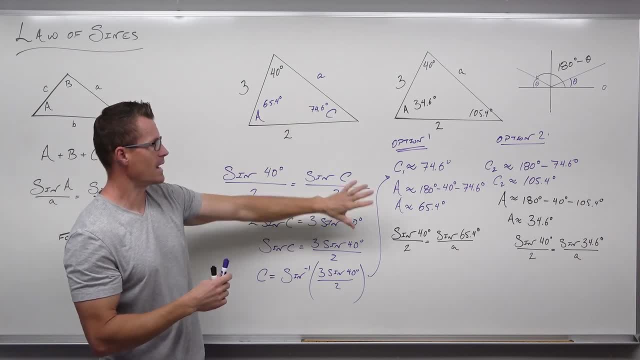 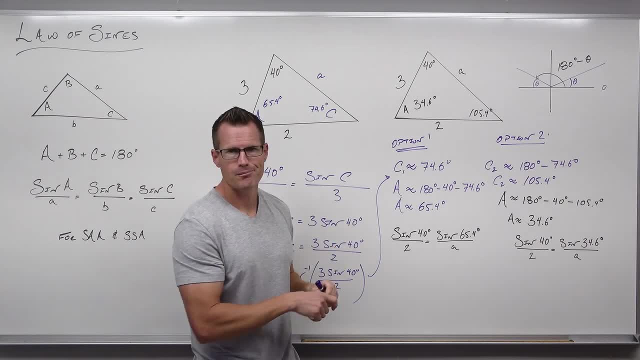 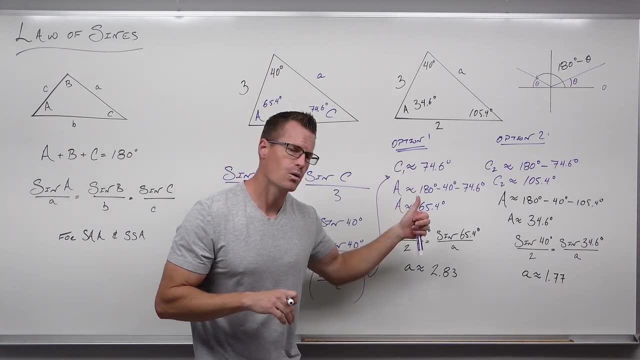 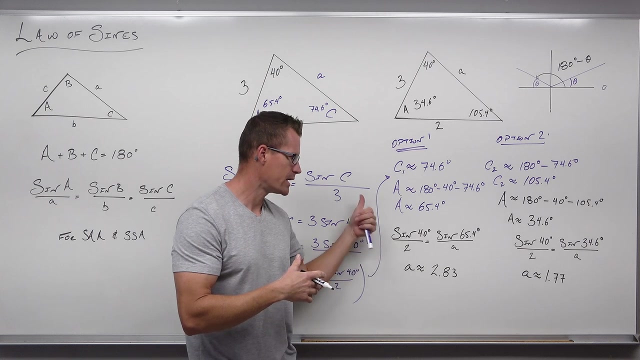 for the second option, my other missing side on my last or my option, two triangle. So A is about 2.83 or 1.77 for those two options. You should work both of those out on your own. We're just cross-multiplying, dividing and rounding. 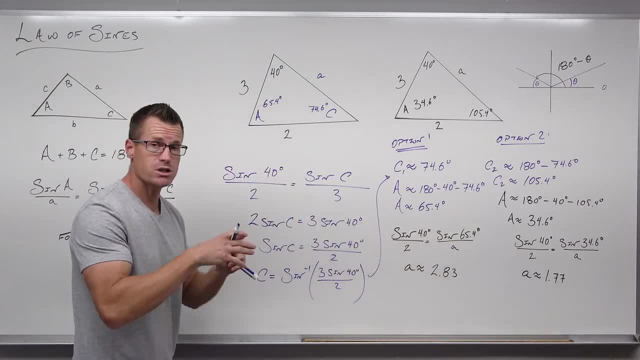 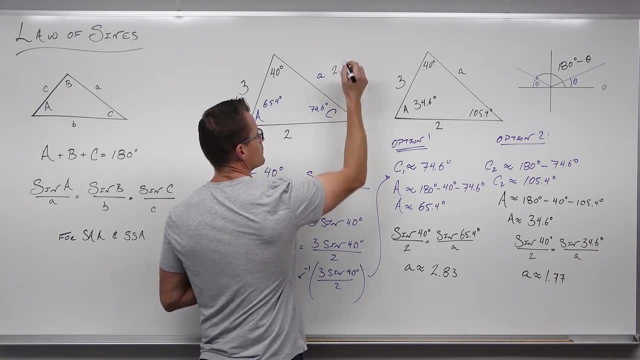 Cross-multiplying, dividing and rounding, And I'm going to put this up there just to make sure that larger angles are opening to larger sides. So 2.83 and 1.77.. I'm going to double check It. 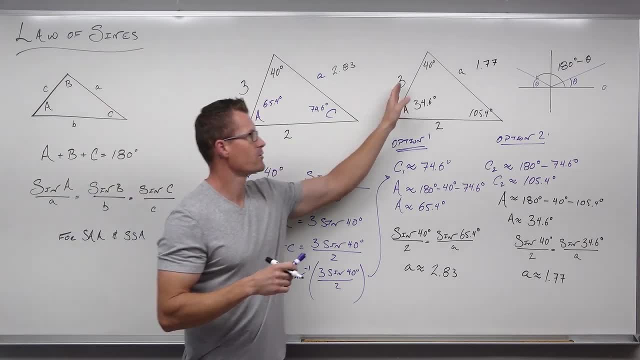 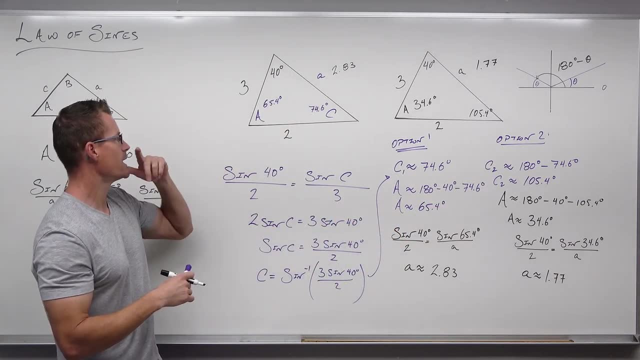 looks like: wow, all three of my angles add to 180.. All three of my angles add to 180.. I haven't broken the interior angle. So that's what tells you whether you have one option, two options or no options. It appears that, um, that my larger angles are opening. 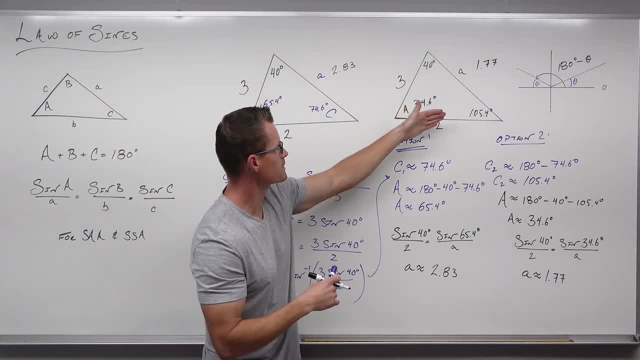 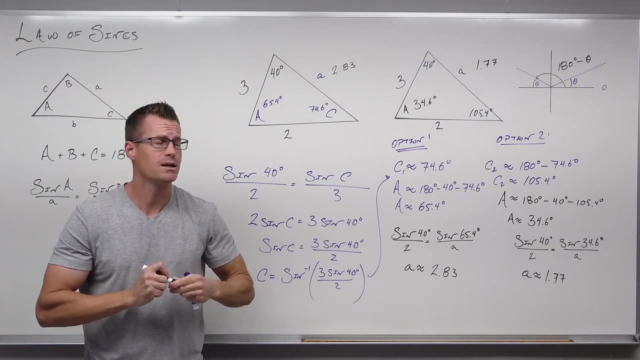 to my larger sides, Smaller angles of smaller sides. That looks really good. So I've used that to check my work, Not to tell me whether I've made a numerical mistake, but at least I haven't made a proportion mistake. I hope that makes sense. It's the hardest one, Understanding that when you find 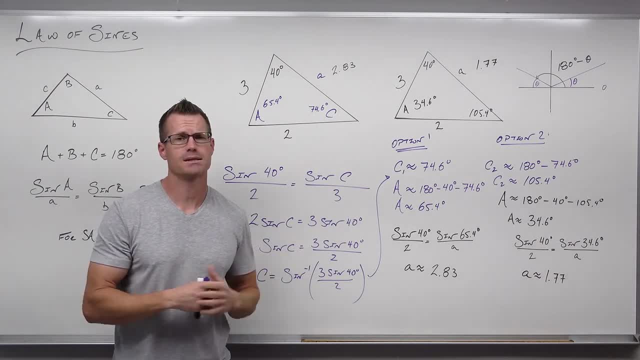 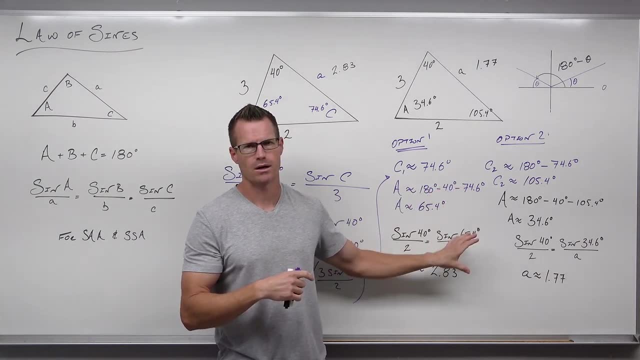 sine, you have two outcomes that will satisfy that sine of an angle. Then which one works, or if both of them works, is a matter of interior angle sum. So check that out. I hope that makes sense. I'm going to come back with one more example before an application about what happens. 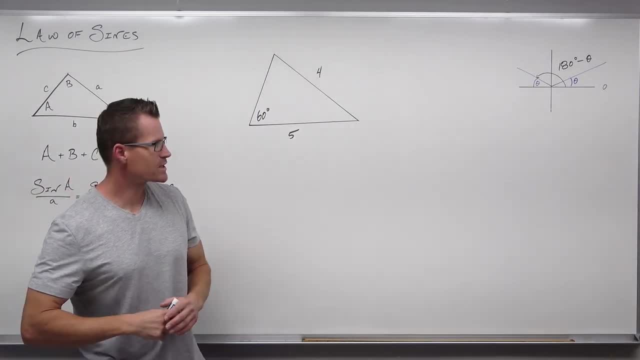 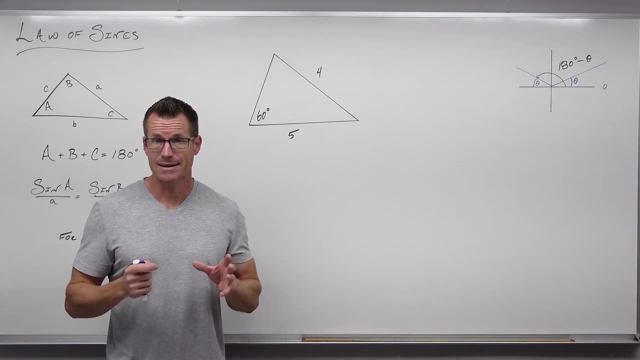 if you get no solution. All right, let's move on to another example. I know I already ruined the suspense for you and told you there is no solution, but let's see why that is. You're actually going to really like this case Once you understand it. you're going to really 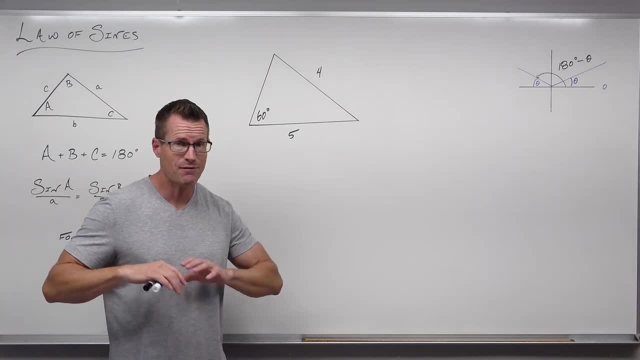 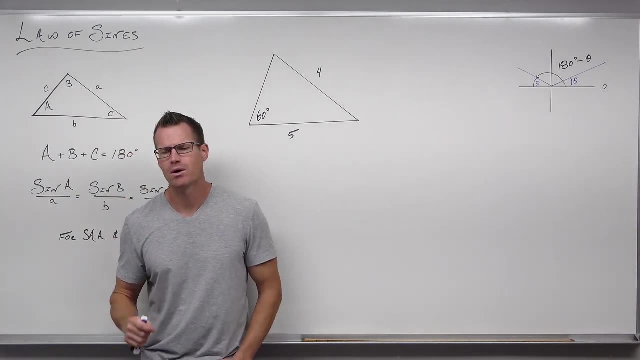 like this case. You're going to think: give me 30 of these because you don't have to do any more work with it. It's kind of nice. So let's go through the whole process. I'm going to model my thinking one more time just to make sure that you see this right, exactly how I want you to. 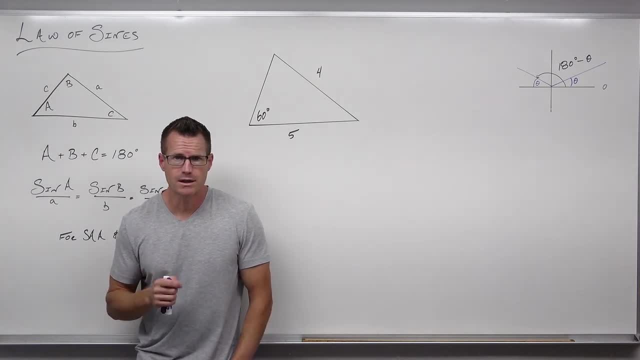 The first thing that we do is we see what works for what we're given. If we have a right triangle and you know it's a right triangle, then you're using right triangle trigonometry If you know that you have two angles. 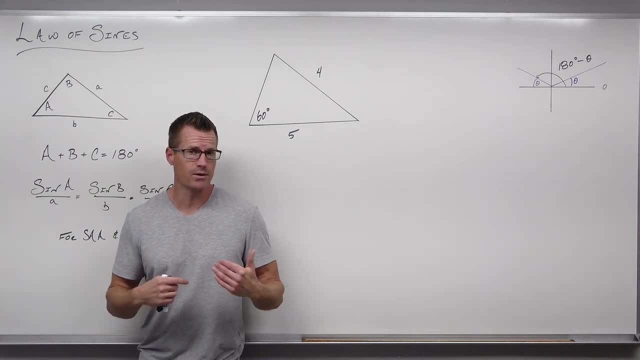 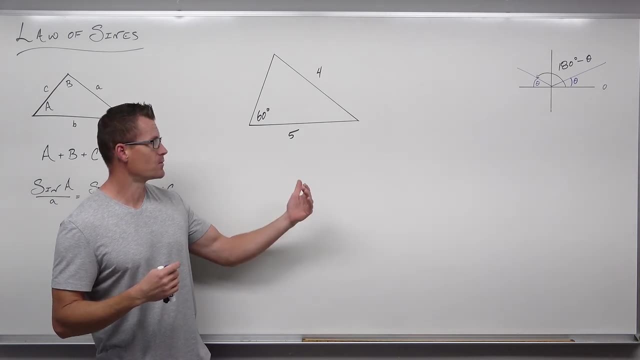 given you're using interior angle sum, We don't need to touch law of sines until that happens. So we're looking at this, thinking, yeah, it's not a right triangle. I'm thinking that's not right triangle. trigonometry: I'm seeing two sides and one. 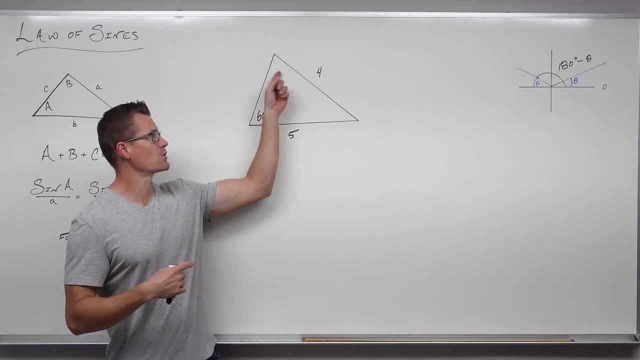 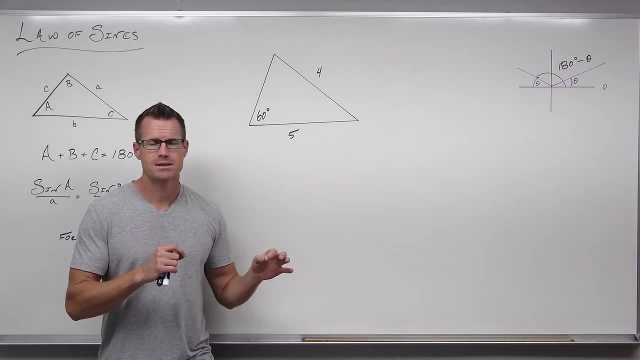 angle that I'm given. That means I can't use interior angle sum to find a third, So I'm really just left with the side-side angle and that means I'm using law of sines. If I would have had an angle here and not here, that would be law of cosines. It's the next thing we're going to talk. 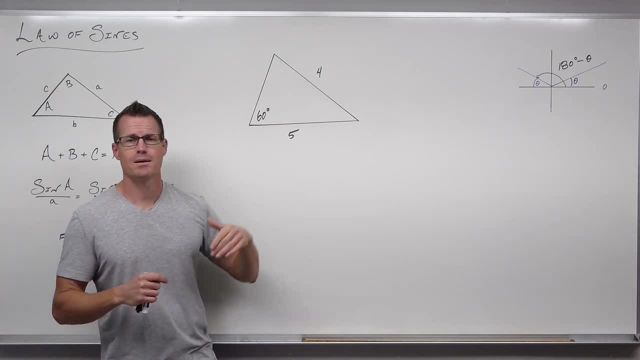 about. So I'm seeing side-side angle or angle side-side. I'm seeing two sides and angles, not between them. This is law of sines, So in my head I'm thinking that I might go ahead and label this. So if this is, let's say, B. 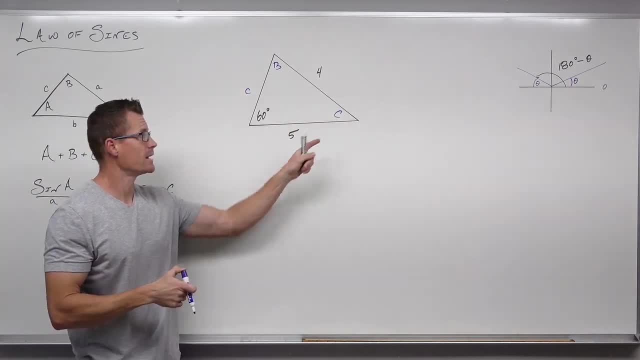 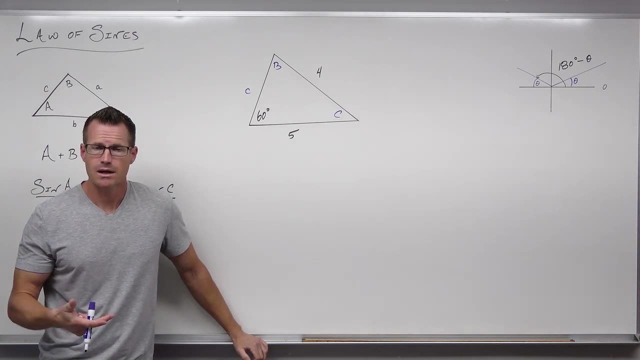 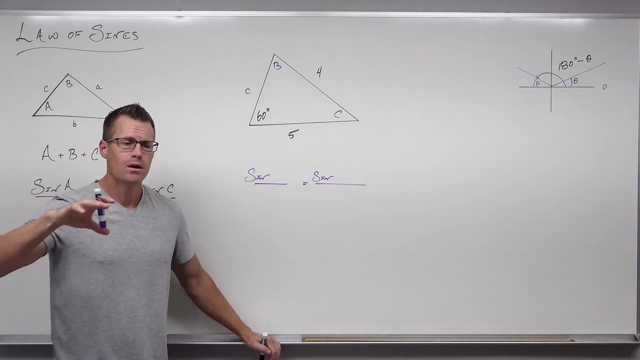 And C, then that would be side lowercase letter C opposite it. After that I'm really just focused on doing the law of sines. So I'm going to set up my proportion. Law of sines works by taking one proportion of things you already know. 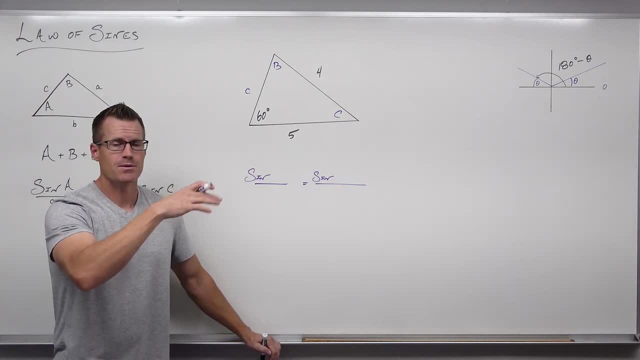 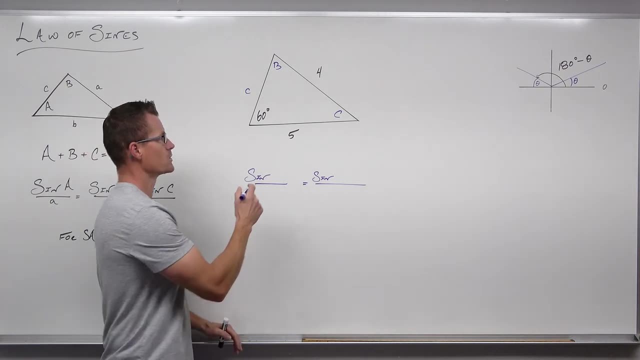 with a mixed proportion of one thing you know, one thing you don't. If you have two sides, that means that you're going to have sine of an angle that you know over sine of a side that you know. So 60 degrees. 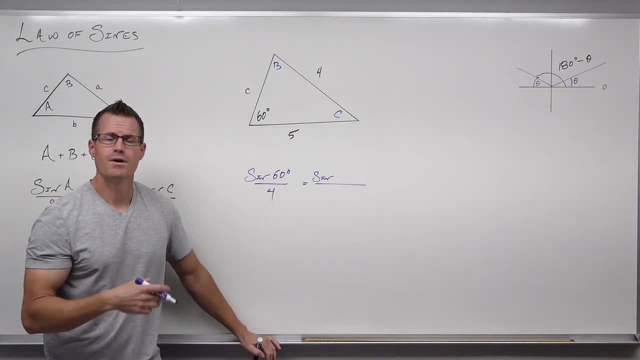 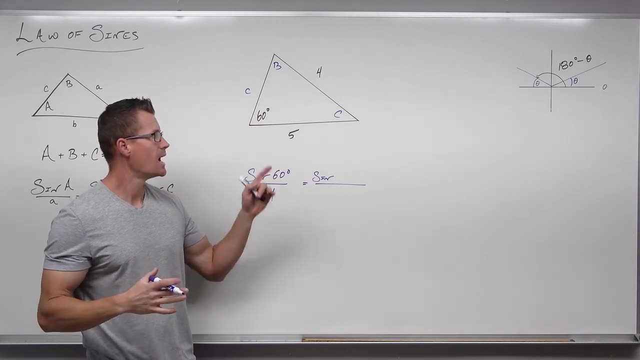 Over its opposite side, which would be four, equals sine of. I need to have one proportion of something that I actually know. I cannot do sine of C over C, because I know neither of those things. I have to choose sine of B over a side that I know. You need to know three things to 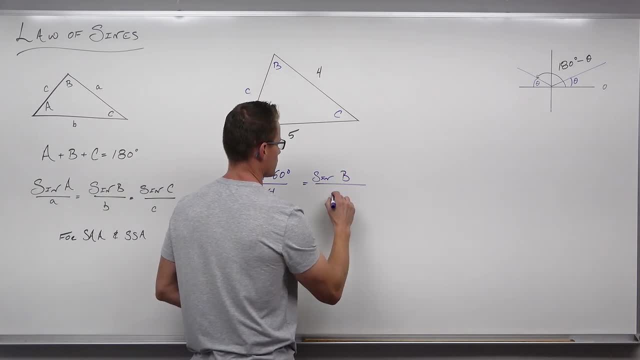 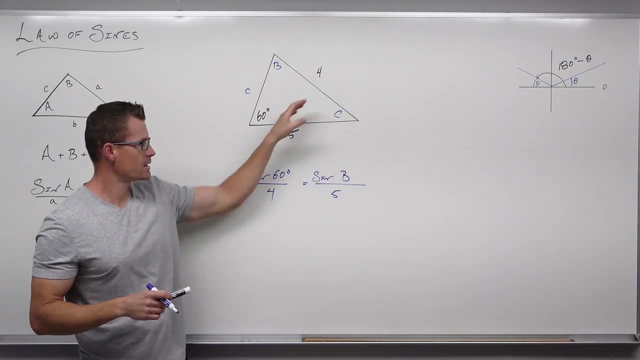 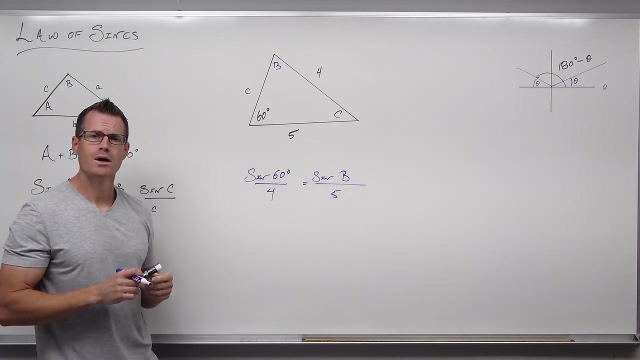 find a fourth And that works. I'm going to double check. Sine of 60 degrees over a side that's opposite it, those are both known. equals sine of B over a side that is known, That's an opposite side and it's a side that's known. So I know three things I'm going to find. 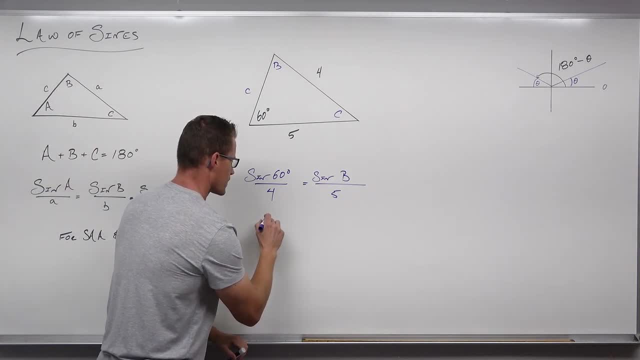 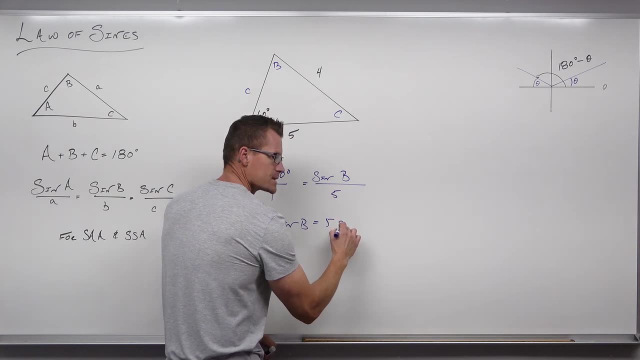 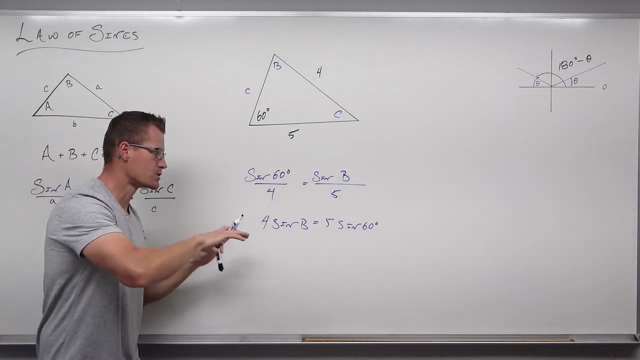 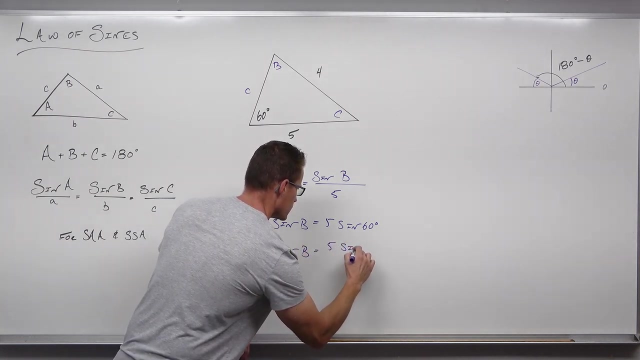 that. fourth, If we cross multiply, we get four times sine B, equals five times sine 60 degrees. Now we're going to solve for angle B. So let's divide by four, Let's do that, And then we're going to take sine inverse. I want you to notice something. 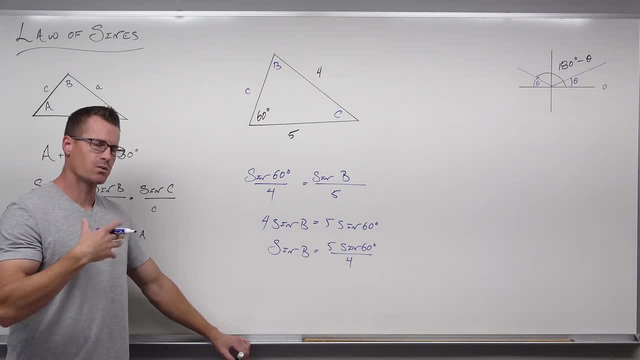 This is precisely what we've done for the last two examples. We noticed it wasn't a right triangle. We labeled stuff. We saw we had two sides and one angle that's not between them. So we chose law of signs, We set up a proportion and then we solved. We solved for that angle In the first. 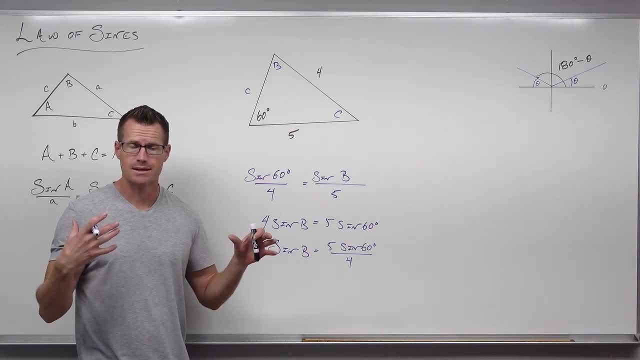 case, we had one option that worked and one option that didn't. In the second case, we had both options that worked and we had to form two triangles and solve them. And in this case, let's let's try to solve for angle B. We're still going to use sine inverse. It's still the same process. 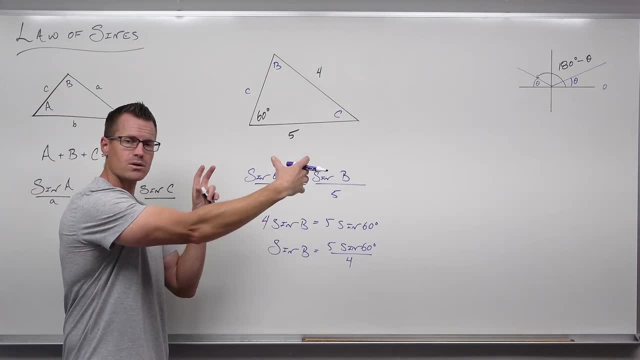 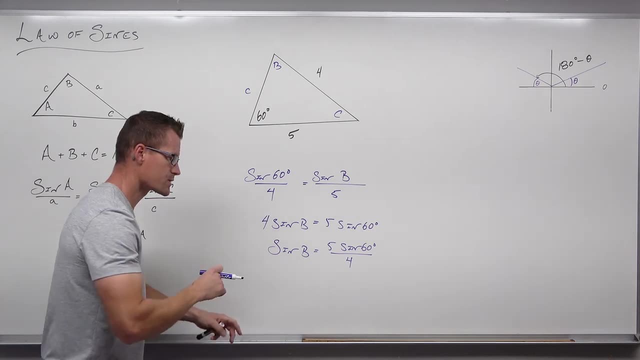 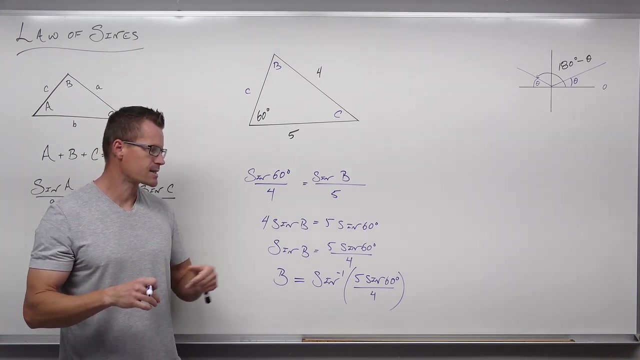 It's what happens next that determines what you do. Do you have two angles that both work, Two triangles? If you have one angle that works, one triangle. If you have no angles that work no triangles, So let's find angle B, And so we have this sine inverse of 5, sine 60 degrees over. 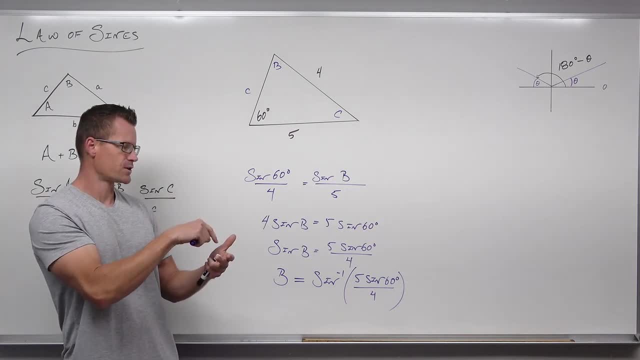 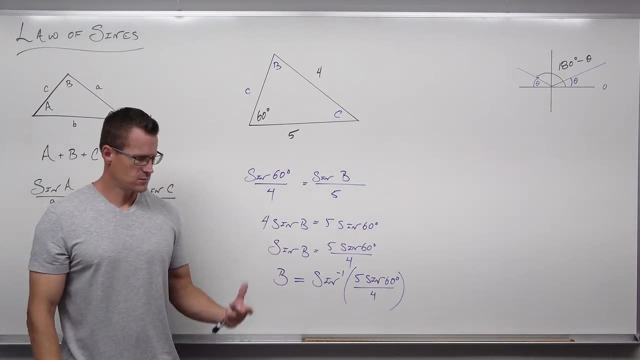 4.. And so you take your calculator out and you plug it in and you go sine inverse and you do your parentheses 5, sine 60, end parentheses, divide it by 4, and it goes. error You go. what do you mean? error, you stupid calculator. Why are you giving me error? It's because this: 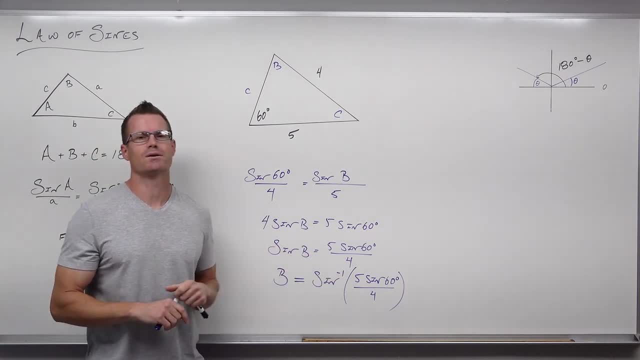 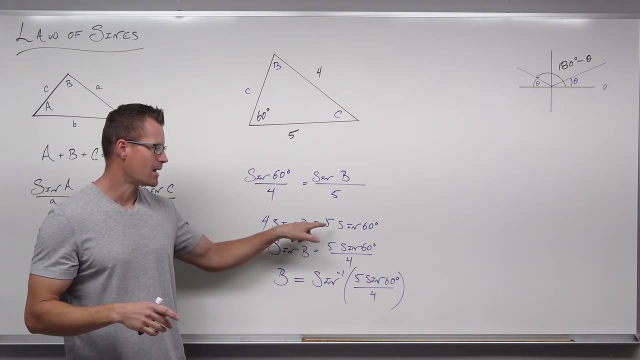 isn't possible. So if you get error here, you done. Why? But why are you done? I want you to go back one step. I want you to go back one step and figure out what this is. Do it on your own. 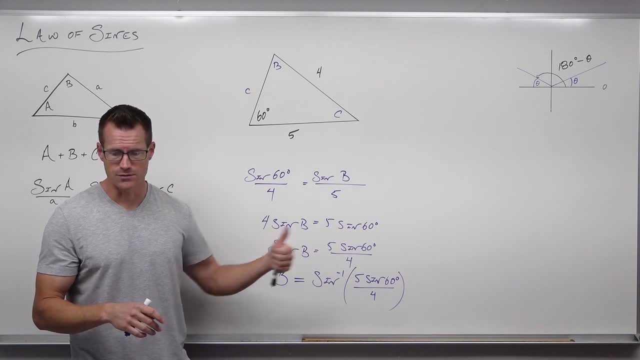 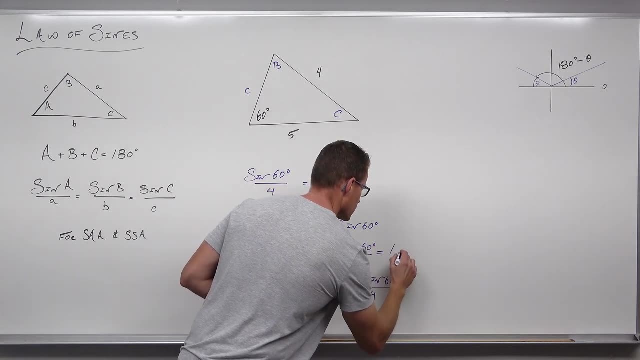 right now: Do 5 times sine 60,, end parentheses, divide by 4. And it gives you 1.0.. 0.082, something, something, something, 1.08, something. Now think: oh man, I hope you. 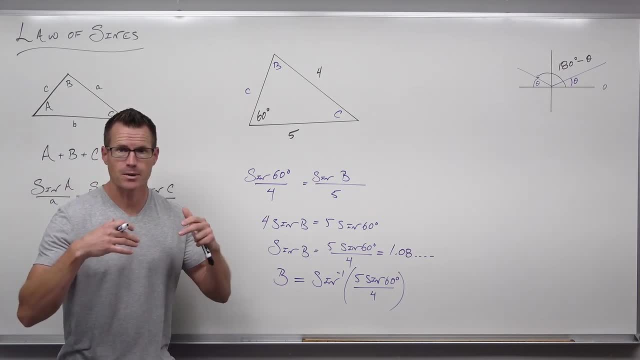 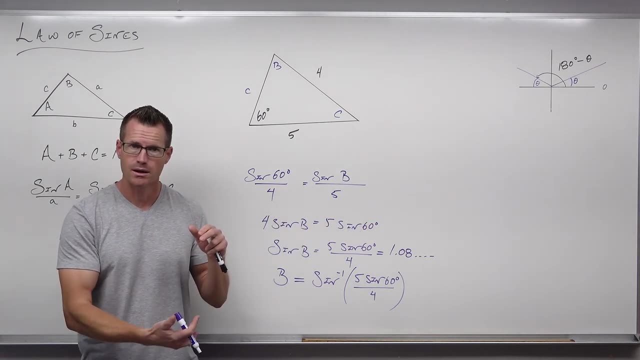 remember What is the range of sine. Like you plug in anything, The domain of sine is all real numbers. You plug in anything you want, But what's the range of sine? The range of sine is negative, 1 to 1.. And since we're only focused on 0 to 180 degrees, the range of this particular sine 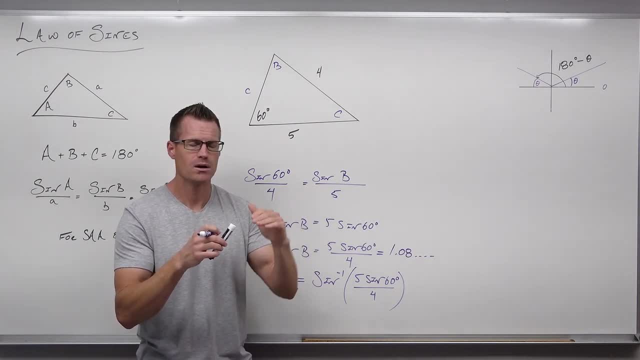 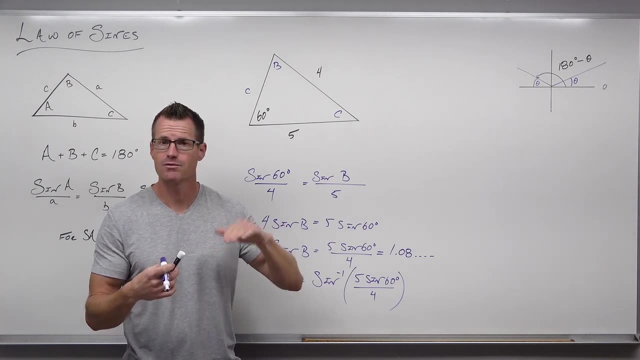 because we can't have negatives who are, are are sine values. here is just 0 to 1.. You will not get out anything if you plug in a number to sine besides negative: 1 to 1, in our case, 0 to 1.. So wait a second, And that that, by the way. 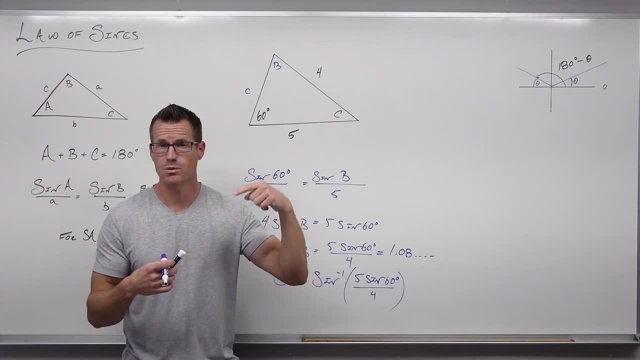 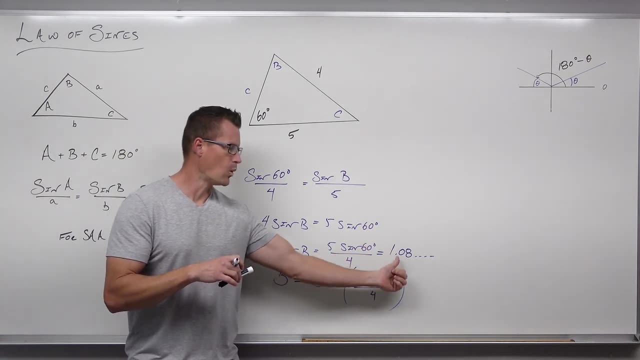 is because we don't have negative angles and all of our angles are between 0 and 180.. So you can only get out 0 to 1.. So look what's happening. This says sine of your angle is 1.08.. When you 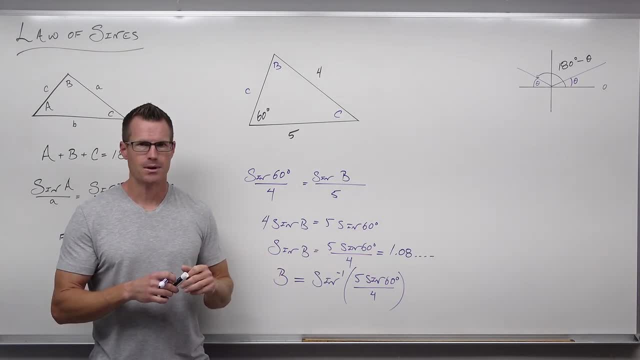 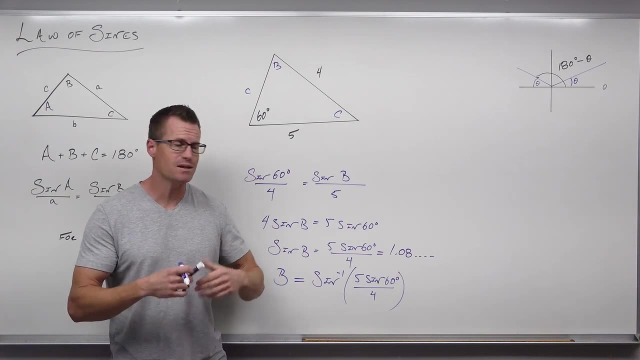 plug in this angle. sine of this angle is over 1.. That can't happen. Sine can give you a maximum of 1.. So this is breaking the range. This is not possible for sine to even give you. So this angle is impossible. There is no angle You can plug in. 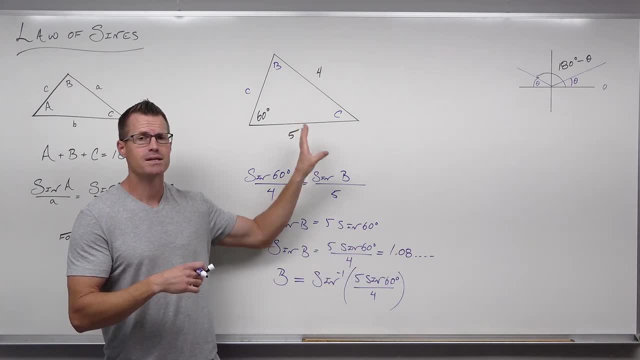 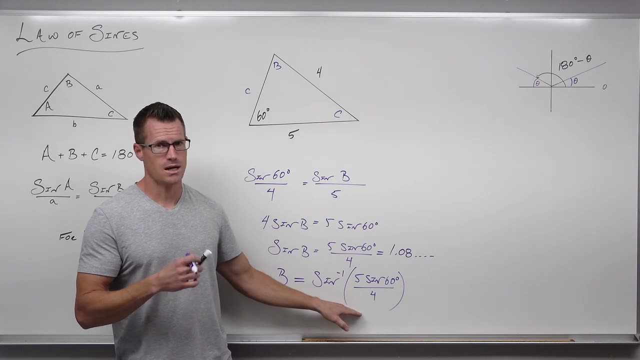 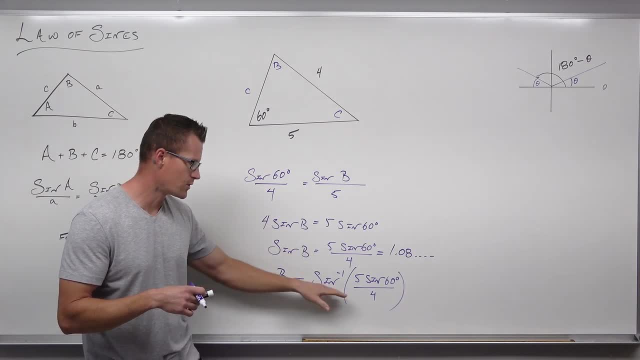 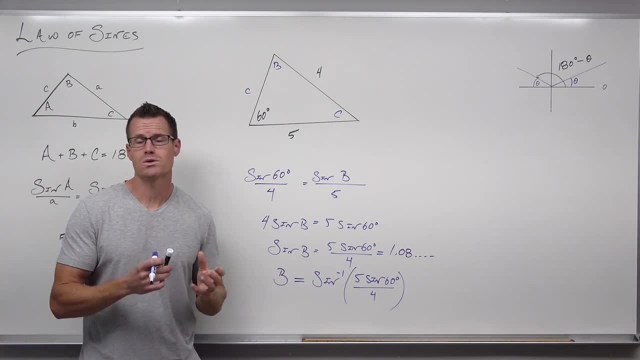 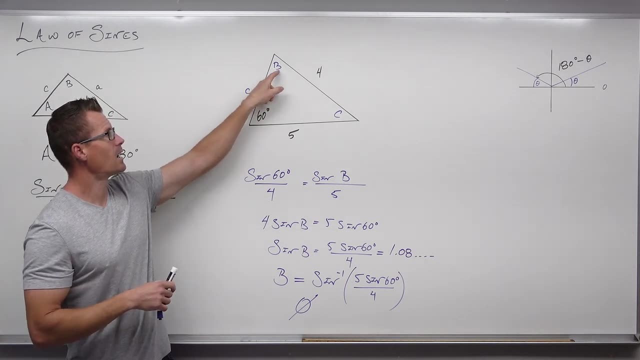 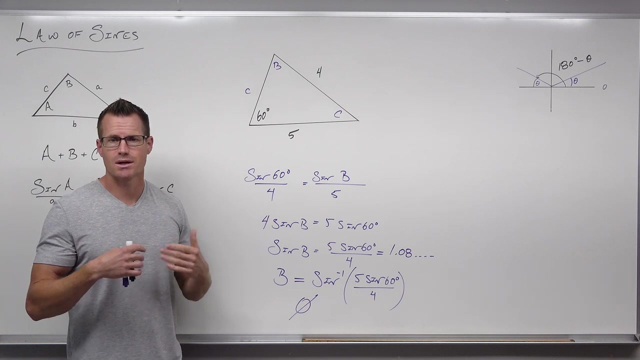 That means that this angle is impossible. There is no solution here. So what that says is that, no matter what you do, you cannot put an angle here that makes this triangle possible. It's not possible to do, And so we have a no solution. This is the case for side-side angle that none's. 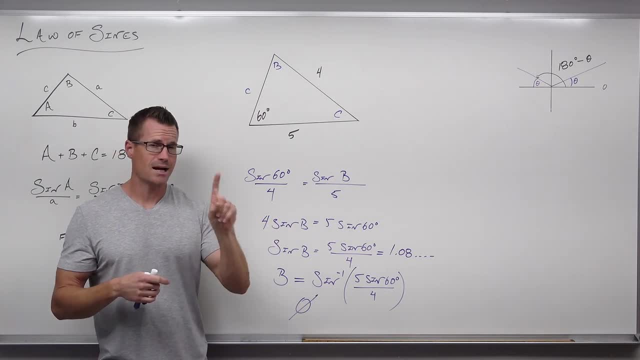 possible. So I've given you no triangle, I've given you exactly one triangle and I've given you two triangles are possible. What about the exactly one- 90 degrees- that will show up in the one triangle case? So that'll show up as: oh yes, you have just one possible And it turns out the other. 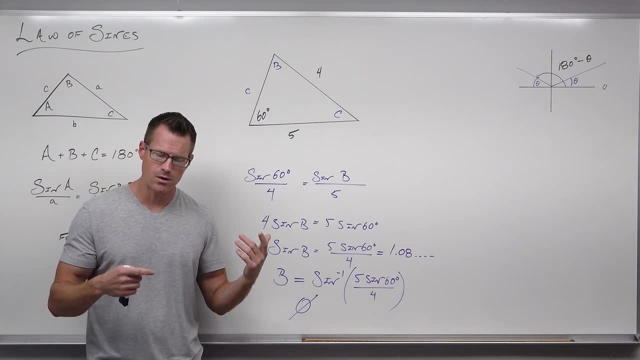 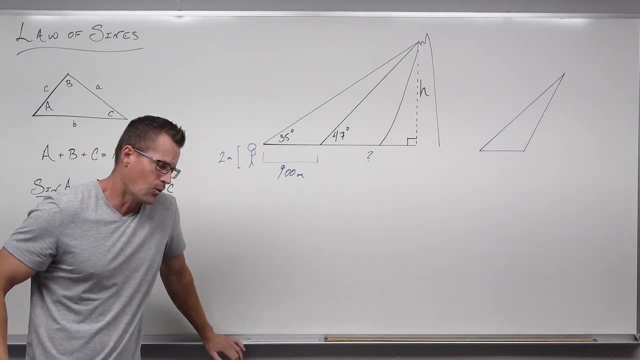 angle is 90 degrees, So that'll work there as well. So we're going to do now- hopefully that makes sense- We're going to come back with one application and then be done. Okay, Last one. So a lot of times. 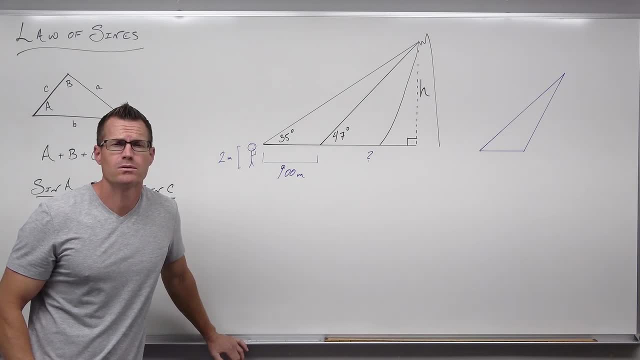 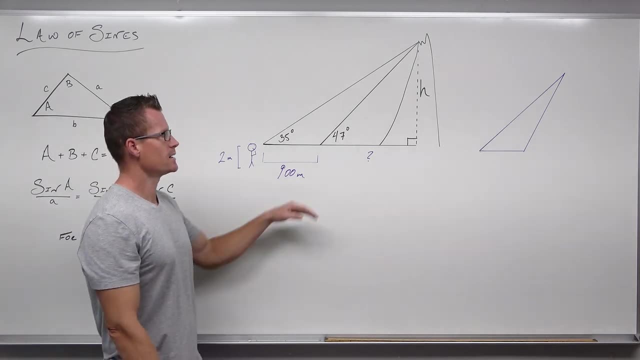 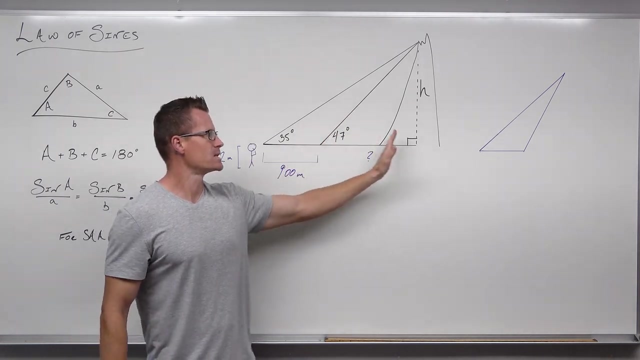 you're given this type of a problem in a right triangle trigonometry section. I actually gave you one in a video that said: suppose that you are standing a certain distance away from, let's call it, a volcano and you measure 47 degrees. Yay, And I am a certain distance away from the center. 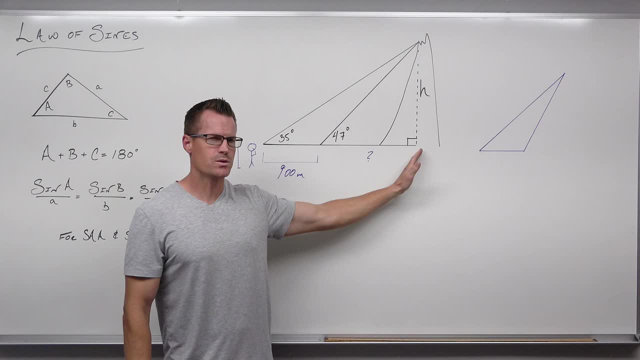 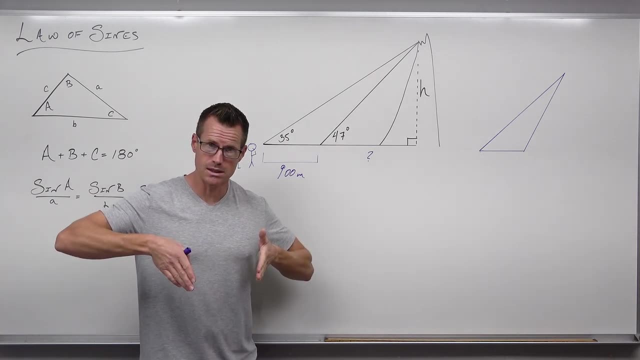 of that volcano. How in the world are you supposed to know how far away you are from the center of volcano? I said maybe you look at like the Google earth thing and you you measure out, like did it distance wise- how far you are. but that takes a lot of technology to do that. So what if you're? 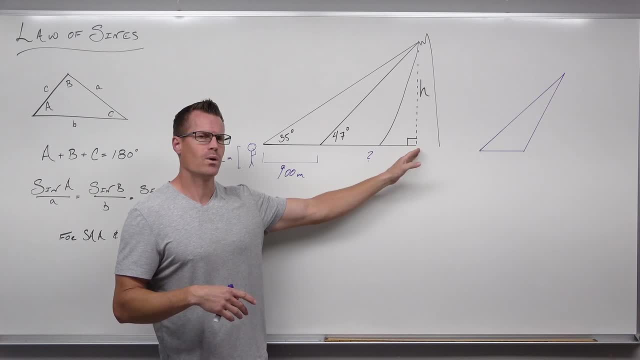 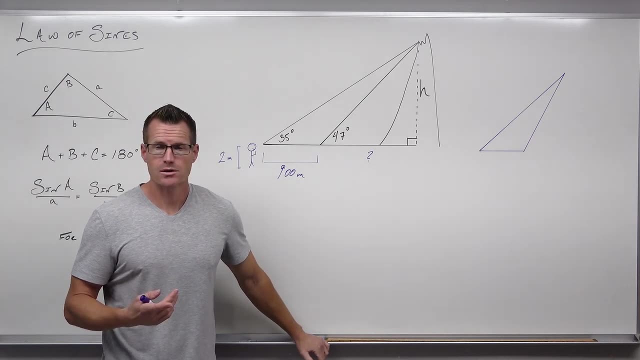 not able to do that? What if you have no idea how far away this is from where you're standing? Could you still figure out an approximation for the height answers? Yeah, So suppose you did this. suppose that you stood at this point. you don't know how far away this is. 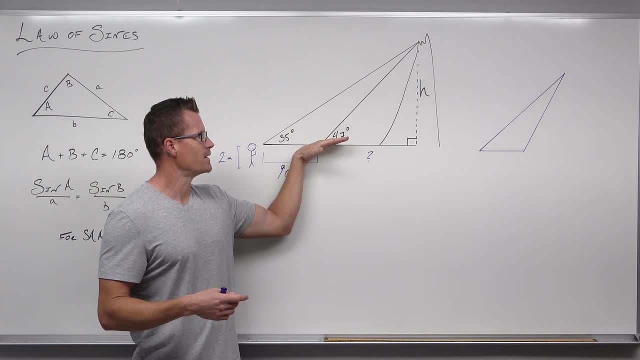 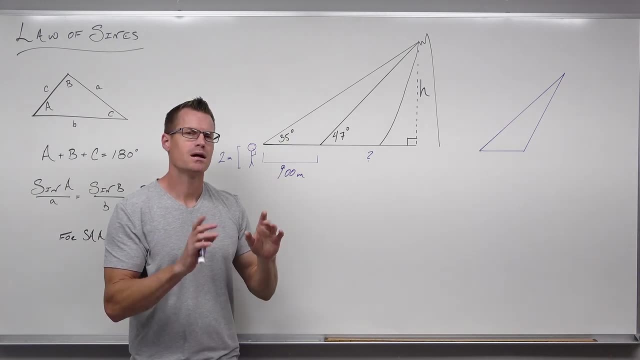 but you measure by looking up maybe a clinometer or something like that, that this is 47 degrees, that you're looking up at the top of this angle elevation, top of the volcano is 47 degrees. You say, Hey, there's something I can do, though, without knowing this distance. 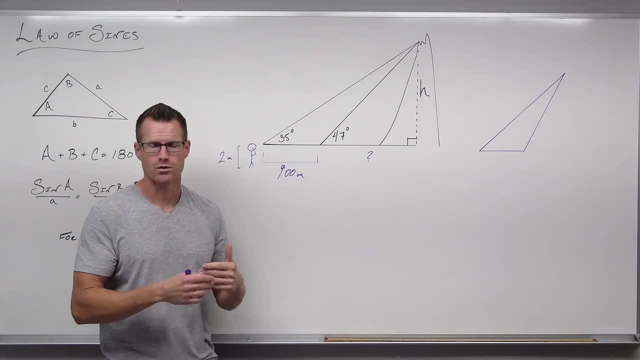 but knowing that I can stand back a certain distance further- 900 feet, 900 meters, whatever- this is 900 meters in this case- and measure the angle again. Now, that's physically possible to do. You could stand at one location, measure, stand a known distance away and measure. 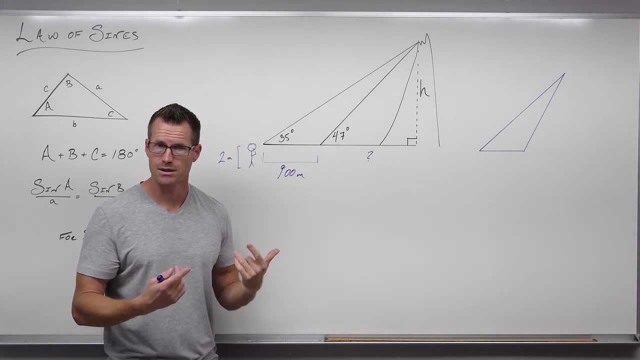 that angle again and find out the height of this, this object. So we're going to. it's a two-step process. Here's what we're going to do: We're going to use this information to figure out what we're going to do. We're going to use this information to figure out what we're going to do. 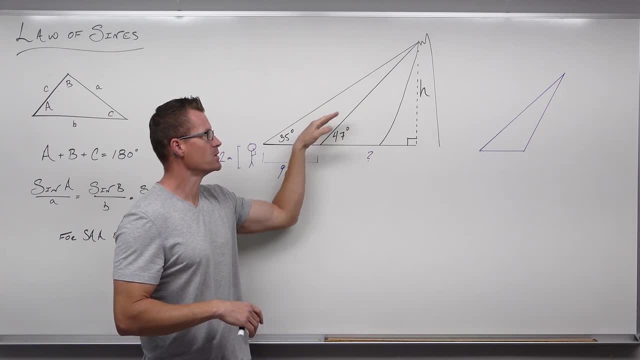 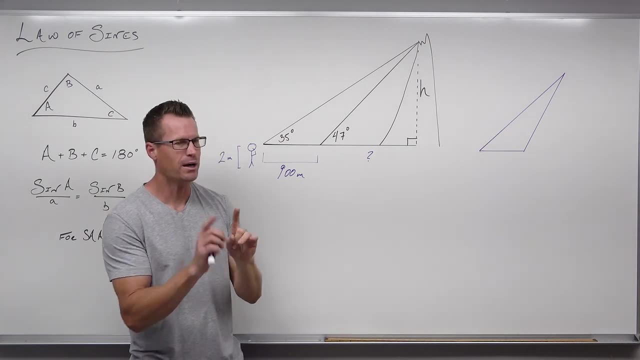 One of these distances and then use a right triangle to figure out the height. that is going to be possible to do with some right triangle trigonometry, but we'd have to know one of these sites first. So let's think about how we can do that. What do we know so far? 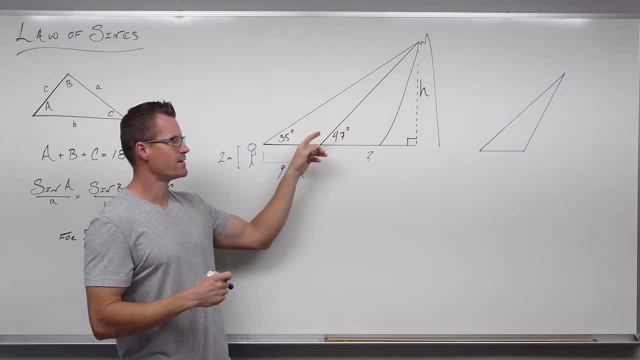 We know that this angle is 35.. We know that this angle is 47.. We know that this is 900.. That's all we know. However, if we think about just this triangle, could you find that angle? Yeah, because that's a. that's a straight angle, That's a. 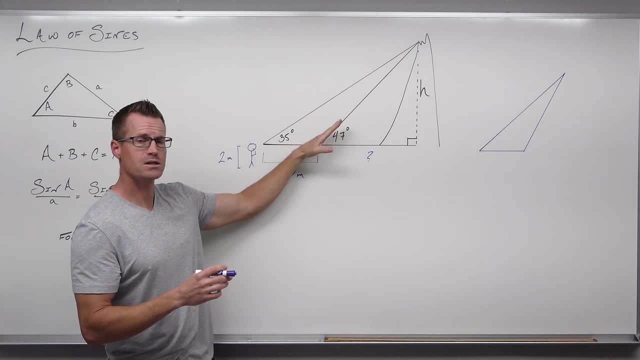 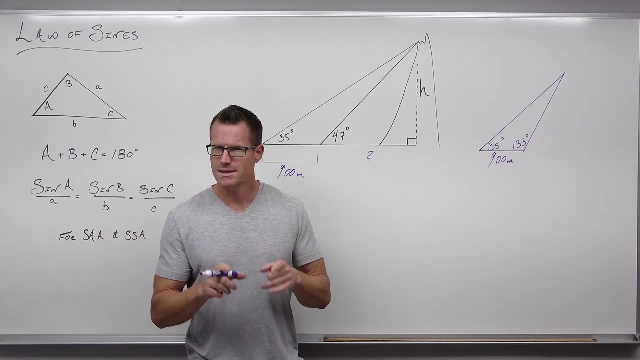 180 degrees. This would be 180 minus 47 degrees. We'll leave you with 133 degrees. Now we're left with that triangle. What does that triangle tell you? Well, you know two angles and a side. that is law of signs. So let's go through the two angles and one side that we have used before. 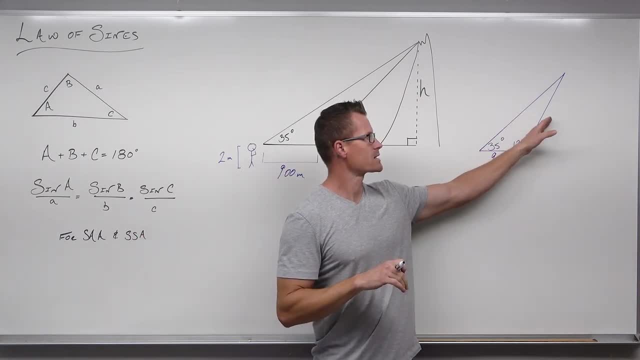 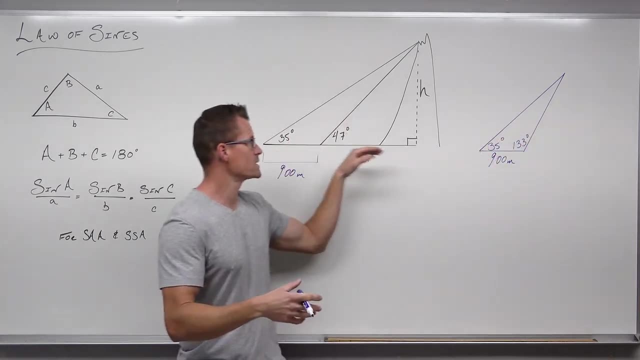 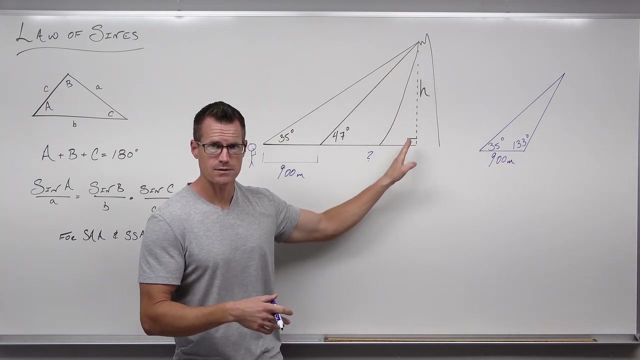 And a couple of examples- the first two examples, to figure out either this side or the side. which one it, it doesn't matter. If you figure out This side, then in a moment we'll be using a right triangle, One side known, one angle known, and you can use sign to figure out the height, If you choose to. 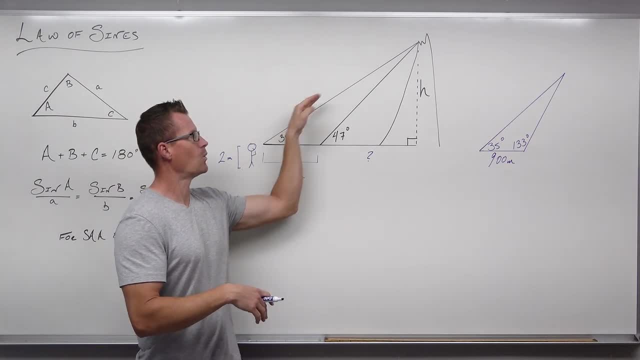 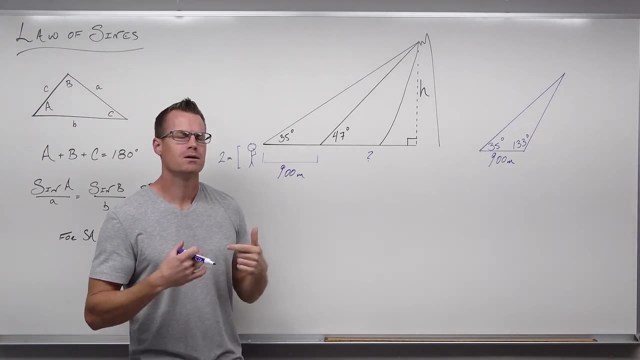 find this side, which I'm going to do. you have one angle known, one side known and you can use that to figure out your height. either way actually works, But the important point here is that you know two angles and you know one side. you're thinking law of signs. 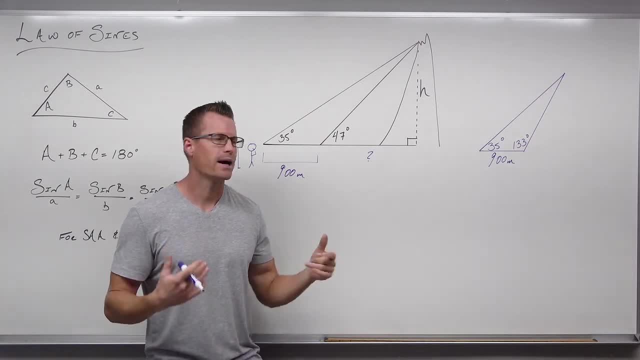 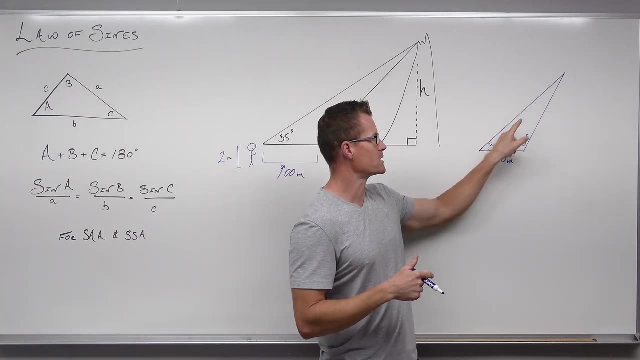 And when we have two angles, before we even use our law of signs, let's find this missing angle, As we did every time. Hopefully you remember the first two examples. You'd have to find this angle. Why? Because this angle relates to the 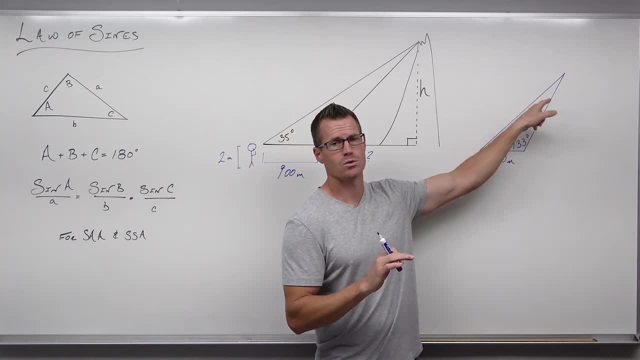 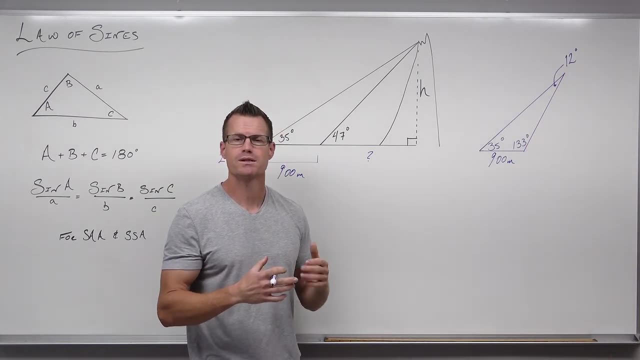 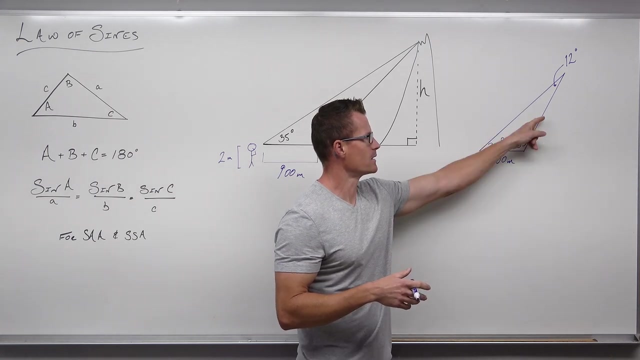 only known side that's opposite to it, That's going to be 12 degrees. So 180 minus 35 minus 133 gives us 12 degrees. Because we know that let's label some other pieces to this. Maybe that's: um, that's angle a and little a. this is angle C and little C. this is: 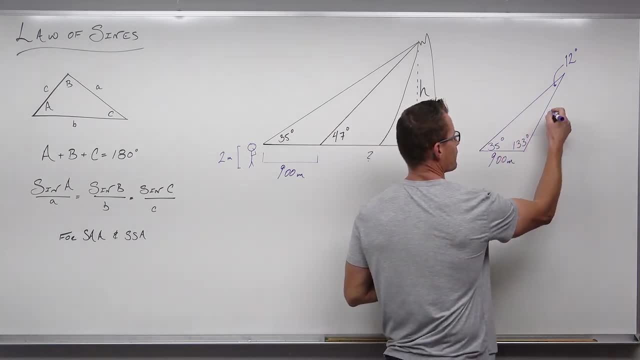 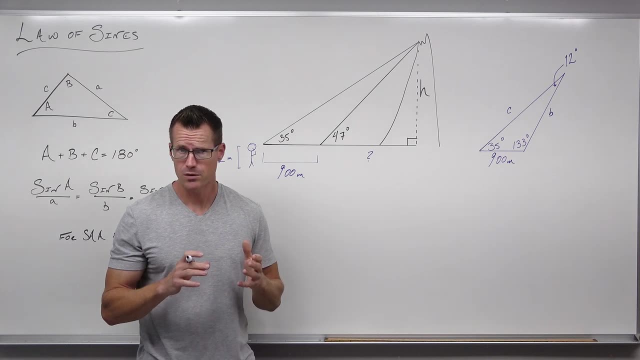 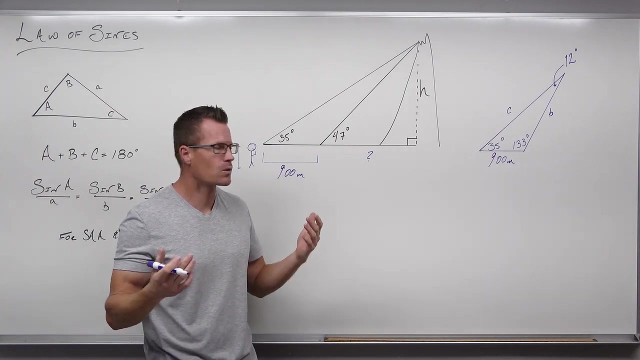 Angle 12. And nine hundred and seventy- we don't need letters for that, And you have your choice. I'm not asking you to find both of those missing sides, really just one of them, because it's all it's gonna take to find the height. I'm gonna choose to find lowercase letter C as a. 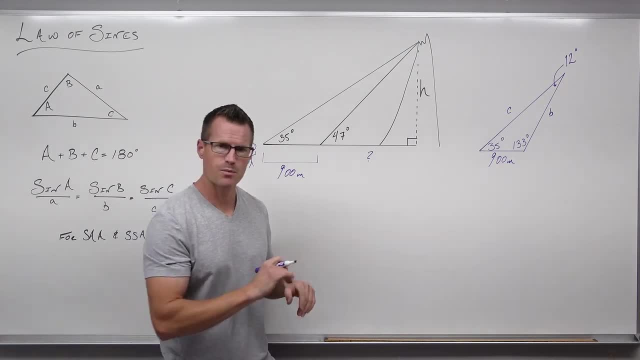 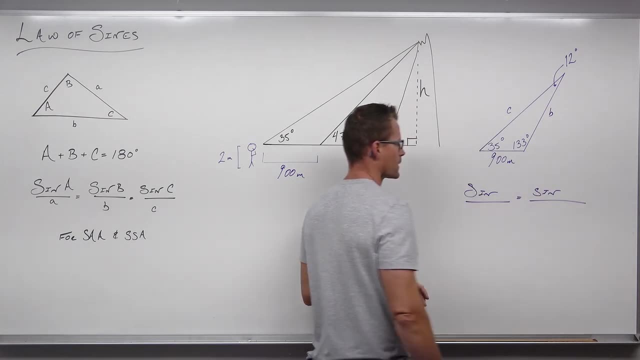 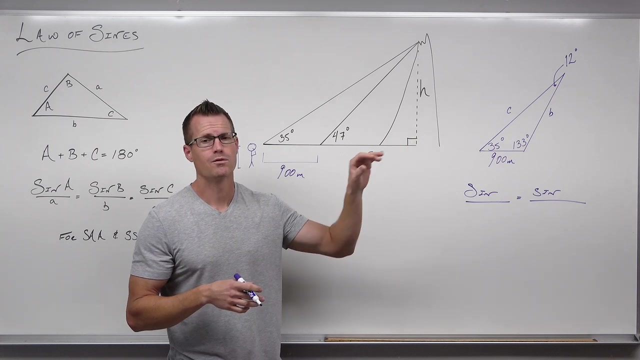 side. So, because we know that this is Law of Sines, let's set a proportion up. What Law of Sines does for the last time is: takes sine of angle over opposite side equals sine of any other angle over its opposite side. Now you do have to use a. 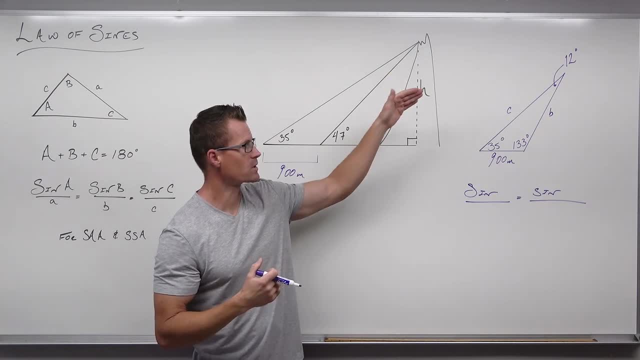 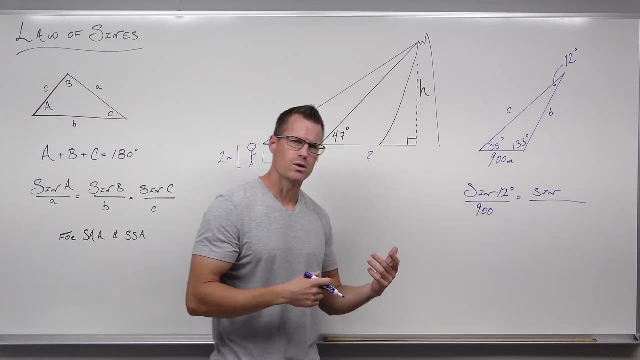 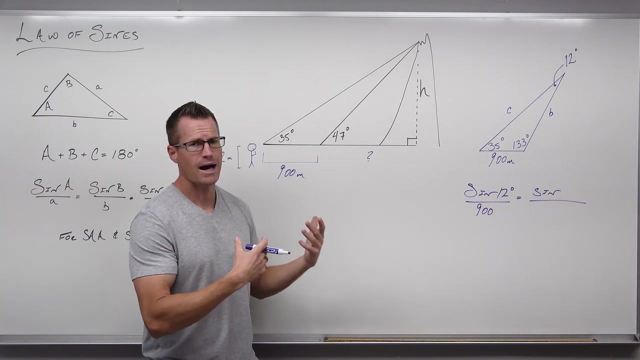 known proportion. so I need to use sine of 12 degrees over 900.. That's why it's so important to use the interior angle sum before you do Law of Sines with the angle. side angle is because you have to have a known proportion. Equals sine of. 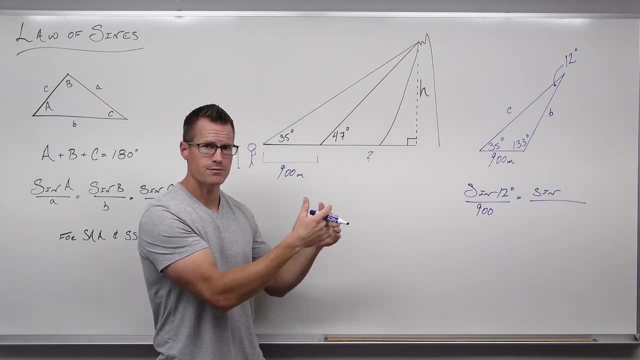 another angle over its opposite side. That's why it's so important to use the another known angle. Remember you will know all three if you have two angles in one side, So a sine of another angle over the side you want to find, In this case I. 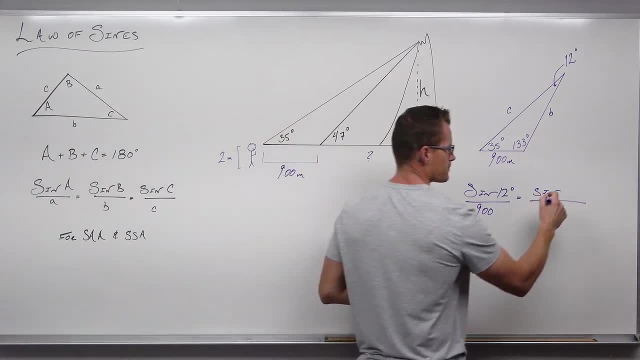 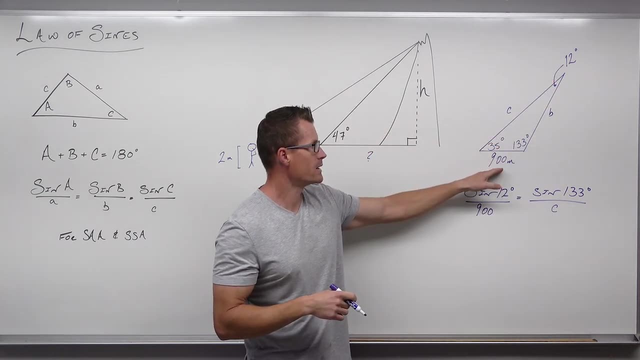 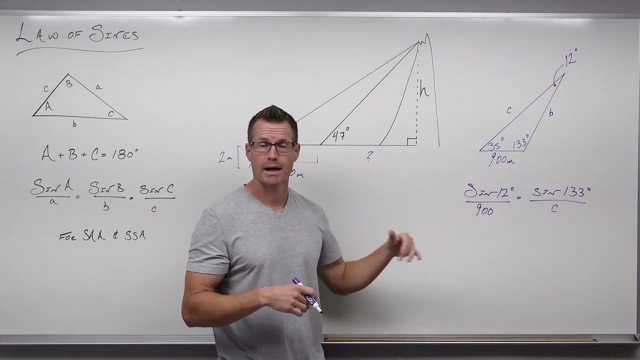 want to find side C. You do with either one. I want C. I'm gonna double check: Angle, I know over side. I know it's opposite Angle, I know over side. I want to find that's opposite Looks good to me. We're gonna cross, multiply and we're 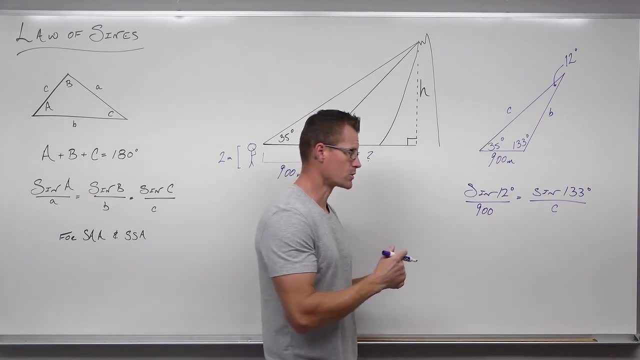 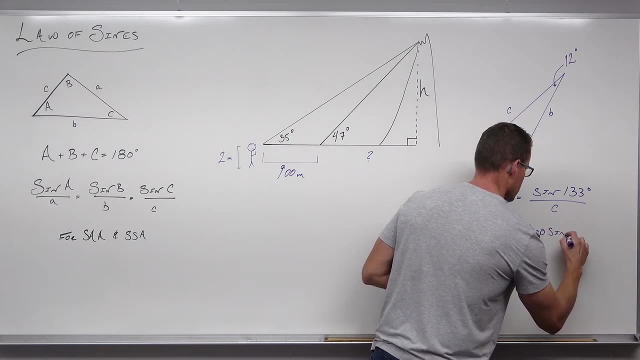 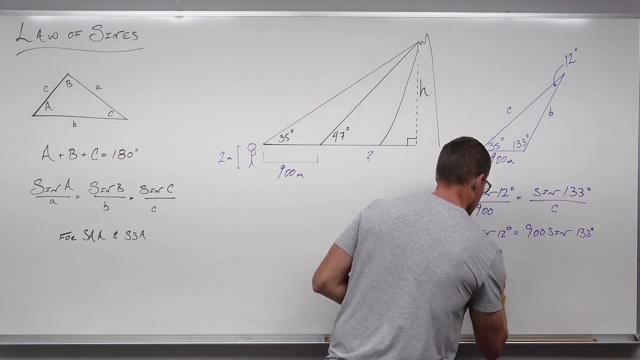 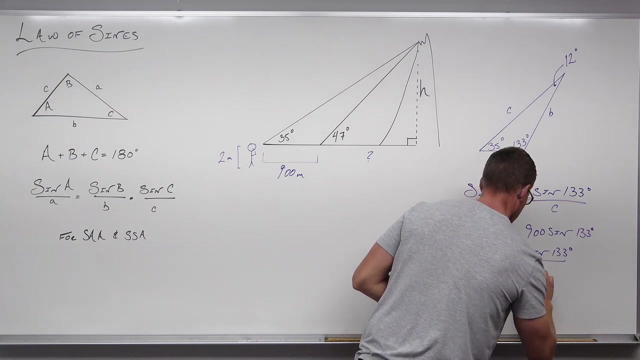 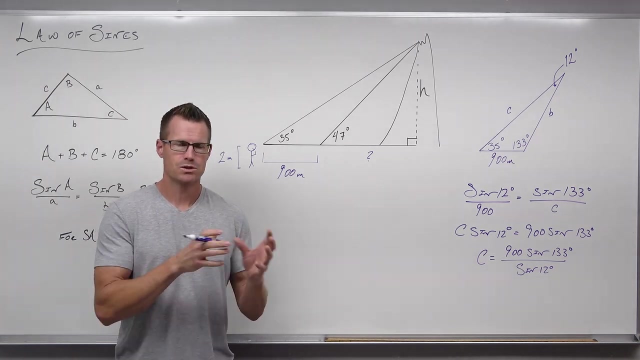 gonna divide, We're gonna end up getting C times sine 12 degrees Equals 900 sine 133.. If we divide by sine 12, we get 900 sine 133 degrees over sine 12 degrees. There's no two-axis. There's no two-axis. 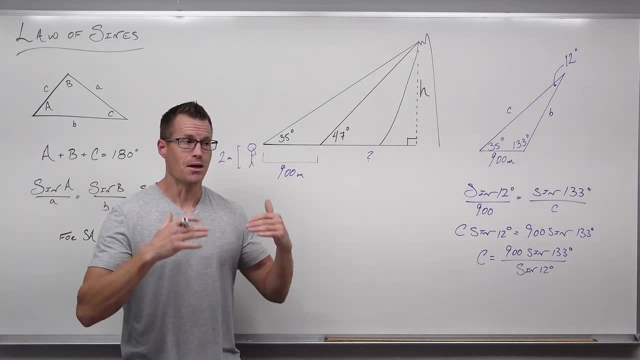 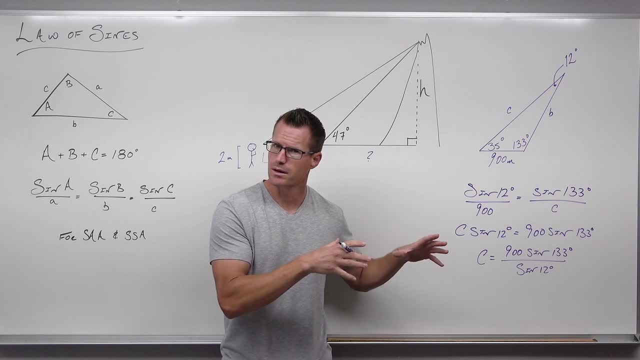 approximate it, we round it and there comes the error in it, And it's okay. It's a little more usable For our Pythagorean theorem. we're gonna actually have to use that rounded number. So we try to avoid rounding any time we can This. 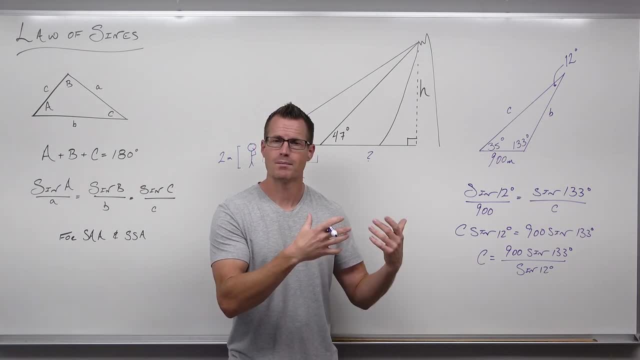 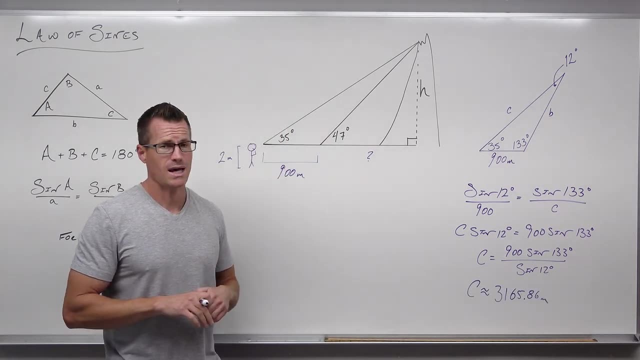 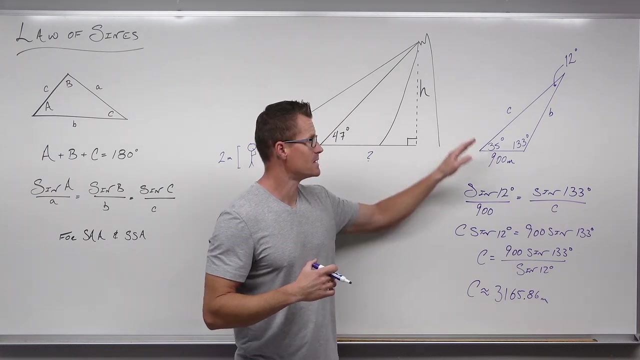 would be exact, But to use it later on to make our math a little bit nicer, easier, We're going to round this and say that this is about 3,165.86 meters. Now what did we just find? This is why we drew the triangle the way we did, so we could identify that this is this side, right here. 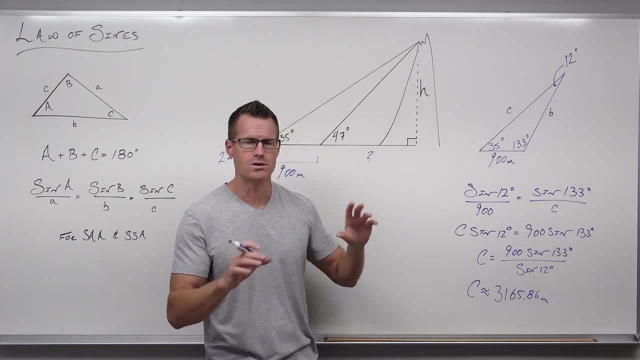 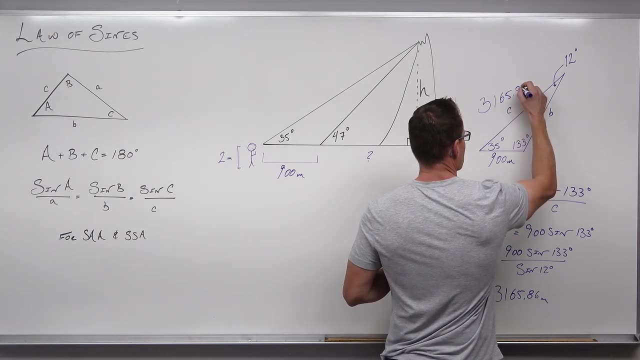 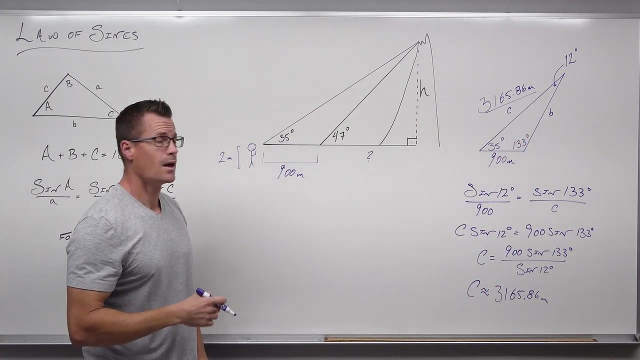 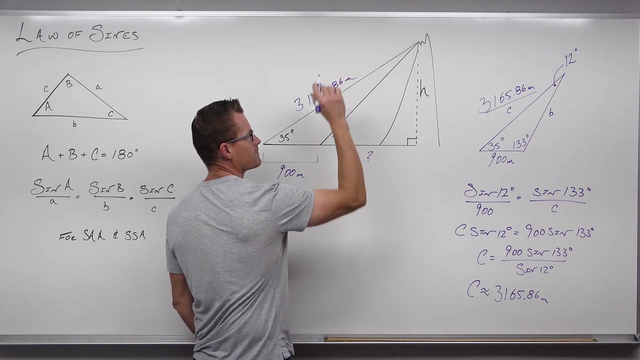 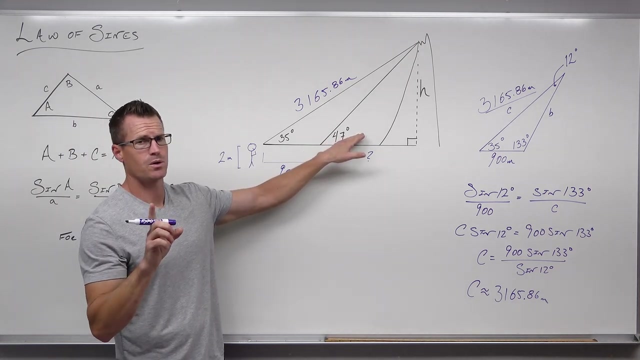 So that's 3,165.86 meters approximately. That also means that this side is 3,165.86 meters And we're almost done. You see, now that we know this, we used 47 degrees for only one purpose really: to find that angle. 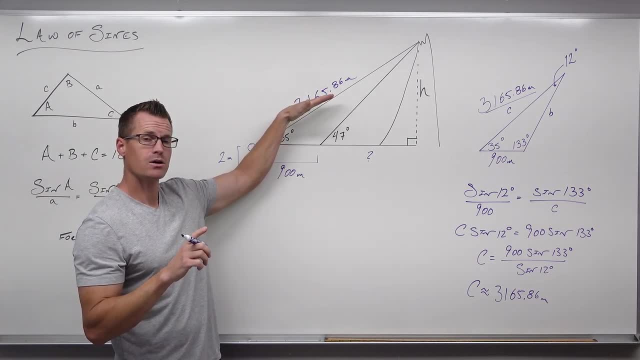 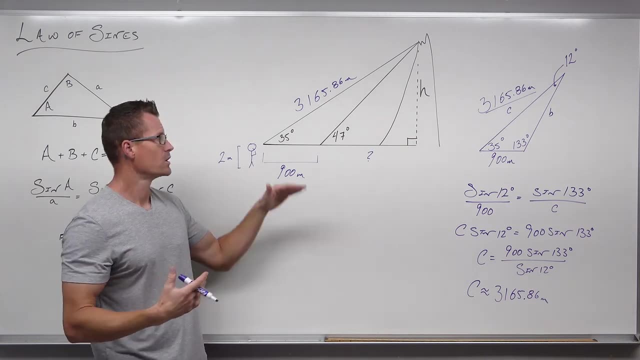 We already knew this was 900, so we found this missing side. Could you have found this missing side? Yes, But in either case you would have gone. You now have this right triangle. You have either 35.. 35 degrees- a height that you want to find- and a hypotenuse. 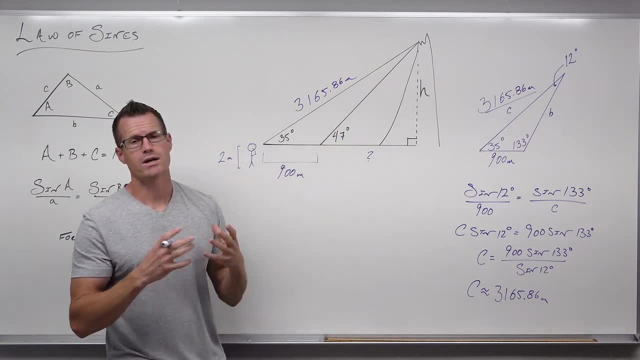 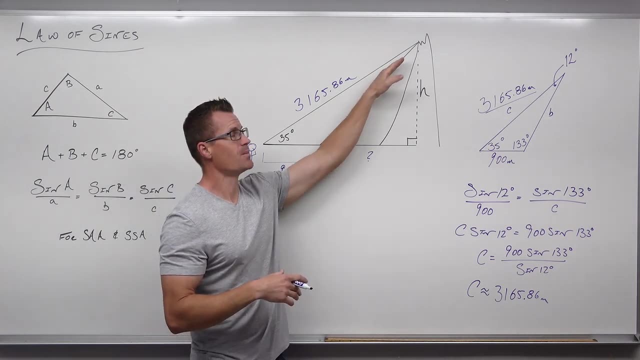 Oh, it's a right triangle Hypotenuse that you know. We can use right triangle trigonometry with the sine function to figure that out. Or if you would have found this side, you would have a hypotenuse that you know. 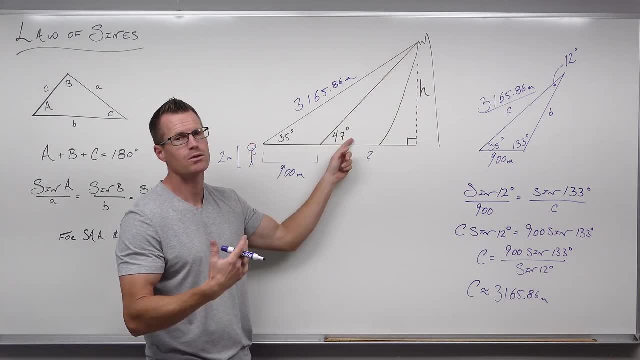 You'd have a height that you want to find and 47 degrees, an angle that you know. You can again use the sine function, but you'll use a different angle and consequently a different hypotenuse Either way. 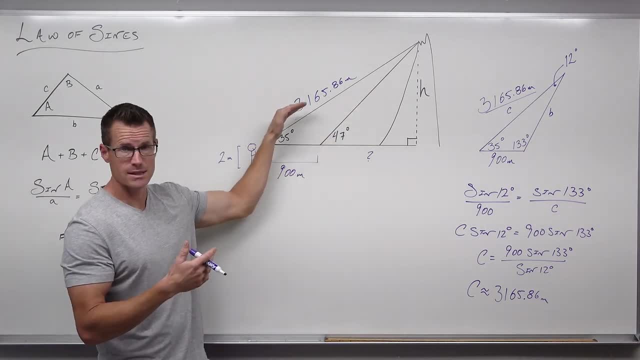 Now, I can't do that one because I don't know that side, I know this side, I know this hypotenuse, So I'm going to label this as: hey, what's the angle that I'm given That angle? 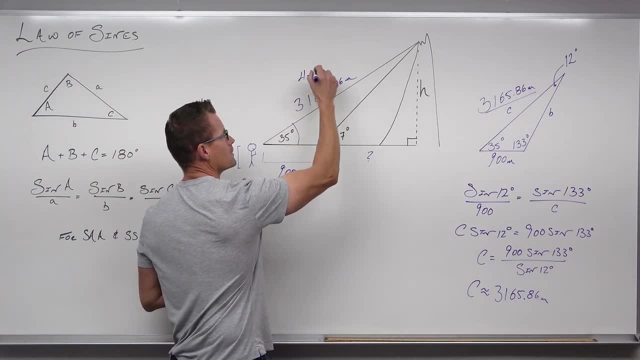 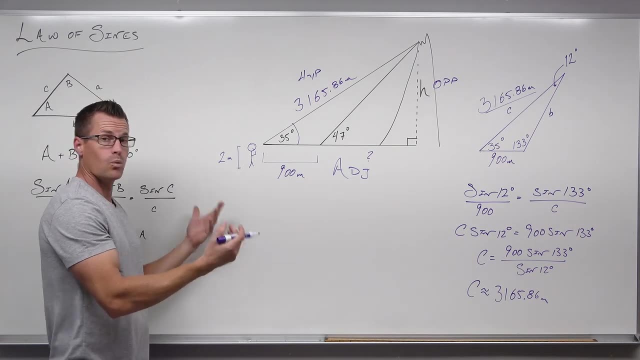 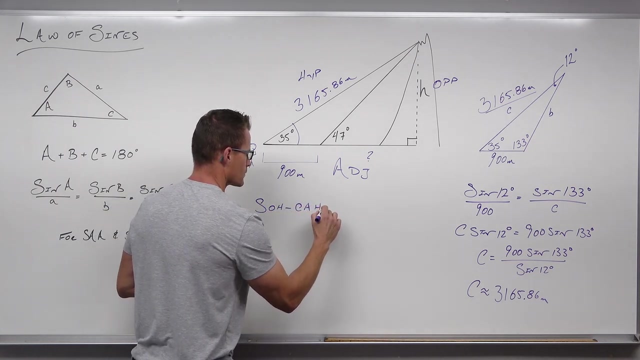 From that angle, label your hypotenuse, your opposite and your adjacent. All right, Well, what do I know? What do I not want to find? don't really care about. In our case, having gone from the angle that I know and the side that I just found, which was our hypotenuse, 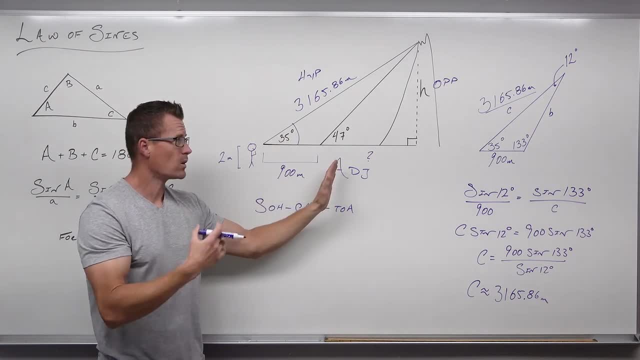 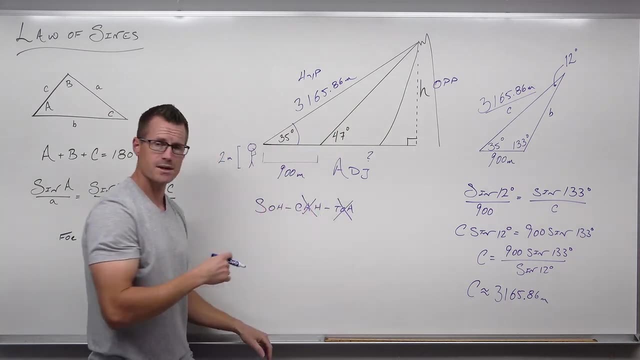 I really don't care about the adjacent side. All I'm really looking for is the opposite, and I've been given the hypotenuse, So adjacent is something that I'm really not concerned about. This says you will be using sine. 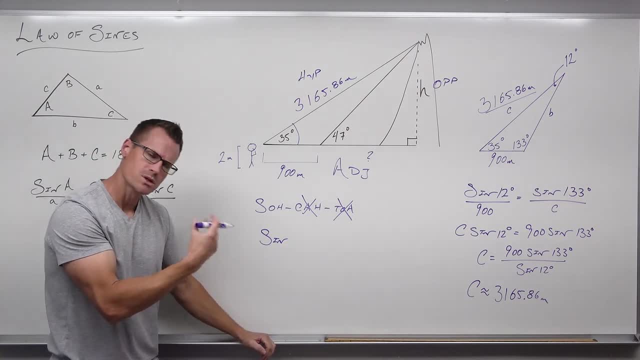 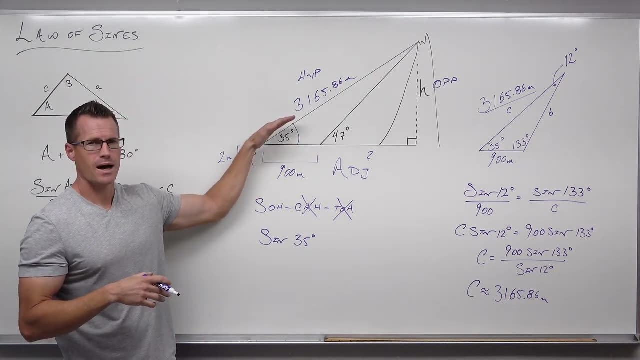 Sine of what? Sine of the angle that you just referenced, which is 35 degrees. Why that one? Why not 47?? It's because you found the hypotenuse for that triangle, the one that had 35 degrees in it. 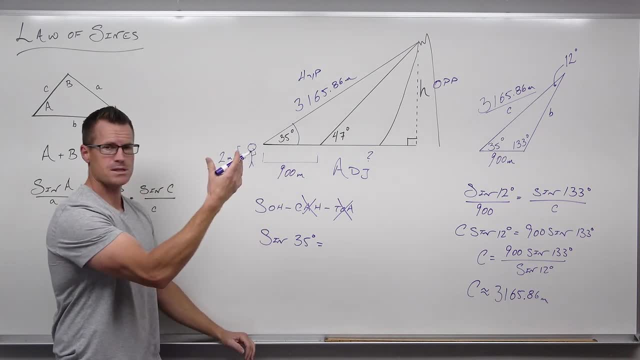 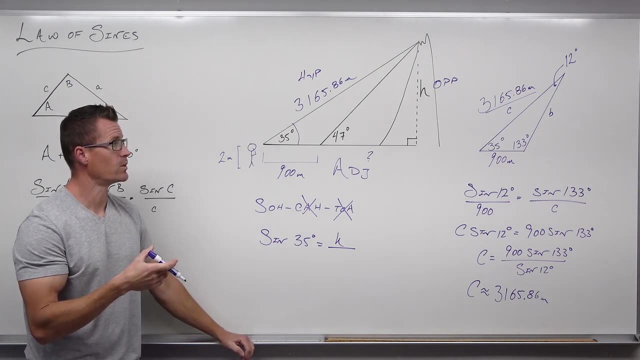 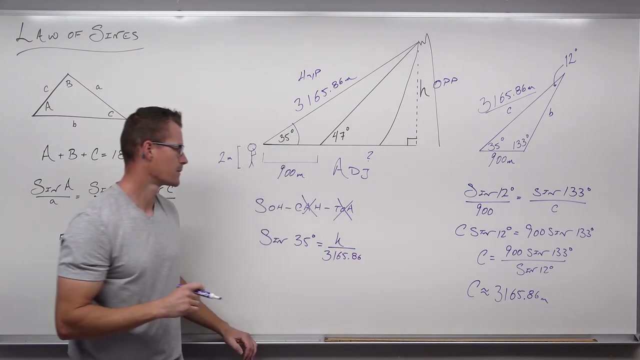 So sine of 35 degrees, Sine of 35 degrees equals opposite. I don't know if it is height over hypotenuse, which is 3,165.68 meters. Keep in mind we try to avoid using rounded numbers if at all possible. 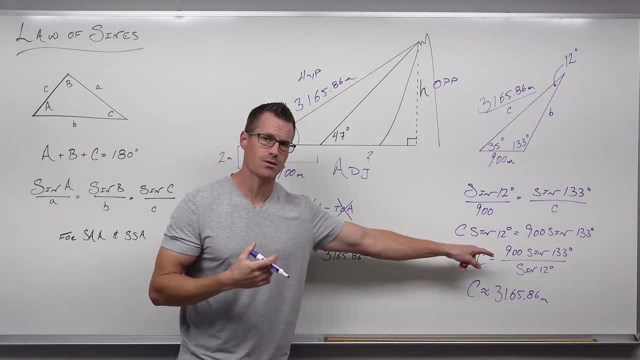 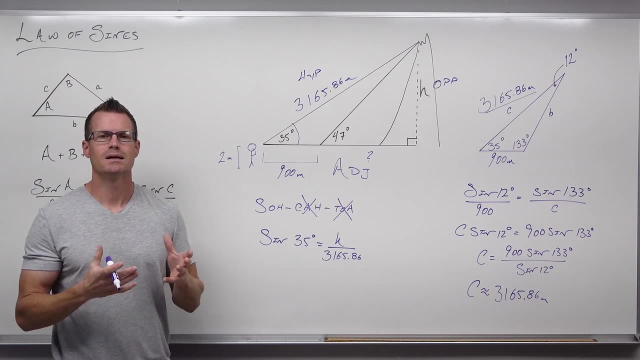 but in this case it's really not avoidable, unless you want to plug in that entire thing. Now, you could do that, You absolutely could, but it just makes our math look pretty, really nasty. Anyway, it's your choice. 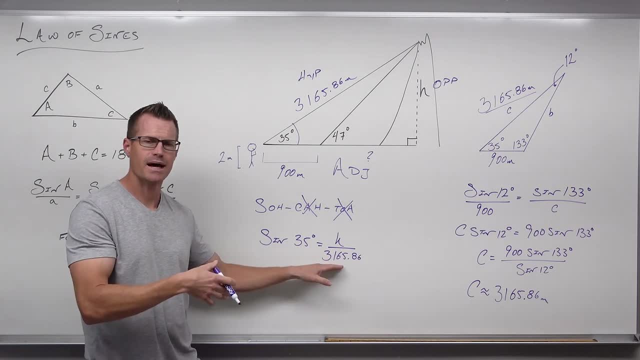 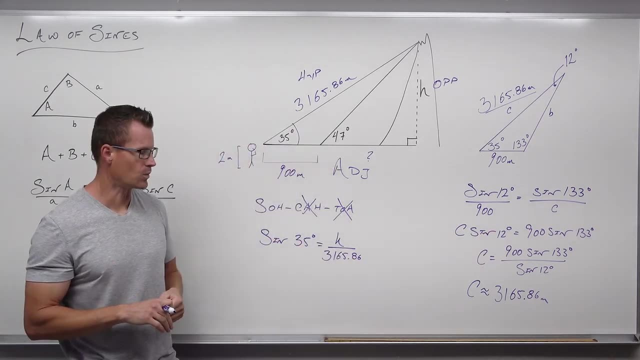 Here I'm rounding and using that because that's what I chose to do, based on the kind of necessity of not using all that junk at one time. You could, but it's your option. So we're going to multiply both sides by 3,165.86.. 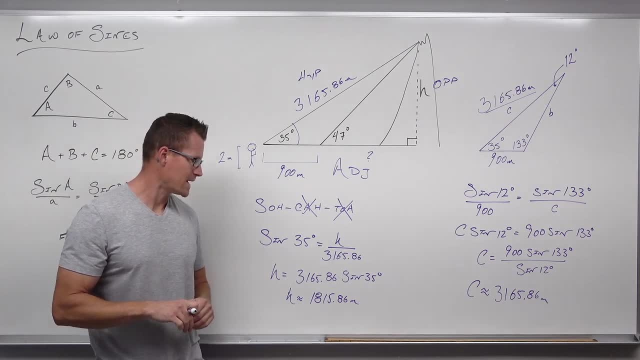 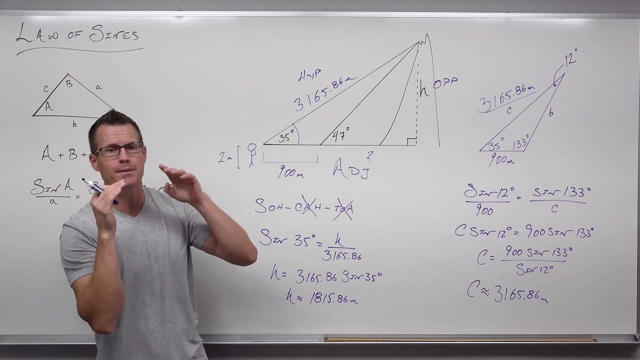 If we do that, if we approximate, we're going to have 1,815.86.. And you're going to look at that and you're going to say, yeah, but remember what you've done. You have a height to you and your face is probably not on the ground looking up at that volcano. 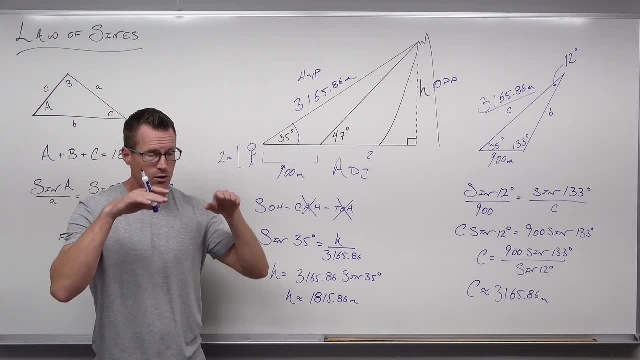 So if it explodes and your face is on the ground, it's going to get burned. So you're looking up from a height of- well, for me it's about 2 meters, So I would have to know what that height is and add that to it.